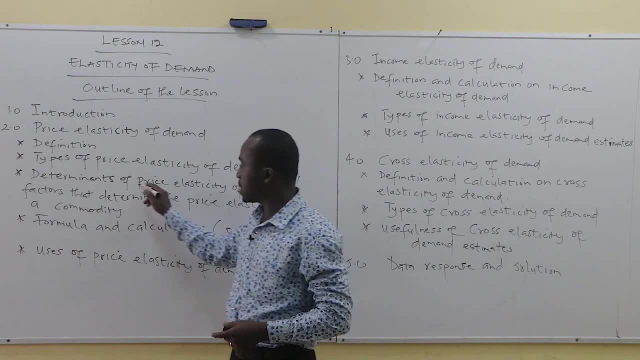 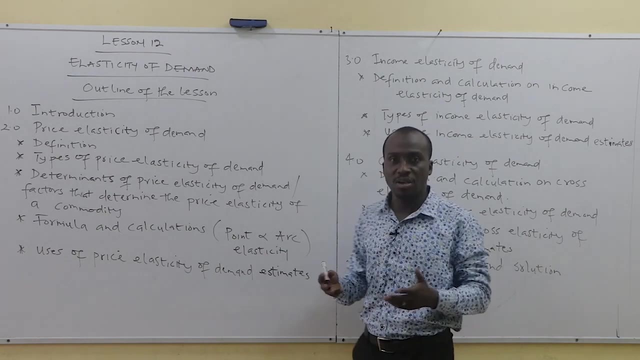 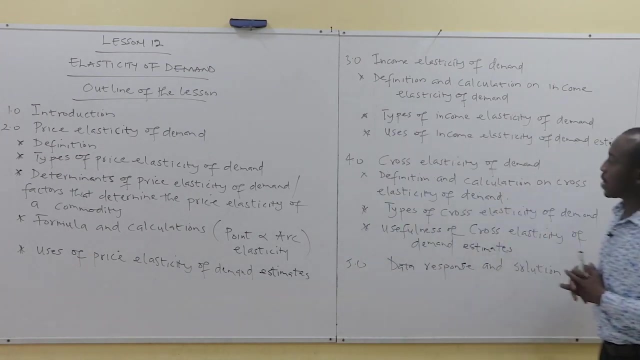 elasticity of demand, the determinants of price elasticity of demand, the factors that determine price elasticity of demand, the formula, the calculations. We got the usefulness of price elasticity of demand right. here, too, you're going to have another type: income loss of demand. you're going to 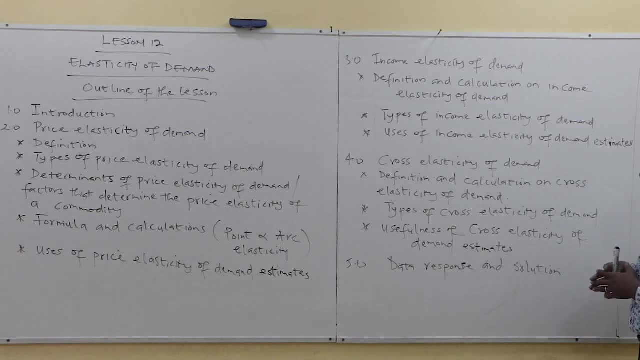 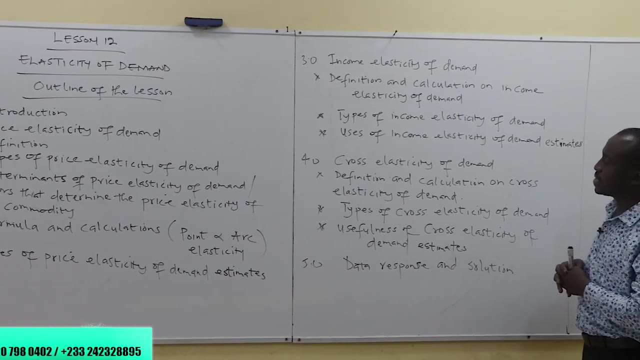 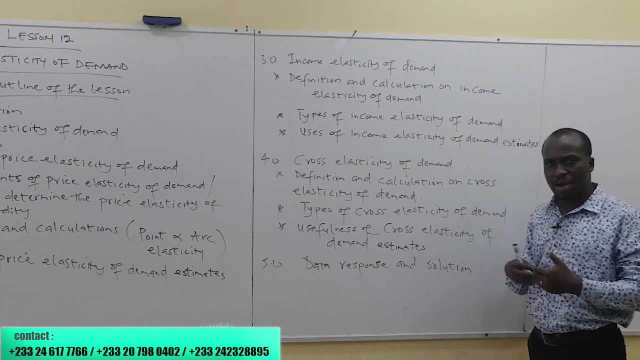 look at the definition, the calculation and the calculations on income analysis of demand, as you can look at the types of income loss of demand and regarding what is the uses, what? why is the why? why is the income elasticity of demand estimates? why is it useful? okay, so you're going to look at the cross last year of demand. you're going to look at the definition. 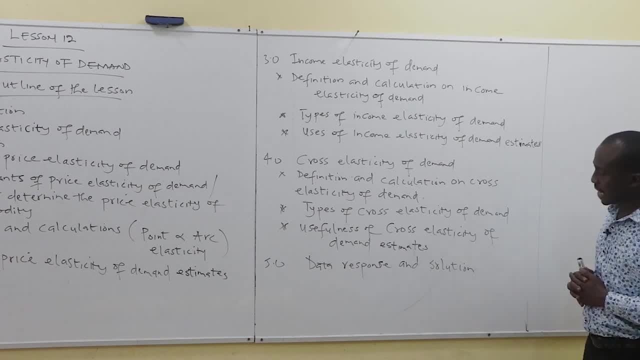 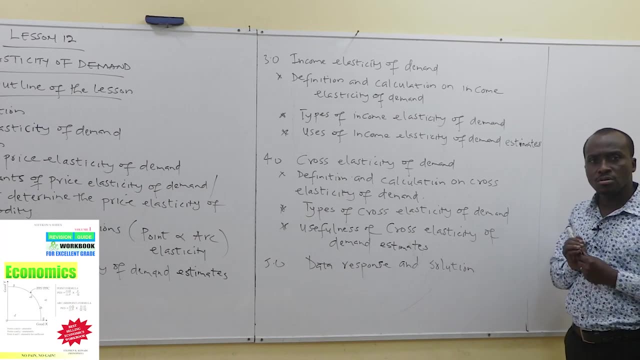 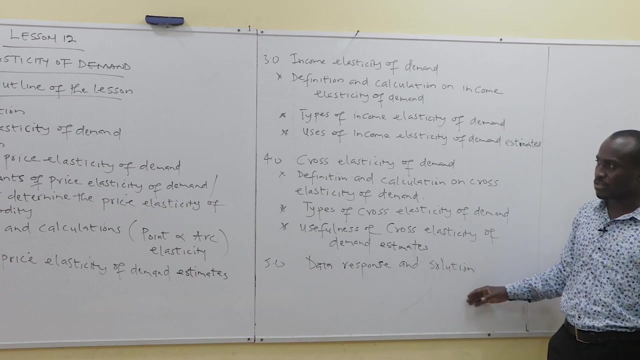 and the calculation of cross last year of demand. you look at the types of cross last year of demand. you're going to find out why is the cross of demand, the estimates, why is it useful? why is it useful? okay, then, after that we will wrap it up with our data response question so that we try to 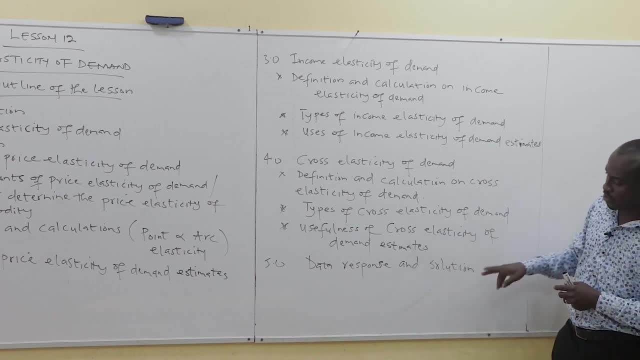 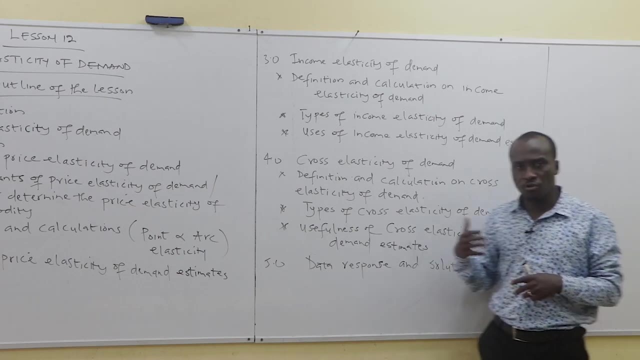 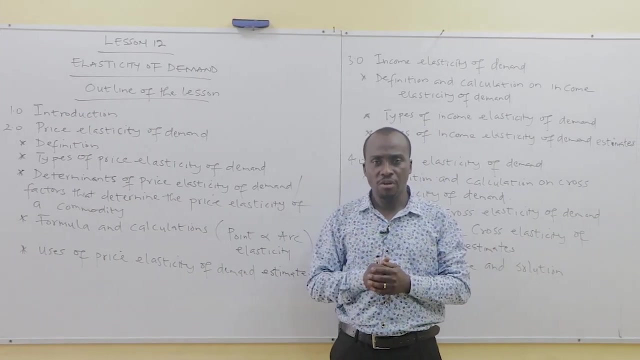 tease out these uh intuitions and concepts to see how we can able to solve our data response question. so i wanted to. it's a very lengthy lesson. i want you to follow it very, very well. we go through all these things and understand these little gritties that bothers on these topics very extensively. it's a very 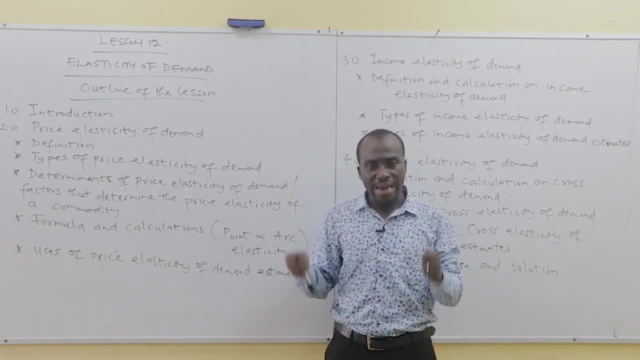 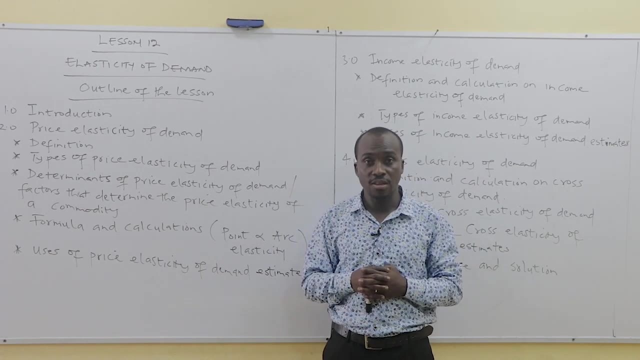 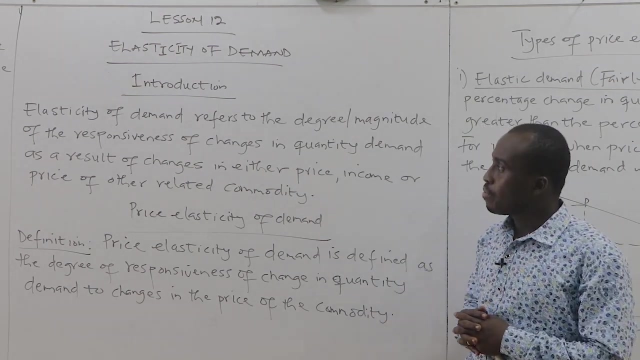 important topic, not only for the classroom, not only for the white exams. it's also even the knowledge for your private life. everyday private life is also very important. so follow this lesson very closely. so we want to look at first, we want to look at the elasticity of demand. before that we 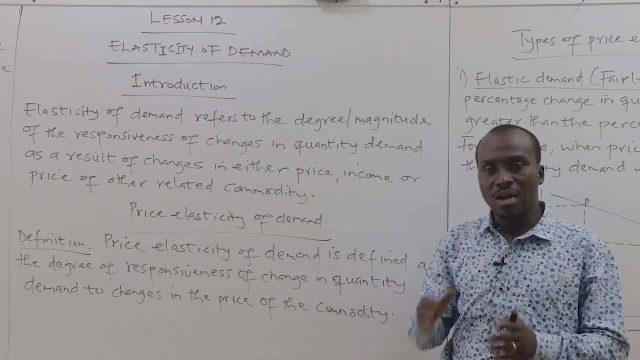 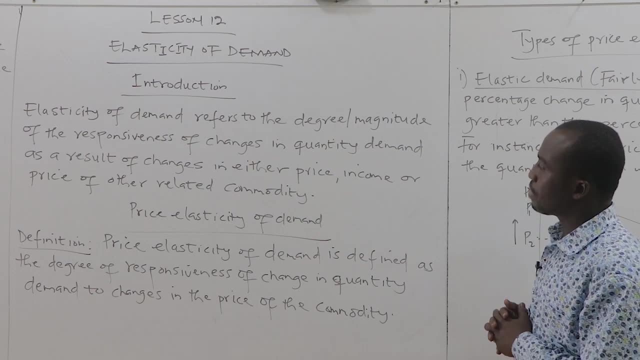 look at what is the general idea when it comes to last year of demand, before you go down to the three types of elasticities. so what's the last of demand refers to the degree or the magnitude of the responsiveness of changes in quantity demand a result of changes in either price. 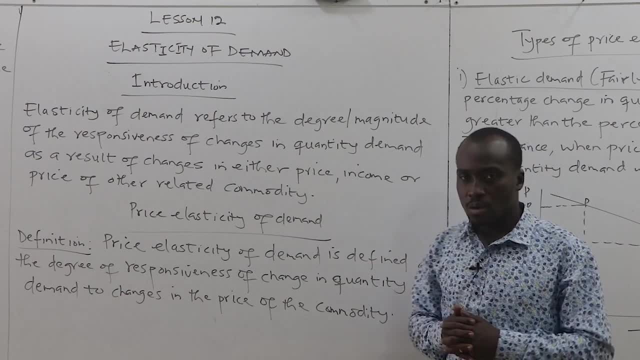 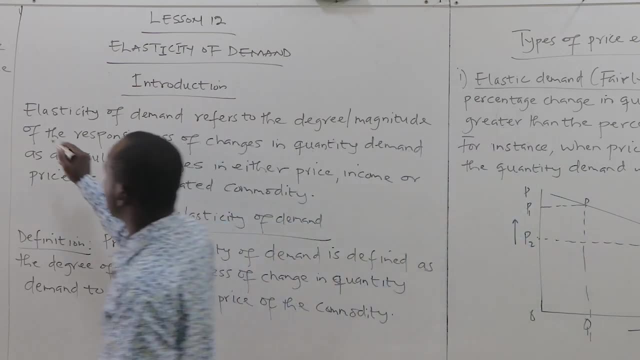 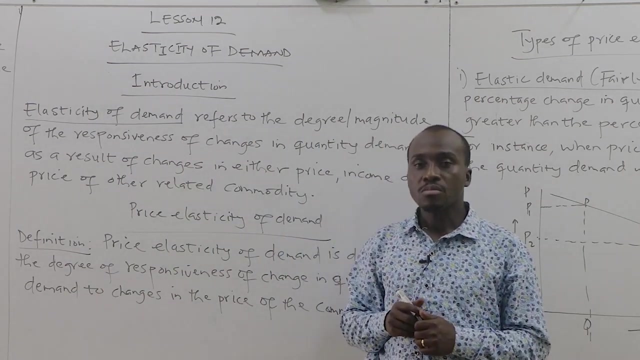 income or price of related commodity. so when you say price loss of demand, what does it refer to? when you say elasticity of demand- here our emphasis is on elasticity of demand. before we come back and take the types and explain them one by one, it basically means that it shows the 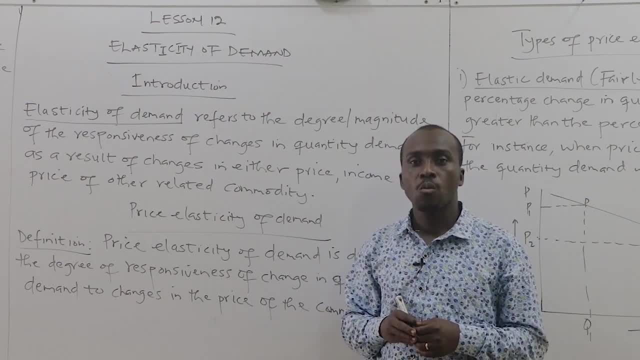 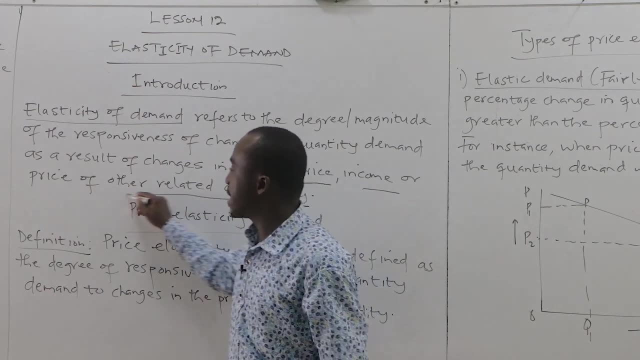 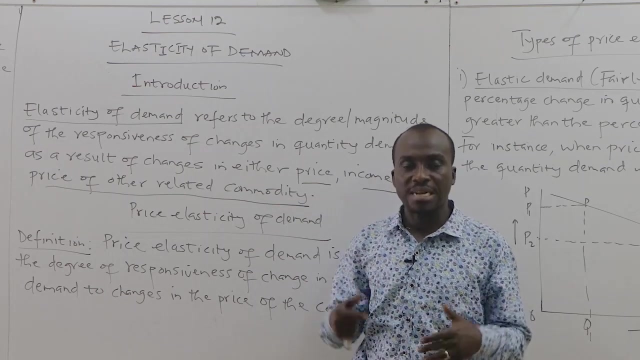 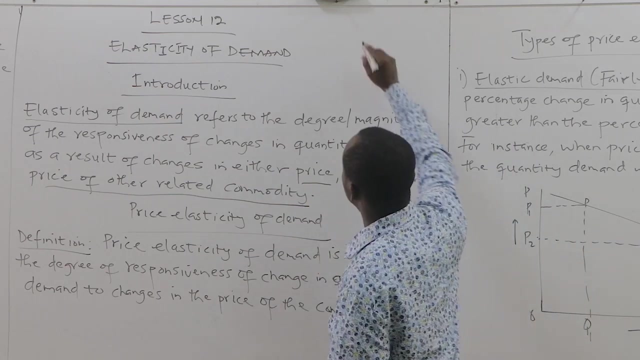 thing to which demand changes whenever there's a change in either price of the commodity income or price of related products. remember, in lesson four, four, eleven, lesson seven, we spoke about factor that influenced demand. in this lesson we want to find out. let's take, for instance, price. we know that whenever price goes up, quantity demand falls right. that one we know it. 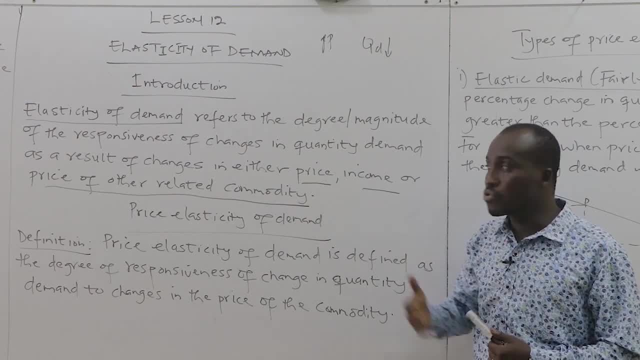 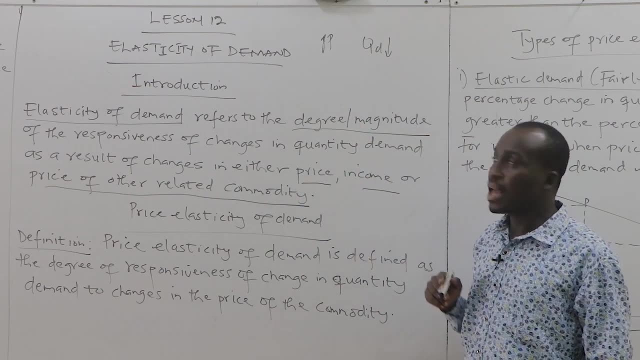 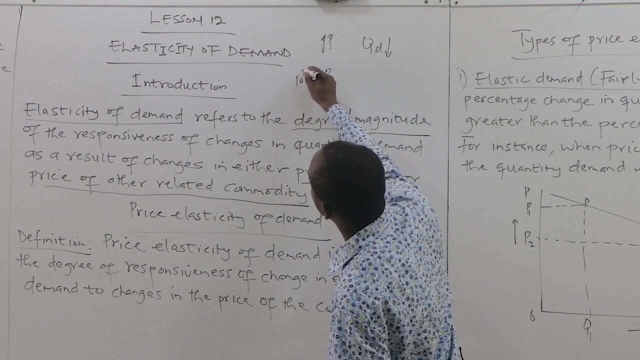 but we don't know the magnitude, the percentage, the degree. so the elasticity of demand tells us the magnitude or the degree. for instance, if price goes up by maybe 10 percent, if price increased by 10 percent, demand will fall. demand will fall by a horse. demand of former may be 20. 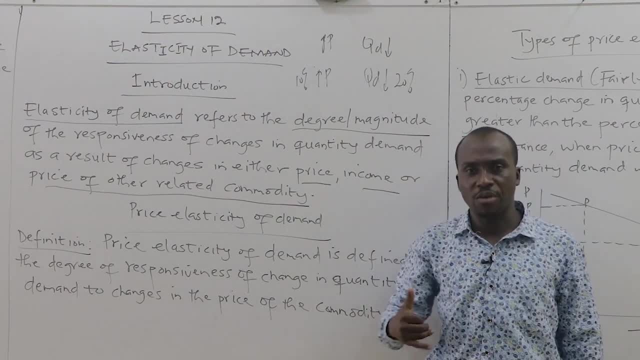 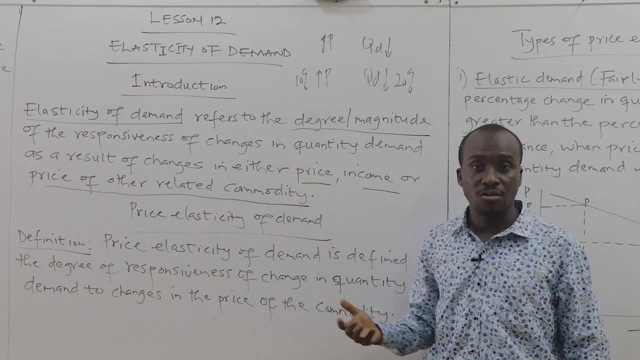 right. so in this lesson we are trying to be more specific. one is not a magnitude by which- price and demand, for when we're treating demand, all that, we've got to know that whenever price goes up, demand or fall, when price goes down, demand will go up. that was. 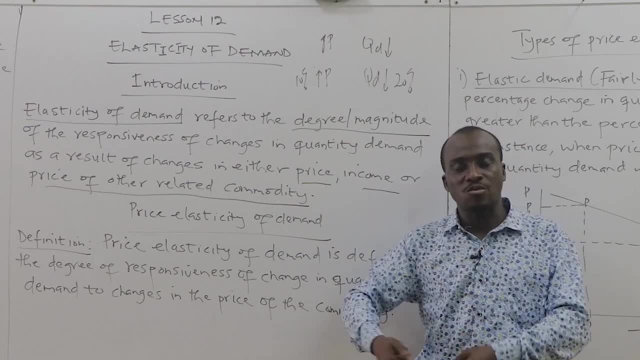 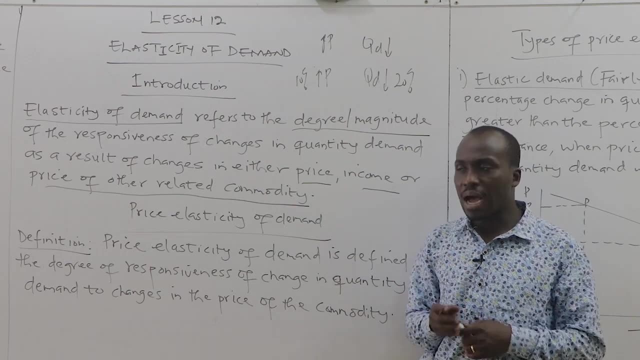 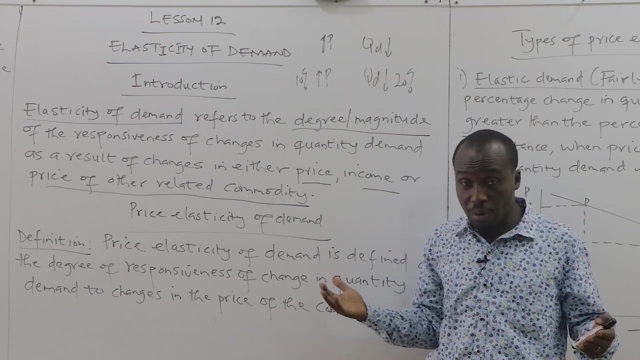 all. but we didn't know the magnitude, the stent to which it would change. it will only change by 30 or 20 percent or 50. didn't know that right. so this topic is giving us more information than what we did on demand. it's just a build up. if, for instance, you have two consumers, consumer a and b, if the price of 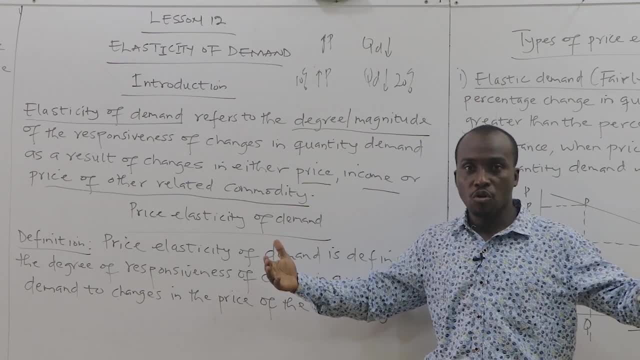 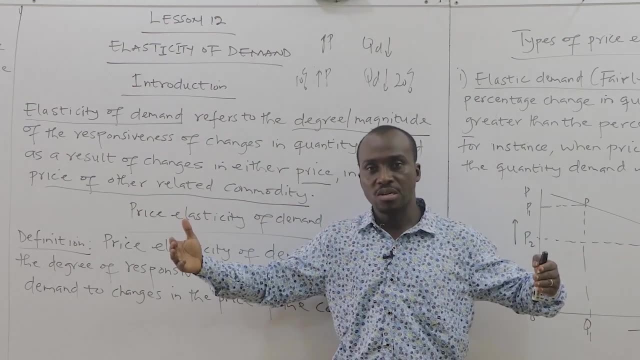 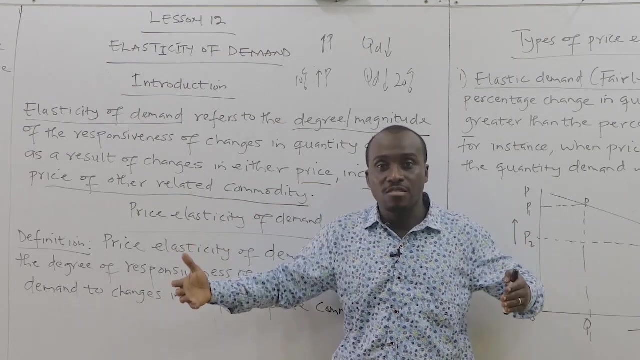 a product you are selling goes up by 10 percent, right, maybe because my a will increase its consumption by maybe 30 percent, because my b will increase consumption by 40 percent. so when price goes down, these two consumers are increasing their demand. but now we know the magnitude. it's not just. 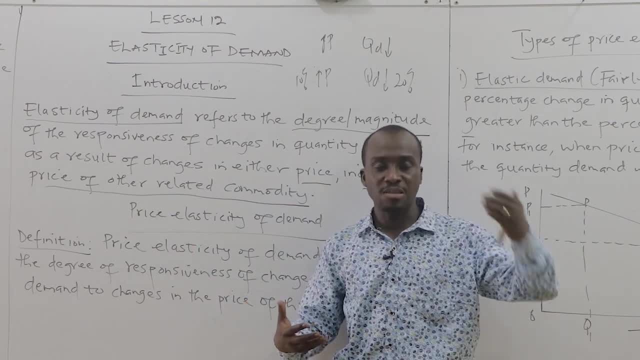 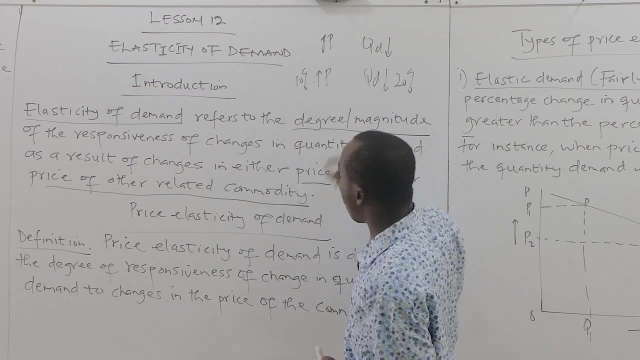 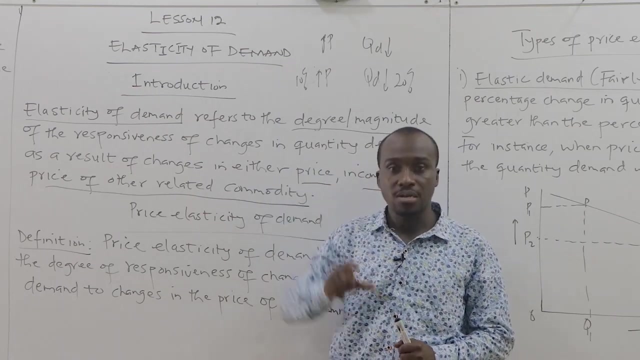 saying they will increase the demand, but we know the magnitude: a will increase demand by 30 percent, b will increase demand by 40 percent, and that's what elasticity is about. it's the degree or the magnitude. it's telling you the extent. by what magnitude will you change your demand, will you? 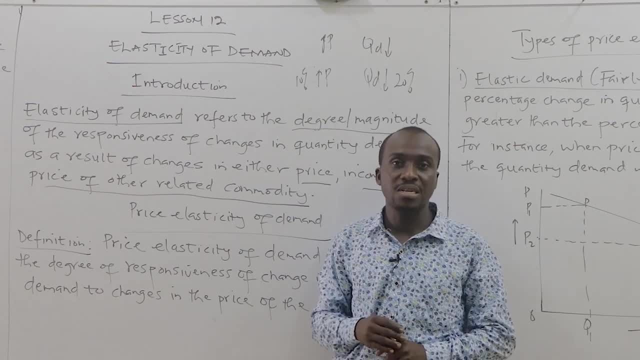 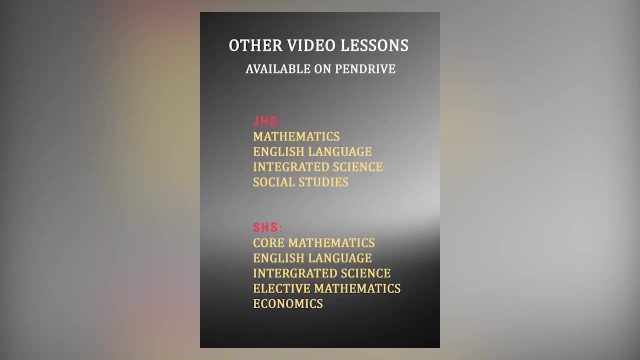 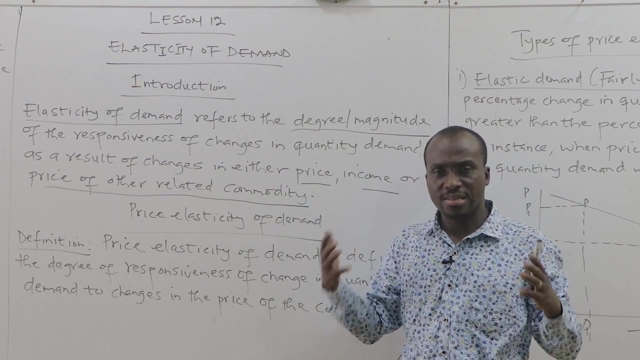 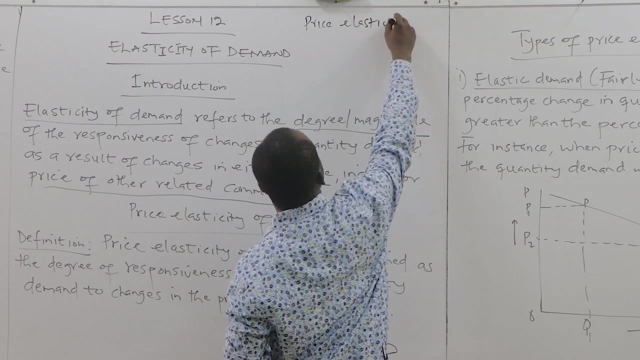 change it by 50, 80, 100, 20, so that we can now tell you the true story of what is going on. when we talk about elasticity of demand, there are three categories, three types of classes of demand. one: we have the price elasticity of demand. 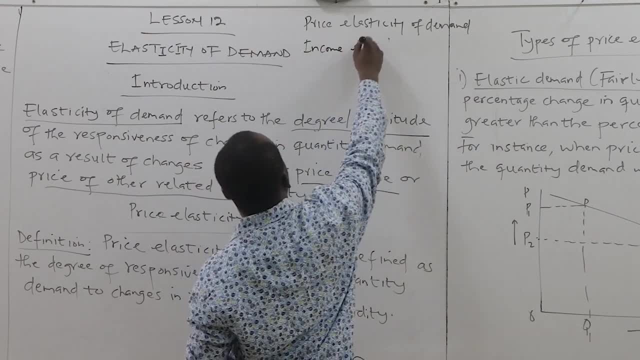 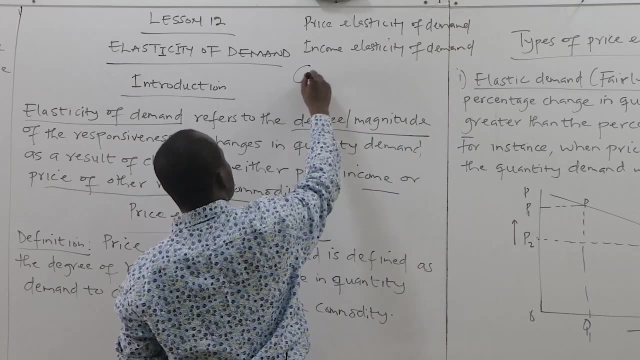 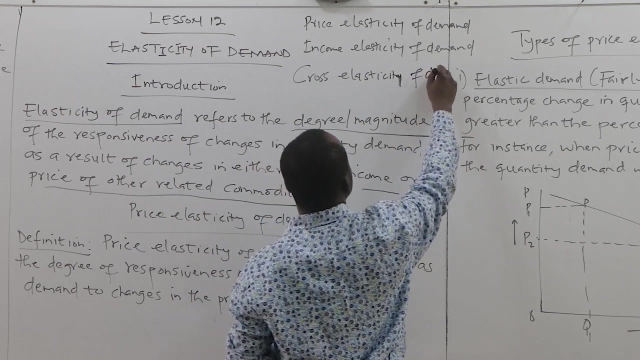 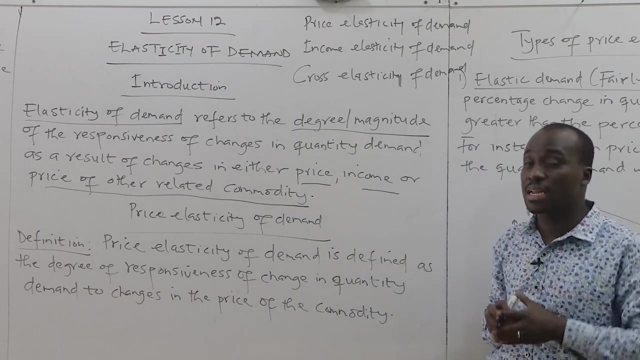 we have the income elasticity of demand. we have the cross elasticity of demand. we have all these three types of velocity. so the elasticity of demand, we have three types. you're going to take them one by one, solve questions and understand all the concepts. we have the price. 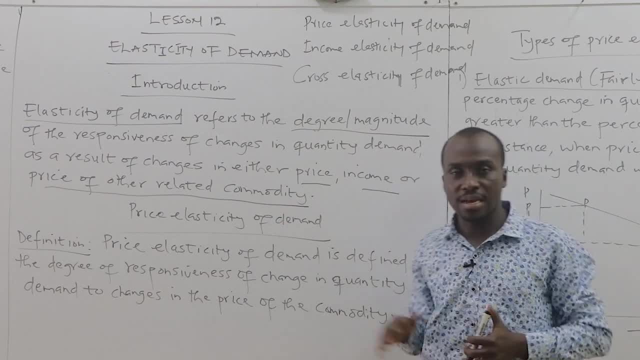 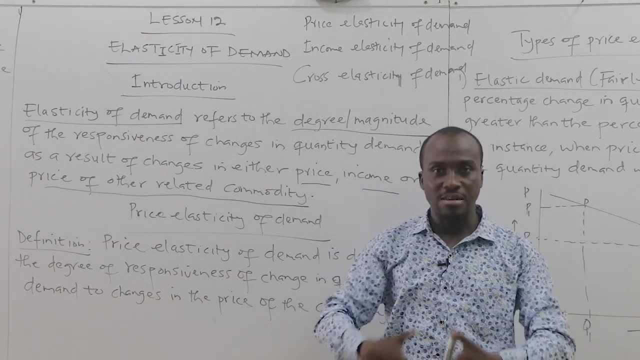 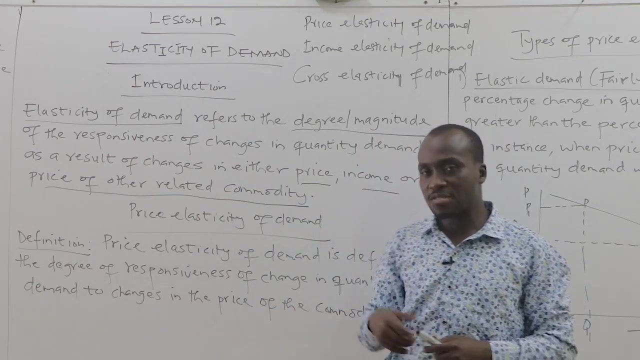 elasticity of demand. we have the income largest of demand and across last of demand. so elasticity itself is a broad topic that tells you how consumers change the quantity they buy whenever there's a change in price, other price, income or price of related commodity. so first, so we are not going to take the first type, which is called 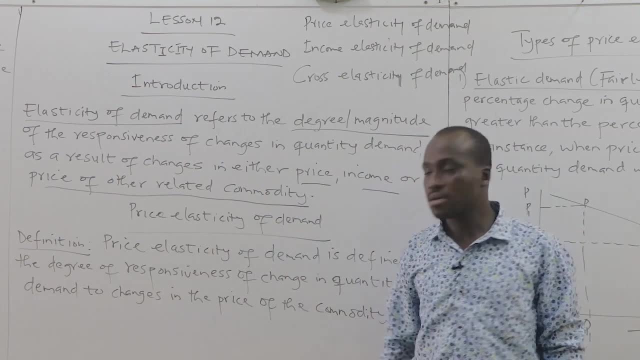 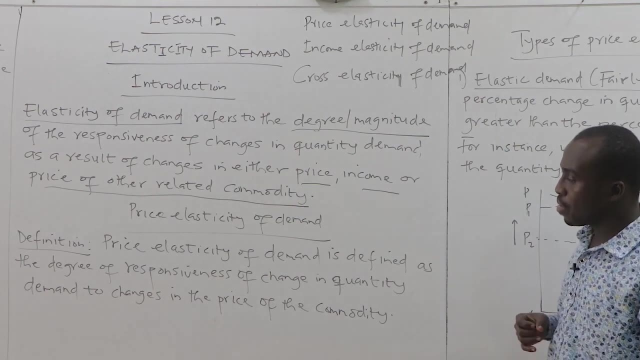 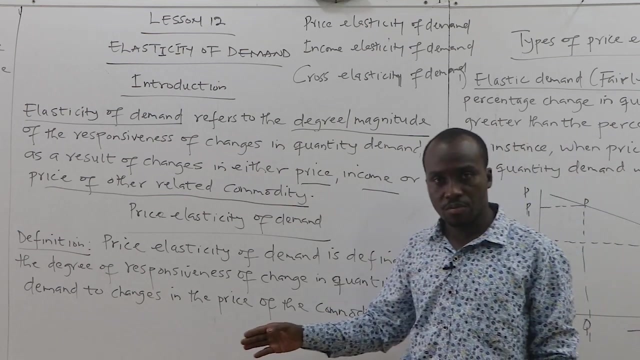 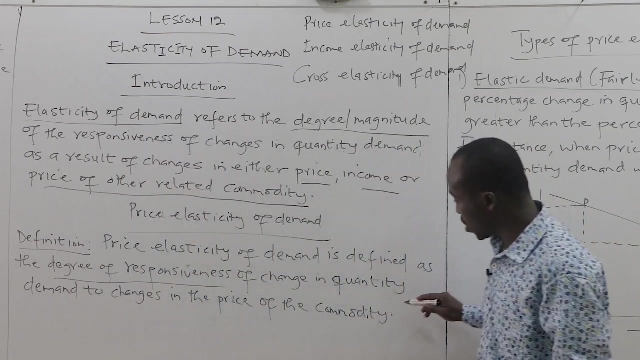 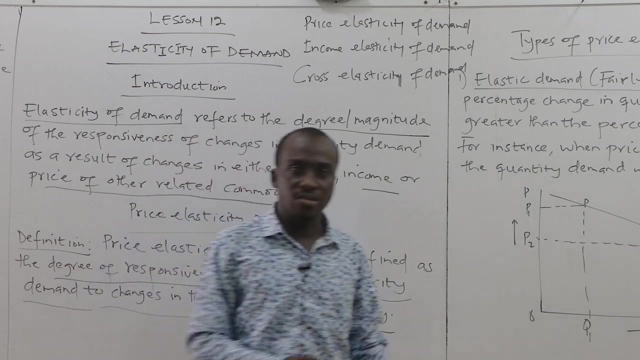 the price elasticity of demand. okay, so price velocity of demand is defined as the degree of responsiveness of changes in quantity demand to changes in the price of the commodity. so it talks about what, the degree of what responsiveness to which consumers would change the quantity they demand when there's a change in what price keywords. so 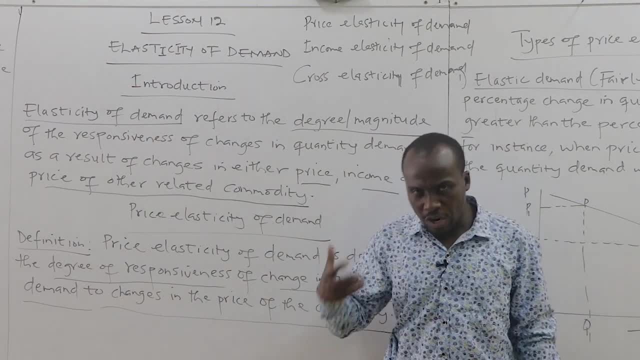 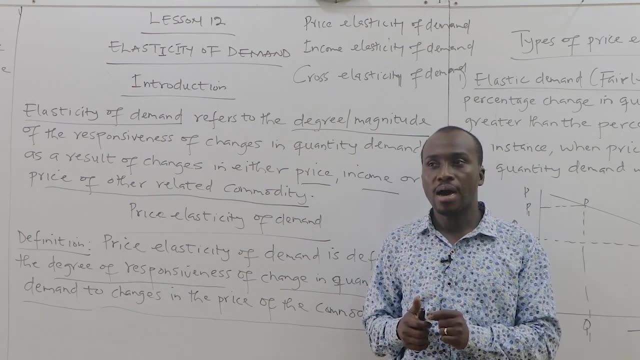 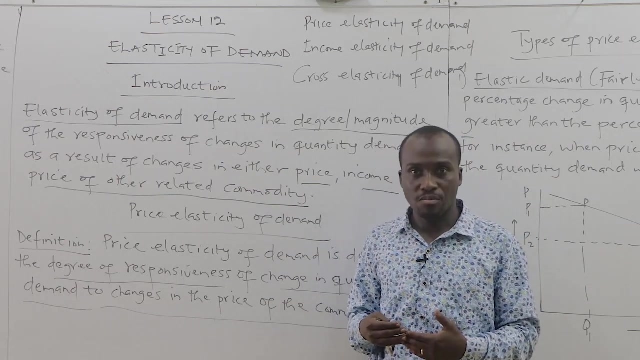 it talks about the degree of responsibility, the degree to which consumers would change the quantity they are demanding whenever they change in price. and, as i was explaining to you, uh, when we're dealing with the concert on demand, we got to understand that whenever price goes up, consumers buy less right, but we didn't know the magnitude. 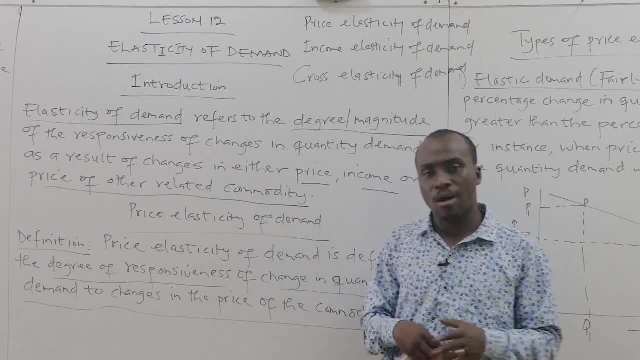 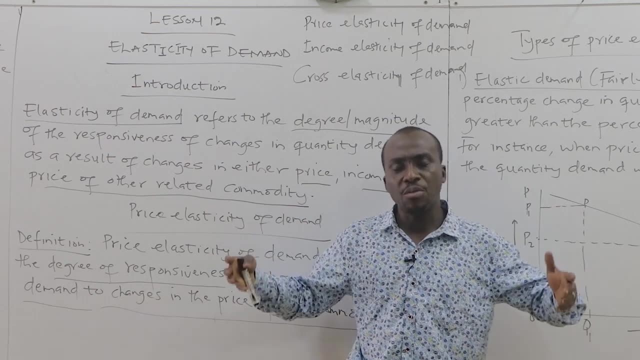 that maybe if price goes up, consumers will buy less. they'll buy less by what magnitude? maybe if you have two consumers, consumer a and b. if the price goes up, consumer a will buy less, but maybe 50 percent. consumer b will buy less, but maybe 40 percent. so even though they are all demanding less, 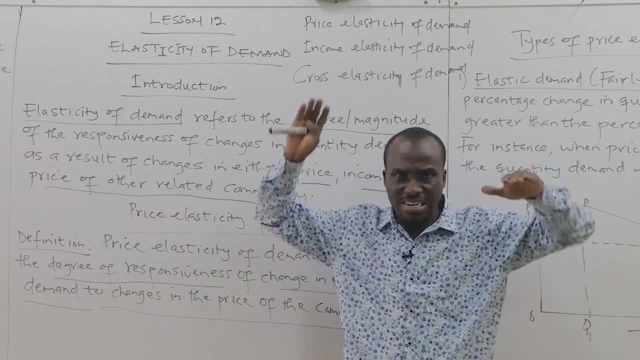 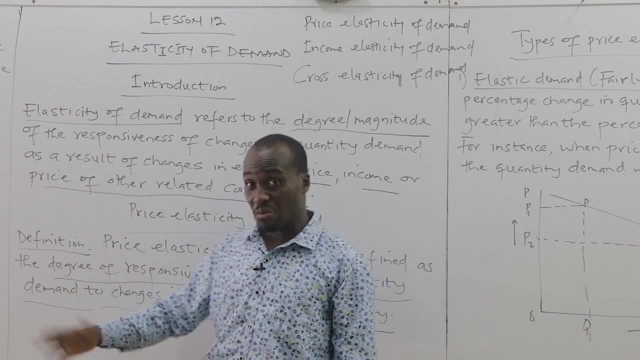 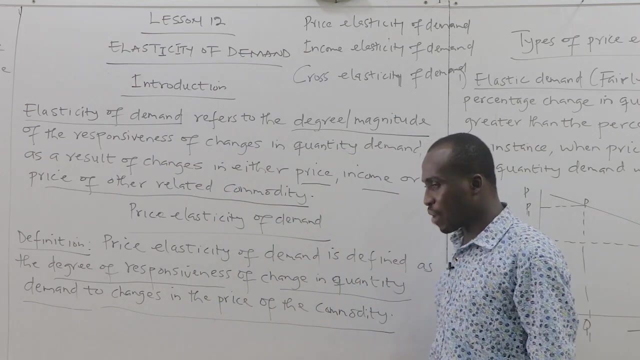 the magnitude is different. the degree, the magnitude, the percentage. so it's a percentage. so people say that is a degree or is the magnitude, or people say the percentage is the degree of response. how does your demand response to change in price if price increased by 10 percent? 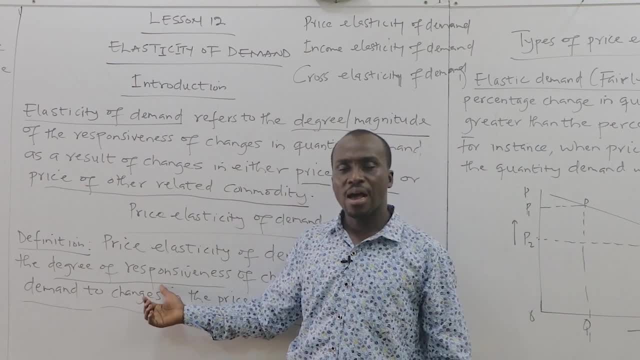 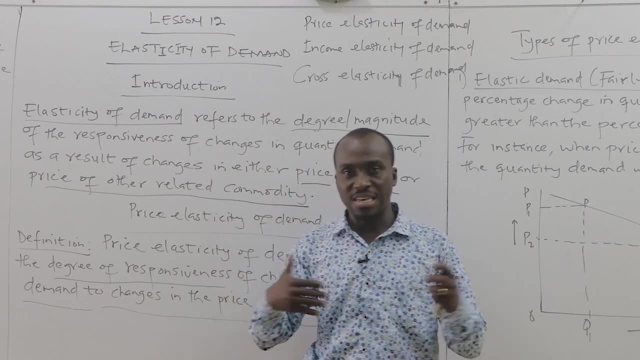 how will your demand response? will your demand increase by uh? will your demand fall by 40 percent? or your demand will fall by 80 percent, or your demand will fall by 100 percent. so we see the different degrees, or to which a consumer's change in quantity demand response to change in price. 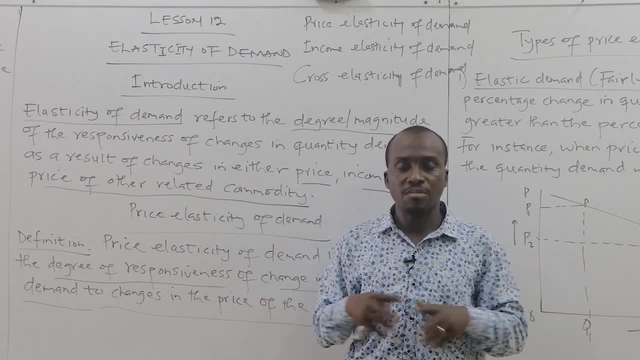 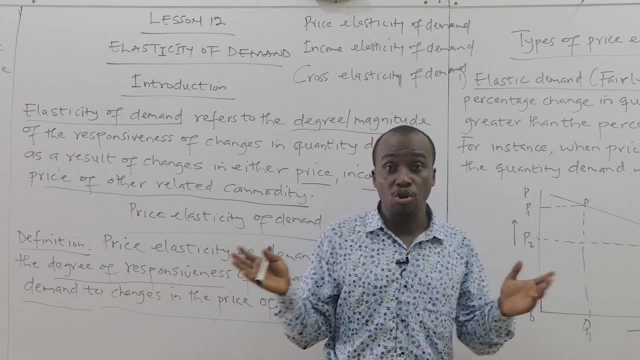 so just try to think about it when you go to the mall and something you buy in the market, the price have gone up by 10 or 20 cents. this 10 or 20 percent? it have gone up by 20 percent. what do you do? are you going to decrease? 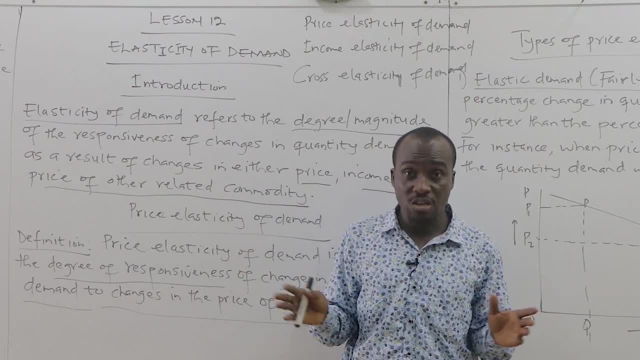 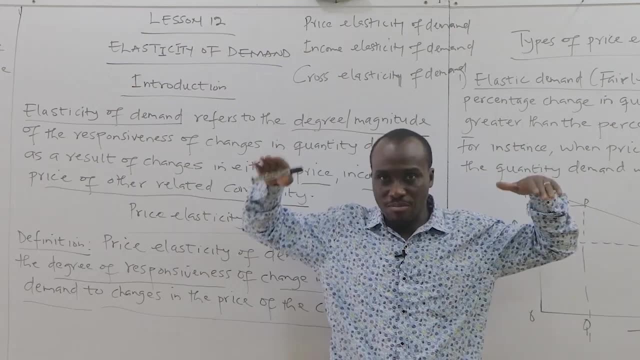 the demand by 10 percent or 5 percent, or 10 or 2 percent, nobody knows. if you are taking two consumers, maybe you reduce those by 15 percent, somebody reduces on by 5 percent. so that's where the elasticity comes, in different degrees, different magnitude to which consumers will change their 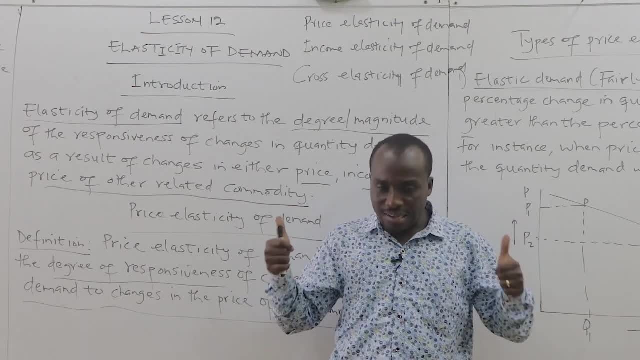 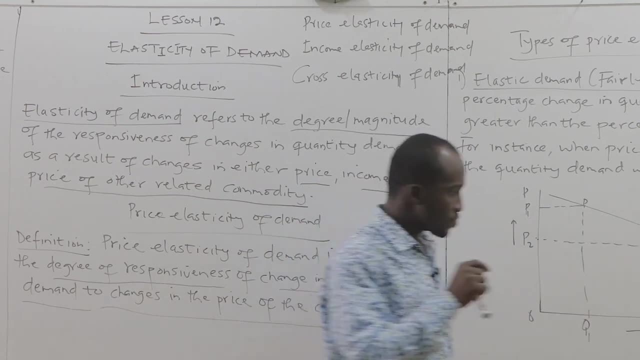 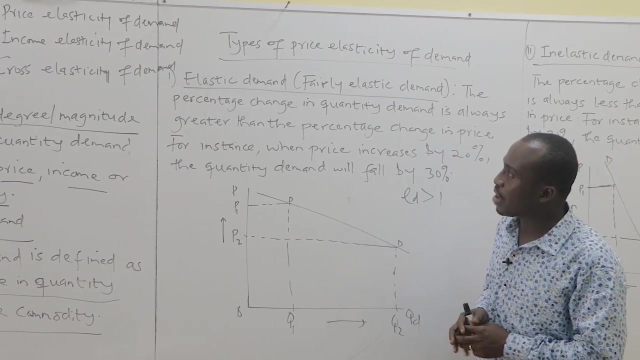 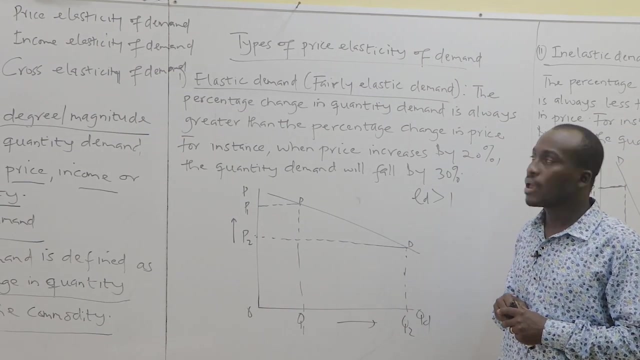 demand whenever price increases. so let's go down and know more things about elasticity, price elasticity of demand. we have five types of price elasticity of demand. we have the first type. we have the elastic demand, or what we call fairly elastic demand. what does it mean? it means that the percentage change in quantity demand by consumers is always greater than the percentage change in the price. for, For example, when price increase by 20%, the quantity demand will fall by 30% With elastic demand. when you say commodities have elastic demand, it means that any time price changes. 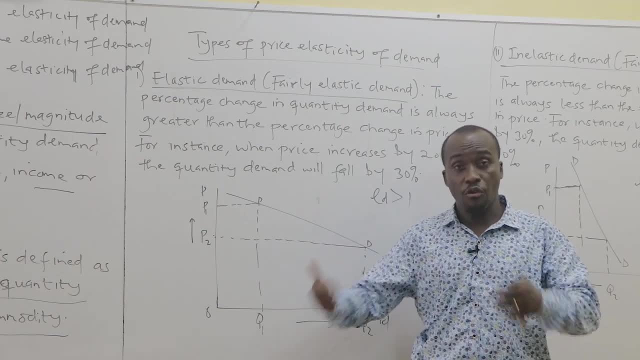 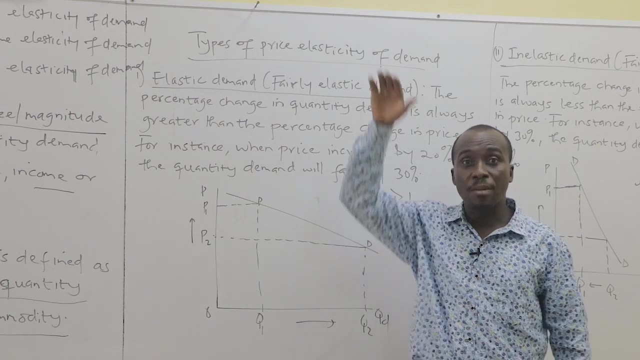 the change in quantity. demand is always greater than the change in price. For instance, you are buying wheat. you went and the price of wheat have gone up by 10%. Then you reduce the amount you are buying by 30%, Or the price has reduced by 5%. 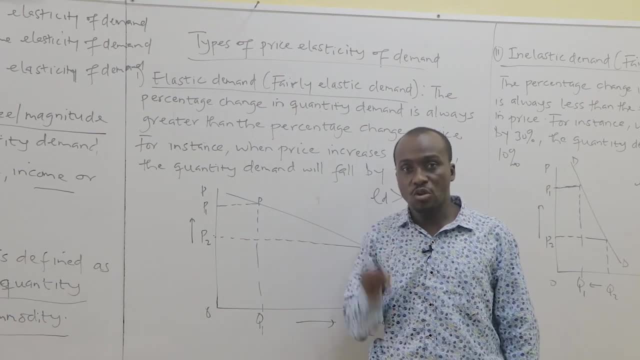 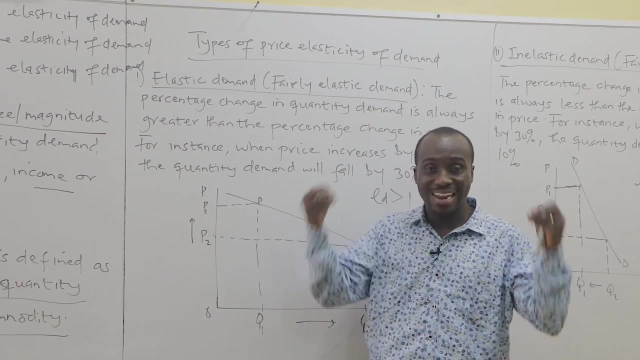 Then you increase the amount you are buying by 40%. That means your demand for wheat, you the consumer, your demand for wheat is elastic. So when we say a commodity you buy has elastic demand, it means that the commodity is very sensitive to changes in price. 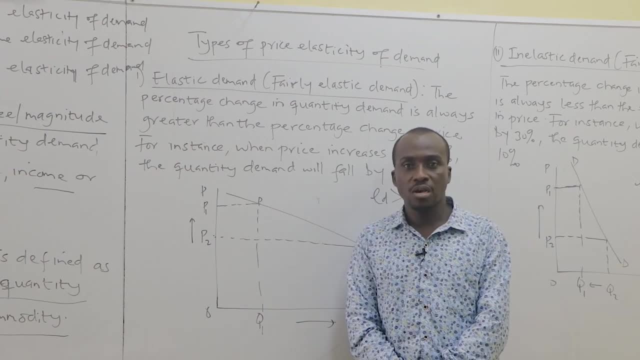 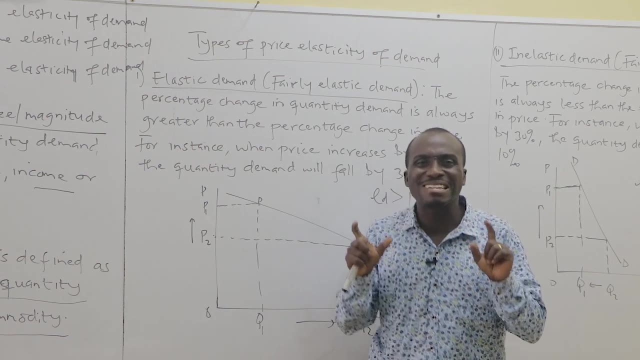 Maybe you buy, maybe wheat, or maybe you buy cornflakes and you discover that the product has elastic demand. What does it mean? It means that the commodity is very, very sensitive to changes in price. So if price increase by a small margin, 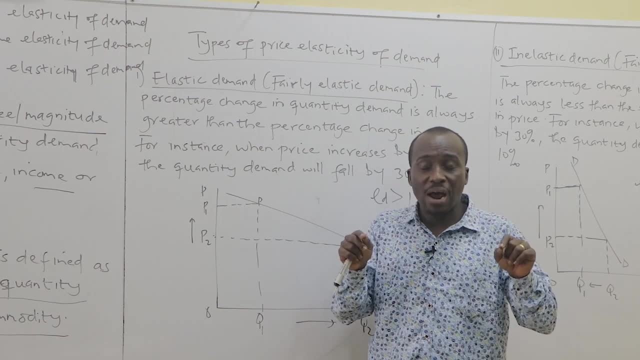 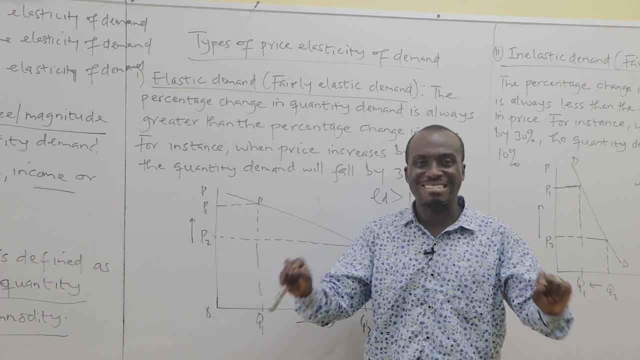 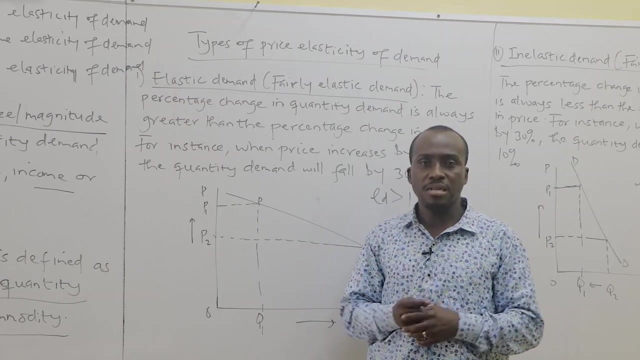 a lot of people will stop buying the product. If the price decrease by a small margin, a lot of people will come and buy the product. That means that the commodity is highly sensitive. The slightest changes in price brings about a large change in the demand. 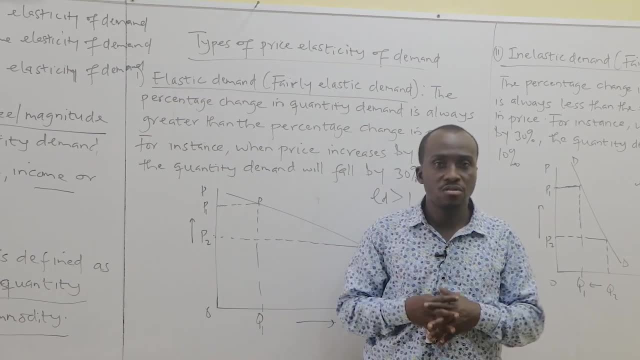 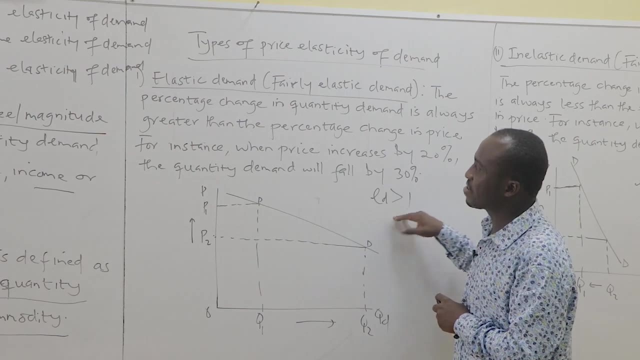 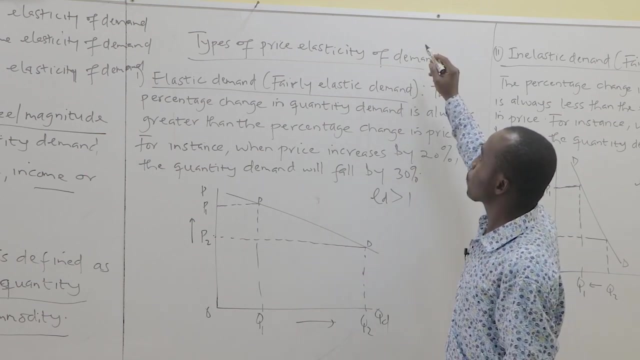 The demand can either increase or decrease. So when you say a commodity have that type of elastic demand, it means that it has elastic greater than one. For instance, let's take maybe you are buying two products. You're buying, let's say, the COVID-19,. 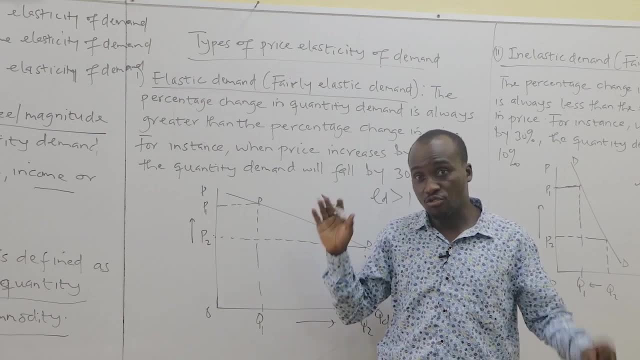 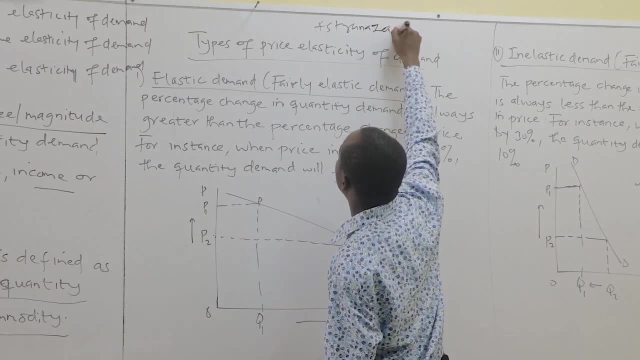 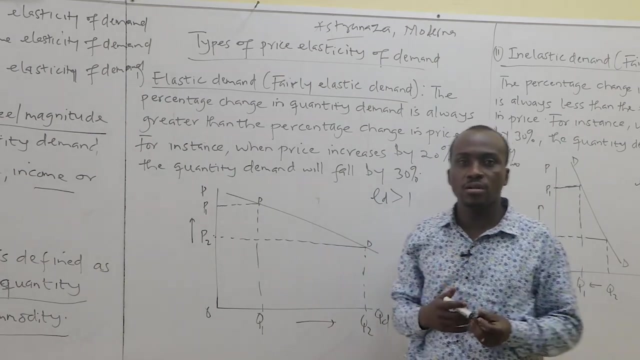 let's look at the vaccines that we have on board: COVID-19, let's assume, Let's take this AstraZeneca and Moderna. Let's take these two. they are perfect substitute, Assuming that a country want to go and buy these vaccines. If the country goes and the price of Moderna have increased by maybe 5%, they will reduce because they are substitute. what would they do? They reduce their demand for this by a large margin, Maybe if price increase of Moderna increase by 5%. 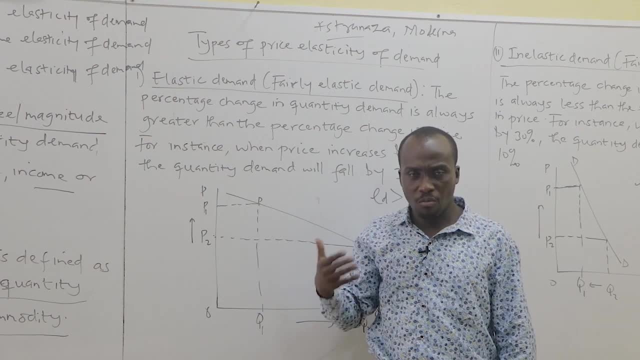 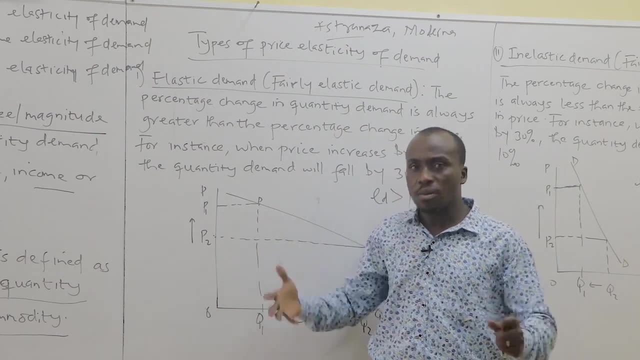 probably they will reduce their consumption or demand for Moderna by maybe 50% And shift that money to go and buy more of AstraZeneca right. So commodities that have substitute behave that way. The slightest increase in the price of one 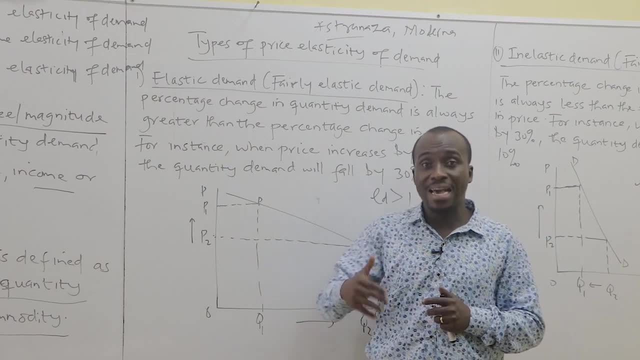 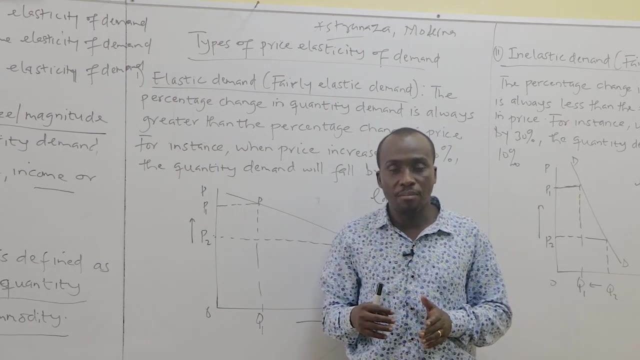 will lead to a large change in that commodity, because the commodity has substitute. Every president- and close up, is on the market. They are all five, five cities And you go to a president that have grown up by five to six cities, A lot of people will shift their demand from president. 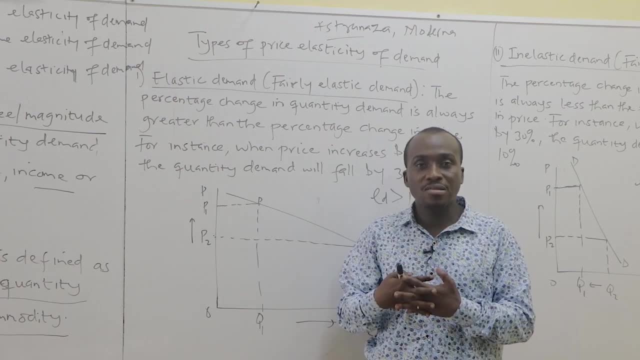 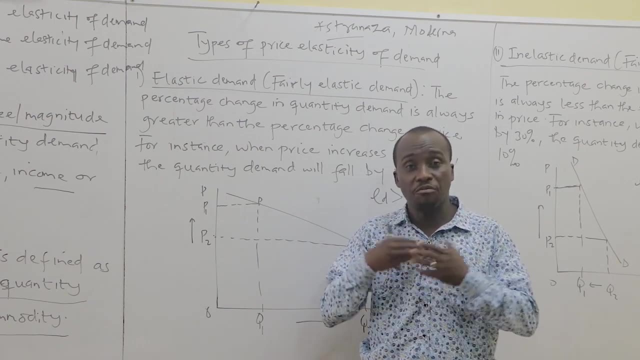 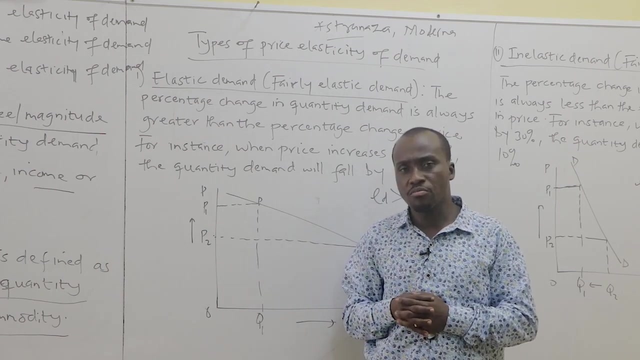 and go and buy closer. That means that a small change in price- if the price of president increase by even 10%, it's possible demand will fall by maybe more than 40 or 50%. That means that the demand for president is very sensitive to changes in price. 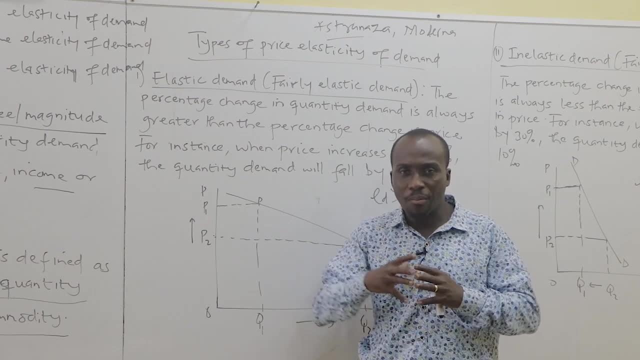 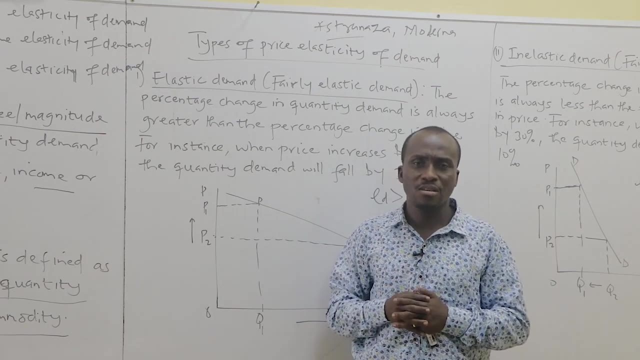 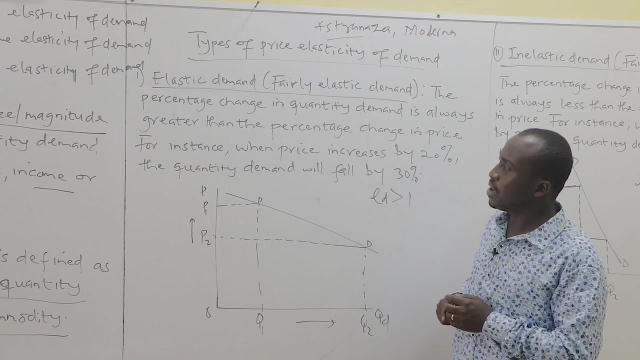 Where, if price increase or fall by a small margin, it brings about a large change in the demand. Later we're going to look at what are some of the factors that cause this When we are finished talking about these types of elasticity. So the elastic demand, or what we call fairly elastic demand. 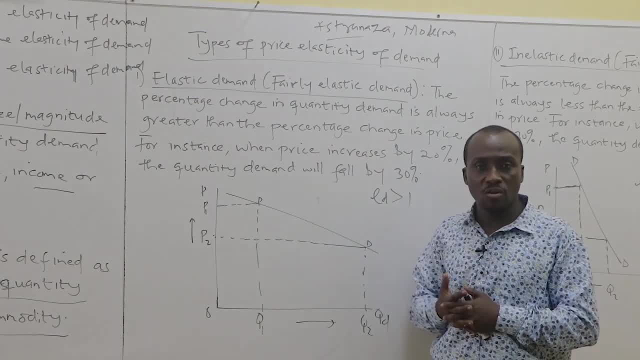 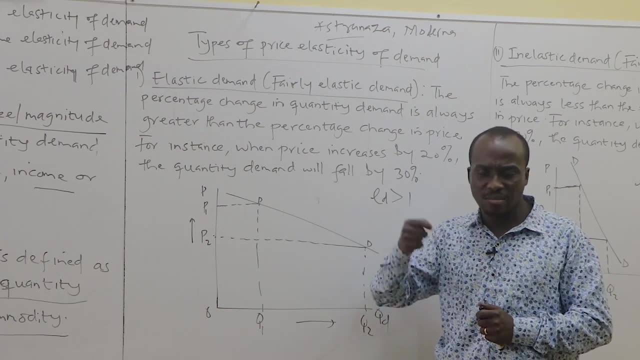 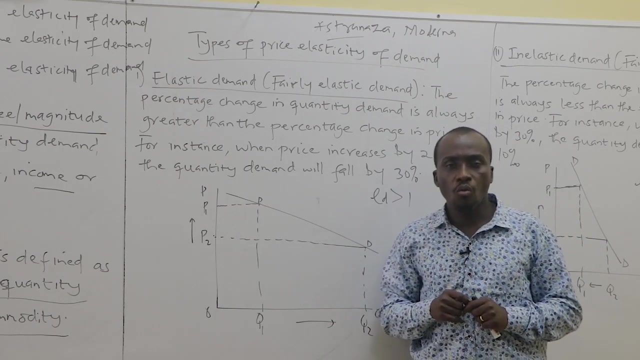 is when the commodity, the percentage change in quantity demand by the consumer, is higher than the percentage change in price, meaning that the commodity is very sensitive. The slightest changes in price brings about a large change in the demand. If price increase by a small margin, demand will increase. 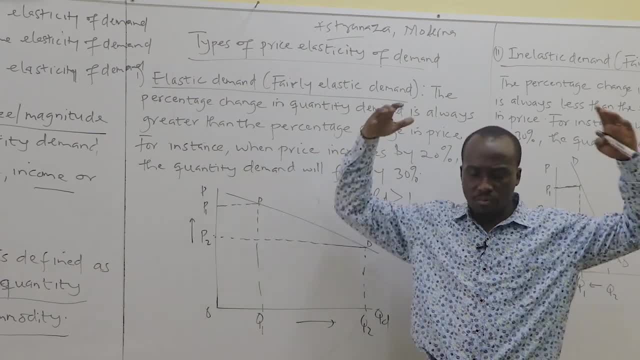 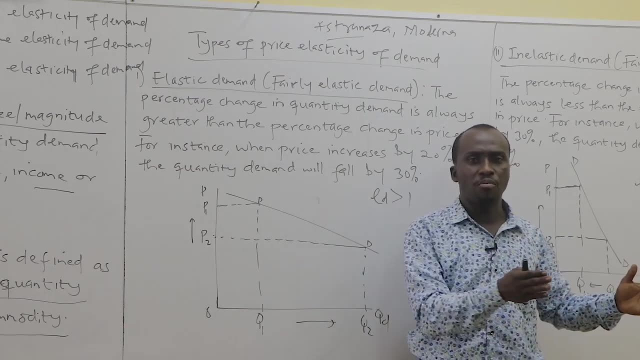 If price increase by a small margin, demand will fall by a large margin. maybe price increase by 5%, demand will fall by maybe 30% because maybe the product has substitute. A lot of people will shift from that product and go and buy a substitute. 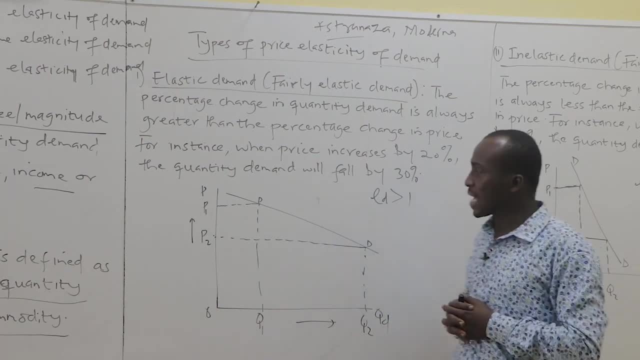 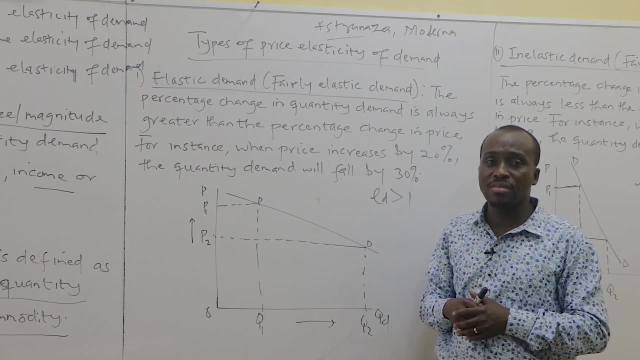 And that results in a large change in the quantity demand. And I gave you example of using a Moderna and AstraZeneca as a vaccine for COVID-19.. We gave that. And also let's look at a diagram too, With elastic demand, the elasticity. 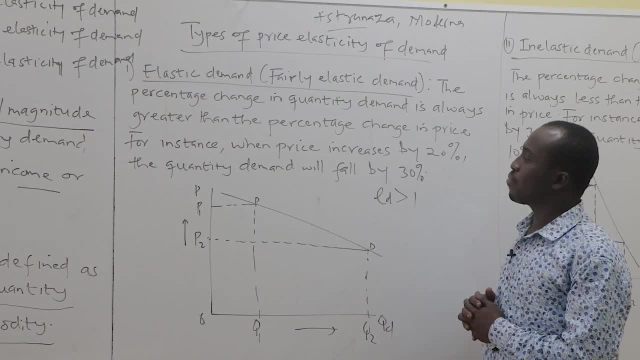 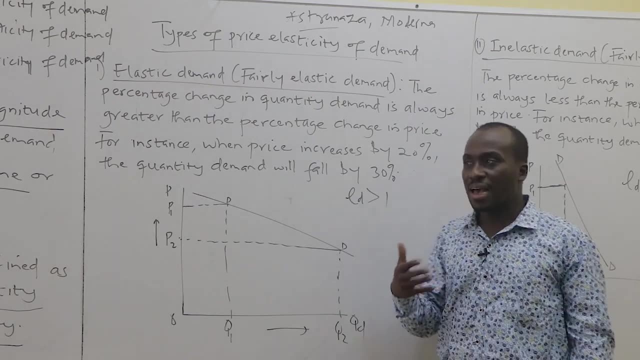 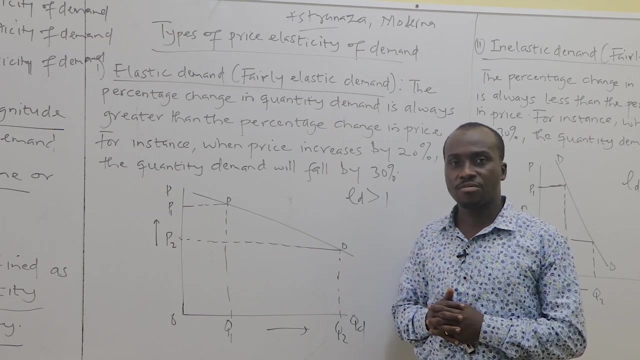 is always greater than one. For instance, when the price increase by 20%, the quantity demand will fall by 30%. That means the commodity is very sensitive to changes in price. In Ghana, for instance, we have Coke and Pepsi. About four or five years ago the price of Coke 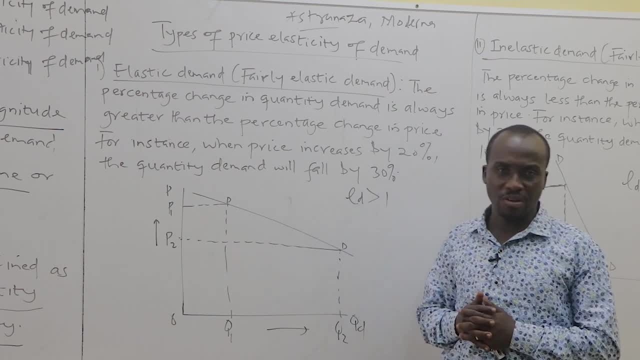 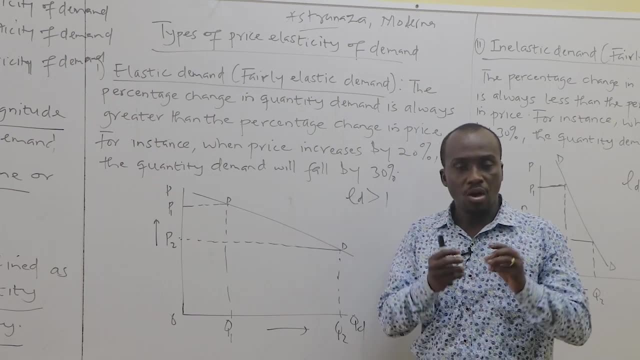 increased from one CD to one CD 20 pesos, while the price of Pepsi remained the same, And what happened was that a lot of people stopped buying Coke for programs, And now the price of Coke has gone up. And now the price of Coke has gone up. 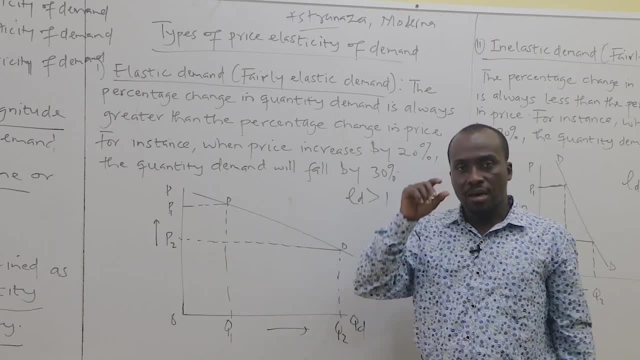 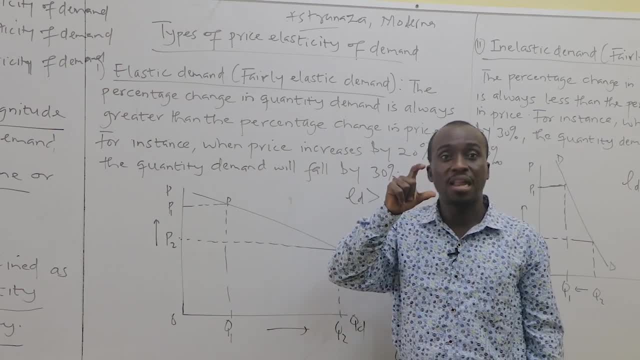 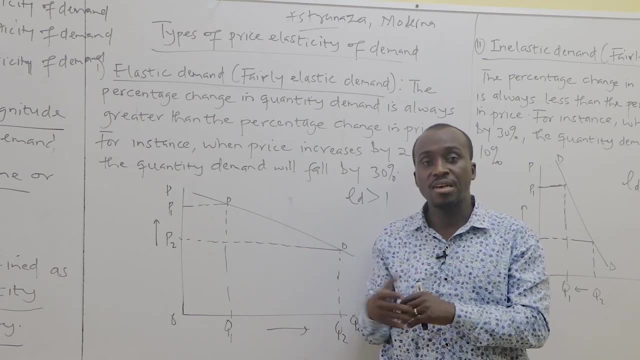 They increased the price from one CD to one CD 20 pesos And a lot of people shifted. There was a large fall in the demand for Coke because the price of Pepsi was the same. That tells you that the demand for Pepsi, by consuming, 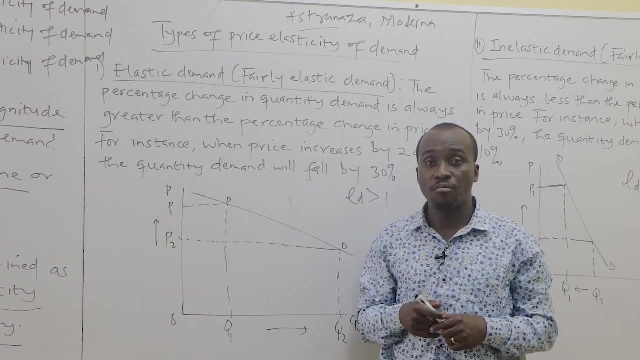 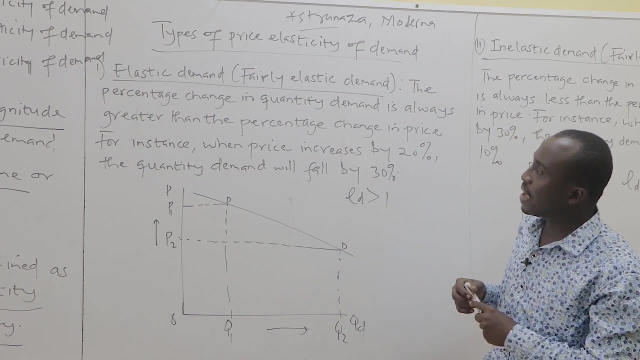 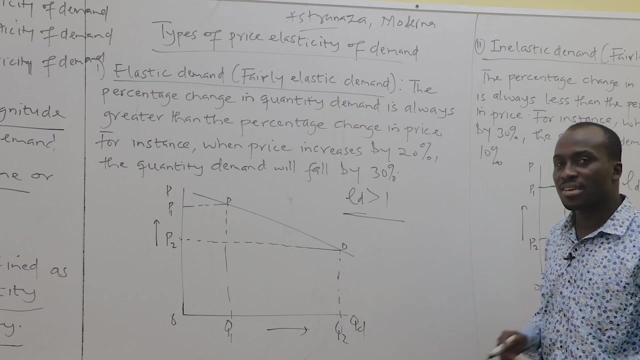 demand for Pepsi is very elastic. That's one typical example. you can actually even lead to risk. And let's look at a diagram. Whenever you have elastic demand, the elasticity is always greater than one, And later you understand what elasticity is greater than one. 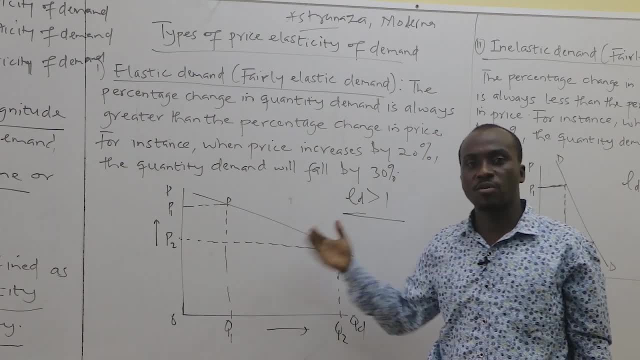 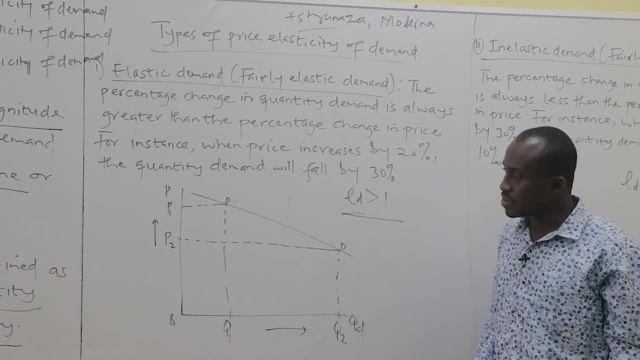 meaning that the commodity is very sensitive to change in price. That's what it means, And later we're going to use calculations that we're going to solve. to understand how these things work when using calculations, Let's see the diagram. What does the diagram mean? 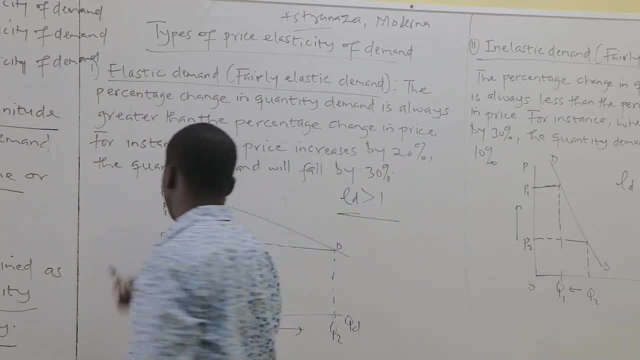 In the diagram we see that the price of Coke is very low. The price of Coke is very low. The price of Pepsi is very low. The price of Coke is very low. The price of Pepsi is very low. But first the price was at P2.. 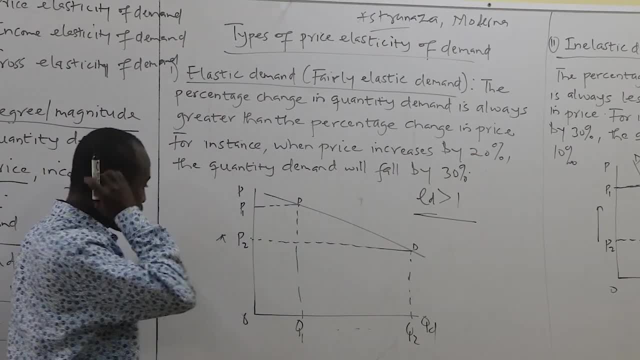 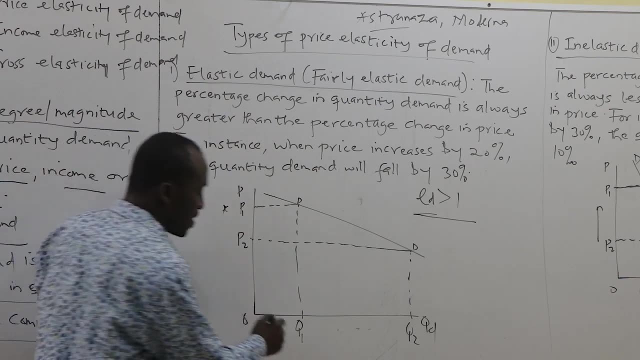 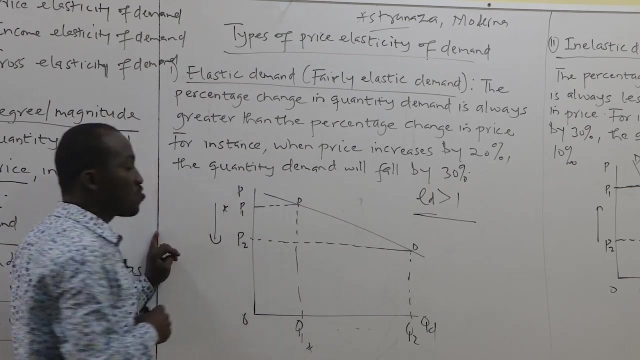 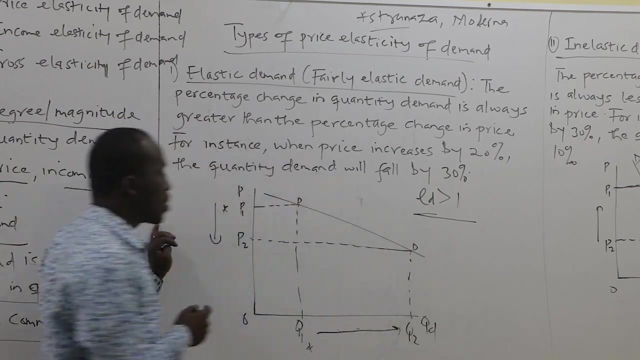 The quantity demand. the price was at P1 here At P1, the quantity demand was K01.. And that's the demand curve. The price falls to P2.. Look at it And then look at it. There's a large change in demand. 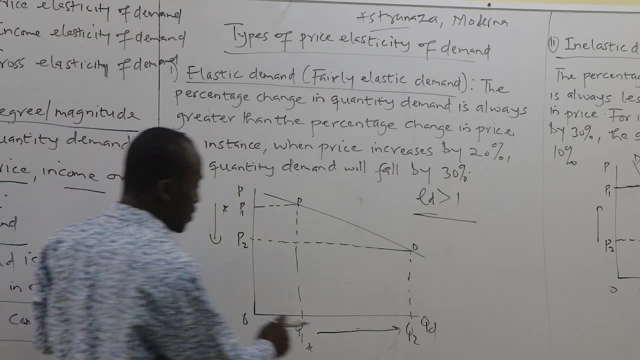 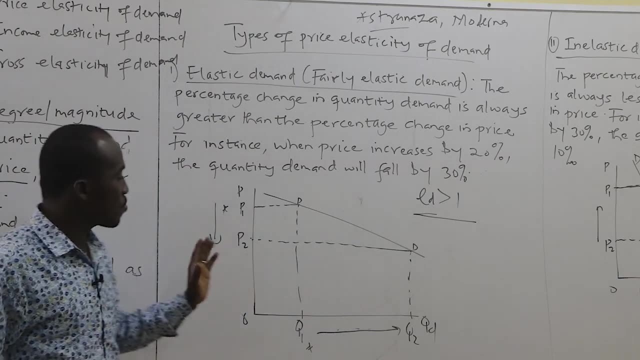 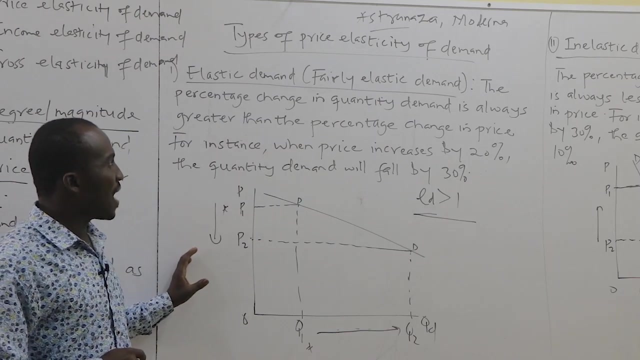 The price just fall by this small margin And there is a large change in quantity demand. So the demand curve here is more flatter. Why is it flatter? It's flatter because the commodity is very sensitive to change in price. In that case we say that the commodity has elastic demand. 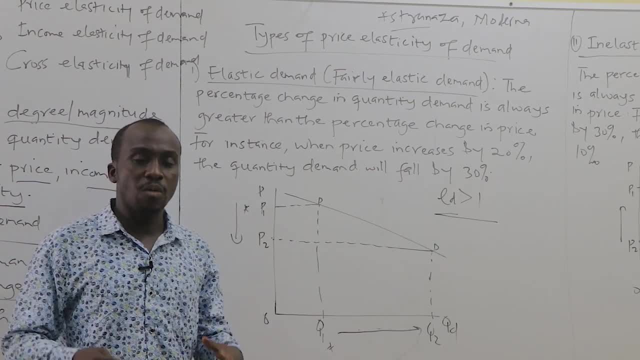 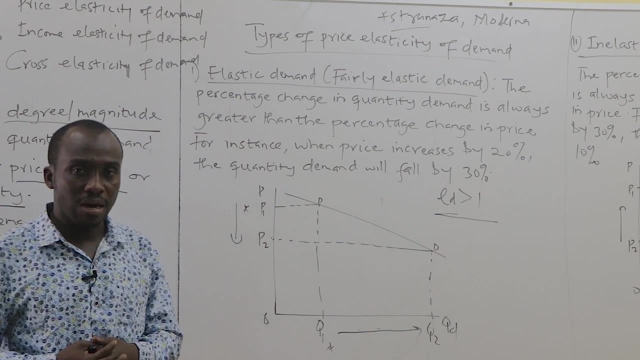 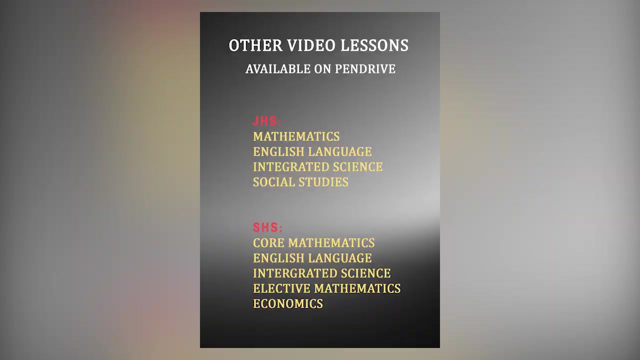 So start examining the things you buy on the market. If the things you buy on the market is very sensitive to change in price, then you can see that the commodity has elastic demand. After understanding price elasticity of demand, the definition, we want to go on to types. of price elasticity of demand. So we have five types of price elasticity of demand. One we have we call the elastic or fairly elastic demand. When do we say that a commodity has elastic demand? When the percentage change in quantity demanded is always greater than the percentage change in price. 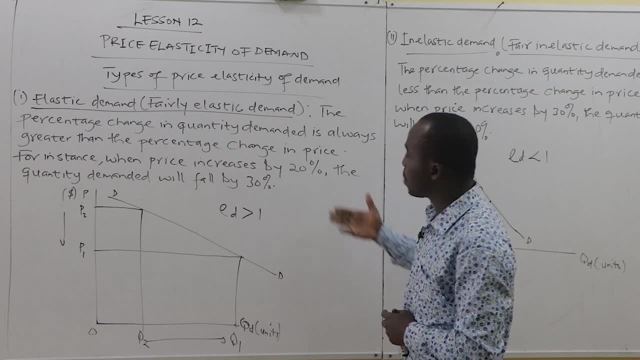 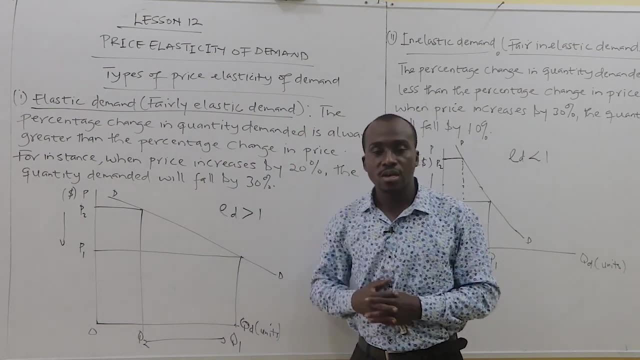 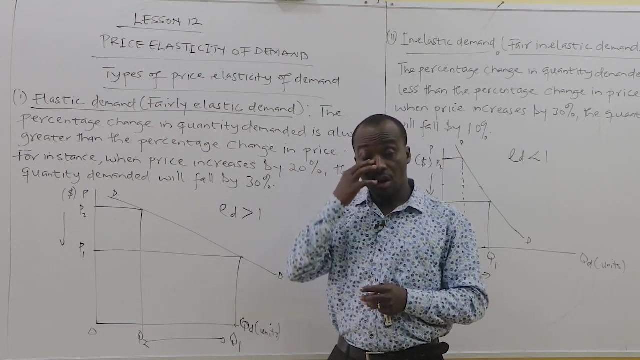 For instance, when the price of the commodity increased by 20%, the quantity demanded will fall by 30%. In that case, what do you see? It means that whenever there's a change in price, the change in quantity demanded is higher than the change in price. 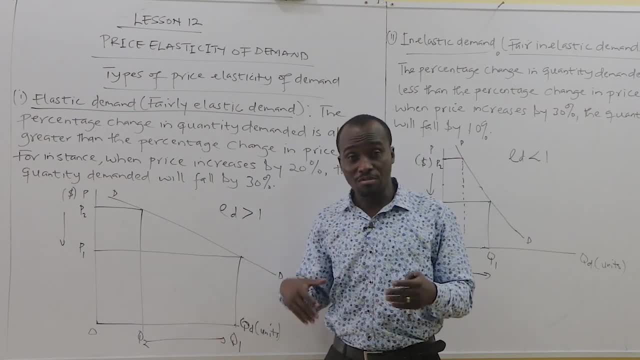 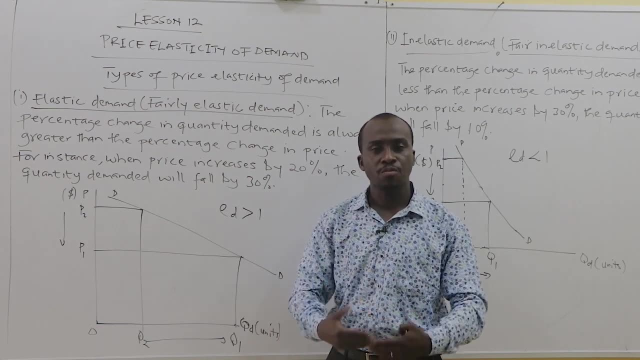 If the commodity price falls by maybe 10%, demand will increase, maybe by 40% or 50%. In other words, it means that the commodity is highly sensitive to change in price. The slightest change in price will bring up a large change in demand. If the price decrease by a small margin, demand will rise by a large margin. If the price goes up by a small margin, demand will fall by a large margin. That means if you buy a commodity in the market that behaves that way, that means the commodity is very sensitive to changes in price. 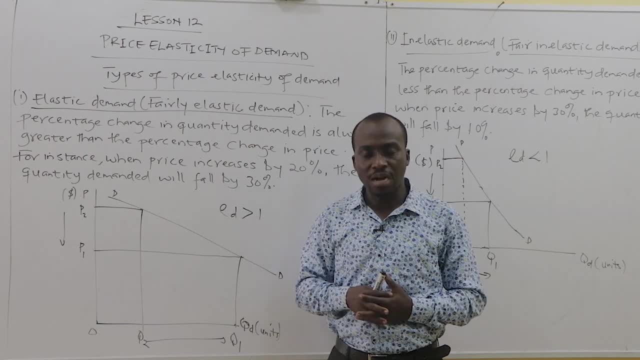 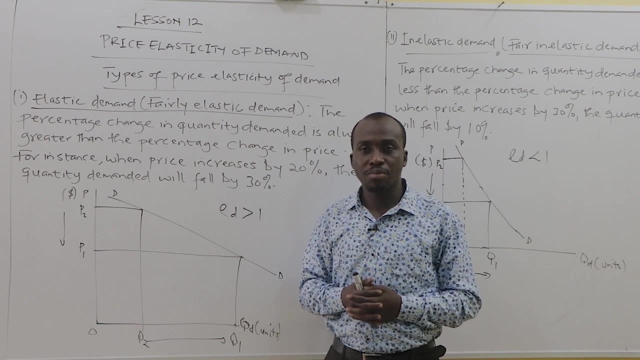 The slightest change in price brings up a higher change in demand. A typical example: in Ghana, for instance, I think about six years ago, we have Coca-Cola and Pepsi, And Coca-Cola increased its price from, I think, one CD to one CD 20 pesos. And the price of Pepsi was the same. A lot of people stopped buying Coca-Cola programs and shifted to buy Pepsi. Why? Because they felt that they can use Pepsi in place of Coca-Cola And in fact, the price of Coca-Cola is increased by 20 pesos. 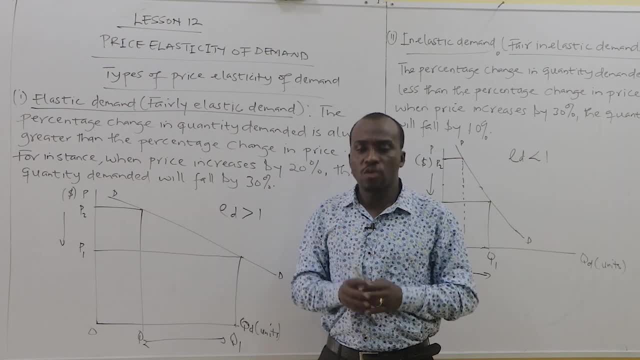 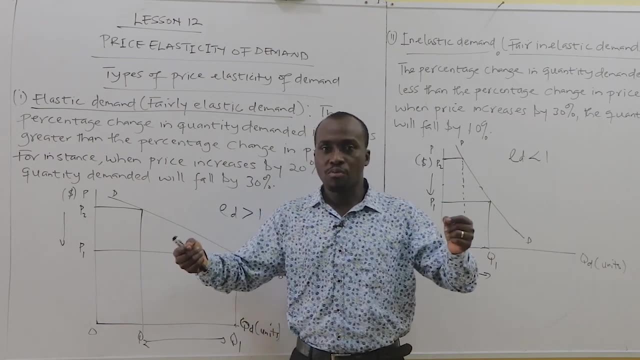 So it's an increase in the price by just 20 pesos. It made Coca-Cola experience a large change, a large fall in its demand. So any product that behaves that way, especially the product that are substitutes, behaves that way because they are substitutes. 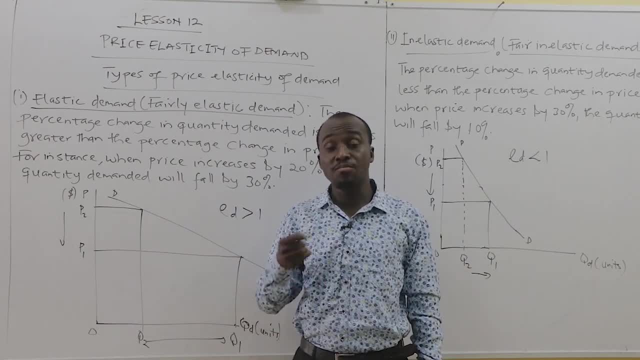 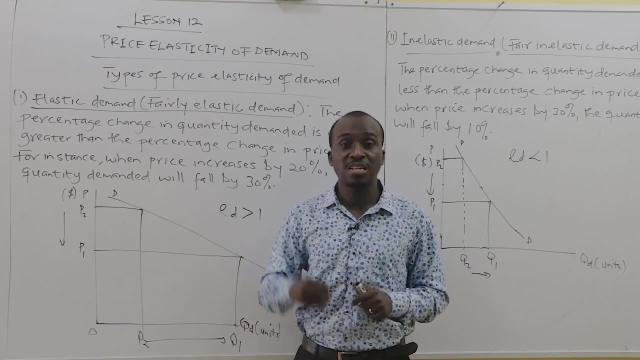 the slightest change in the price brings up a large change in demand because people can switch to each substitute, In that case such commodity. we see that the demand for such commodity is elastic. say the demand for that product is elastic. so look at the things you buy. when is it changing price? 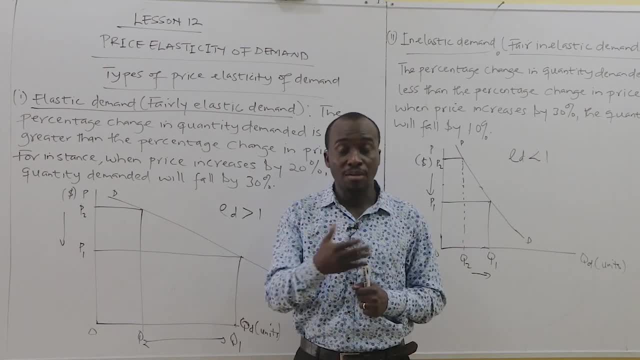 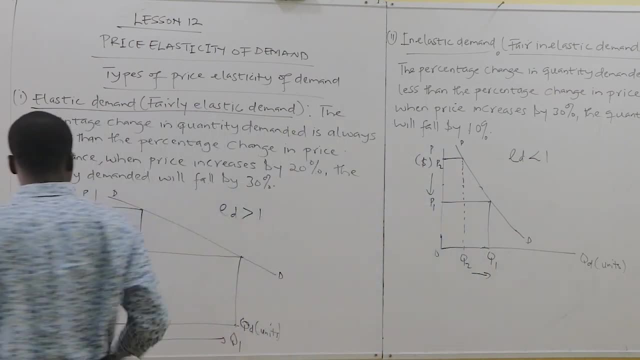 how do you behave towards that thing and see whether the things you buy in the market, is it elastic or in the last. so let's see. so let's use this diagram to explain the point here. what do we see here? here, remember, we have our price outline, here we have our origin. 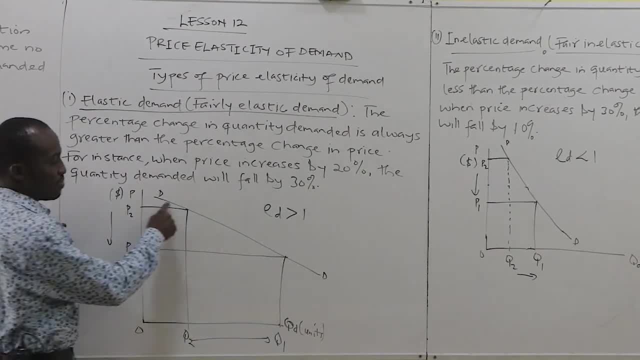 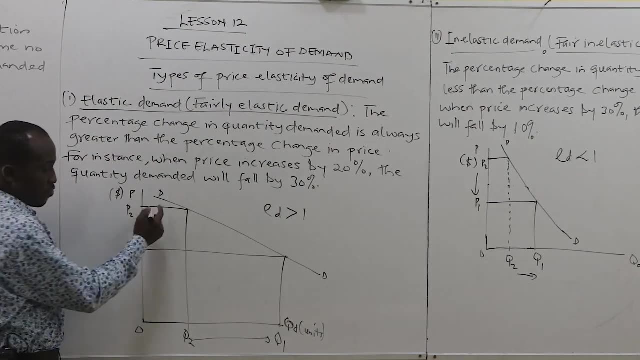 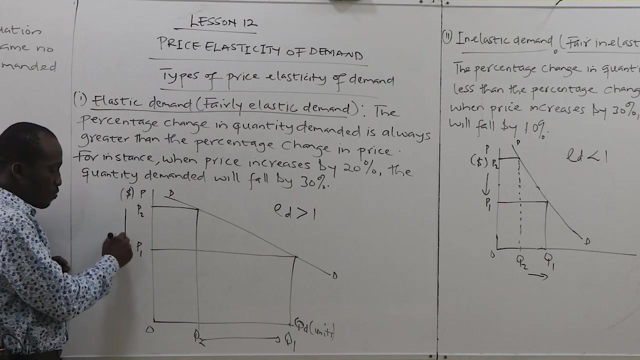 we have the quantity right, so let's we have our demand curve here. let's assume that price was at two when price was up to you. if you trace the price down to the demand, we're going to have ko2, that's quantity two. when price reduced to p1, what happened? demand if you trace the p1. 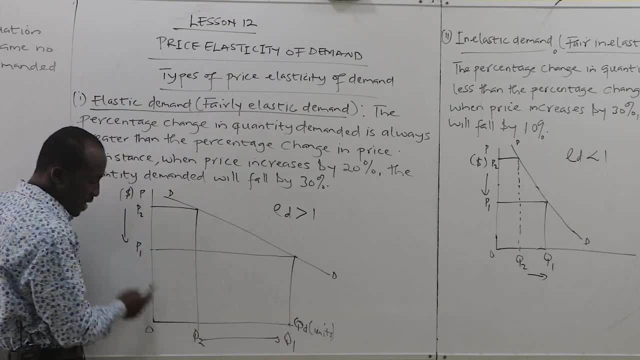 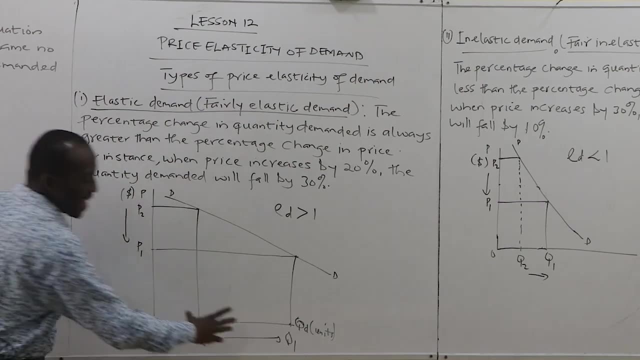 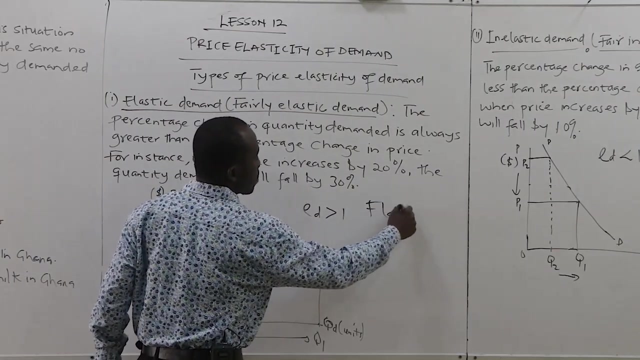 to the demand curve. the demand increases to kill one. what do you see? a slight change in price has brought a large change in quantity demand. so here the demand cave is more or less. it's more flatter, it's flat. i see that the demand cave is more flatter. it's flatter because the commodity 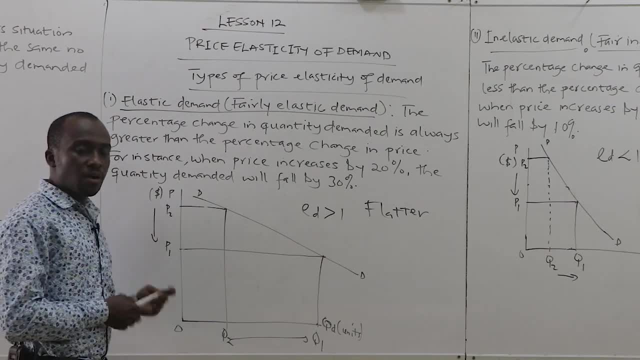 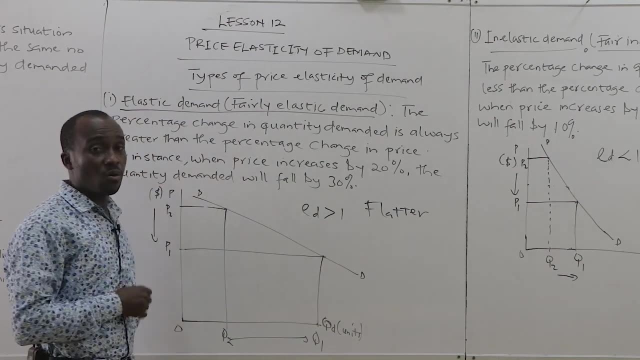 is very sensitive to changes in price and the elastic. when the commodity have a lasting demand, it means that the elasticity is greater than one. so when you say any without elastic demand, the last is greater on one. it means that the commodity is very, very sensitive to changes. 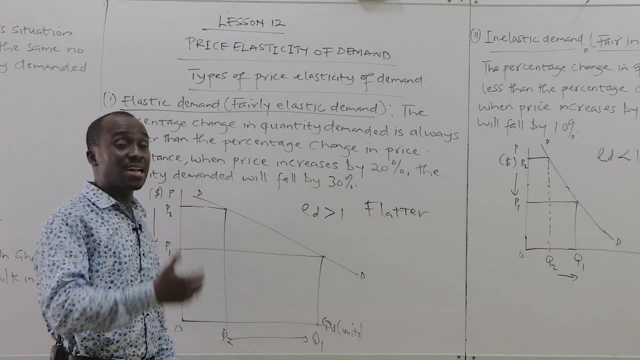 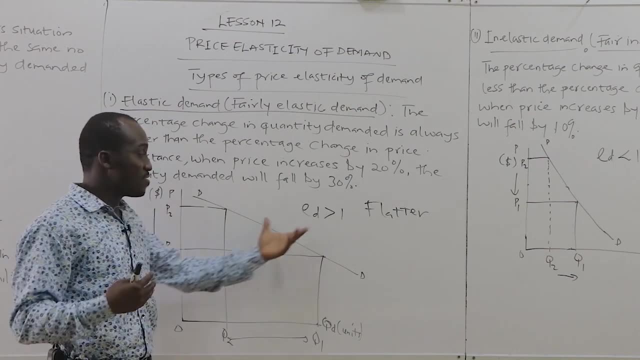 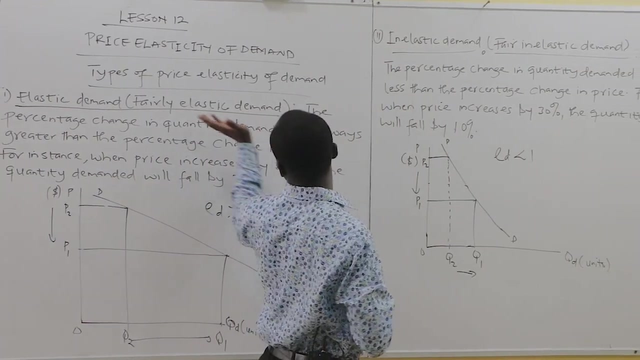 in price. so with represent a change in quantity demand. it's always greater than a percent change in price. that's what it means for at this stage. later we will take questions to solve and see when the last will be greater than one or less than one. let's also look at this. the opposite of elastic demand is the inelastic demand. 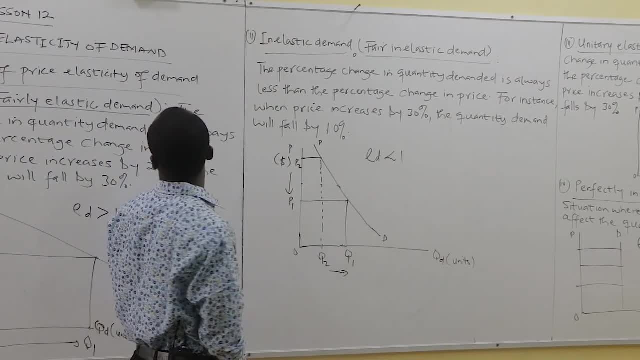 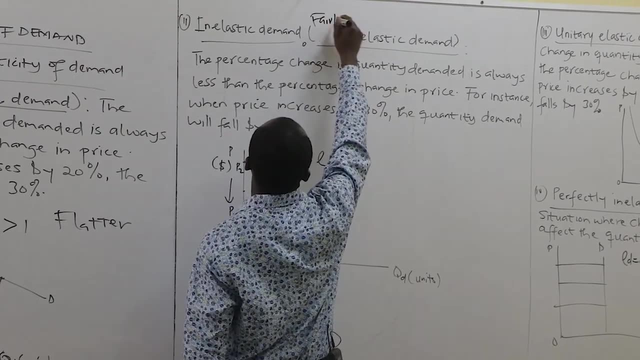 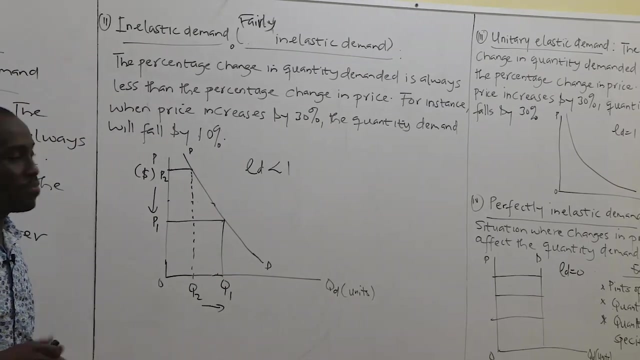 you are inelastic demand, or what you call the fair, the fairly, the fairly elastic demand, fairly inelastic demand. so either you see a product, either i say it's inelastic demand, or you can say fairly inelastic demand, the same thing. what does it mean? it means that the percentage change. 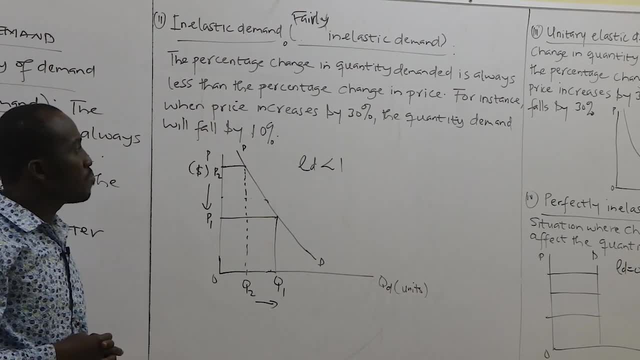 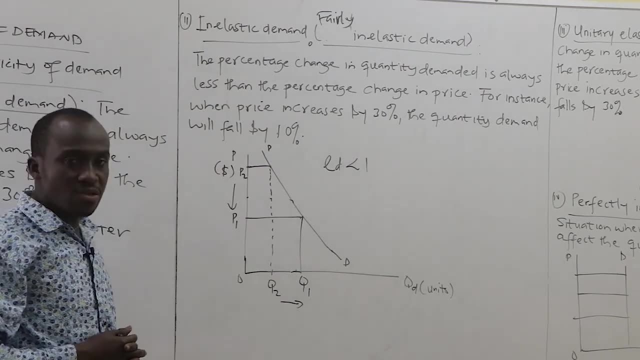 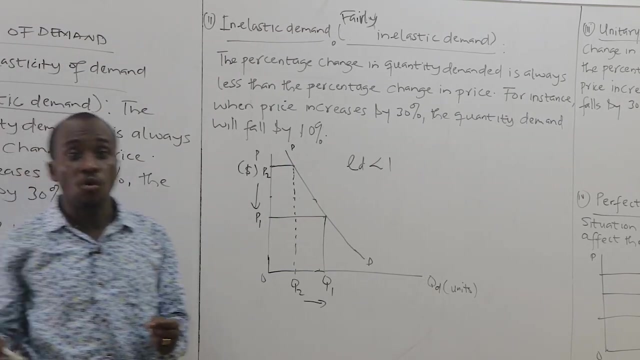 in quantity demanded is always less than the business change in price. for instance, if the price increased by 30 percent, quantity demand will fall by 10 percent. in that case, so assuming a product, the price increased by 30 percent but demand for only by 10 percent, that means the commodity is not highly sensitive to change in. 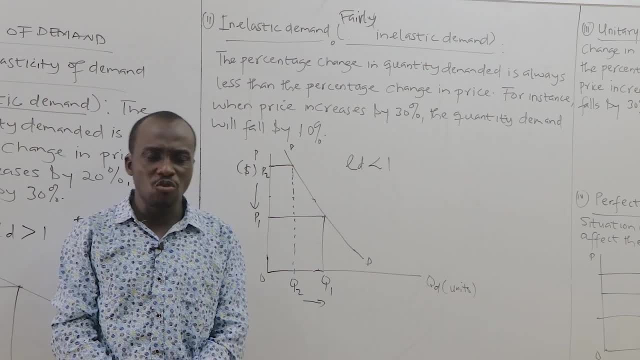 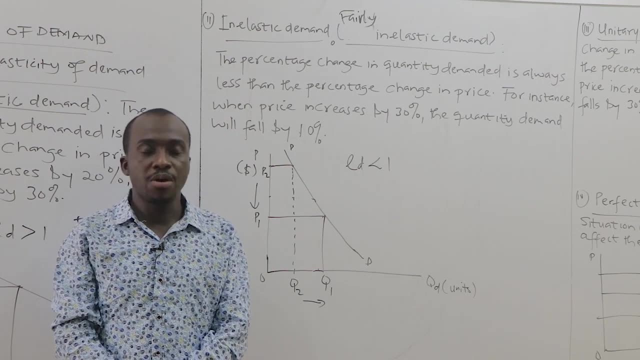 price. so change in price does not affect the demand. so even though demand will fall, it will not fall by so much. why, for instance, maybe the good is a necessity. maybe you are renting a room in here in a crowd where people rent two bedrooms for 500 ganas- it is a month. if next month the landlord 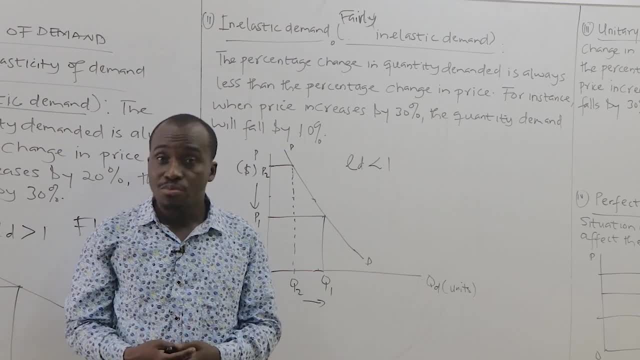 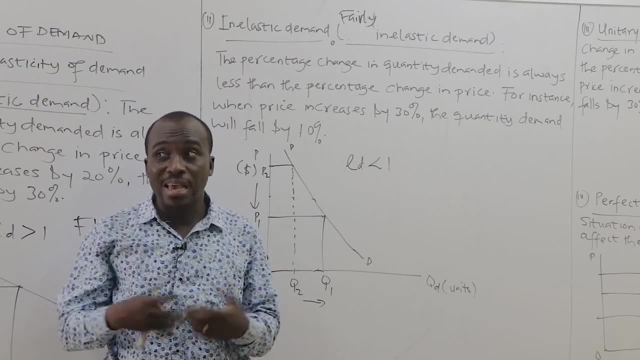 is going to increase it from 500 to 700, what will you do? you have no option to still buy it, so your for that product is not sensitive to price, or you relocate. if all landlords are saying they're charging that amount of money, what do you have no option but to keep on buying or people relocate. 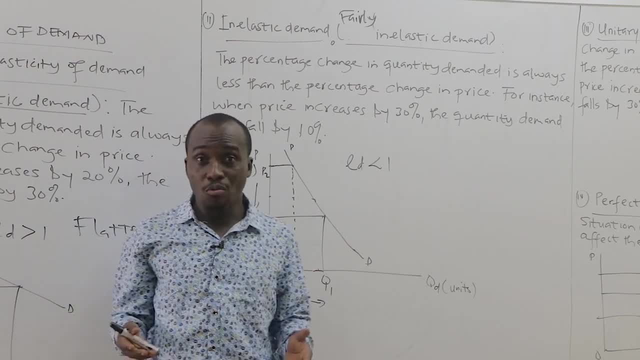 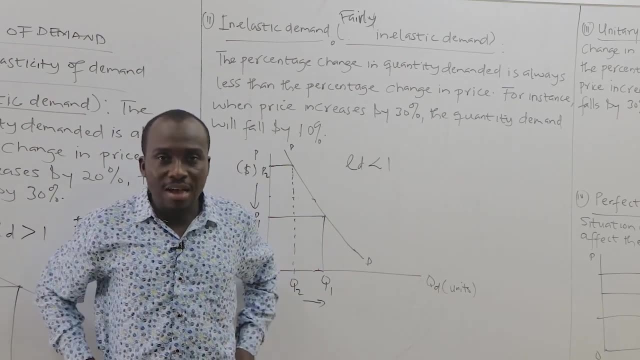 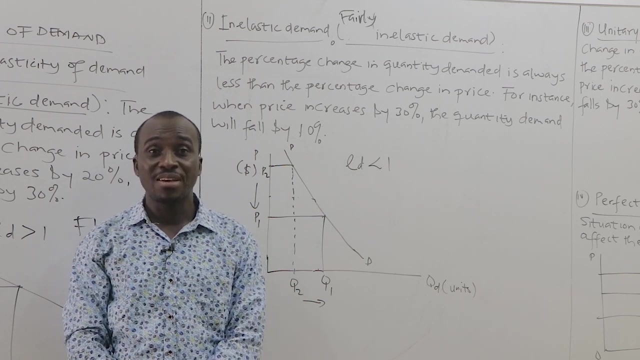 from across to other place. how many people, how many a few people, cut down their demand because some people cannot relocate. so goods that are substitute. for instance, the doctor acts you to buy a drag that you need to take every month. you, when the price was 10, the price of increase to 60, what? 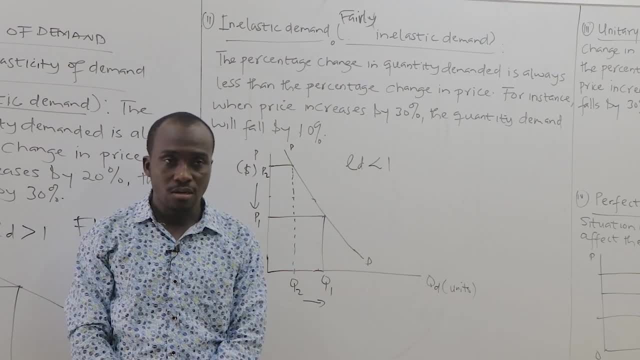 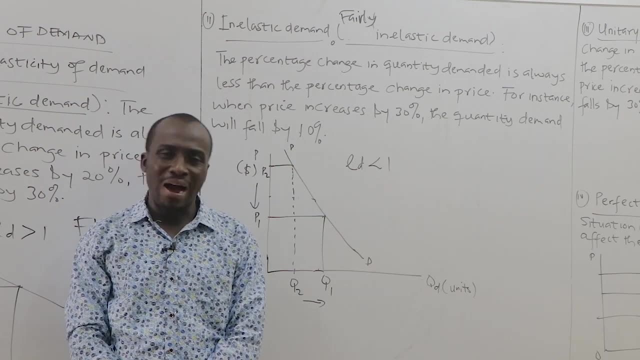 will you do? you are supposed to take that drug every month. will you say that because the price have gone up so you die? certainly not, you try to. maybe maybe if you're going to buy 20, maybe you buy 15 or 16, and yesterday you demand it. so such commodities, we say they're inelastic, demand they. 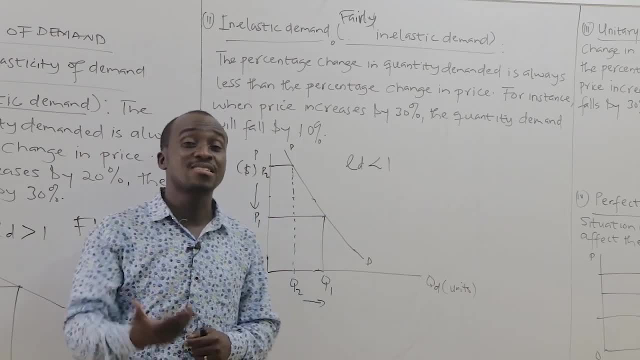 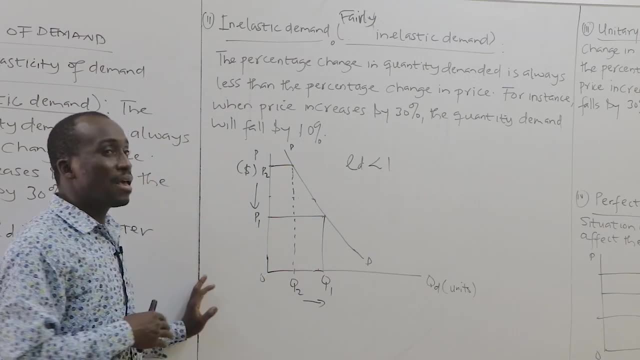 are not too sensitive to changes in price, especially when there's an increase in price. the people who stop buying are very few. a lot of people keep on buying. so we say that that commodity is inelastic or what is it fairly elastic? so it's the opposite of elastic. so in 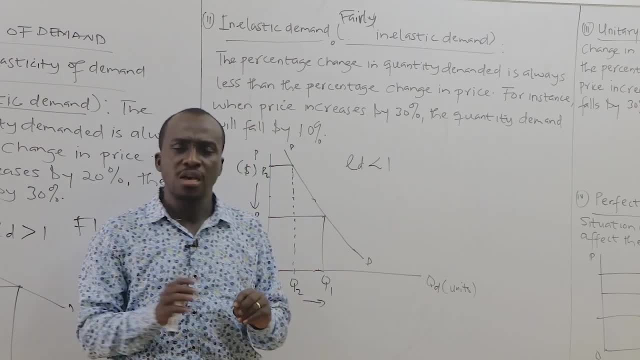 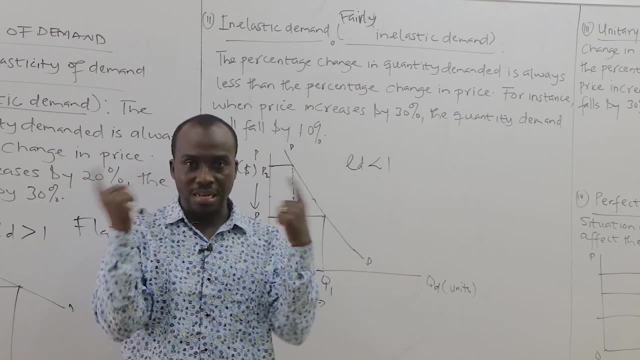 a commodity that's not highly sensitive to change in price. if the price increases, few people stop buying. a lot of people keep on buying. that commodity is said to have inelastic demand, so start wrap your mind around it. the things you buy on the market, on the street. see which of these. 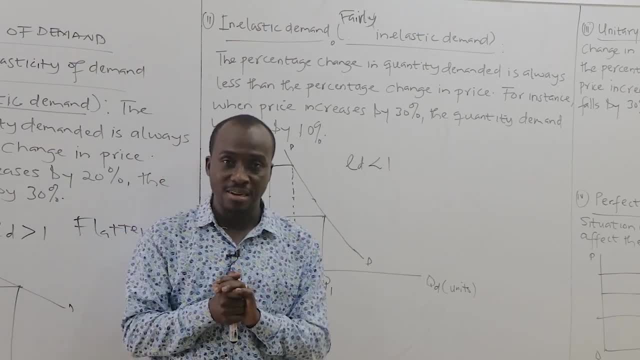 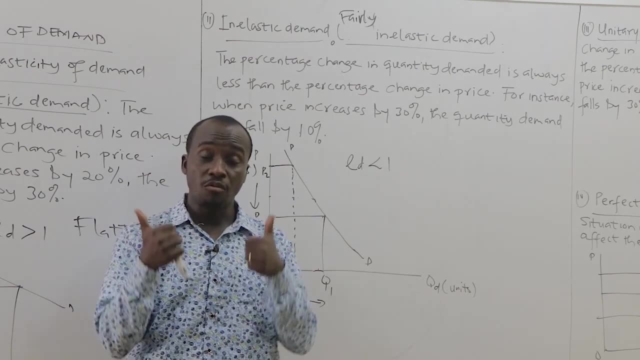 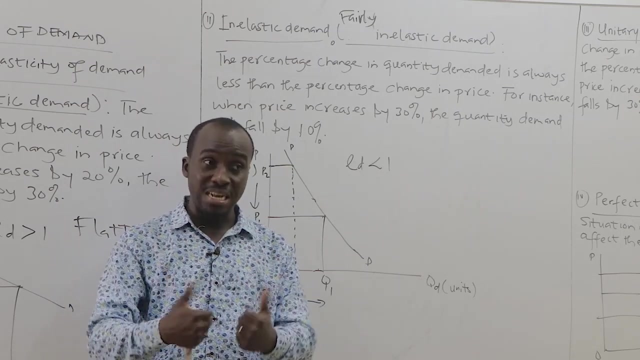 schools falls category into these elastic or inelastic demand. it's very practical, it's only for writing the exam buyer for everyday life. later i'm going to tell you the importance of these, this intuition about price assistant, what it means to you as an individual, as tax expert, the government, international trade policy expert, you're trying to actually effectuate. 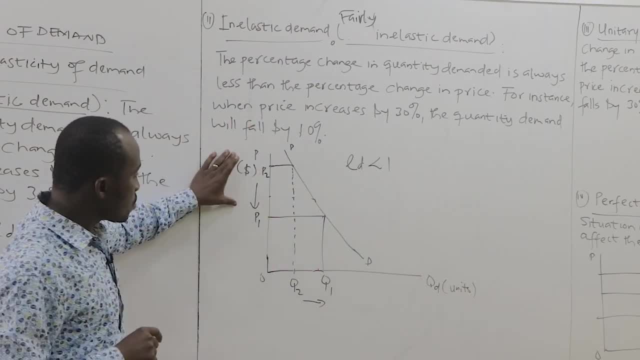 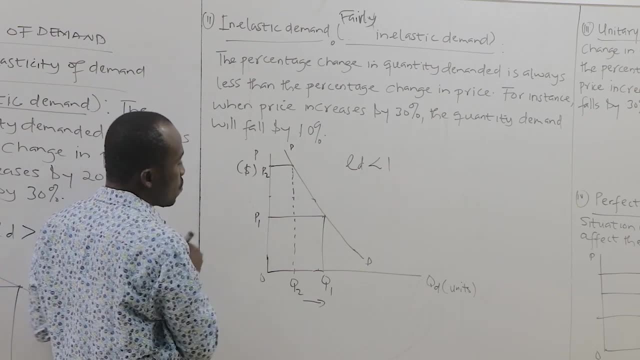 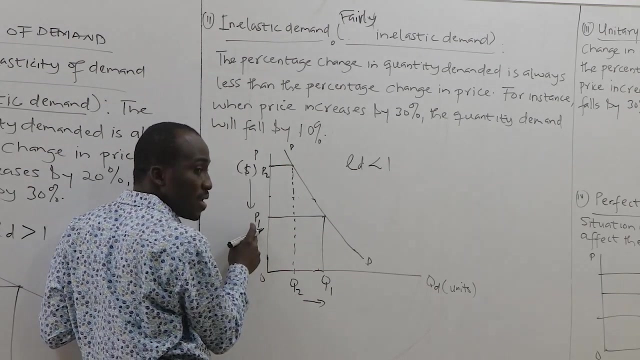 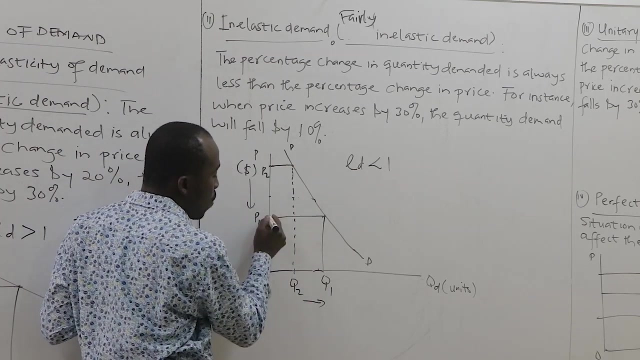 the irrelevance of these things. so let's see here, let's use the diagram to depict what they call the elastic demand. first, the price was at p2 and the quantity demanded was killed to you. the price reduced to p1 and demand increased by q1. let's see, so if you trace the p1 line to the demand line and you trace 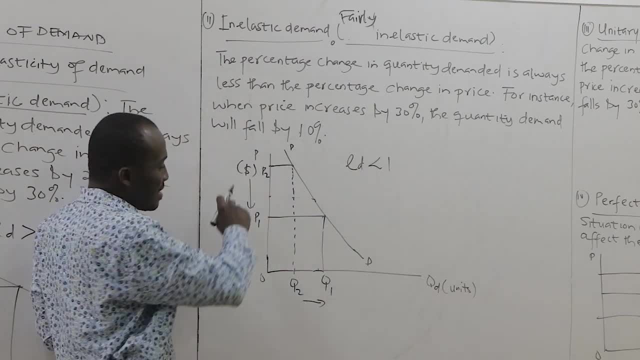 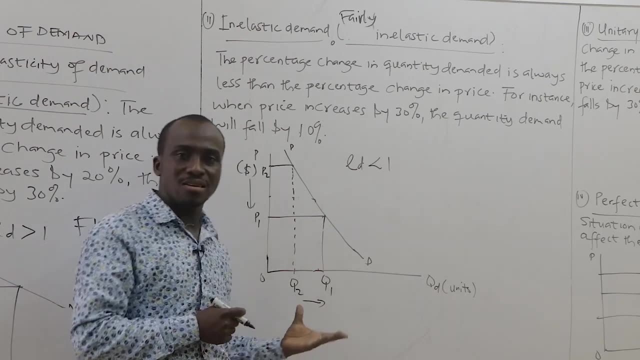 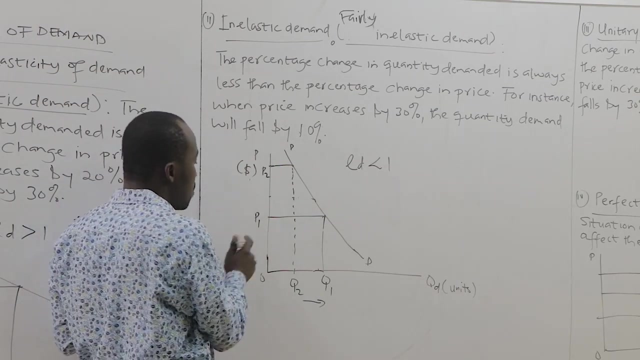 it here. what do i have? q1? what does it mean? they look at it, the man, look at it, look at the space. the change in price is higher than the change in demand. you can do it vice versa. where price increases, you can have the same thing. the price was at p1 and people were demanding q1. right, the 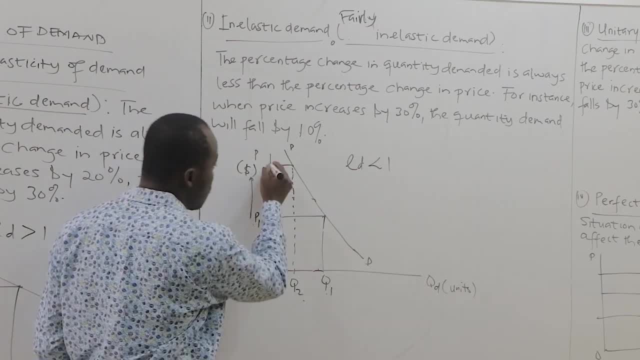 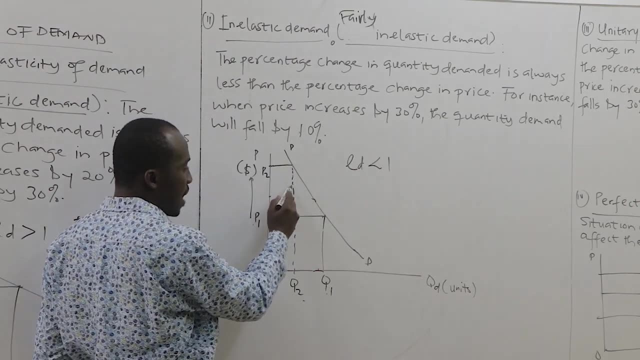 price increased to ph, you demand force. if you p2, you trade the p2 down to the quantity line, you're going to get killed. so this is the p2: trade into the demand line, bring it downwards, downwards, down again. you're going to get killed. and let's have this. what? what do we have here in this case? what? 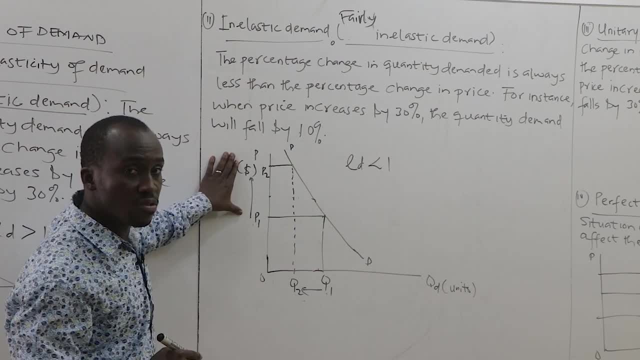 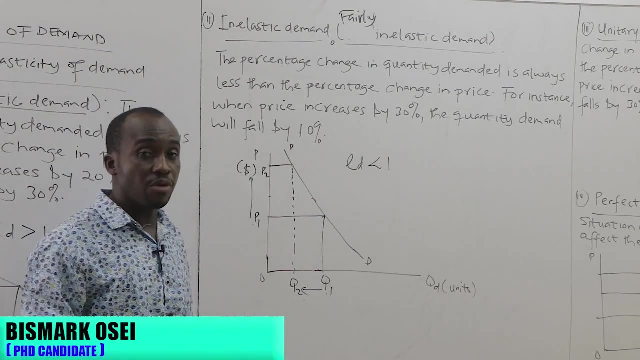 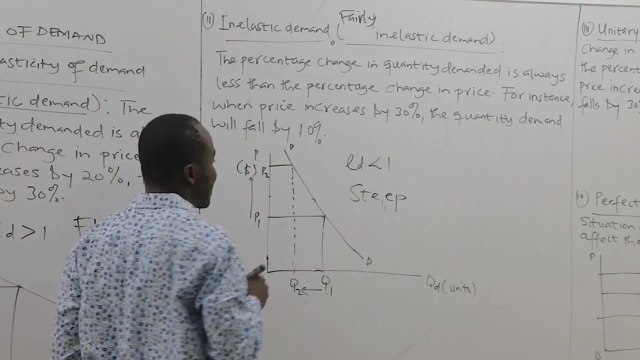 do you see? there's a large change in price but there's a small change in quantity demanded. that means that the commodity is slightly sensitive to change in price and the demand cap here is more steep. is steep here in the case of elastic or small flatter, but here it looks quite steeper. and then 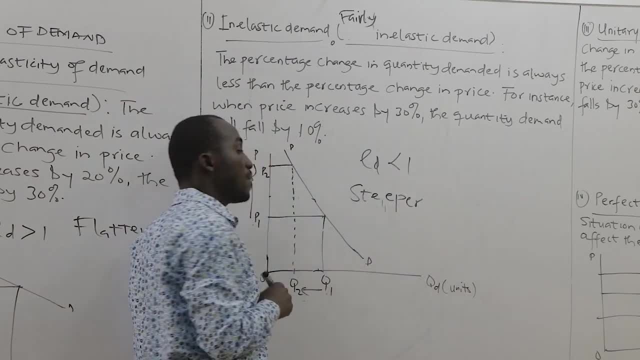 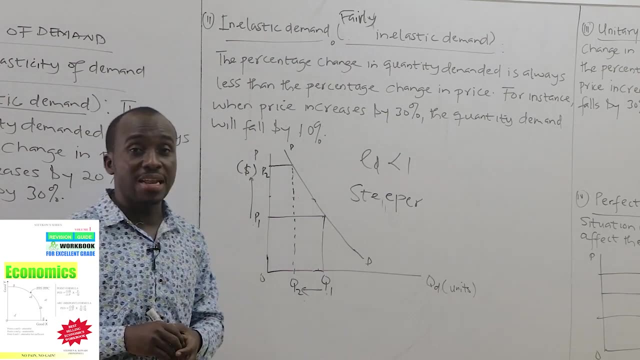 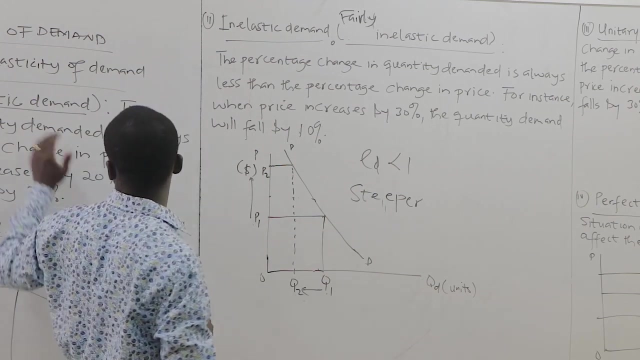 elasticity of demand is less than one, and then elasticity of demand is less than one. so when a commodity have inelastic demand, of failing elastic demand, it elasticity is less than one. so you have seen that for elastic, inelastic demand. you are seen now for inelastic demand. let's go to unitary elastic demand. what do you need to elastic demand? let's see unity. elastic demand is when. let's see is that is that the percentage change in quantity demanded is always equal to the percent change in price. hence, when the price increases by 30 percent, quantity demand also will. 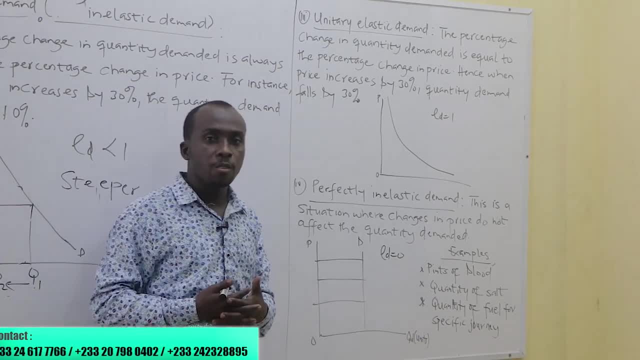 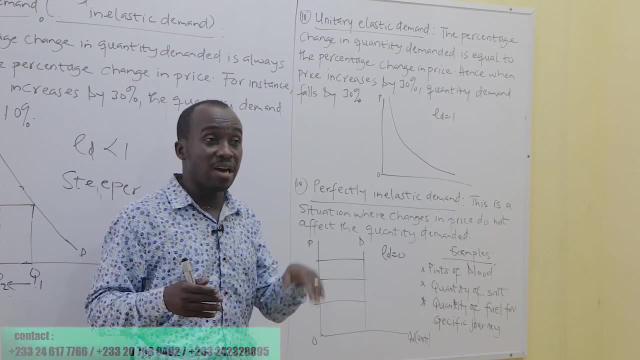 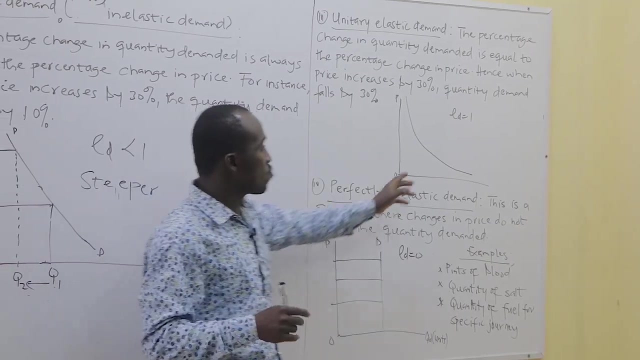 fall by 30 percent. so when you need to elastic demand, the change in price is because the change in demand. if price falls by 10, demand will increase by 10. any price increase by 20, demand will reduce by 20. so the change are almost the same. so you have velocity equal to one. 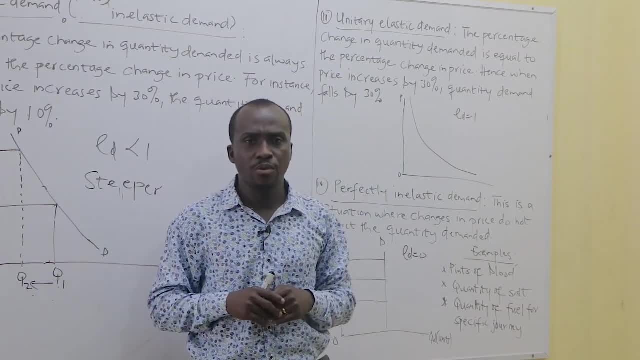 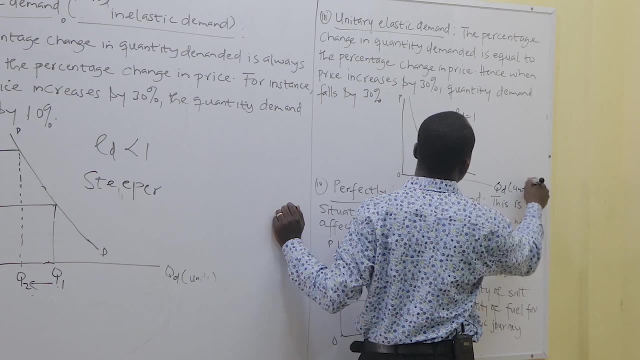 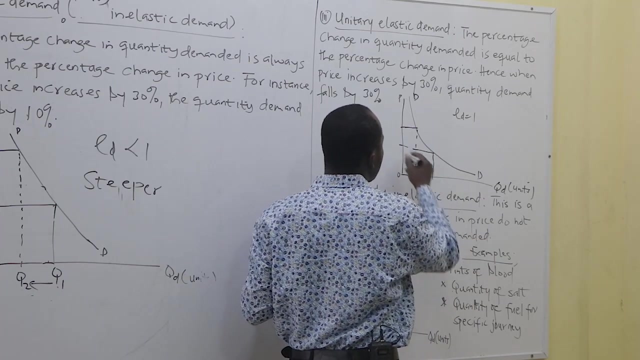 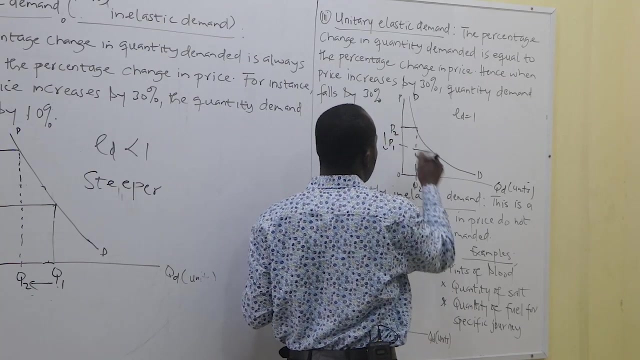 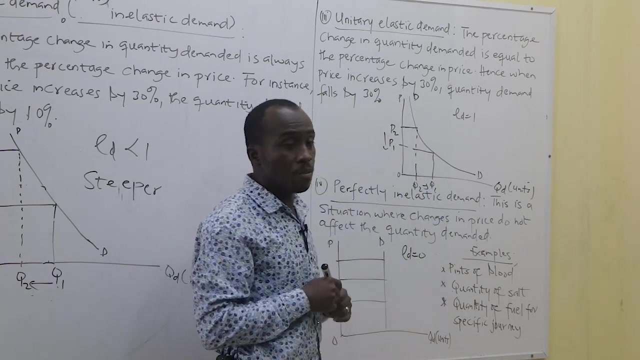 in rare cases, only few commodities behaves that way, right? so if you look at that, if you look at the diagram here, yeah, we have quantity demand d here, d here, this, half one here, this, half one here. so they change. so the change in price and the change quantity is the same and elasticity is equal to one. 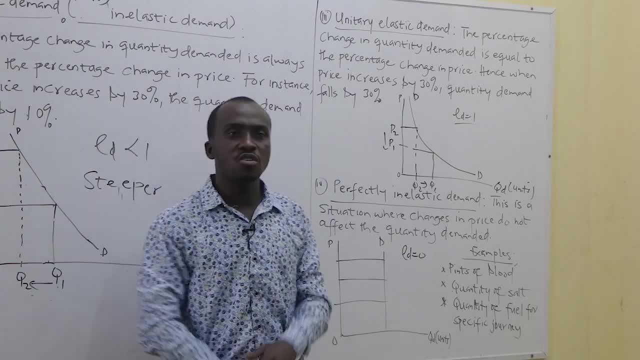 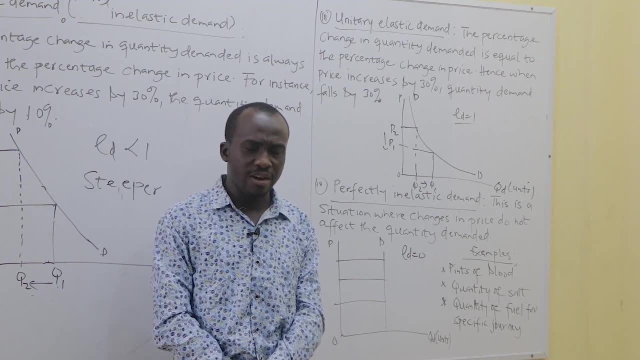 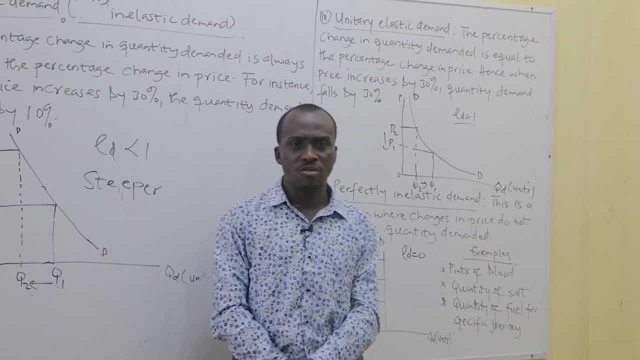 in most, but let's me say that most of the goods highly. do you see any commander behave that way? even though we say it's just carry, it's sort of carry correct, but in practice how do you see a commodity behaving that way? where price have increased by 20 percent, demand falls by 20 percent. it's counted as very. 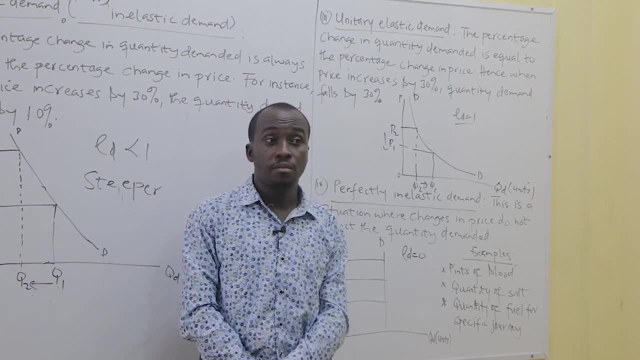 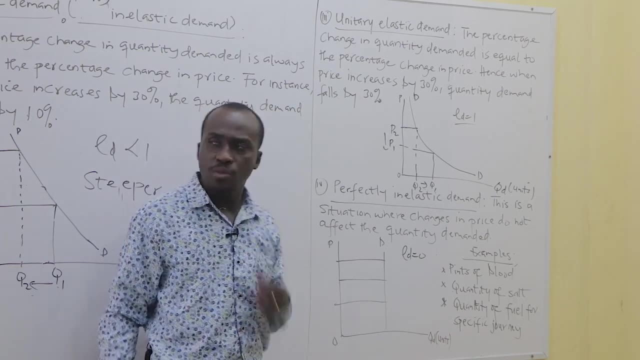 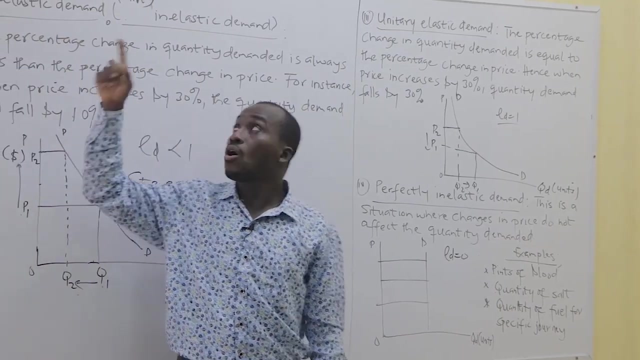 difficult to see. but for theory it's possible, but it's difficult to see. let's go on. another one we want to see is what we call perfectly inelastic demand. the fear we said is in a lot. don't confuse at here i, i, we say inelastic demand or fairly inelastic demand. at id we say that perfectly. 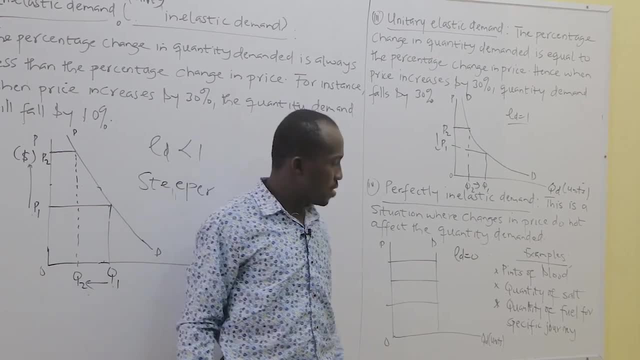 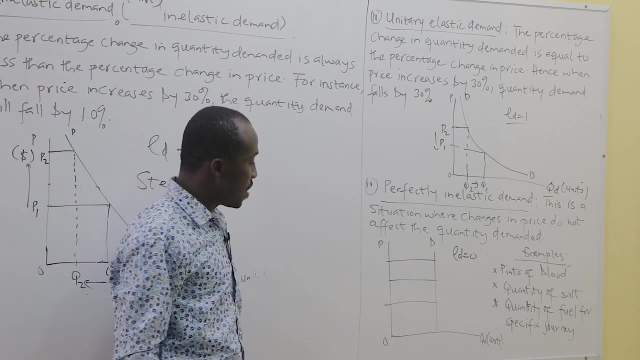 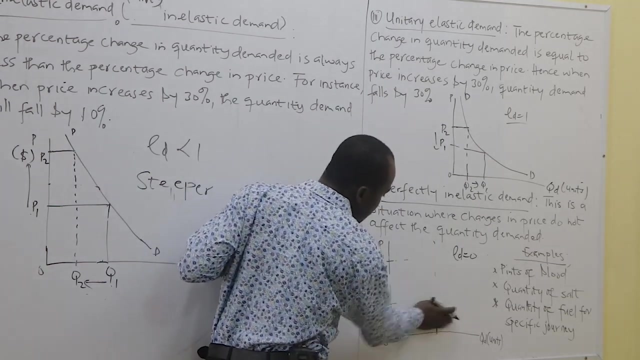 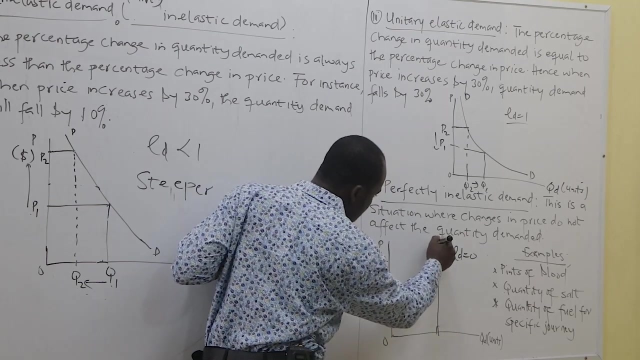 inelastic demand. what is perfectly inelastic demand? this is the situation where changes in price do not affect the quantity demand. we fairly inelastic demand when price changes. let's look at the price, the price. get this diagram. let me sketch something for you to see. let's see: 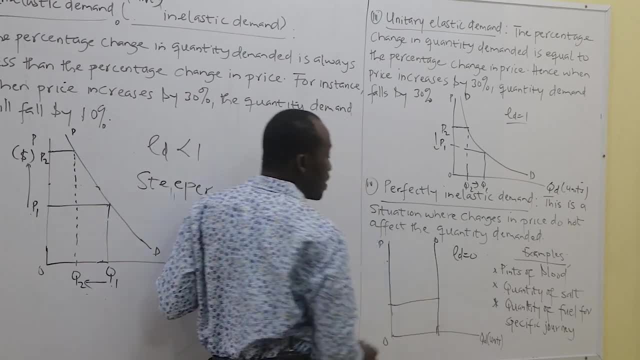 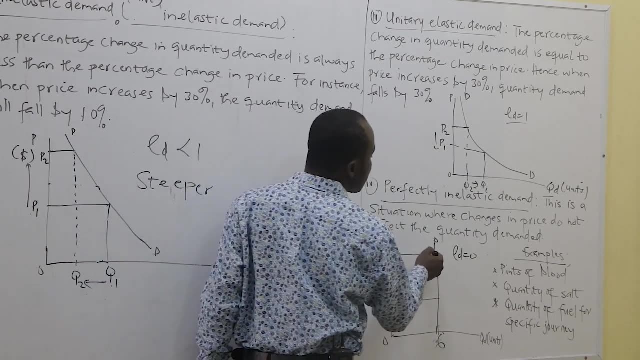 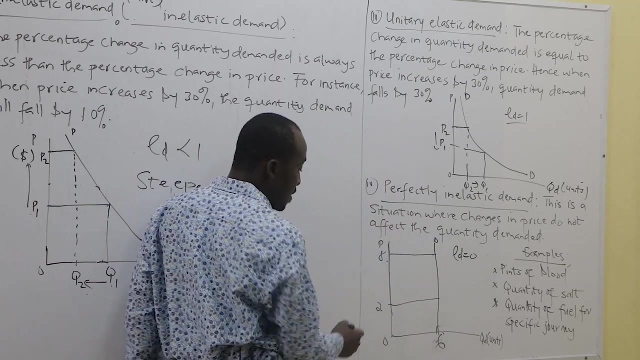 let's say this: the price was here, the demand, the quantity demanded was still constant. if it's six, it's still six. the price increased from, let's say, the price was two, it increased to eight. still demand is still fixed, it's still six. the price reduced to one, still demand is. 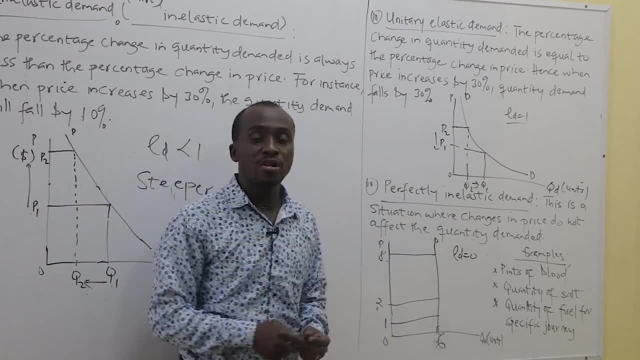 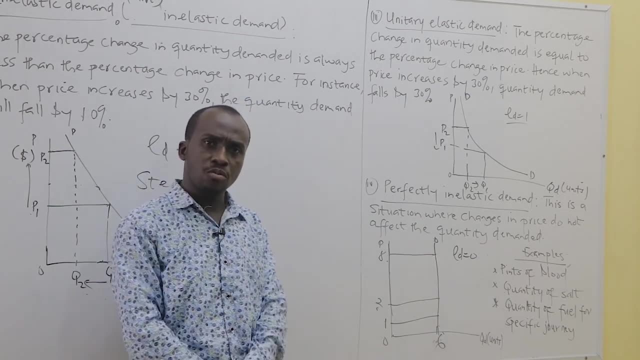 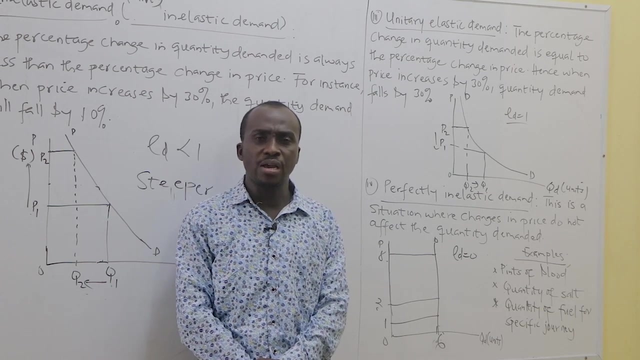 fixed. so whether price increases or decrease, people demand for that product is the same. it remains phased. okay, because they: how is it possible in real world? can you go to the market and see any product that behaves that way? let me, let me see that it's very in the real world. it's. 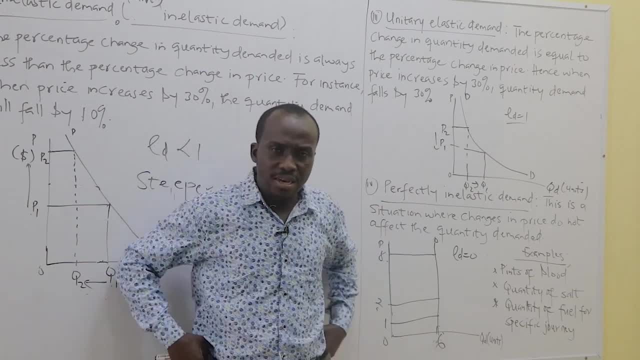 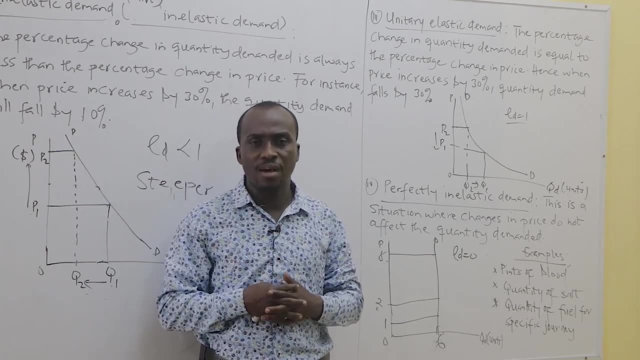 very difficult to see product that behave that way, but the exceptional product that behave that way. it's not common to see that thing happening in the market. it's very enable to see it. now our product, we believed see that thing happening in the market or any place. but sometimes it does. it does happen. let's 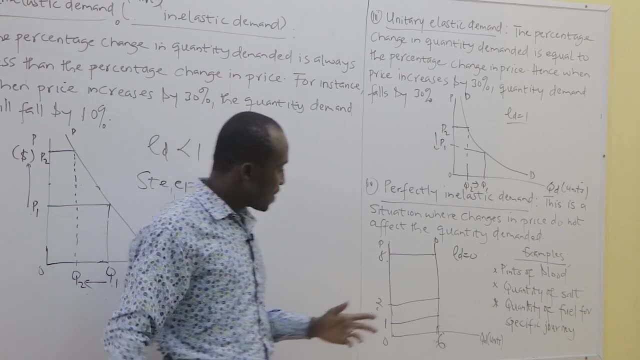 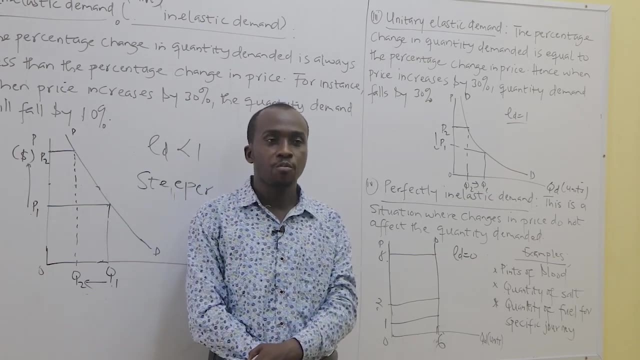 look at some few examples i can use to explain to you one example. let's look at what i call the pinch of blood. when you, for instance, you go to the hospital, doctor tells you that you need maybe five pints of blood. right, you need it, you need five. when you go the price of increase, you can't say 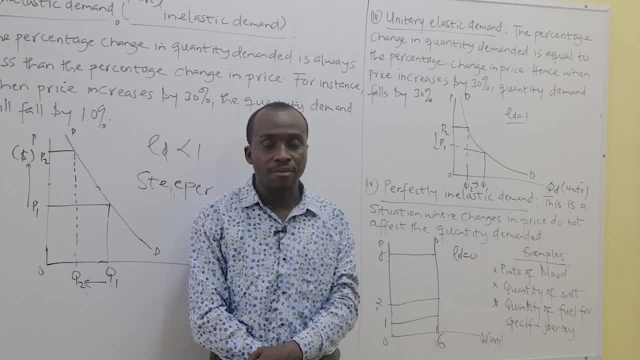 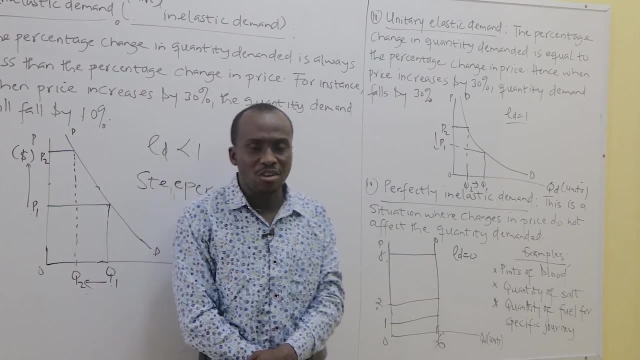 you buy less than four, you need five. you have to buy five. hour you die. if you go and the price have reduced, you can't say you want to buy more and i put it in the fridge when you need to go and take it. you cannot do that. so whatever the price goes up or goes down, you have to buy the same. 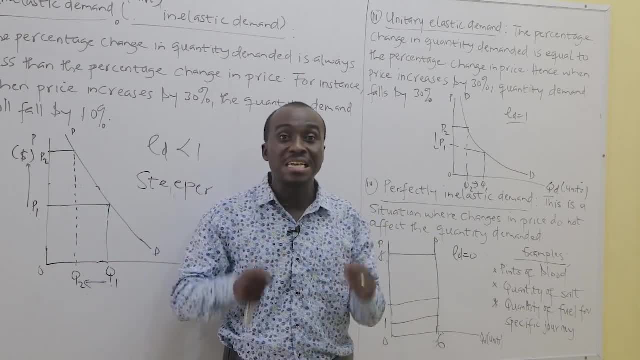 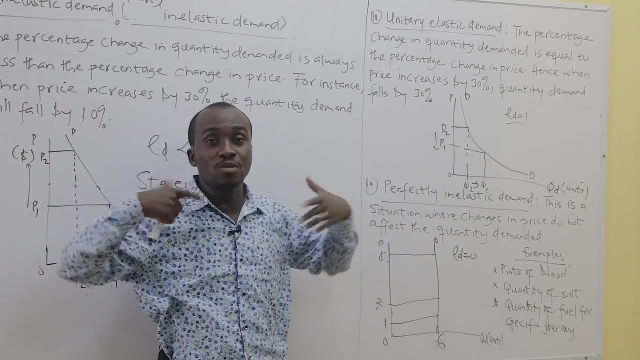 pints of blood because you need that, the quantity. you need that moments to survive. you cannot buy more and store it. you cannot store blood and you cannot buy more than that. you will die if the price falls. huh, so a good a commodity like this behave that way also. we have what we call the 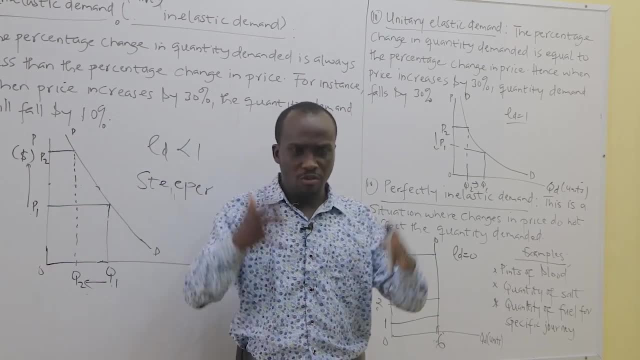 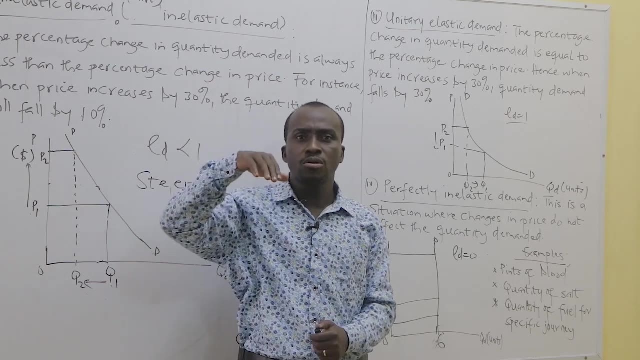 quantity of salt you put in your food. if you're preparing, maybe, palm nuts soup, the quantity of salt you have to put in is the same quantity. you can't say that when you win, the price has gone up so you reduce the quantity. the food will not taste nice. you can't say that. 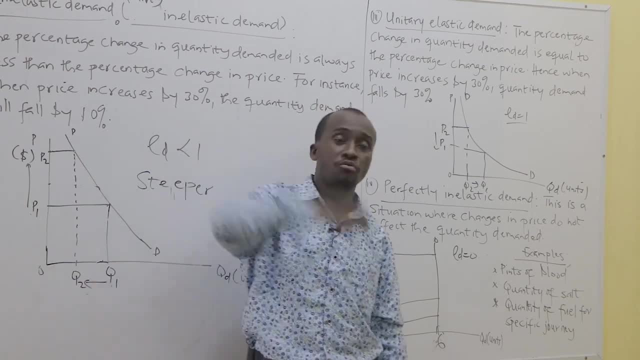 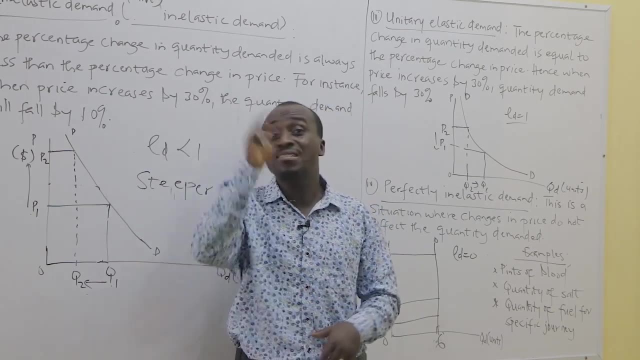 when, when the price have gone down so you want to put a full bucket of sugar salt in the thing, it's not economic. nine, so the quantity of salt you put into your food at a particular time remains the same, no matter the change in price. if the price will use or the quantity you put in will be the 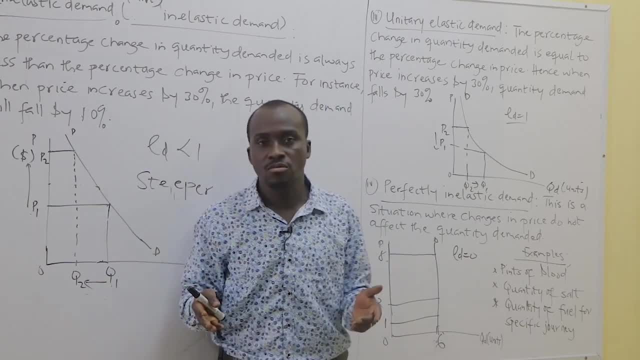 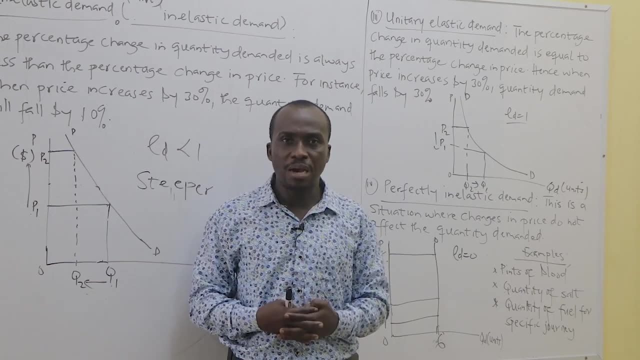 same quantity, because you cannot make it more salty or less salty. so this is a difficult example against you. another example is the quantity of four you use for a journey. maybe i'm traveling from here to accra with my private car. i have to use maybe 10 gallons of. 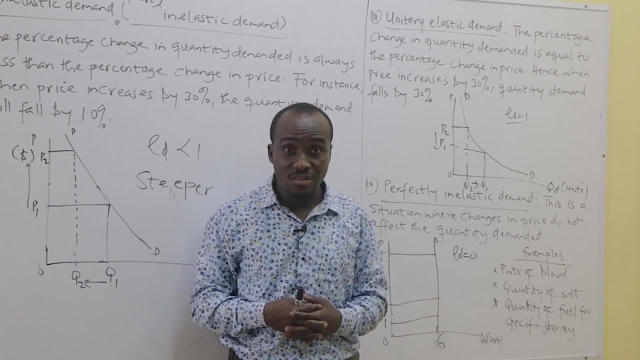 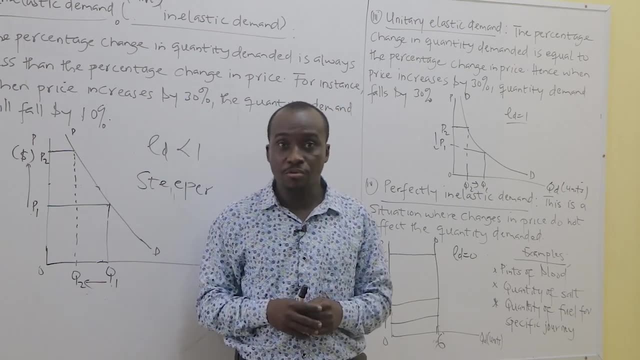 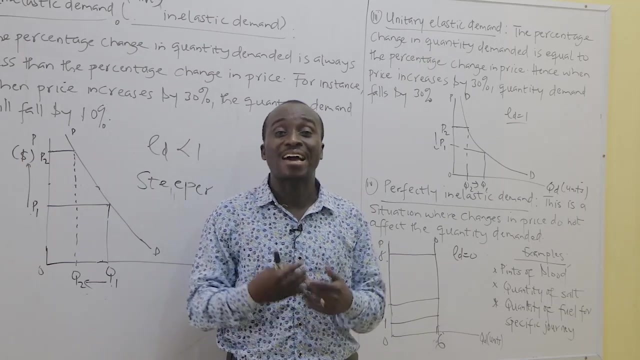 wool. without 10 gallons i cannot get to my destination. if the price reduces or increases. if i need 10 gallons of food to make it to kumasi in ashanti region, i have to buy the same quantity whether the price reduce or force, because if i buy less i cannot travel. if i buy, i buy more. where am i going to keep it right? so you buy the same quantity so that you can travel to wherever you want to go to if you don't have a place to store it. if you buy more, if the price have reduced, you don't, you buy more, you might not have a place to store it. 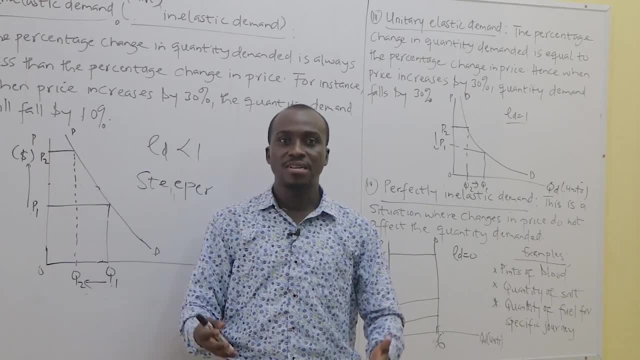 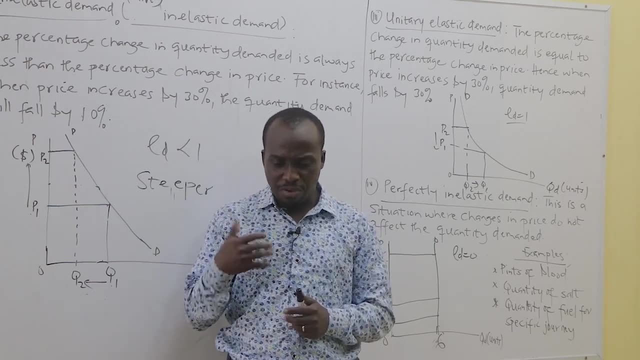 if you buy less you cannot get your destination, so you buy the same quantity you need at that moment. so in that case the goods behave perfectly inelastic. but let me, let me first be very real that it is a quite a. it's quite, quite powerful to know that only few communities 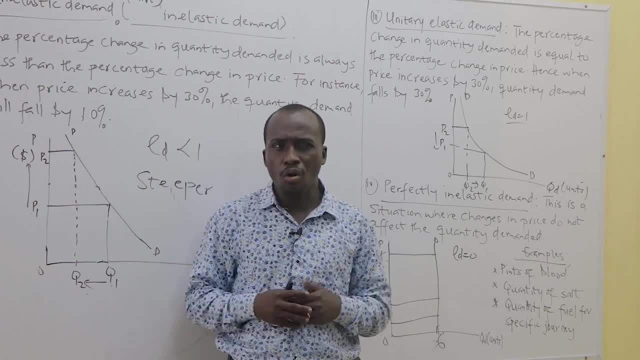 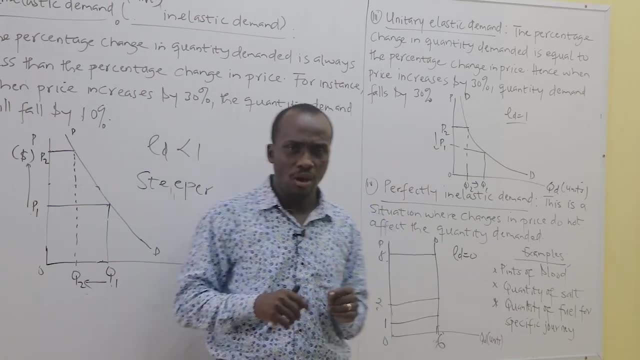 behave that way. it's only few commodities. you cannot think of a more common behavior that will. the price change is, yes, the demand remains the same. it's very few, but they are very exceptional commodities you can think of and yet the elasticity is equal to zero. ются is going to zero because quantity remains. 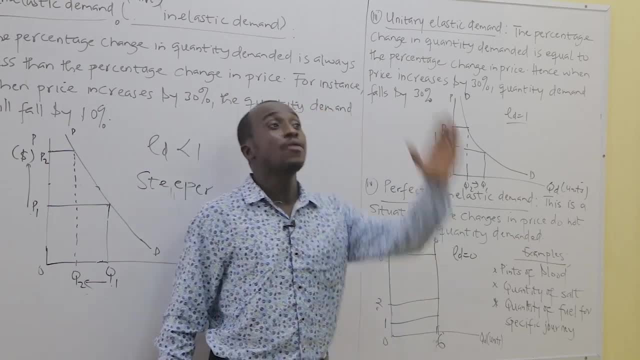 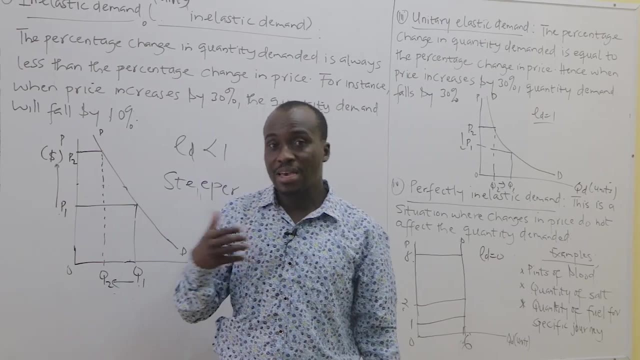 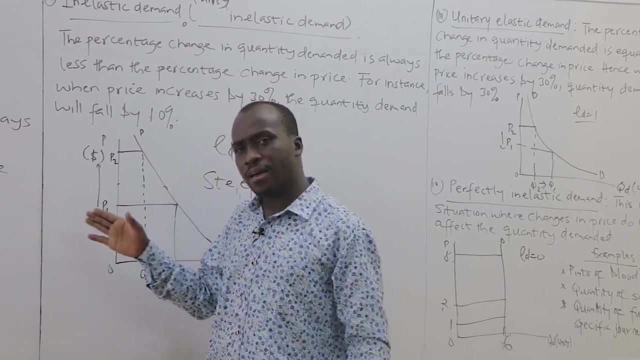 constant. the quantity you're buying at one moment remains constant, so the elasticity is equal to zero. later, when we start solving these things, when we get the answer, we can try to crystallize them. Is it elastic or inelastic? So don't be oblivious about their sign. 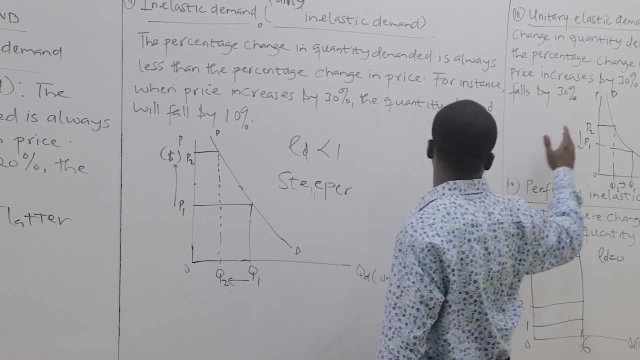 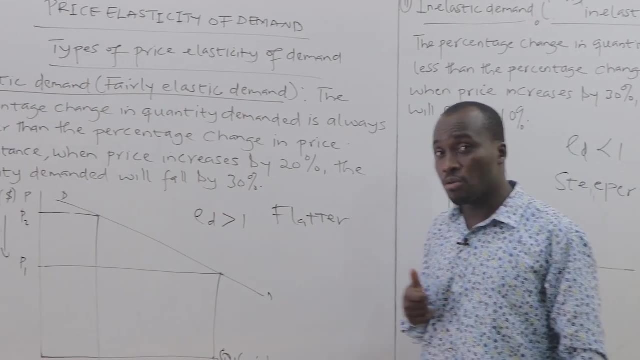 This is greater than 1.. This is less than 1.. This is equal to 1.. This is equal to 0.. Let's look at the fifth type of elasticity. Then we go on with our lecture. Let's look at the fifth one. 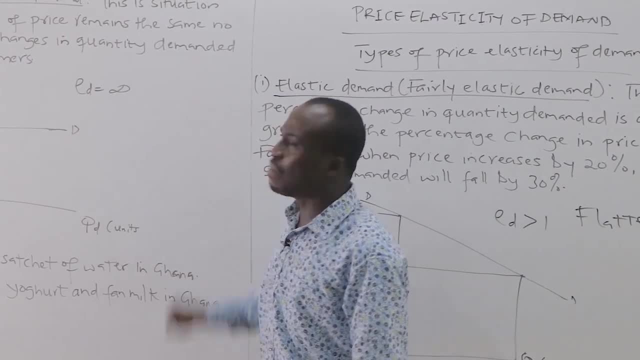 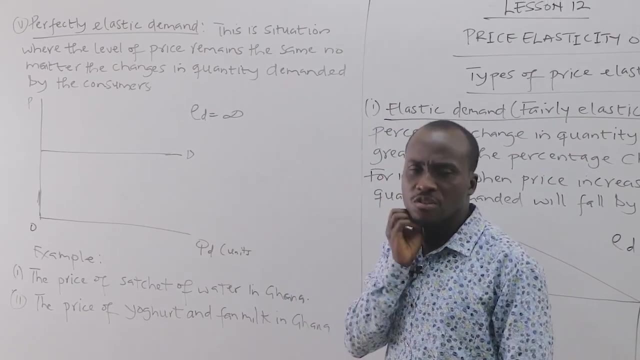 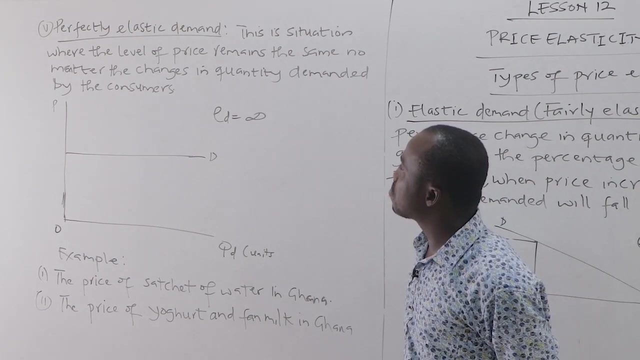 The fifth one talks about perfectly elastic demand. And here we have what? Elastic demand, or fairly elastic demand? We have perfectly elastic demand. Don't confuse the two. What is perfectly elastic demand? It is a situation where the level of price remains the same. 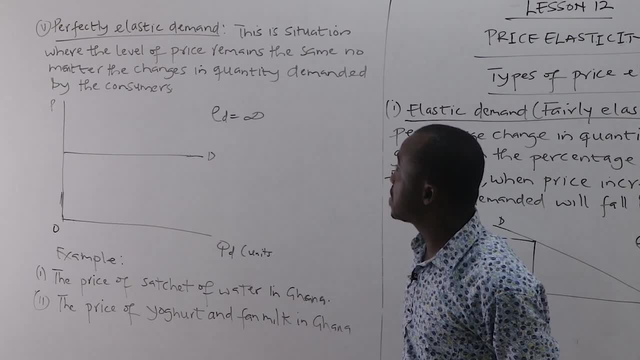 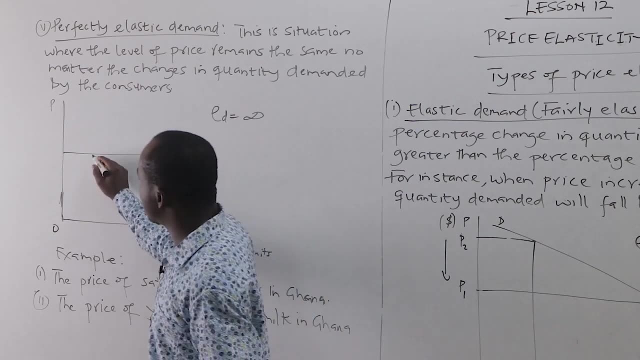 Remains the same, no matter the change in quantity of demand by consumers. So what does it mean Here? the price is the same Whether demand increases to 4.. If demand is 4, the price is 8.. The price is still 8.. 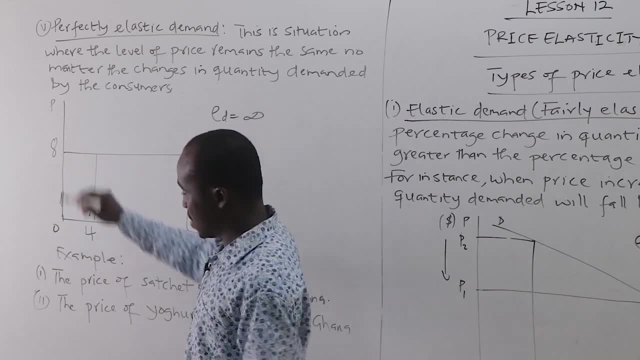 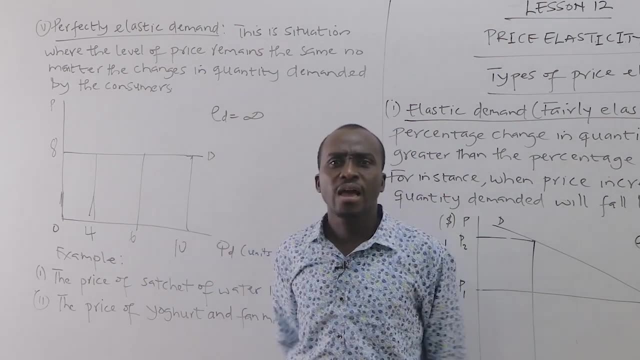 If demand increases to 10, the price is still 8.. If demand goes to 6, the price is still 8.. So the price remains the same regardless of the change in quantity of demand. So whether quantity of demand increases or decreases produces the good at the same price. 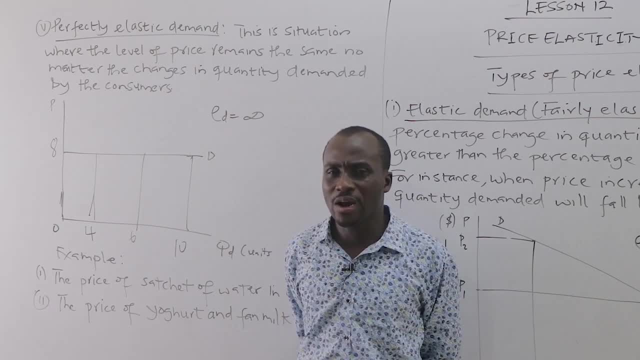 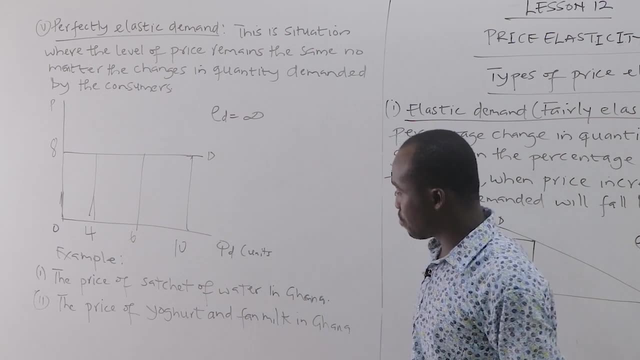 That's something also very difficult to fathom. How does this thing work in the real world? There are a few commodities that behave that way too. What are some of them? In Ghana, for instance? the price of sachet water, for instance, in Ghana. I don't know. 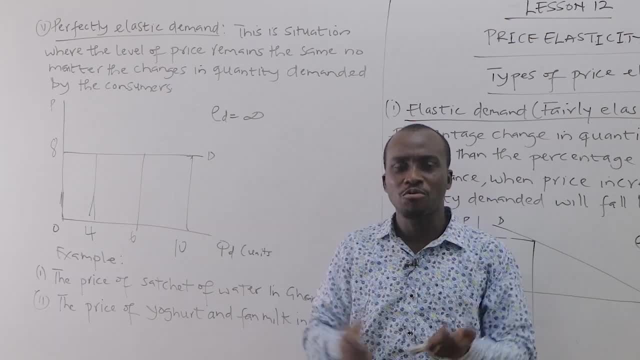 but we back here in Ghana, we have water. they put it in sachet water. we drink The price. We have one. it's been sold for 20 pesos and the price has been the same for the past 6-7 years, right? 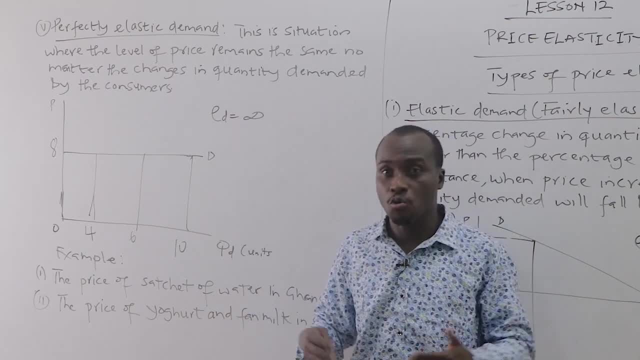 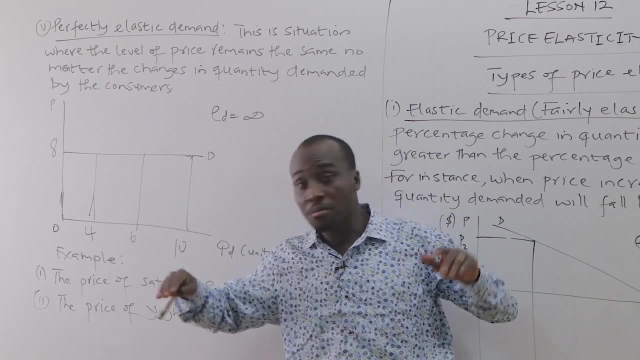 People are demanding more. Every day in India, people drink water. Yes, sir, the price has remained the same almost about 6-7 years. you are buying the same at the same price. We expect that, as the demand has gone up, the price will go up. but yes, people are buying the same. 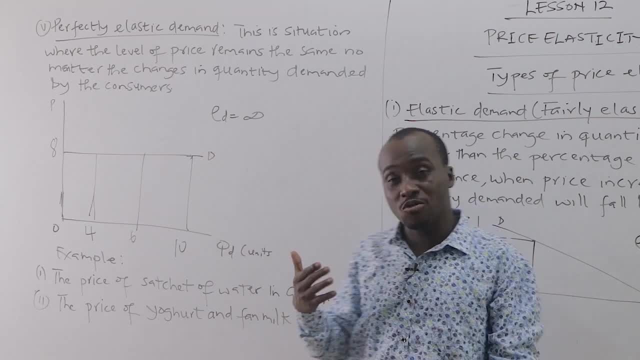 The price is still the same, The price of in Ghana also, we have what we call yoghurt and farm milk. I don't know what they have in Senegal or Ivory Coast or wherever, or Caribbean. who are listening to us? 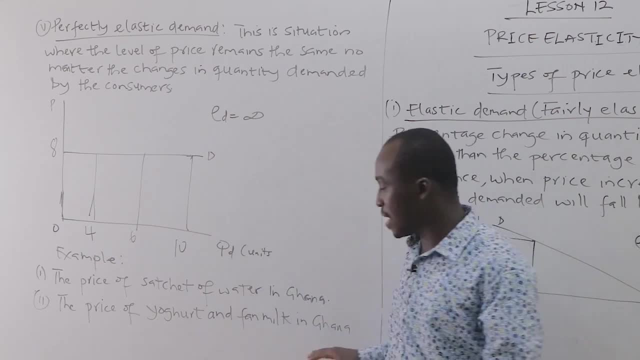 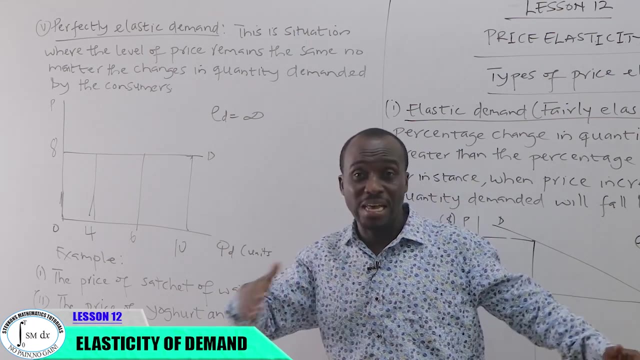 The price of yoghurt. they are just ice creams We use in Ghana. The price has remained almost the same: 1 CD to 2 CD. The price has almost remained the same for so many years. It remained the same for almost about 8-7 years- that recently they changed it. 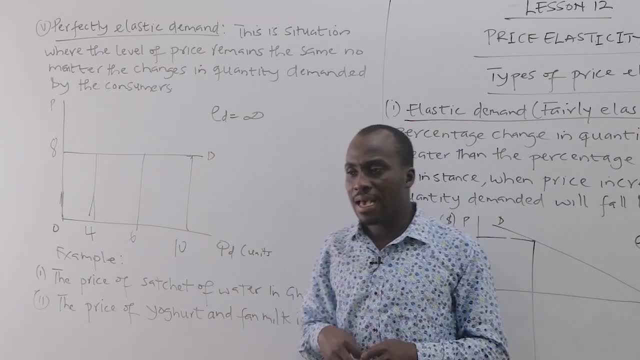 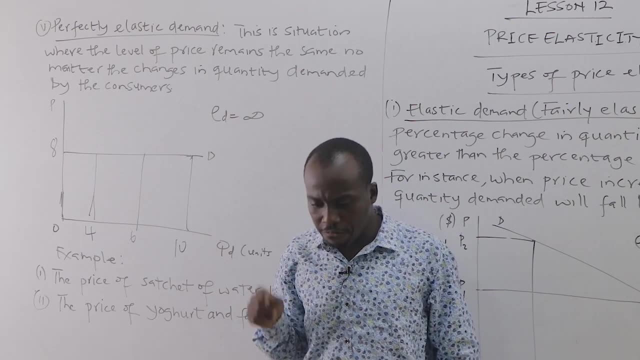 So there are few commodities that behave that way. right, But it's very difficult. It's only few commodities that behave that way And elasticity here is equal to infinity. Let me first, let me activate. let me reiterate that I told you about 5 types of elasticity. 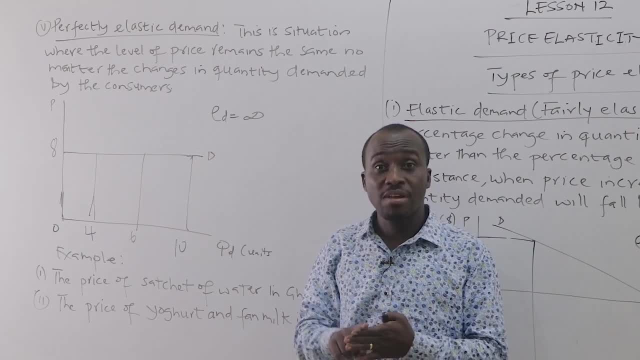 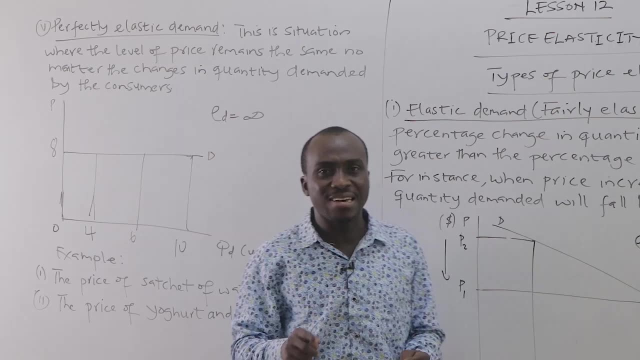 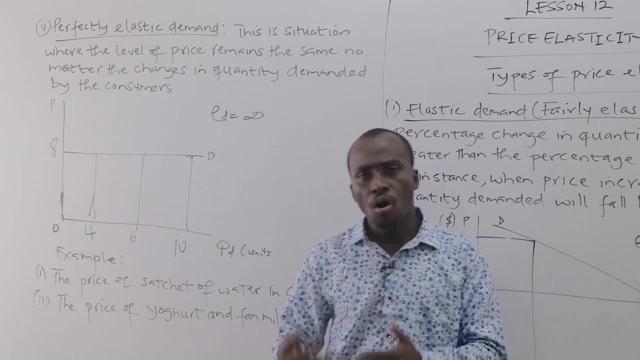 Elastic demand, inelastic demand, Elastic demand, unity elastic demand, perfectly elastic demand, perfectly elastic demand. Among all these five, perfectly elastic, perfectly elastic, unity elastic are extreme forms. Only few commodities behave that way. Most of the commodities we buy on the mall, on the markets. 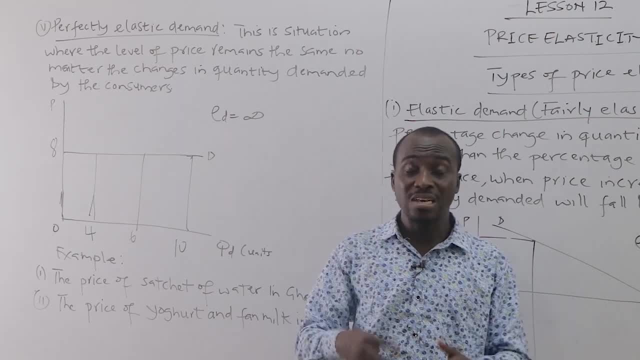 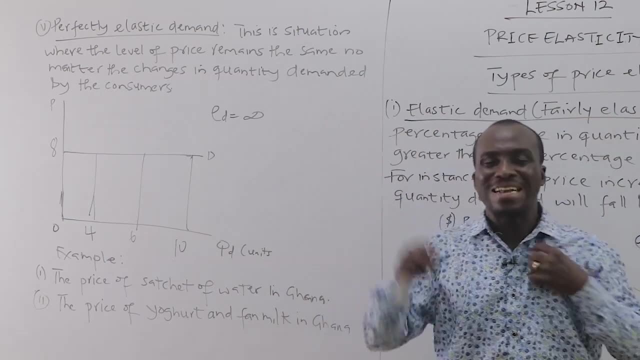 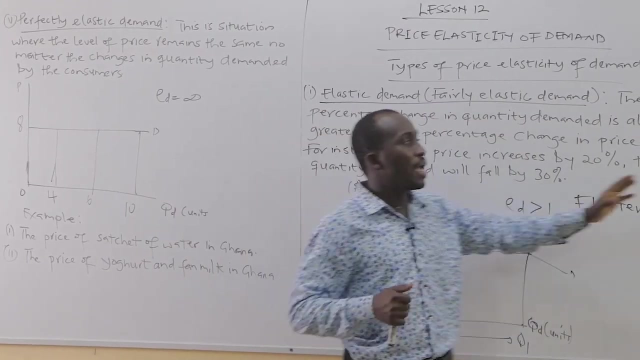 in our homes, in our schools, in our job. most of the commodity can be categorized into elastic or what Inelastic. So majority of them, about 95% of the things we buy, is either the commodity either is elastic or inelastic. That other three are extreme forms in hardly all case, by having 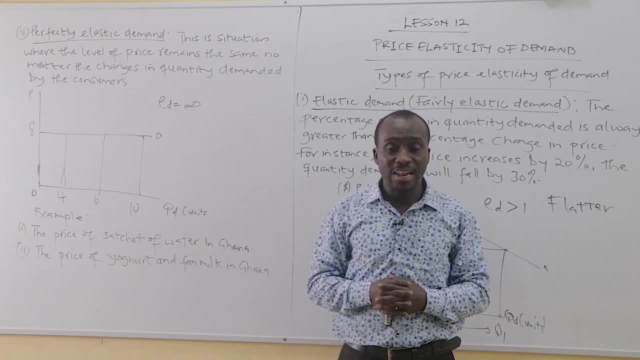 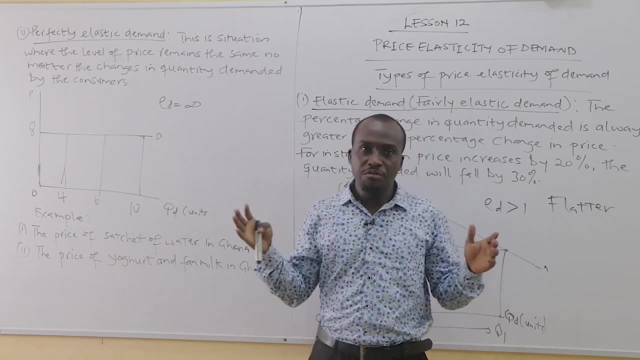 in early exceptional cases. Once again, I want to tell you that all these things we have in here, we have them on the pen drive. This is Lexator for you. We have up to. we're going to have 15 set of. 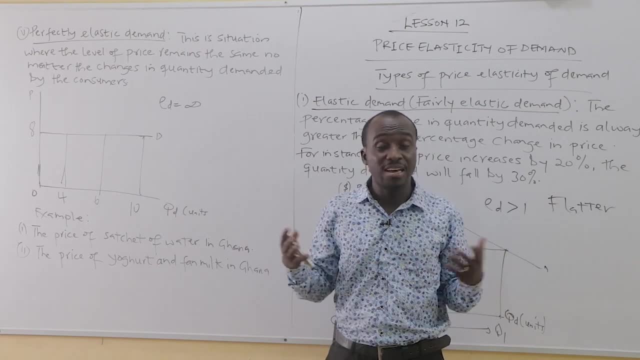 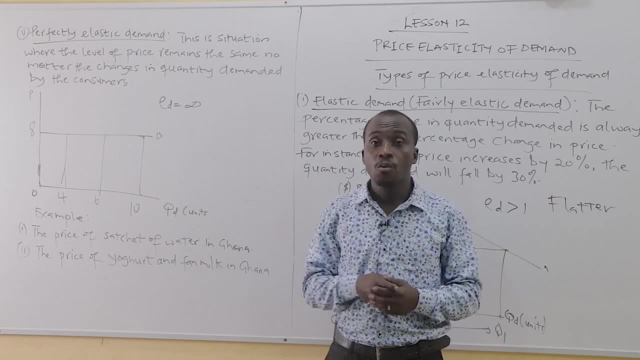 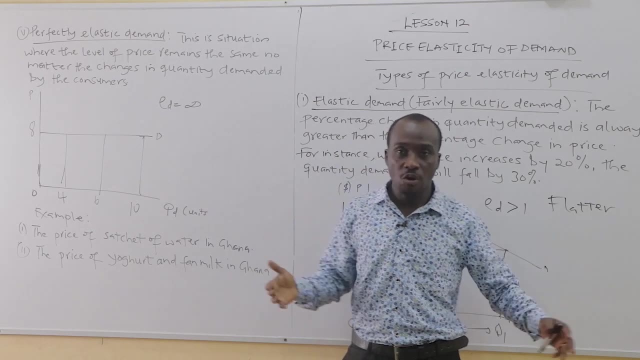 everything to you. here Again, you have the book. In the book we have all these notes, the data response. We have a place where you can also solve questions and mark yourself. We have over 200 objectives for you too. We have CD. that comes with the book. So 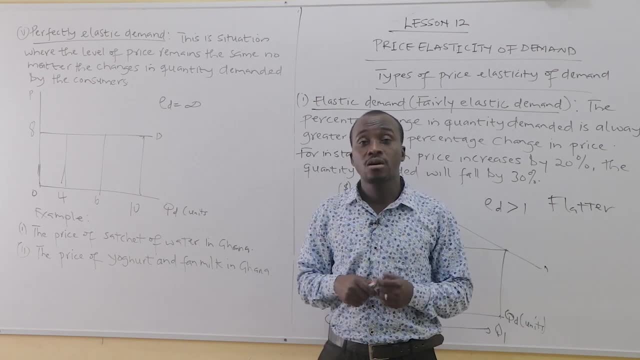 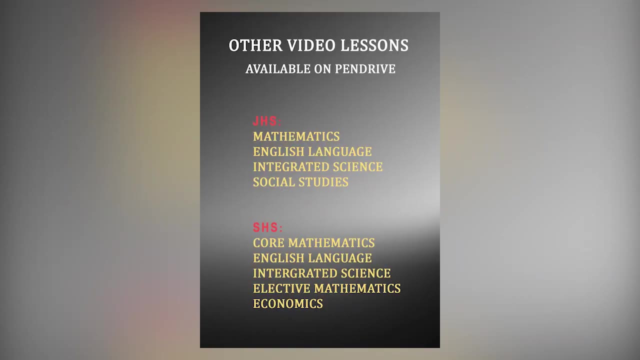 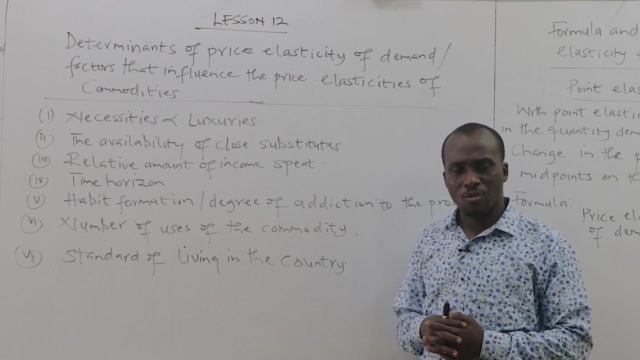 these are things for you and I hope you follow all these lectures very continuously. We have come to one very important aspect of this topic and one of the most popular questions they ask in the WASI. I tell you that most of the goods you and I will buy on the market. 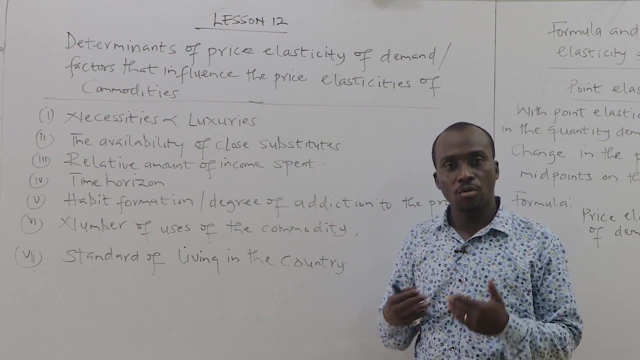 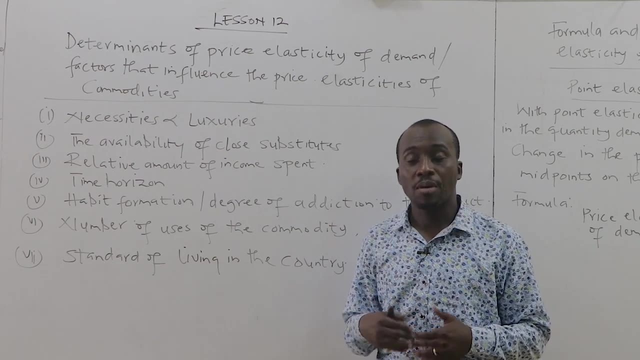 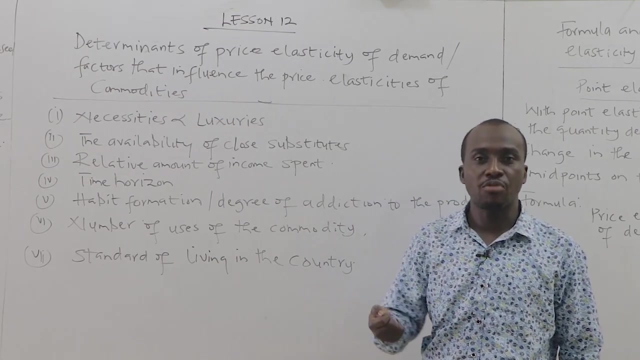 most of them are either elastic or inelastic, And I said that when the commodity is elastic, it means that it is very sensitive to change in price. The slight change in price bring up a large change in the quantity demanded. When a commodity is inelastic, it's not too much sensitive to change in price. 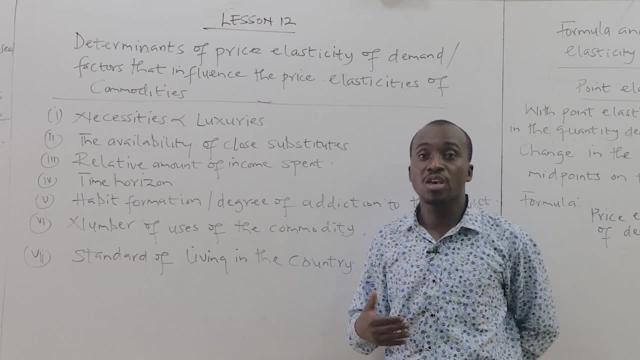 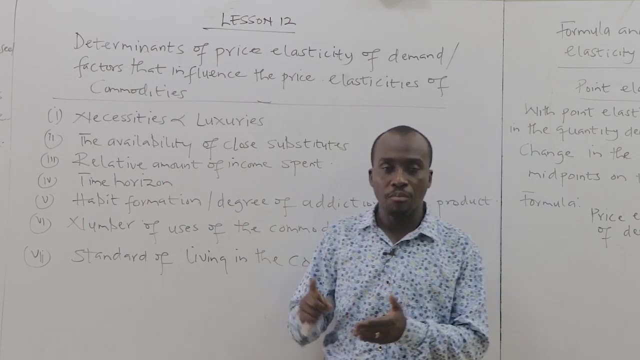 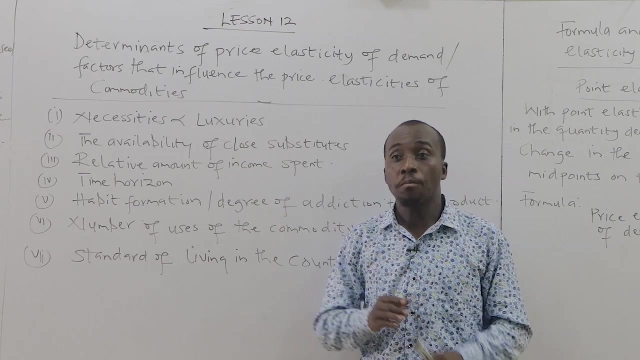 So if the price even increases, people keep on buying the product. Only few people stop buying. So most of the things we buy, whether in America or Canada, in South Korea or Japan or China or India or Ghana or wherever- in Nigeria, Senegal, Sierra Leone- Most of the things we buy. 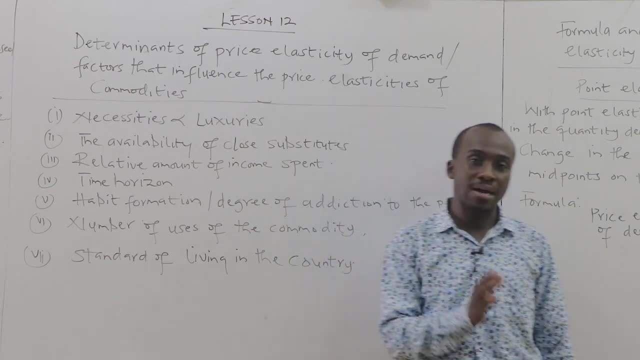 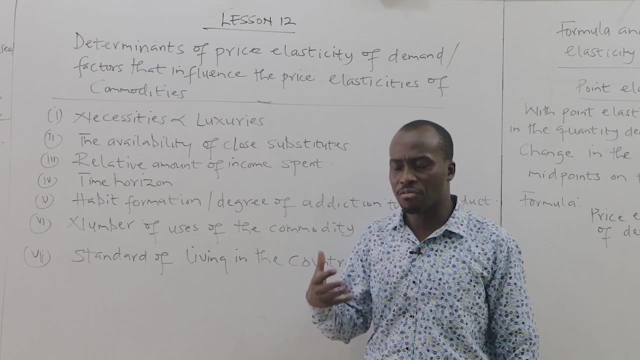 majority of them is: either the commodity has elastic demand or inelastic demand. So you want to find out what are some of the factors that actually precipitates or what are some of the factors that make some of these goods inelastic. What are some of the factors that actually precipitates or what are some of the factors that make some of these goods inelastic? 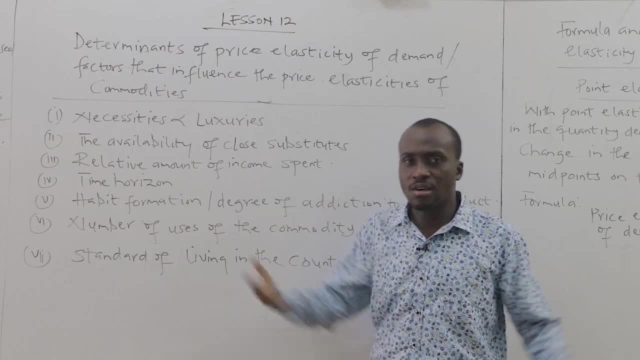 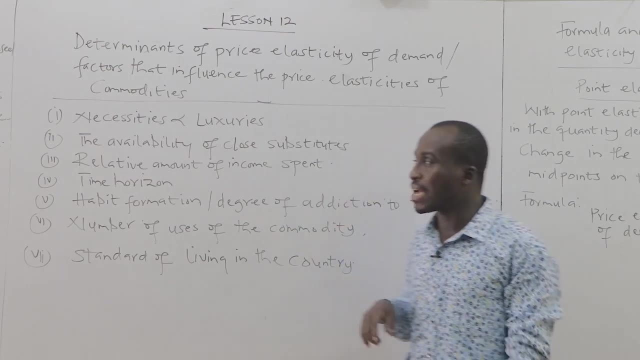 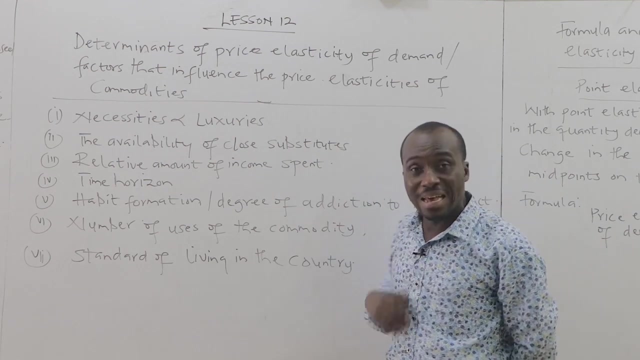 goods elastic or inelastic? Is it of just a miracle that some goods behave elastic, some goods behave inelastic? So let's try to fathom what actually cause these things. Number one: one of the reasons that cause a good being elastic or inelastic is whether the commodity is a 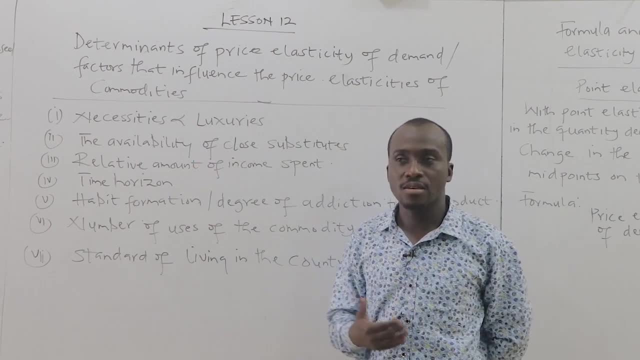 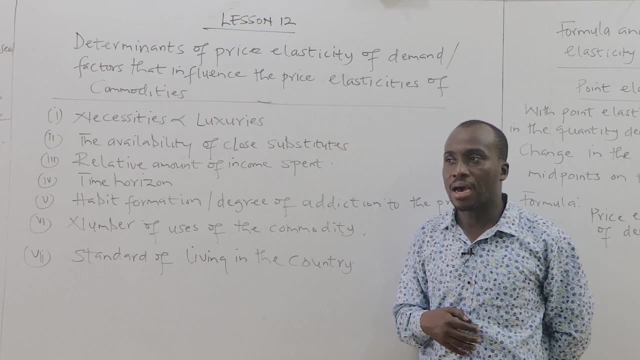 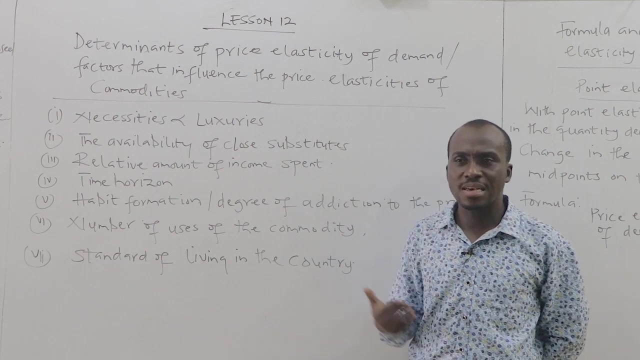 necessity or is a luxury? What is a necessity? Necessity is a commodity you cannot live without, like food, like shelter, like clothing, like accommodation and those things. They are necessities. So if the price even increases, you cannot say that you are not going to wear clothing again. 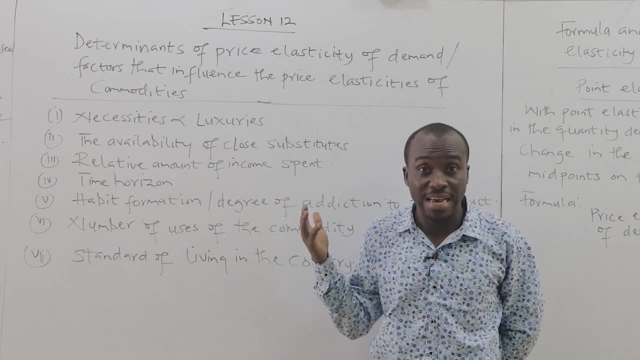 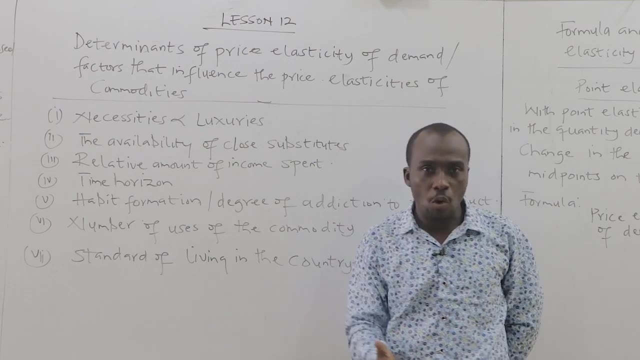 if all kinds of clothing have gone up? You see, now you want to walk naked in the 17th century, Or what would you do? You keep on buying. Maybe you reduce your quantity by a small margin, but you keep on buying. You can't say that there's water is expensive, so you don't drink water again. And what are you going to do? Right, Such things are a necessity. A necessity tends to have inelastic demand. Even if the price increases, only few people stop buying. The rest we keep on. only few people- a majority of them- will keep on buying. You just complain. 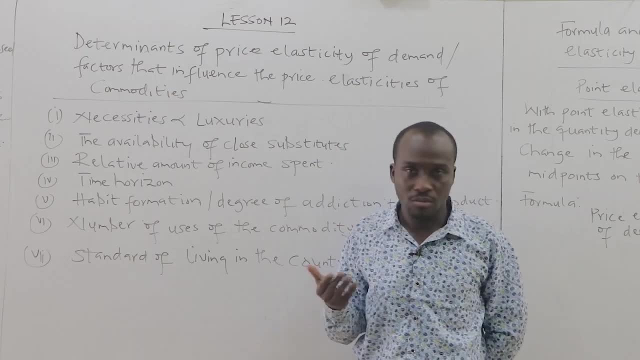 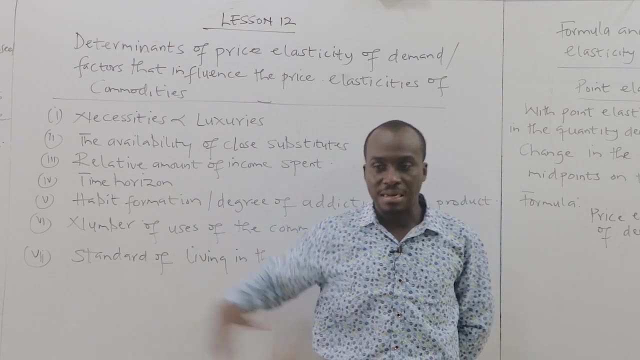 for two days, three days. you go back and buy because you cannot live without them. So components that are necessities tend to have inelastic demand. So those who sell such a product, they take advantage of this and increase the price astronomically. Because if there's a drug, you need that drug to survive Every day. What will you do? Will you say that you will not take the drug because it's expensive? Even if you have to go and sell your property to come and buy the drug? you will do that. 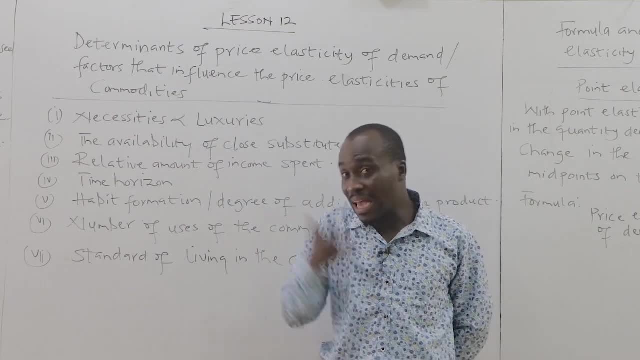 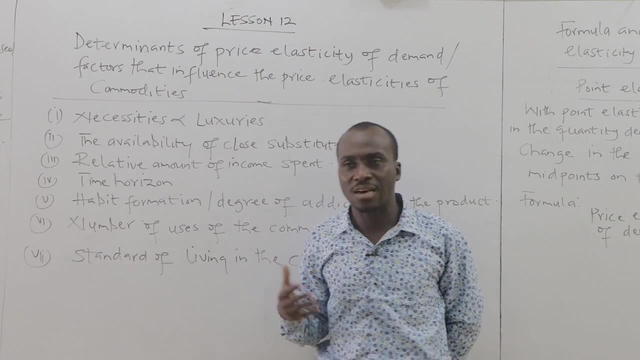 So your demand in that instance is inelastic. Regardless of the increase in price, you are still demanding it Because you cannot do it When a commodity is a luxury. when a commodity is a luxury, there are goods you cannot do. you can do without them. If you have it, fine. If you don't have it, it's okay. 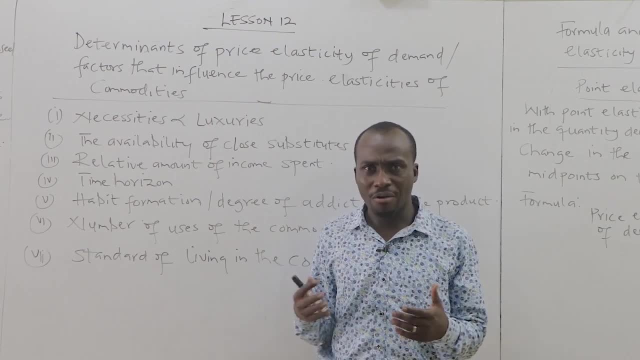 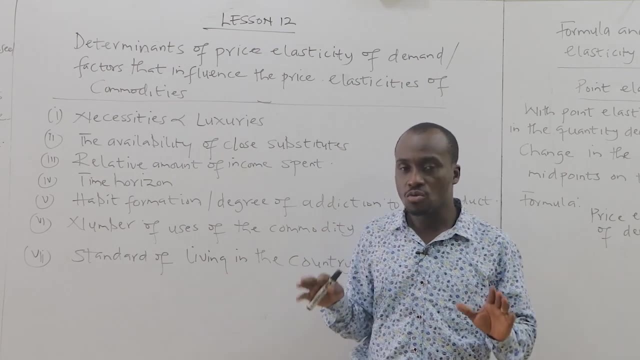 Somebody said I have a diamond ring. Somebody went to buy a diamond ring, maybe $100,000. It's nice. Maybe you want to show to everybody that you also have arrived? Fine, That's cool. You want to be someone who is an illustrious person? Fine. But 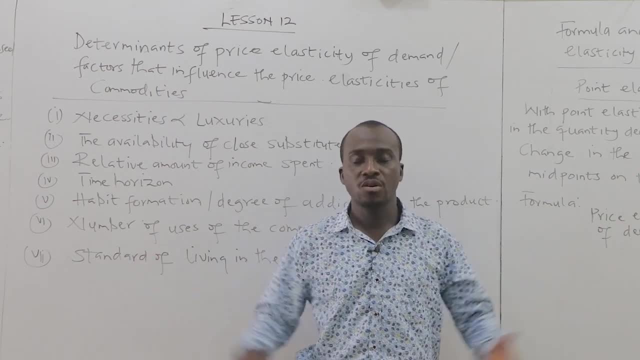 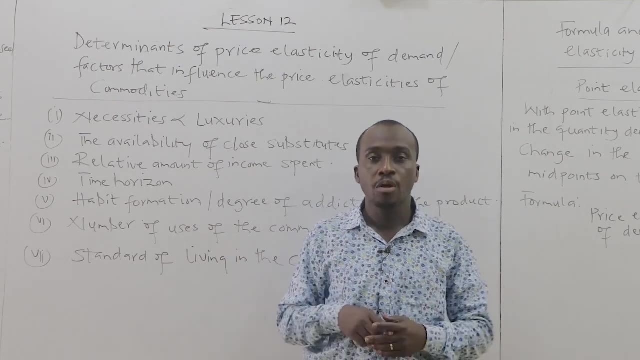 if you don't have it, you will not die. I have not seen a diamond ring. If I don't have a diamond ring, I'm still alive. Such goods are cosmetic expenditures. Maybe you want to show off class, that you are part of the bourgeoisie's class? Fine, But in a real sense. 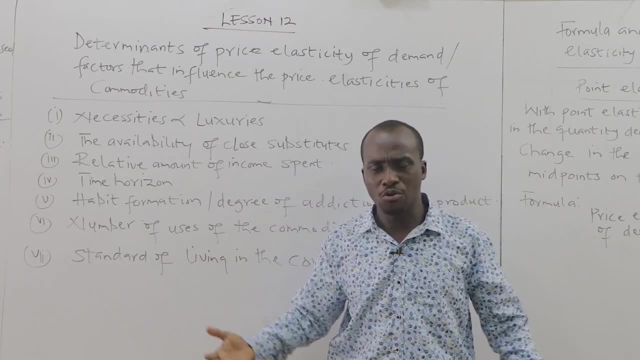 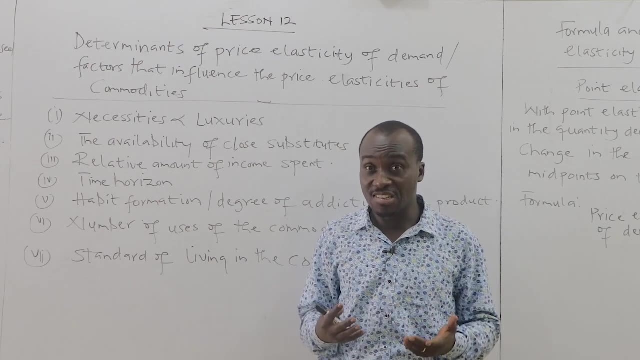 if the price increases? if the commodity is a luxury to you, what will you do? You try to shift away from it Because you cannot do that without it. If the prices are good, the price is too high. My demand will be very sensitive. I will decide not to buy it, Because without it. 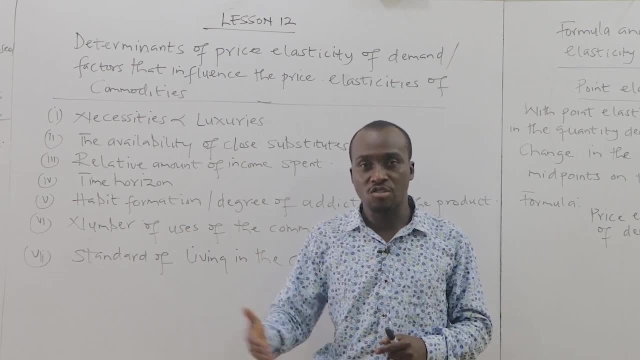 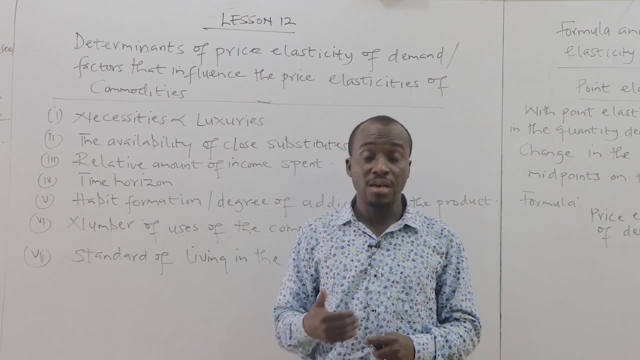 my life goes on. So commodity that tends to be a luxury to you- and sometimes commodity that tends to be luxury- tends to have elastic demand. Commodity that tends to be necessity tends to have inelastic demand. But let me say this pertinently, perpicuously. let me say that 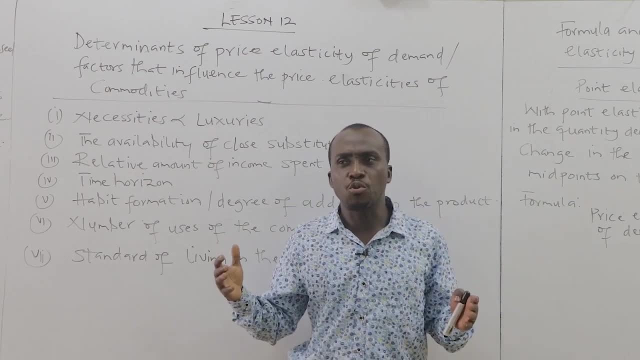 whether a commodity is elastic or inelastic, it depends on you. Some of you say that, oh, private cars are luxurious. No, it depends on what you're doing. If you're a very busy person, you need a private car, right. 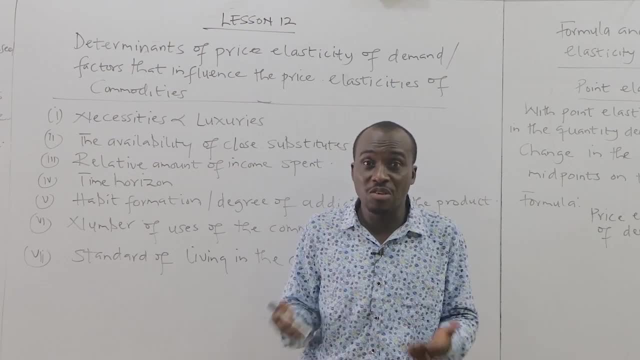 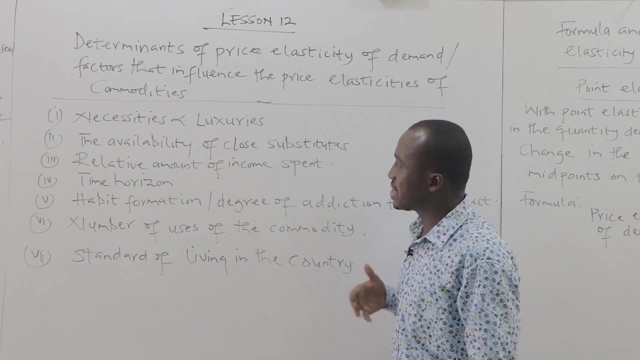 People that are not very busy. a private car will be a luxury to you, But somebody that is busy, you have a lot of rounds, you need a private car. See that. So when a commodity is a necessity, it tends to be elastic. When a commodity is a luxury, it tends to be inelastic. 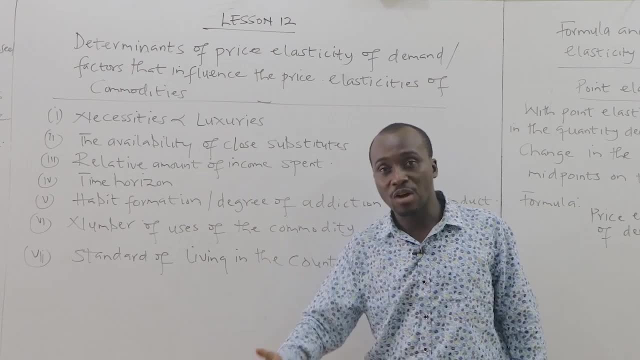 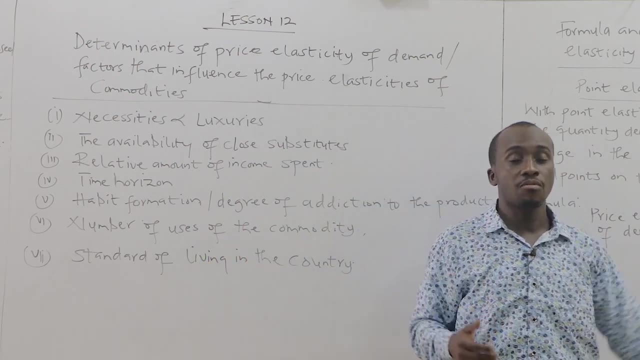 And when a commodity is a necessity, it tends to be inelastic. People cannot do without it. When a commodity is a luxury, it tends to be elastic, Because people are prepared to shift from that commodity and go and buy the commodity they want, because 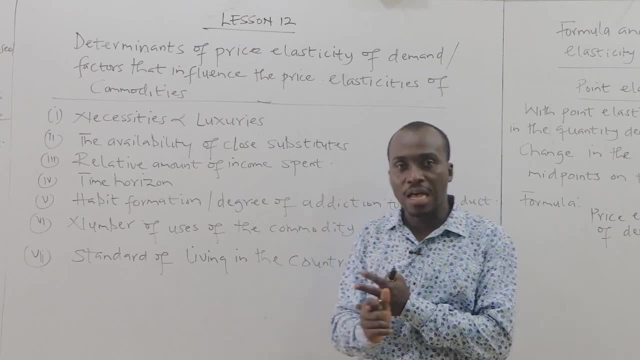 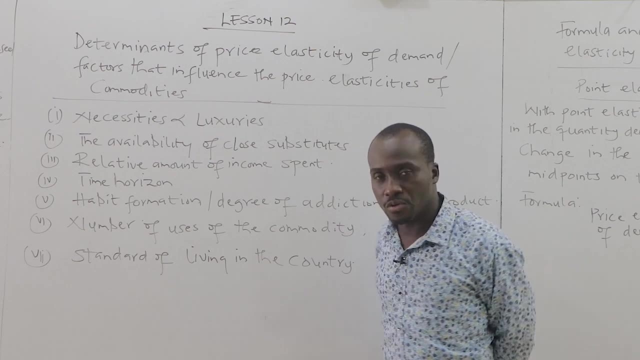 it's a luxury to them. So necessities are inelastic. Where goods are luxurious has elastic demand. demand number two: the availability of closed substitutes. the commodity you're buying doesn't have closed substitutes on the market. if we are going to buy, I'm 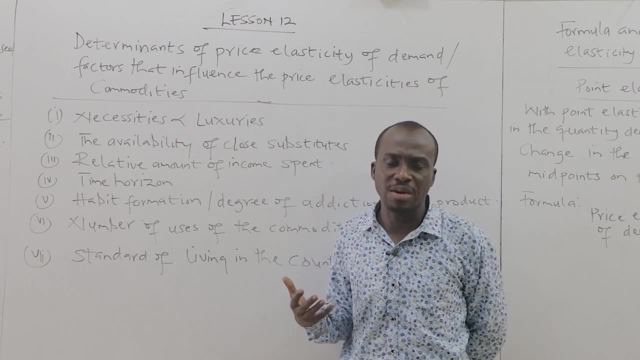 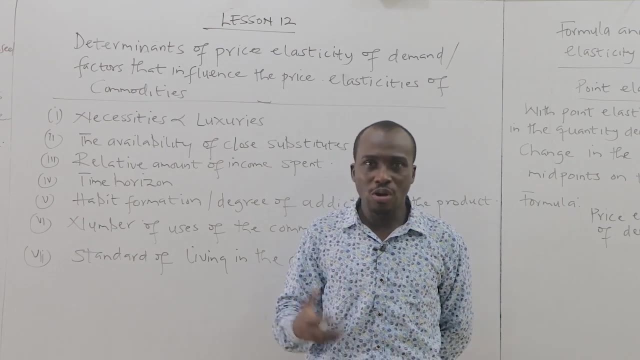 going to buy cement and when I went to the market, there's only cement that Gassam cement us some years back, Ganesh, to have Gassam cement. if you want to build your hardware with cement, you have to buy from Gassam. what do you do if you go to? 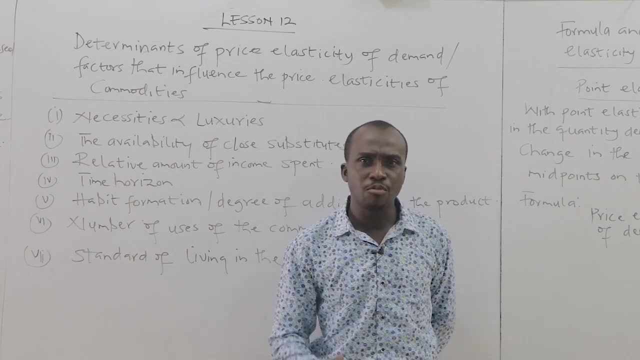 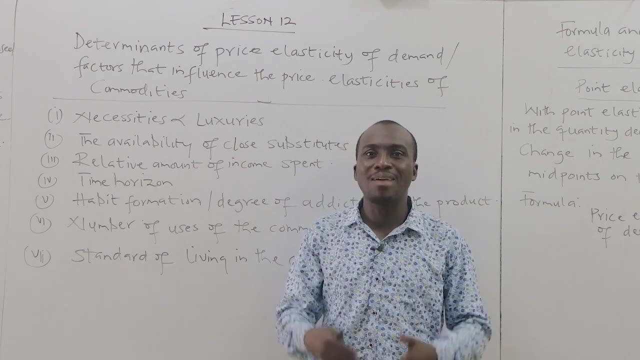 the price I'm going up, you are still demanded. maybe you're going to buy hundred bucks. you carry them. divide 90 bucks, right, but I still demand it, right. well, you don't have any place to get something to buy again. did they allow for any imputation and they allow for any manufacturing? so if you come on, 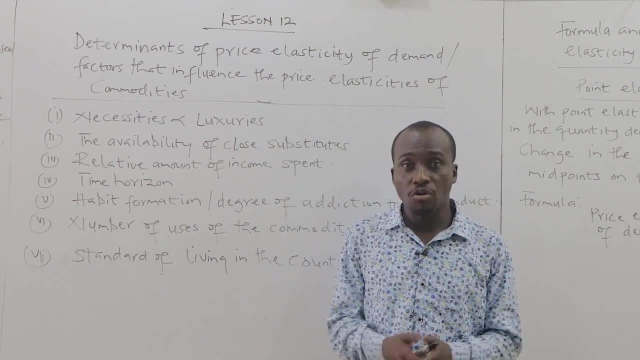 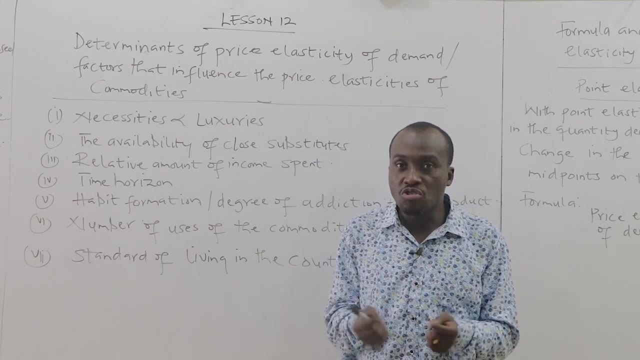 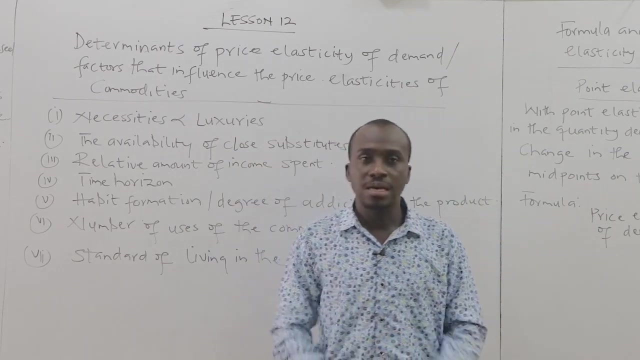 doesn't have any substitute. you're marginalized, you're being forced to buy the product and therefore, in that case, a demand becomes inelastic. the price have gone up. you can reduce your demand by small money, but you need a community at all costs. it doesn't have any clues of it. you need to build your house in. 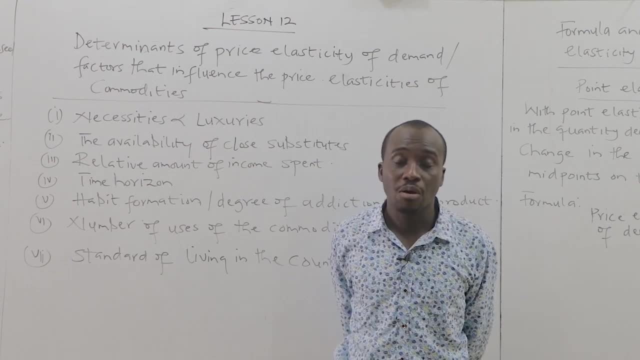 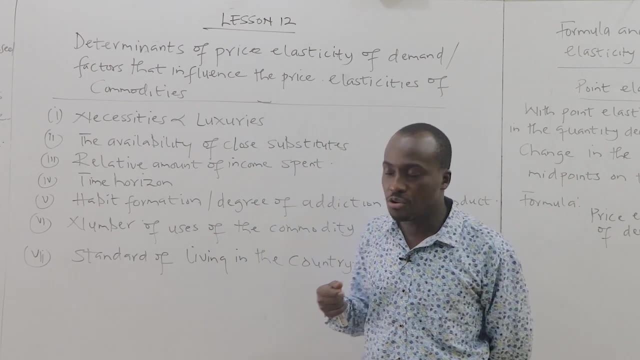 Gassam, Ghana. we don't build house with with. we don't build house with with wood. we build house with cement. I don't know, in some country they build house with wood and all those in Ghana. we don't do that if the commodity has substitutes. if I'm 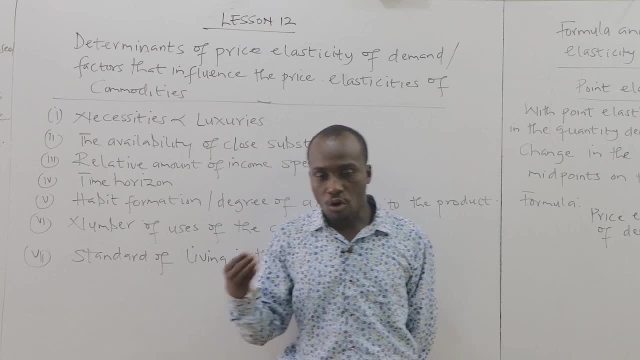 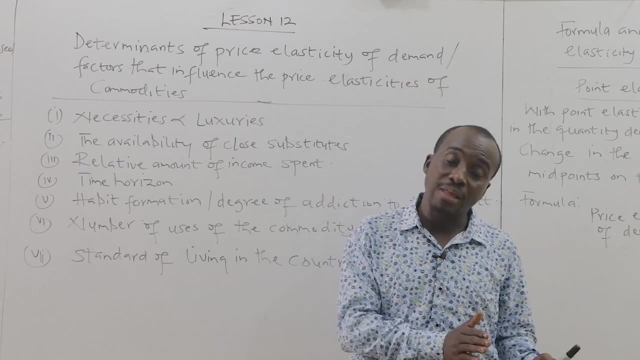 going to buy pertinence. there's Colgate if I go and I've got personally, the toothpaste is the toothpaste in Ghana. if the price is too expensive, what would I do? I move away from that and whereby a substitute. so any commander have substitutes. 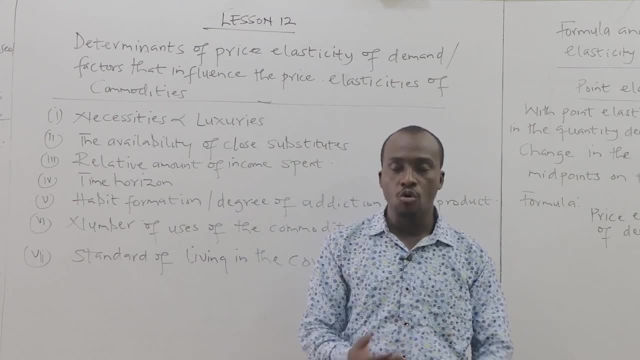 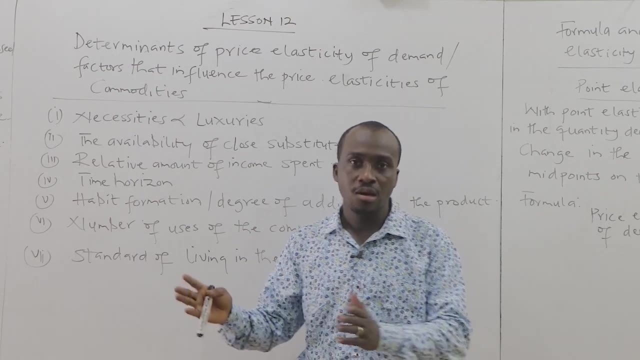 tends to be elastic because you can easily switch. if I go and the price I've gone out for maybe, president, I'll have a higher response. our response, very high, to the increase in price, by moving away from the purchase of president to go and buy close-up. or you can say: cast, I want to buy a. 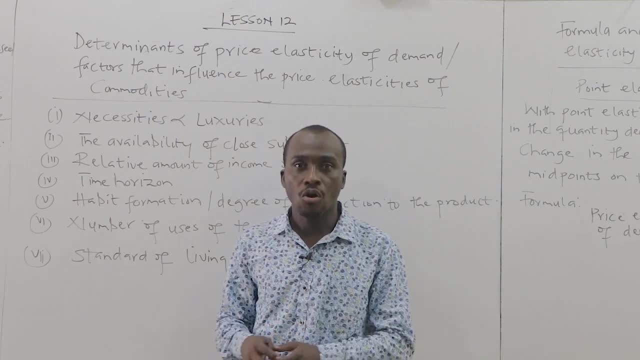 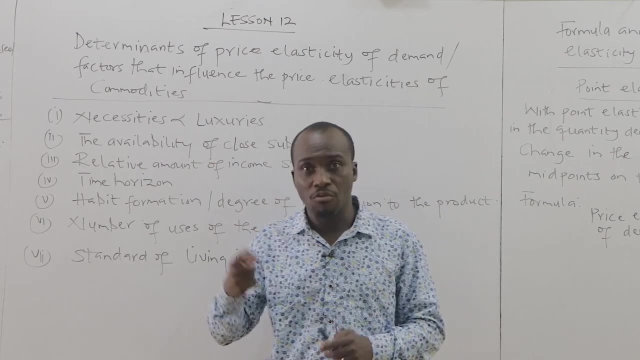 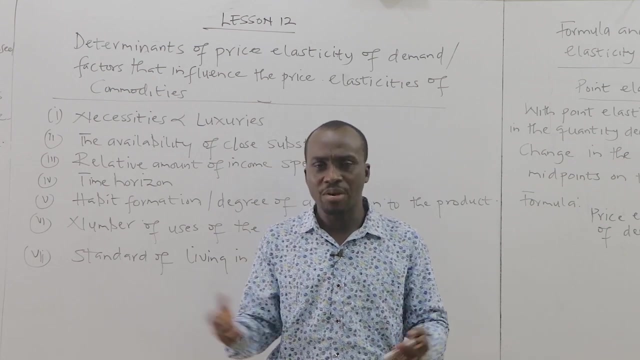 Toyota car when I went to take a very expensive hand design or care, what about? so once they have substitute, demand tends to be elastic. so if you are selling a product, you have to be very mindful about this: that if my product is a substitute, act should I behave. if it doesn't have any substitute, I should. I. 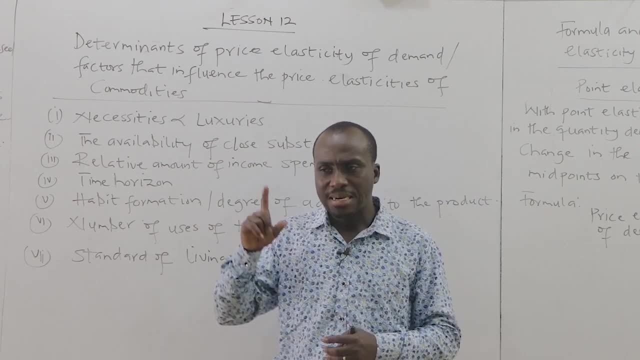 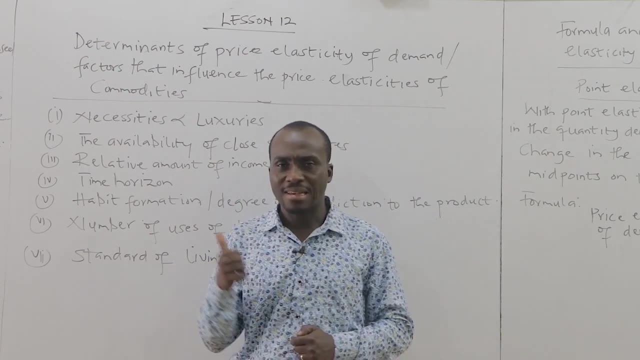 be so. people who works, who are truly operating. the market takes all these factors into cognizance when it comes to fixing their prices. they're able to phantom that their product you're selling has an elastic demand, or any elastic demand in so dear you have to think about how you have to price it. 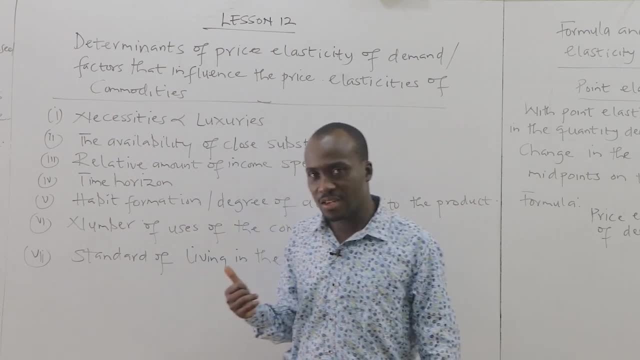 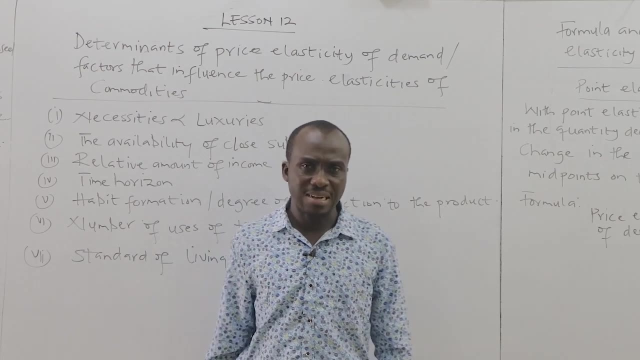 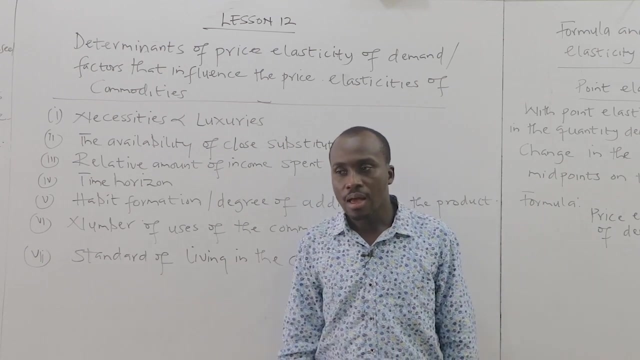 starts what I told you, the the idea of the solicitor is the only for you to write the exams and guau. also for everyday knowledge, those writing to business won't do anything to business and that's when government tax expense is very important for them. although we look at the amount of income spends, how 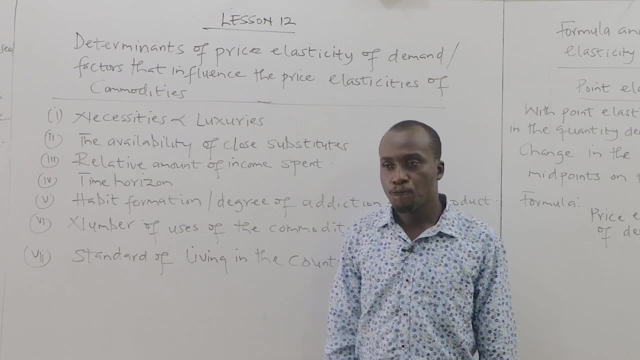 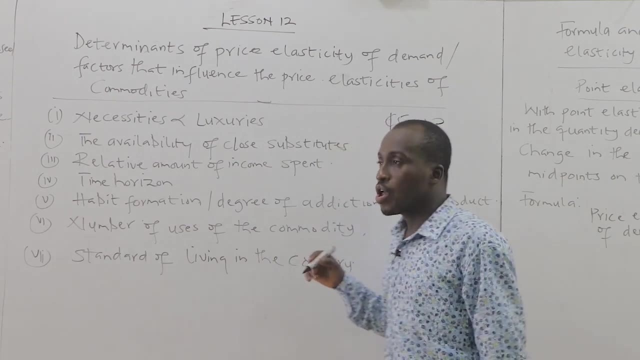 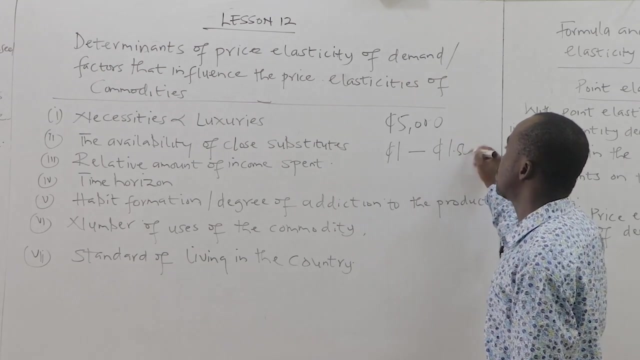 much of your income do you spend on the commodity? maybe you take 5,000 Ghana cities. let's assume it as somebody who earns 5,000 Ghana cities. he's going to buy a pen. when he went, the pen was one CD and the pen is one CD 50 pesos. you. 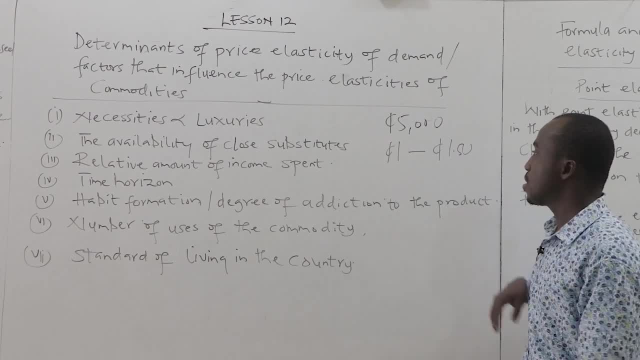 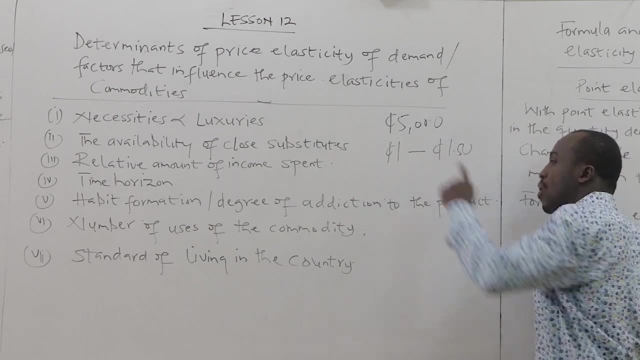 see that the price have increased from one CD to one CD per pesos. but you see that the person earns so much of money- the salary is too large- that this 50 pesos constitute a small chunk of his income. what is 50 pesos to somebody who earns? 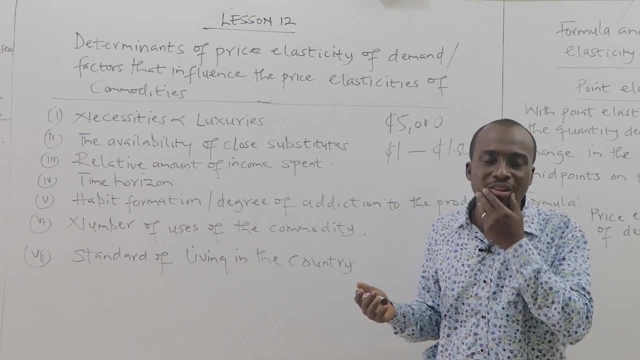 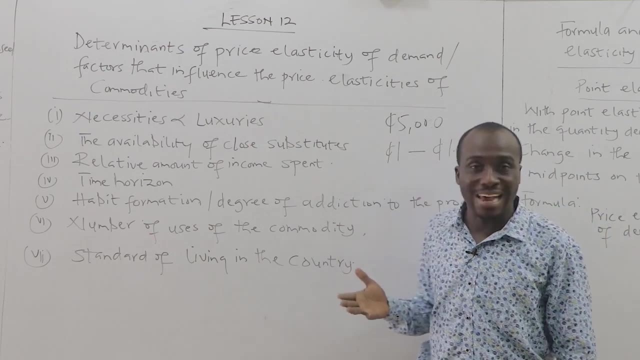 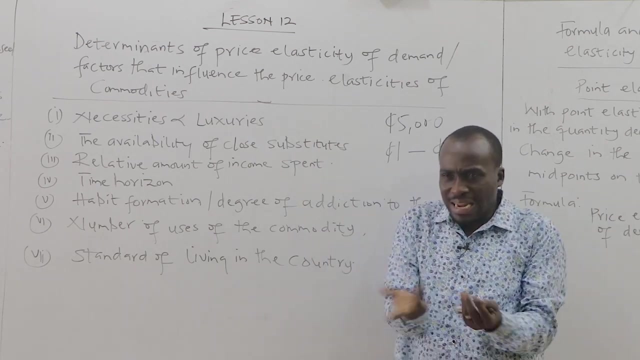 5,000. it's negligible. so he will not even notify that the price are gone up. so, Goose, any commander takes a small chunk of your income. your demand becomes inelastic. if you go and leave, the price have gone up anymore. you don't even take notice because that money is very negligible. it doesn't affect your. 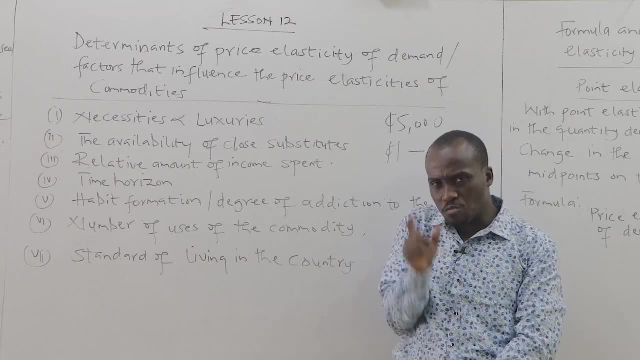 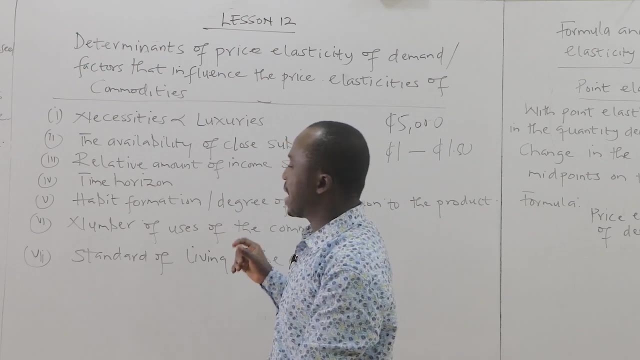 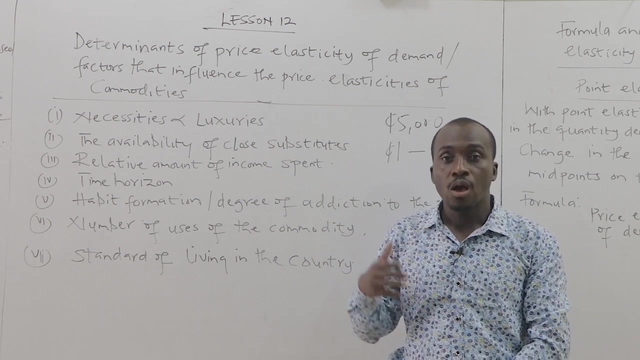 salary. so much so you're okay. so, Goose that takes a small expenditure of your income, Goose that takes small amount of your income, tends to be inelastic. you sometimes lose sight that even a price have gone up because it doesn't matter. it doesn't it all to you. but, commander, take a higher chunk of your income. 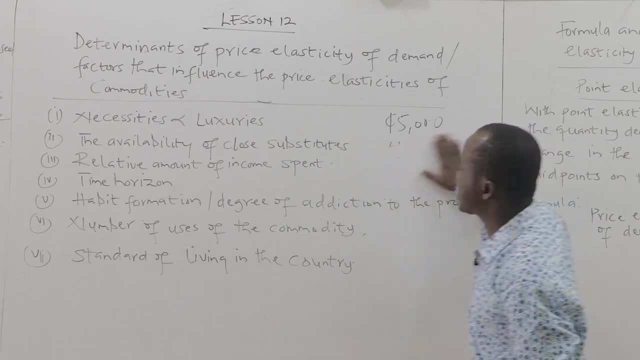 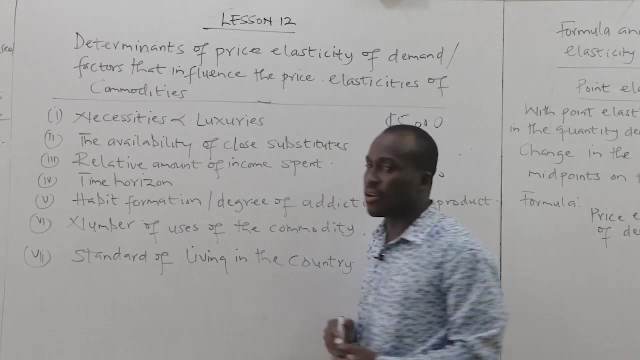 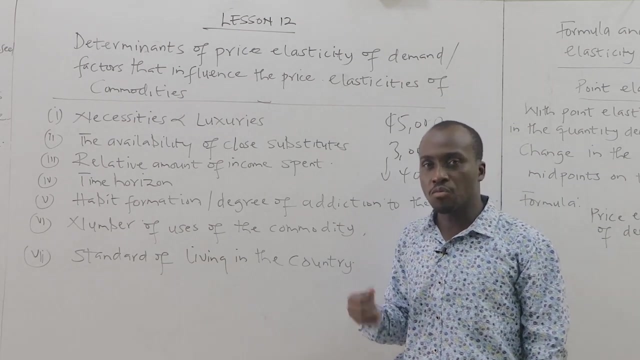 if I earn five thousand- I'm good by pronoun it- put up the straight thousand. when I when the price have moved from three thousand to four thousand, I'll be very mindful by the increase in price, why, if I buy the product, it have taking almost all my salary. so, commander, takes a higher chunk of your income in most. 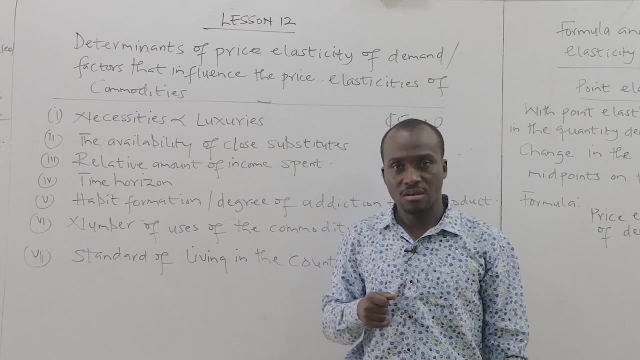 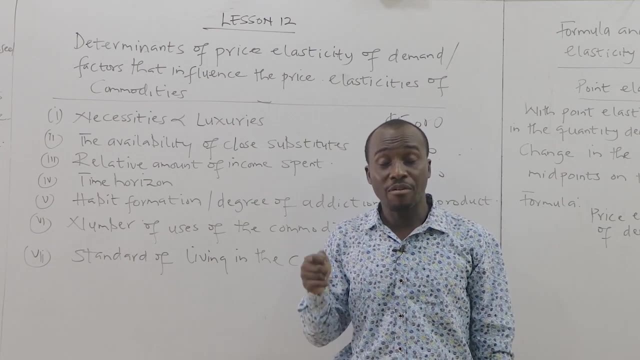 cases, company tends to be inelastic. right commit, tent to be elastic. story comedy that takes a higher chunk of your income in most cases springs to be inelastic. what community we last story company it川向あの. a higher chunk of your income, the commander. you become very sensitive to change in price because 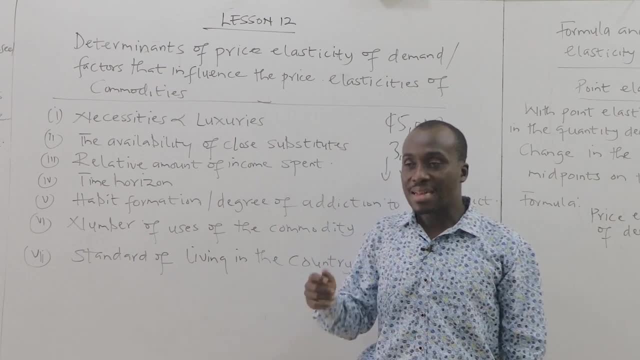 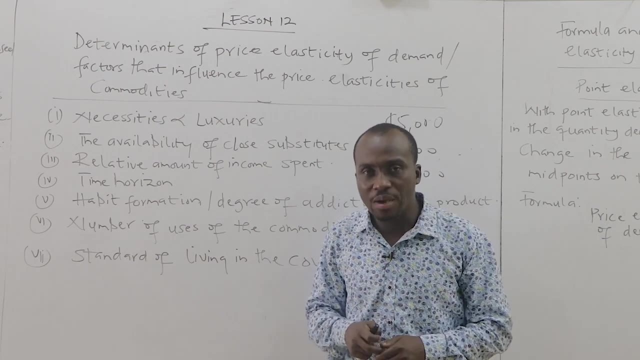 you can become very sensitive to change in price. another, commodities that take a higher point of income tends to be elastic. commander takes small chunk of your income, tends to be inelastic. and quarter takes a higher chunk of your income, tends to be elastic. so yeah, you're beginning to. 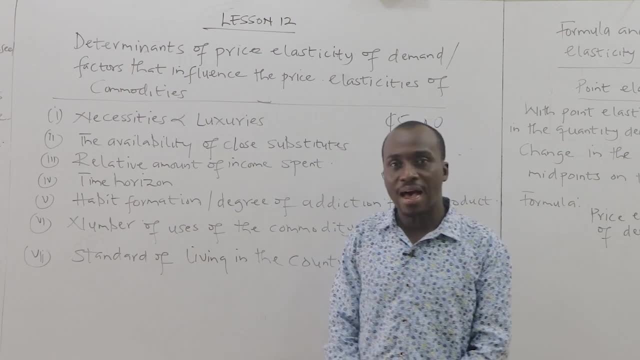 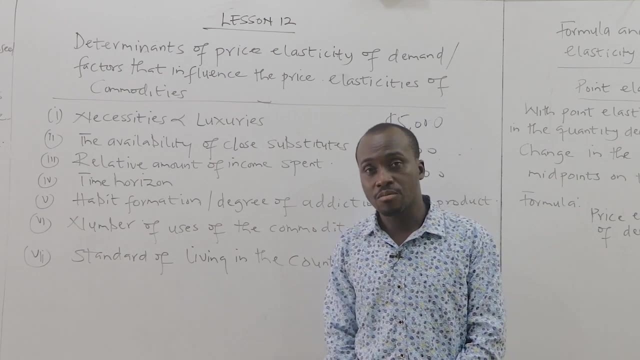 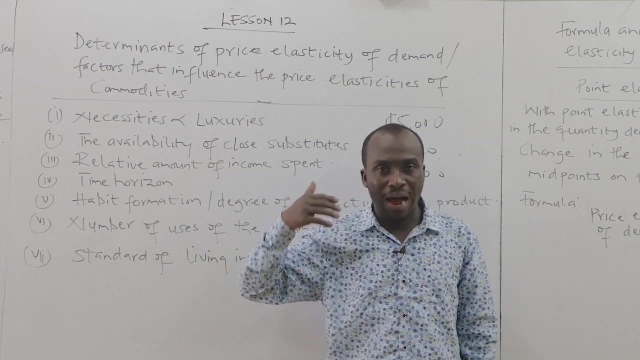 understand why some groups are elastic as a moves are inelastic. the commander takes a small chunk. your income tends to be elastic. the commander takes the higher chunk of income tends to be elastic. so we have: what about a time period, the time period you saw you. you buy the product. it's 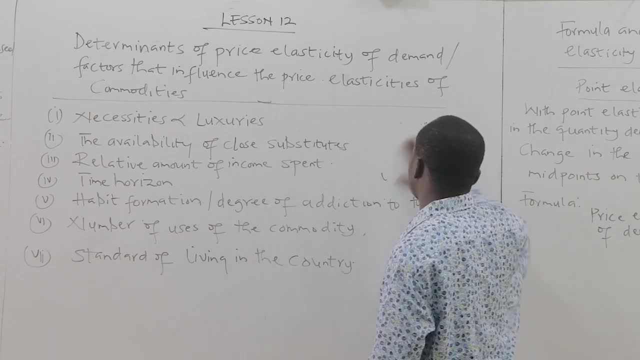 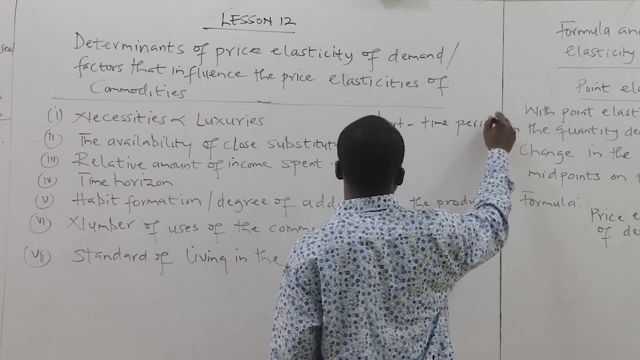 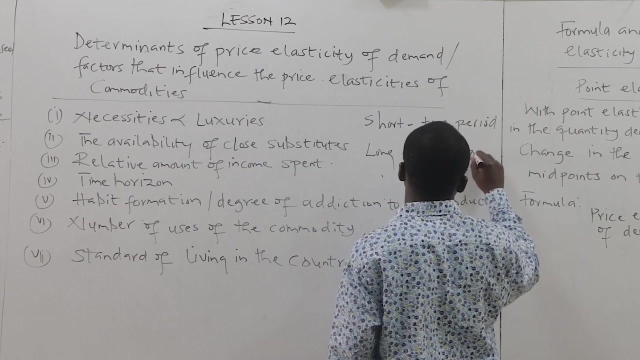 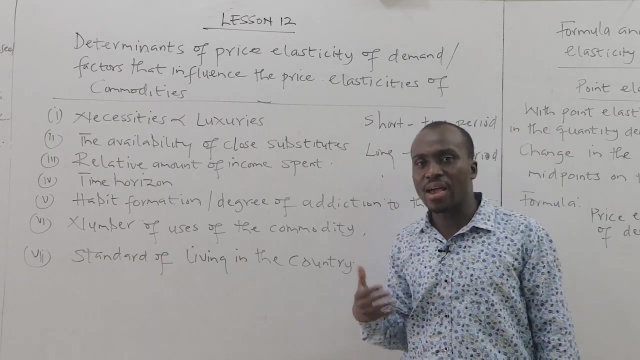 also very important. by the time period you're considering this short time period. let's a short time period. you have a long time period, so let's take this two time period: short time period, a long time period. probably you're buying a product, right? i'm buying a. 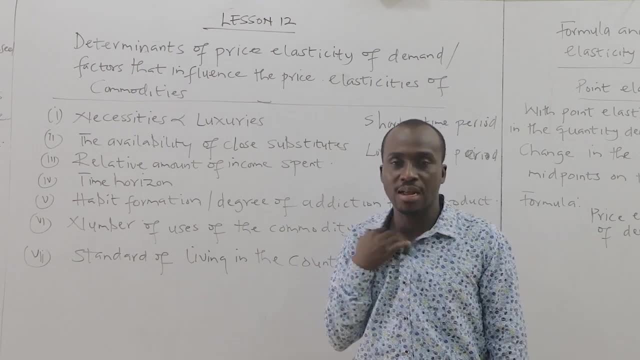 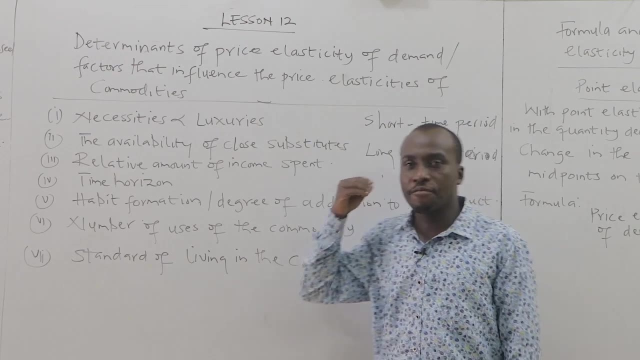 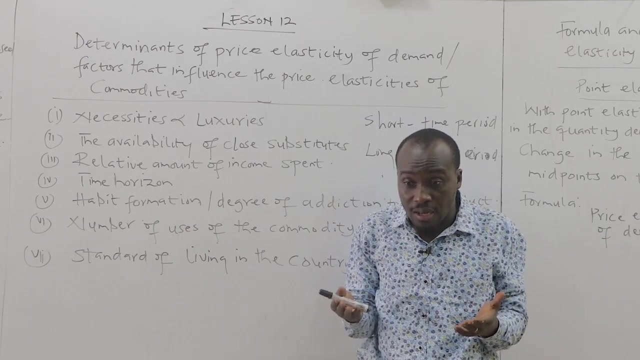 product, maybe here in ghana where cantonment right cantonment- is a suburb in ghana. the price have gone up in cantonment in a short run. in a short period, meaning the first two or three days or four days- i've not discovered any place i can get the same product to buy. so what do i do? i keep on buying. 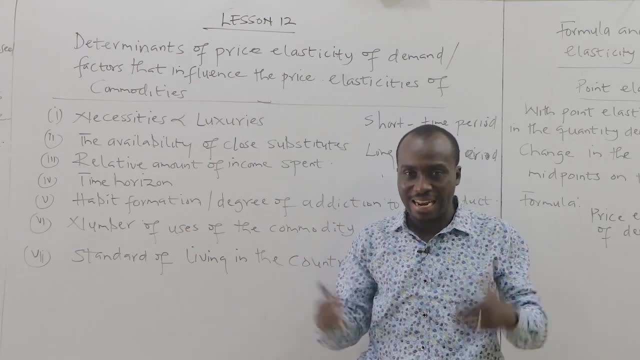 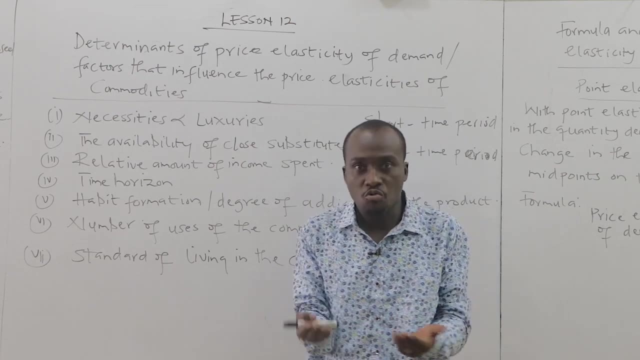 my demand becomes elastic. the price have gone up, but i've not discovered any other place in accra where i can get the same product to buy at a lower price, right? so what happens? what happens is that in a short run, within one or two weeks, i'll keep on buying the product because i don't 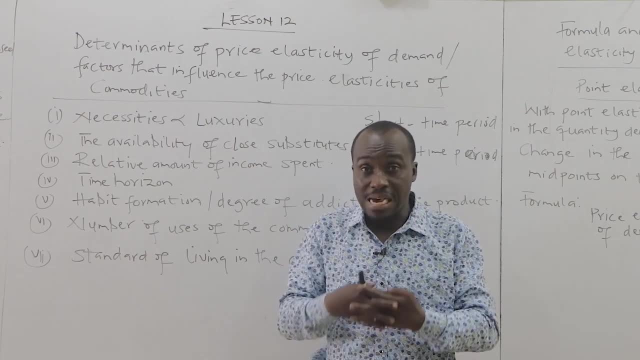 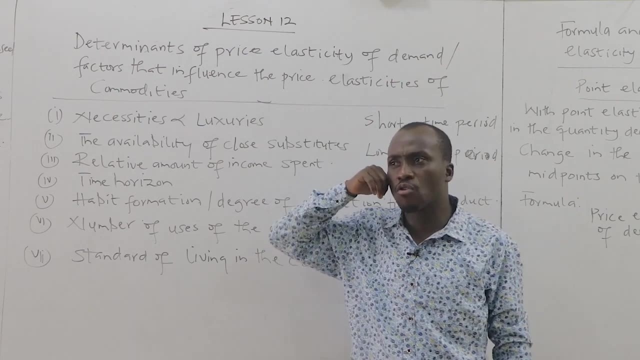 have any. i don't have any option. in that case, your demand becomes inelastic in a short period. in a long period- let's say maybe one year time or six months time- you get a friend, the frame course you are. you told me that you're buying a product at counterment. i've seen one of the 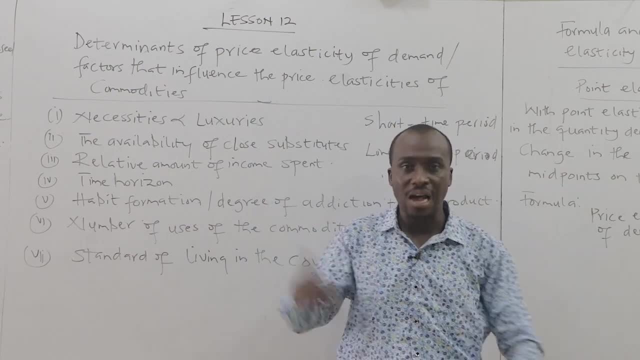 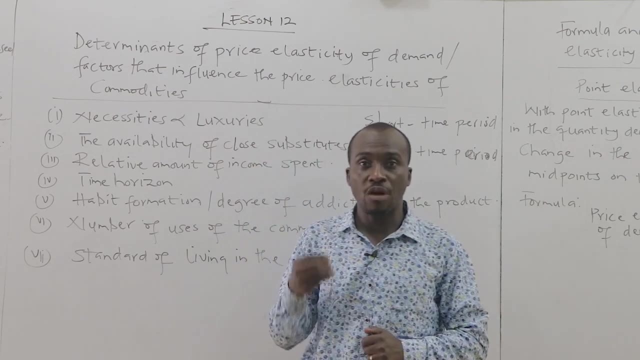 products as spin test. it's very cheap to stop buying from counterment and kind of buy from my area in the same quality. in the long run you will shift your demand from that product because you are able to discover that you can get the same product to produce at a lower price. 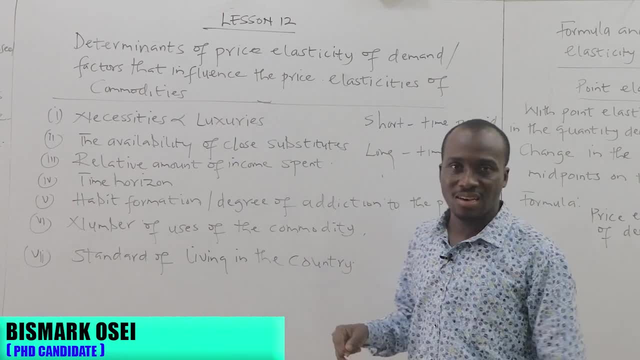 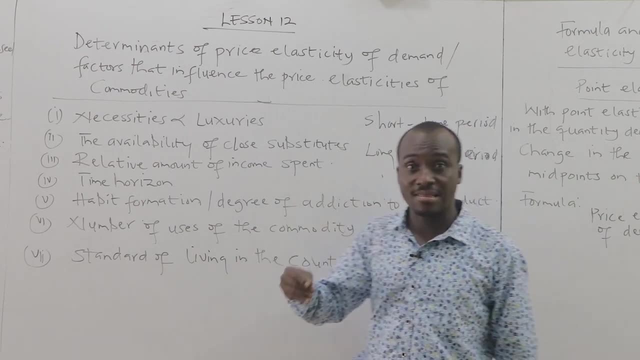 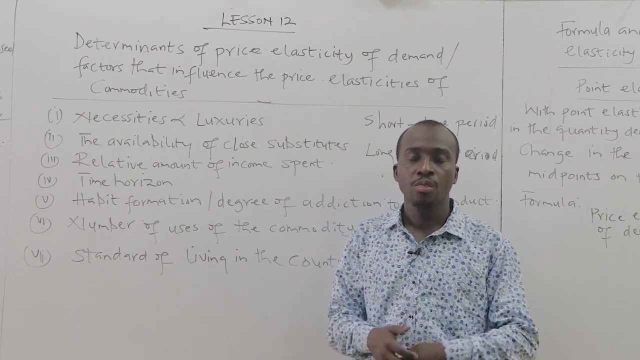 right. in that case your demand becomes elastic in a long run. people's demand for product becomes elastic in a short run. people's demand becomes inelastic because they are marginalized. they have a short period. they are able to discover that the other other places they can get the same product to buy a very cheap price back here in ghana. what the 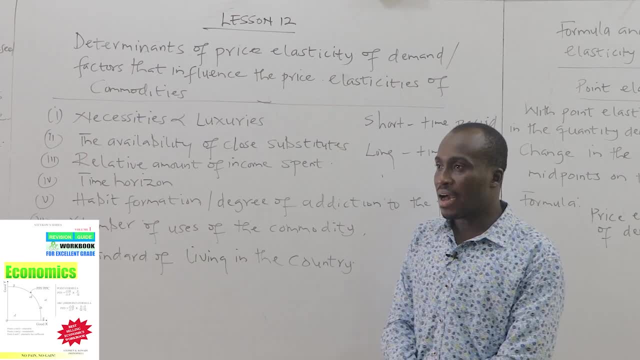 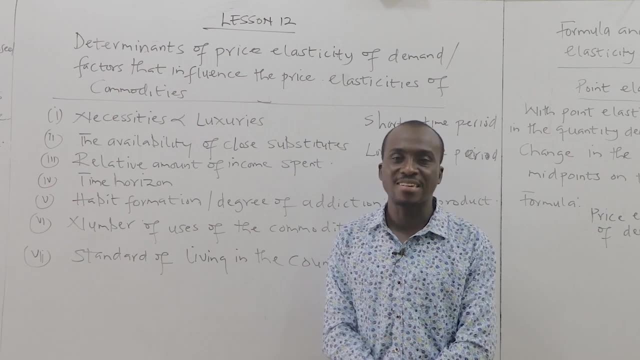 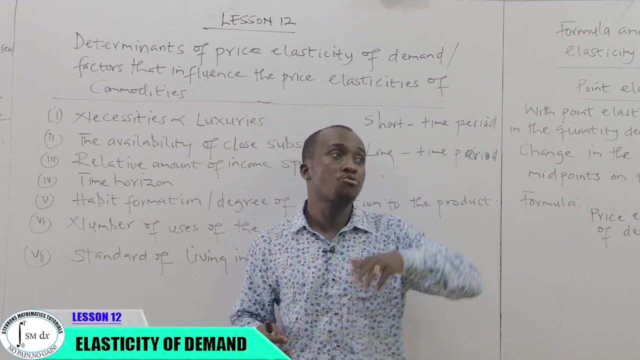 degree is that if you want to buy food, stops and, uh, only buy food- starts with a cry. it's very expensive. those who have cars, they drive to the villages and hinterlands. they get them very cheap. so in a long run i've discovered that i'll not buy food styles in accra. i will drive to. 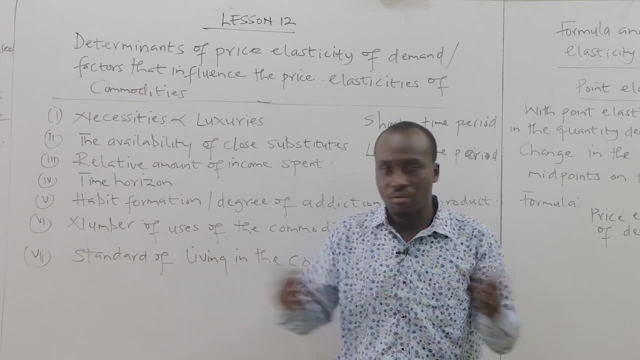 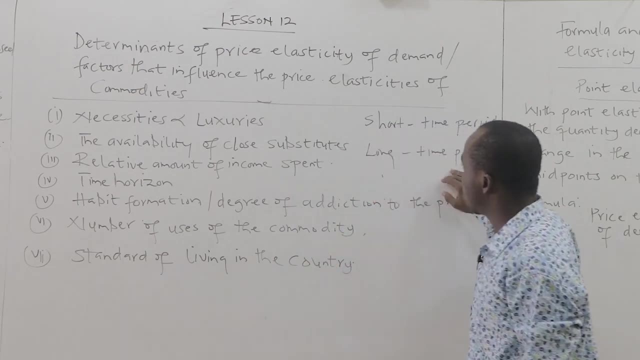 i'll drive to the ascot of accra, go to villages and towns and buy the product and bring it to a crime comments: have it for my family. that's one thing they can think of. so we have that issue of in a short run. demand tends to be an elastic and the reason because you're not able to discover. 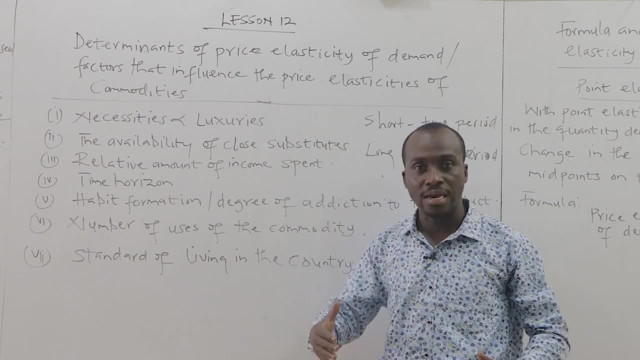 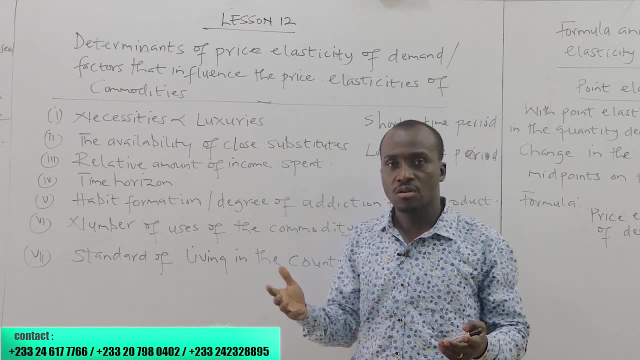 any other place can get the same thing to buy. so you are marginalized. you keep on buying in the long run. if you're able to discover that place, what do you do? you cut down your demand and you go and stick to the product you want. so these are the dynamics. 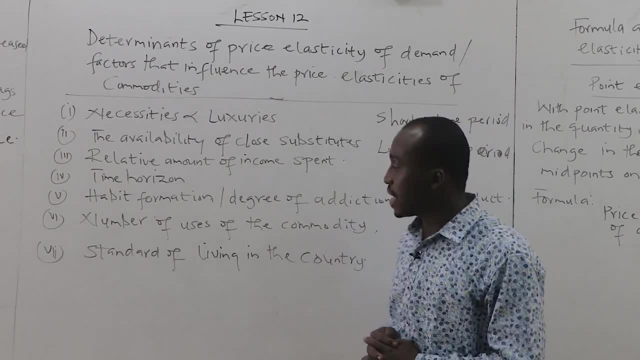 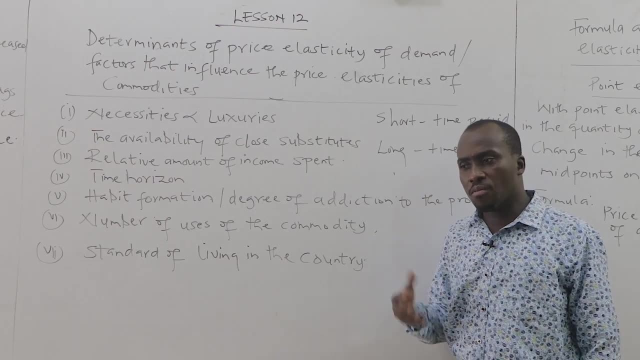 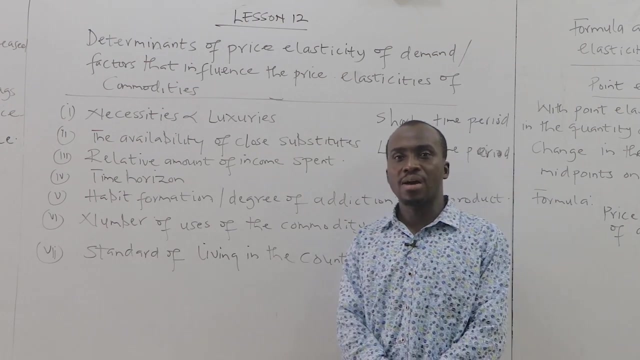 another factor that affects influence whether your demand is elastic and elastic. it's what they call habit formation, a degree of addiction to a product, when a consumer develops addiction for a product. for instance, there are people who have decided that me, i like bm cars. whether toyota or design is very cheap, i don't care, i always buy bm cars. 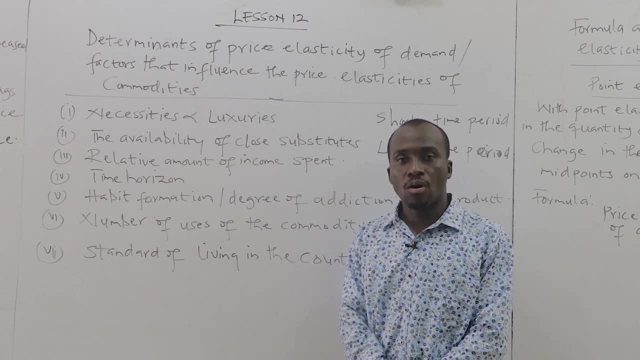 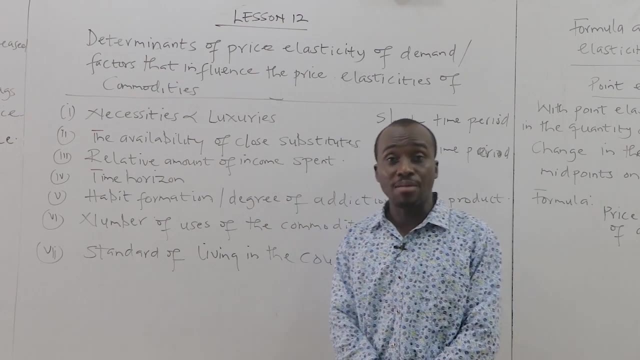 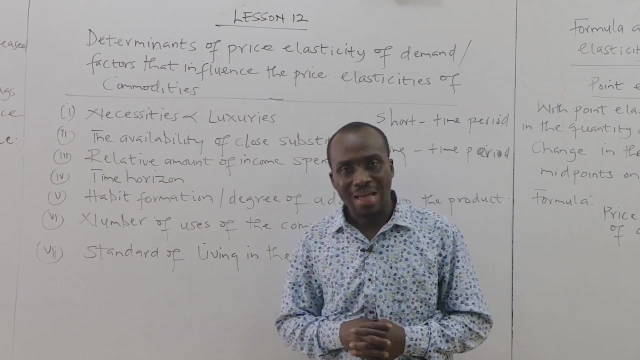 if such a person have developed addiction, doesn't care about whether the price of bm or mercedes have gone up. the person will still demand toyota, they still demand the bm cars. so such a person we are going to see how the market is going to develop, but it does not mean that every product 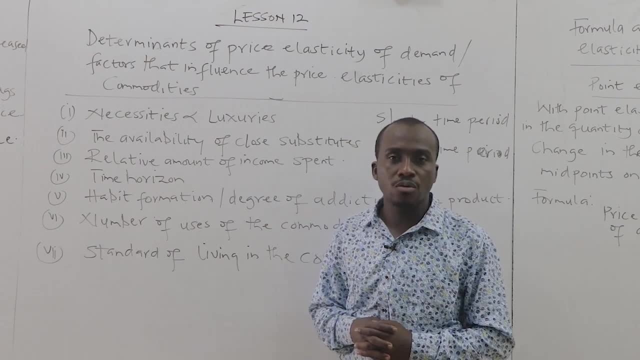 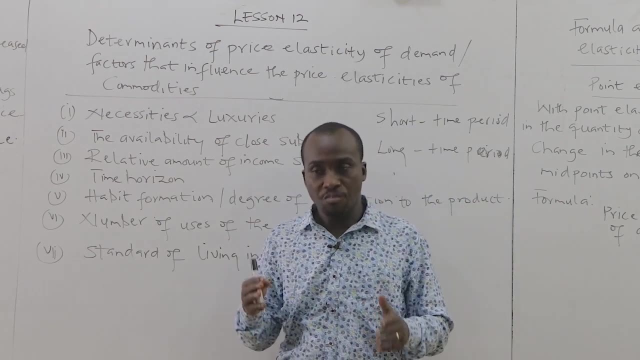 is inelastic. part of the long term is inelastic, so i will be put. the people develop addiction for a product. they don't care about how cheap the other product are. that's the product they like. maybe they have used it for a long period. people use a product for a long period of time. those 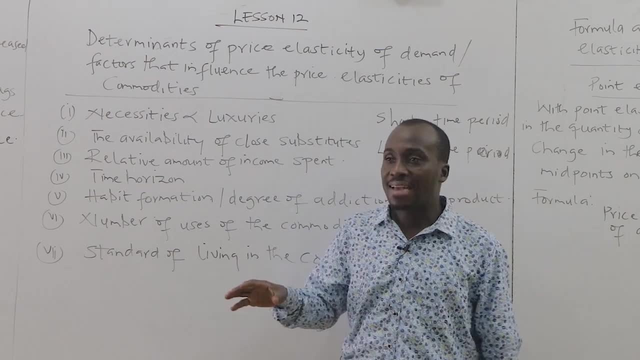 people like product that and they don't care whether the price have gone up. they still demand it. somebody said i want you. somebody else says you like iphone, he doesn't care. itel and other phones- techno phones are relatively cheaper, but that's the iphones you like. it doesn't care going to finn 4500.000. if you don't buy it, you will use it for your business. you will spend the money. 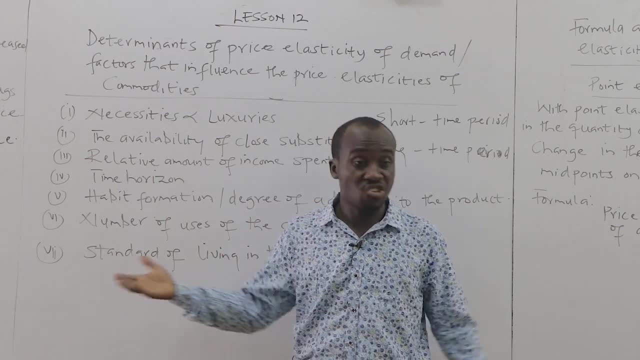 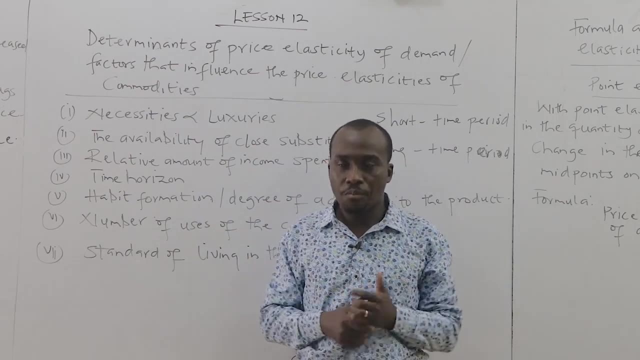 going to spend four thousand, five thousand to buy iphone, while other phones are cheap, right? so because you have used that phone for so many and you like how the phone performs, so the person developed an addiction and therefore his demand will always be inelastic for that product, unless 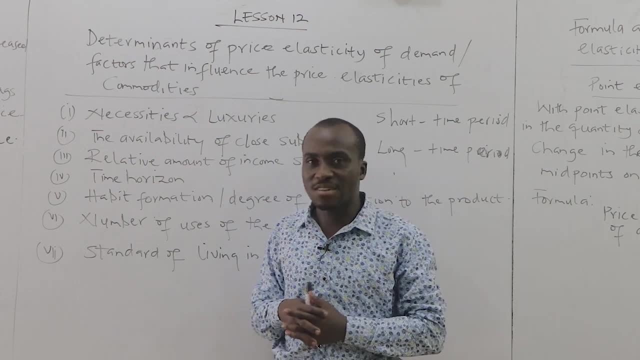 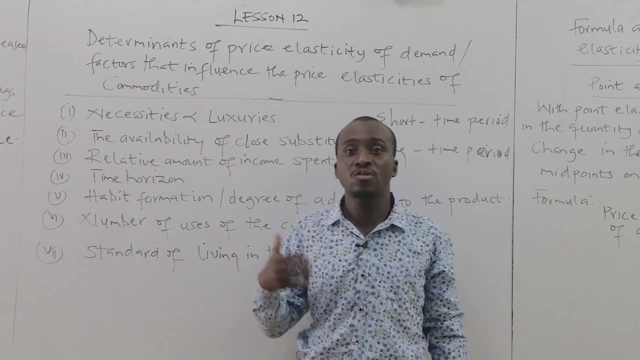 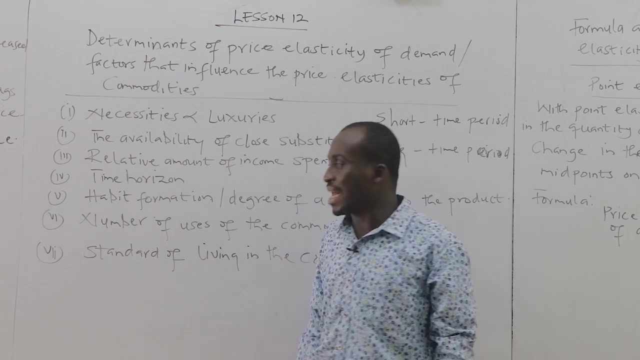 he changes his addiction. some people are being addicted to hard drugs and alcohol. it doesn't care. the increase in the price of this alcohol hard right, they will still keep on demanding that product. in that sense their demand is inelastic. but if you don't have any addiction for your product, 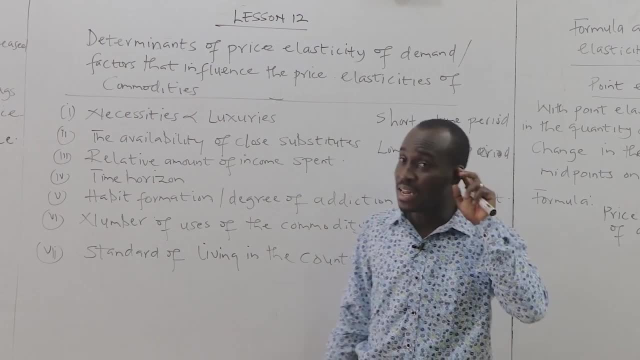 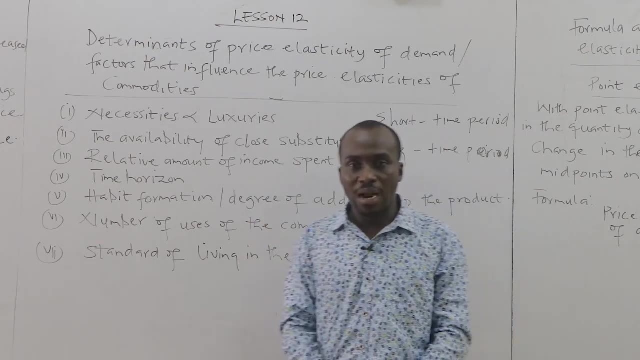 me. for instance, i don't have any addiction for cars, any addiction for phone, any phone. once the phone is good, it's average me, i like it. if i'm going to buy maybe itel phone when i went the itel phone is very expensive, i'll just go and stop buying, go and buy what is relatively cheaper. 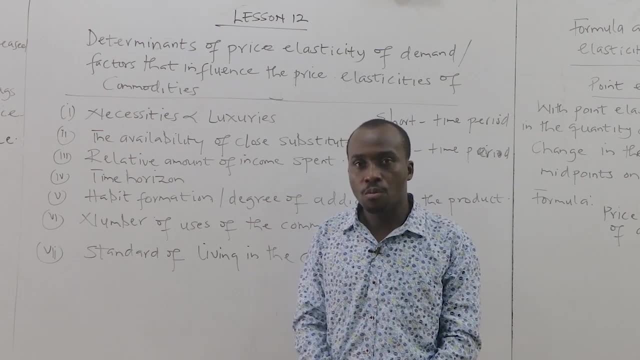 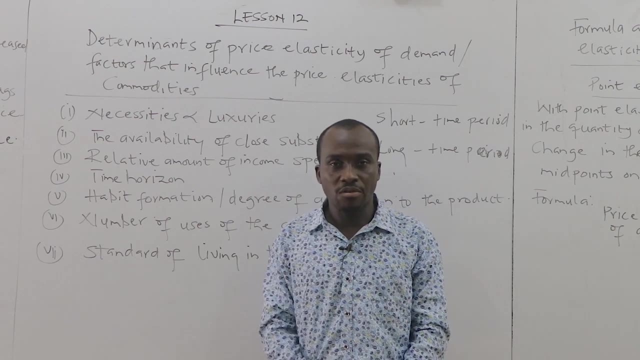 you can give me the same function, but i don't have any addiction for a product. so if you don't have any addiction for a product, the demand tends to be elastic- the slightest increase in the price of the product. you want to shift your demand because you don't. have addiction for that product. those who have addiction. when the price is even increased, they reduce their demand by a small margin. they keep on buying, but that's what they like. they don't care about whether other price are even cheap, whether they have substitute. some people behave. 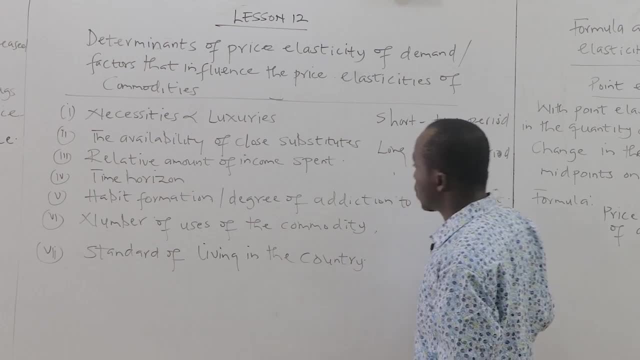 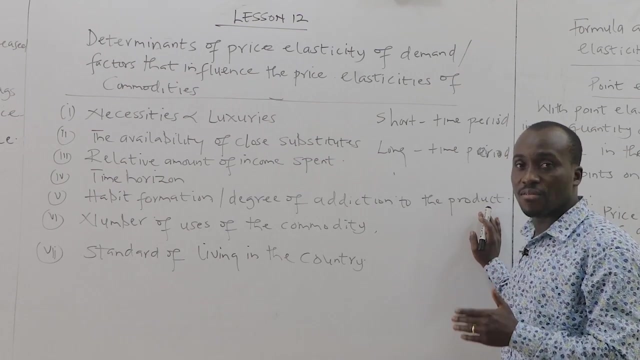 that way in that case. so what you want to see? that when people, when people develop addiction for a product, that's a happy formation- their demand for that product tends to be inelastic. but people doesn't have any addiction for a product. their demand tends to be elastic whenever the 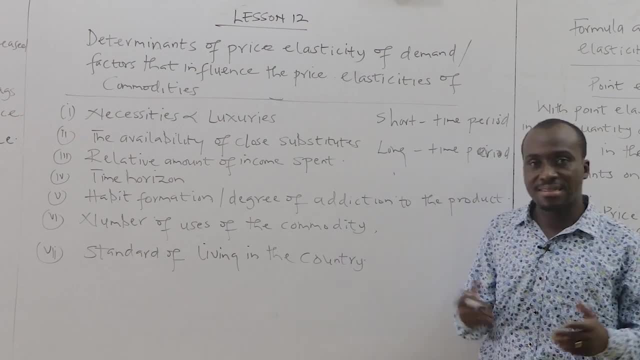 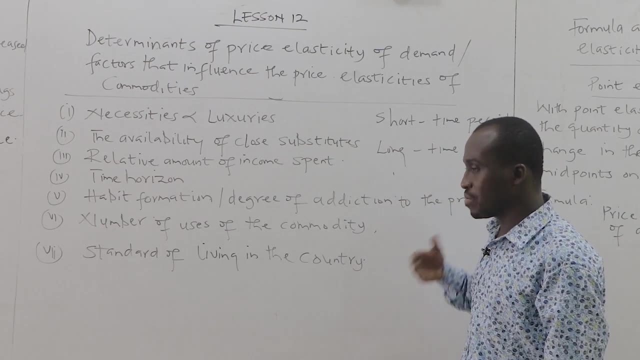 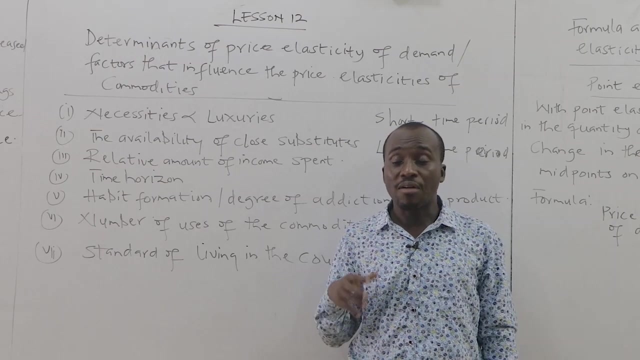 price goes up, they will shift from that product and go and buy any product they think their money can afford because they don't have any addiction. i mean the number of uses of the commodity. some commodities can be used for several purposes. somebody can have a matar, the matar commune, yeah. 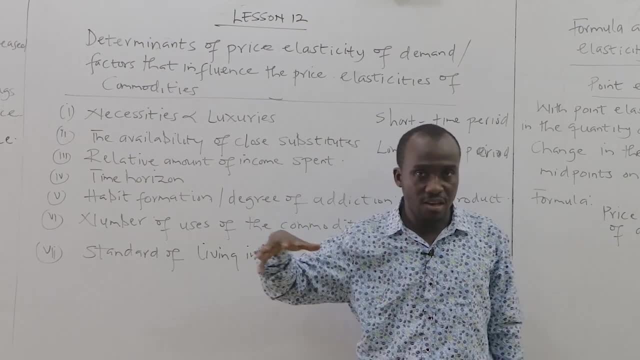 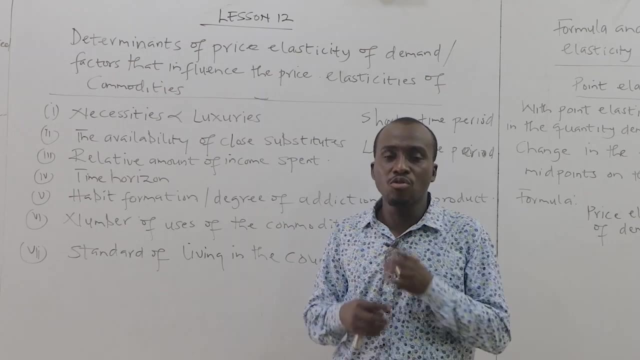 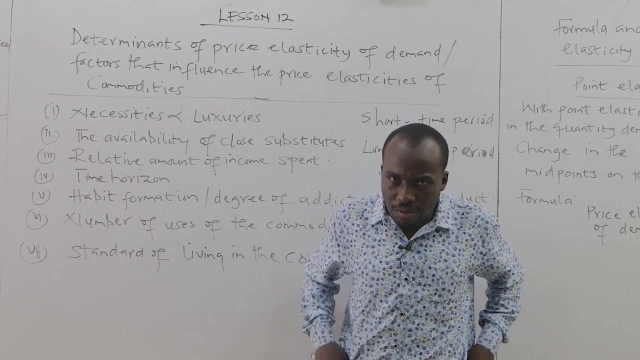 it can have maybe copper or lead or tin, you can use it for a lot of things. even if you have copper, maybe a half tin or bronze I can use for a lot of things. if a commodity can be used a lot of things, their demand tends to be inelastic, if the price even goes. 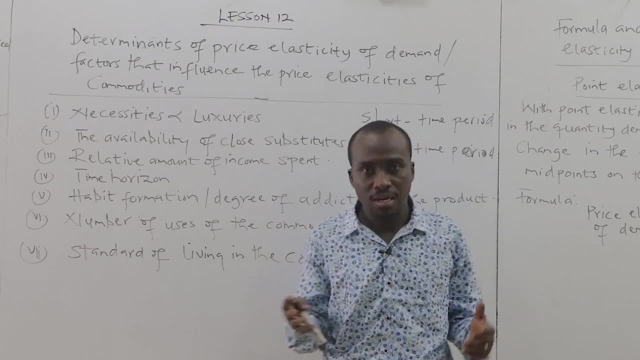 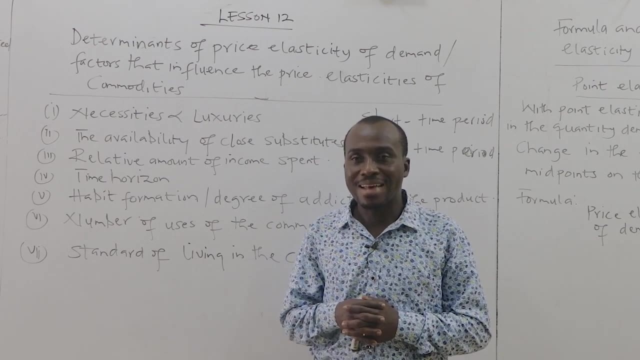 up. the person is not so bothered because once you get access to that product, the product can be used for a lot of things. the commodity they have is a composite demand- the commodity can be used for a lot of things- tends to be inelastic. the consumer is not so much worried about the price. all that he cares about is that he has to get. 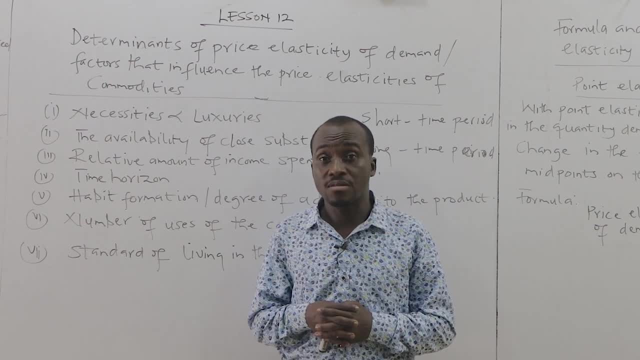 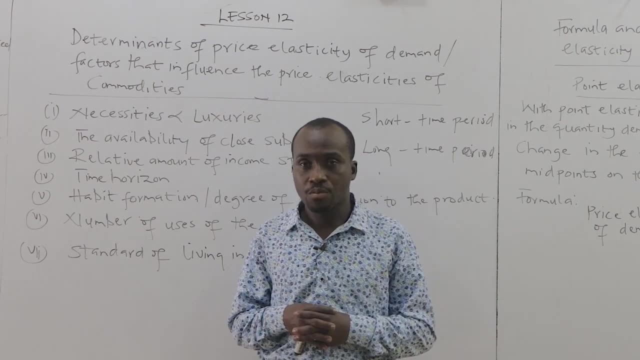 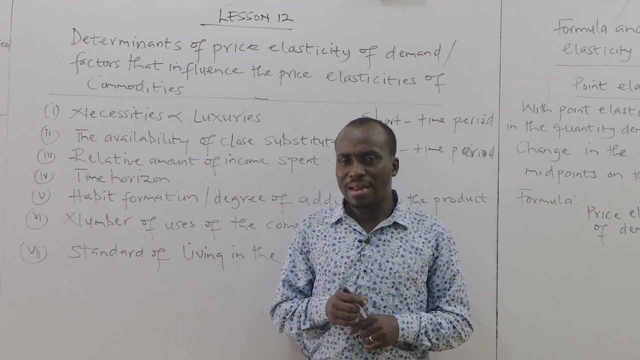 the product and wants to get the product. he can use the product to do a lot of things. so he answers why. products that have a lot of use, that have demand, tends to have inelastic demand common, don't have a multiple uses. for instance, what if you buy? if you buy food, what do you do? literally, I use the eat. 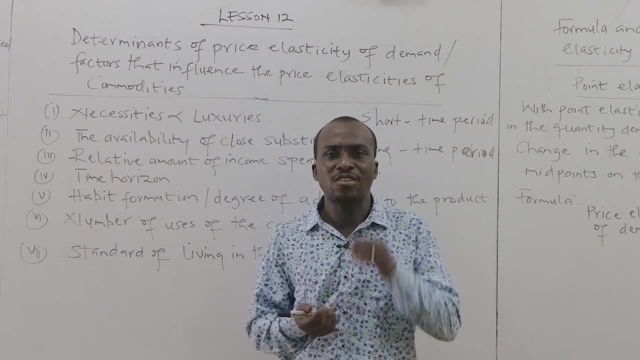 the food. you can use the food for any other thing. if you buy credits on your phone, what do you do? the put a phone talk the talk time. they pair their product to each other. you waste your time here in product. you зап 은неbra 토 ف we. 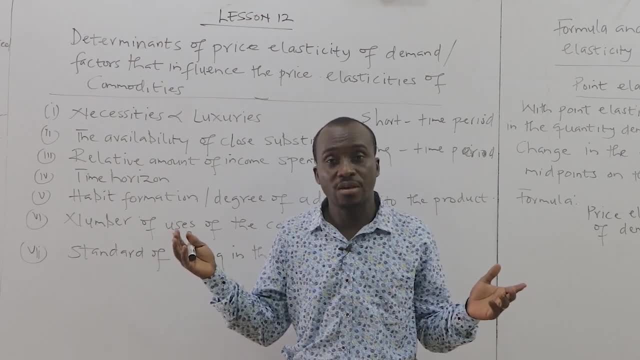 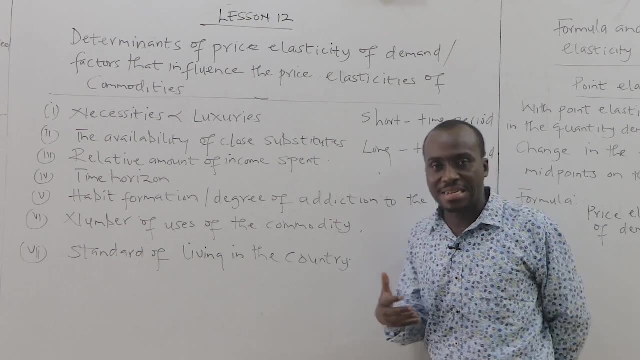 credit. in Ghana we call it credit. just put it on your phone, that's all. you can't use it for any other thing. so if the commodity doesn't have a multiple uses right, then in most case consumers demand for that product tends to be elastic anytime there is a change in price or increase. 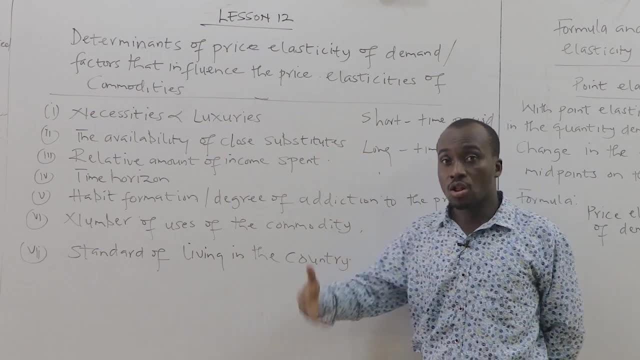 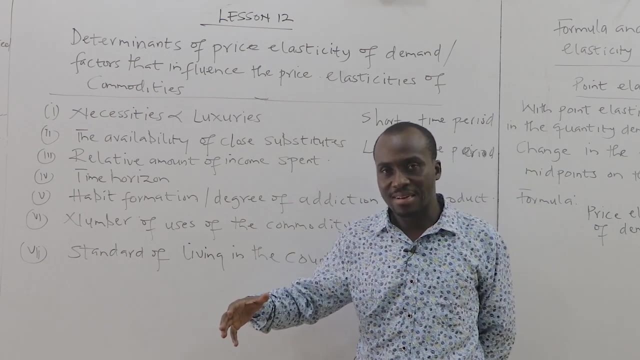 in price. they will shift. a lot of people stop buying because the company doesn't have a lot of multiple uses. you don't have that sort of materials used for that product so you might have a lot of uses. tends to have elastic demand. the community have a lot of uses that can be used. 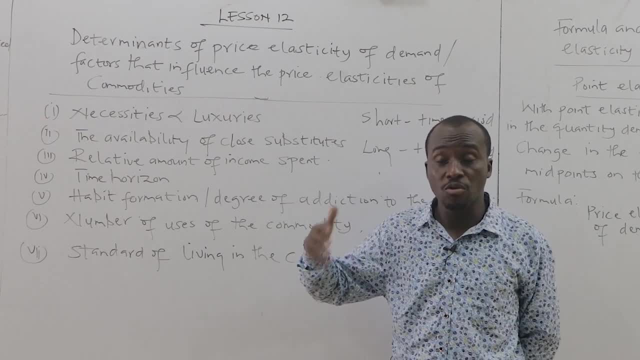 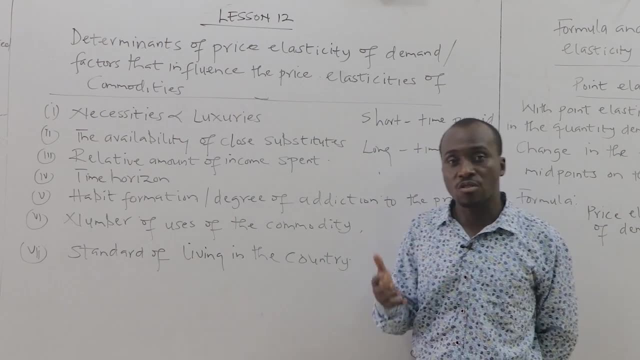 for a lot of common. they can be used for a lot of, for a lot of uses, can be used to a lot of items. tends to have inelastic demand, but the commander have a limited uses in it in it, when it comes to consumption, tends to have elastic demand. then the last one we want to talk about is the, the, 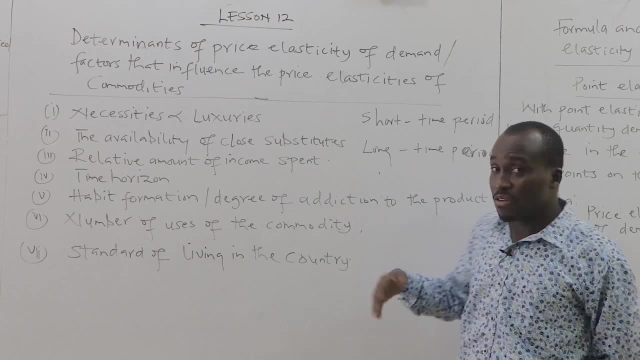 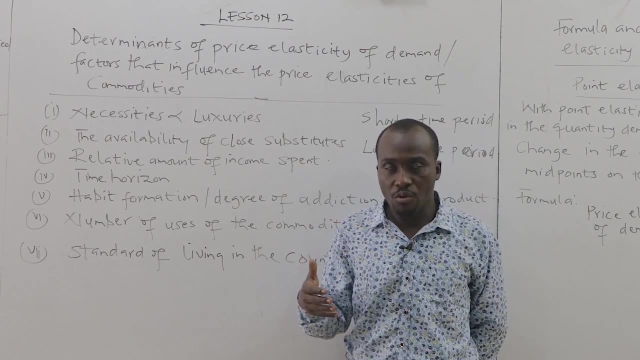 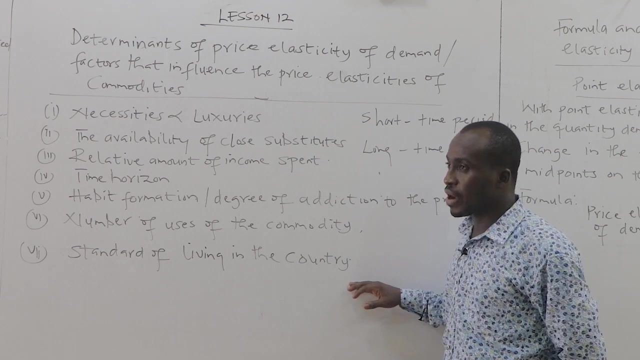 the standard of living in a country. the standard of living, what a standard of living measures? it measures the wealth of the people. so whenever people, people secure more jobs, we'll get. people are paid very well, they- they have a proof- standard of living. so whenever there is a standard of living increases, right people work. 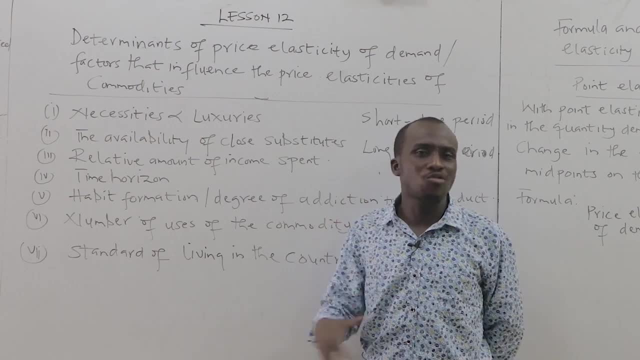 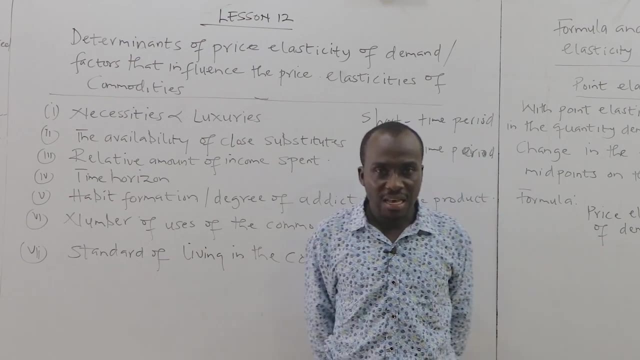 for improving. people have more money to buy a product and they are not so worried about the increase in price. there are enough jobs, they are paid weekly, they have money to spend. they want to go to a nightclub, they want to go to the picnic. they want to spend, so they are not bothered about. 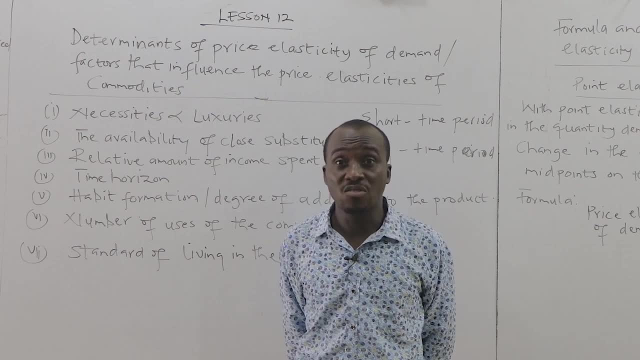 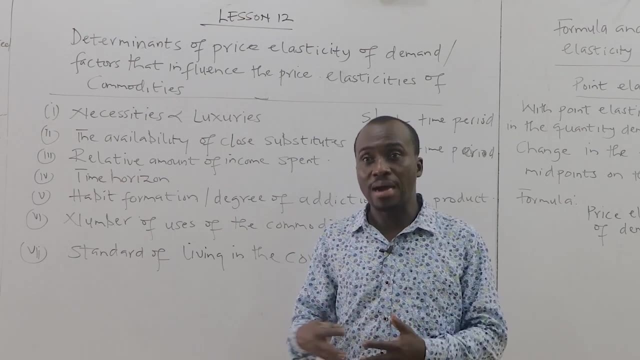 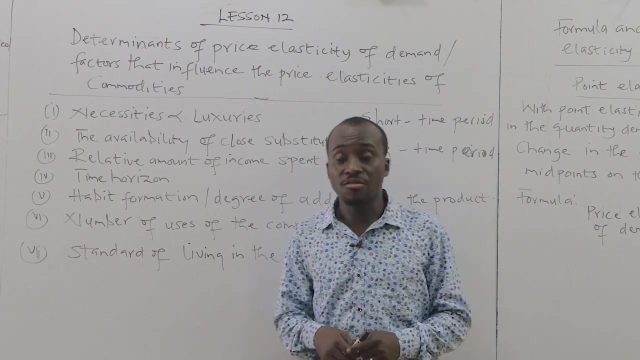 so much about the increasing price. all that they care about. they have money to spend. in that case, if they, the country, is experiencing this higher standard of living, most of the things people buy would tend to behave inelastic. but i don't believe it is low in ghana, in south sudan and, uh, central african. 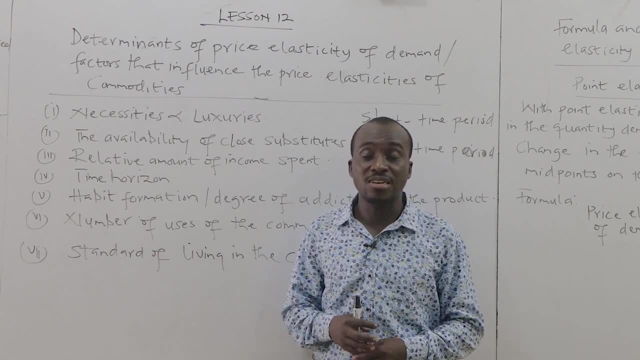 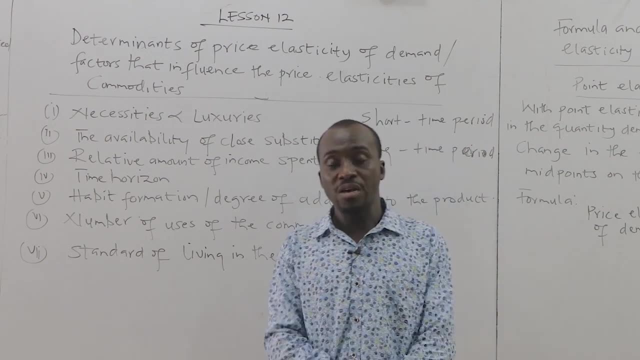 republic, in gambon, they're starting from living, probably in ghana. in Nigeria too, whenever price increase- because some of the contains very people doesn't have the money even to carry on, they would tend to behave the goods. they tend to be elastic. so what is it that? when the company 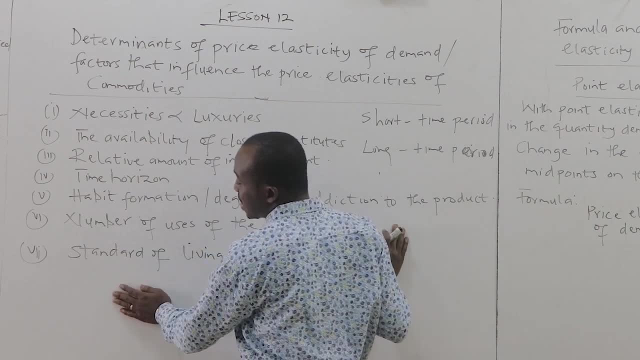 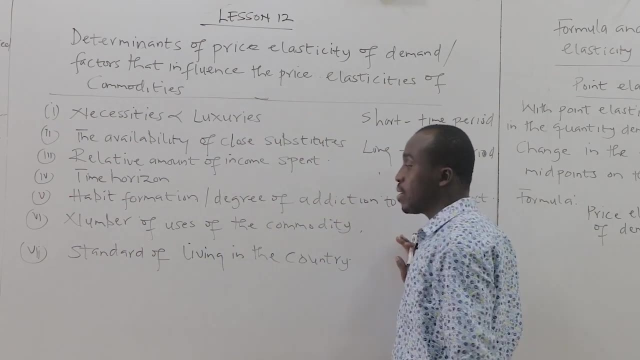 of instead of living. if the country is very high, the commodity tends to behave consume. the commodity tends to have elastic demand. it tends to have inelastic demand. when the country have a higher standard of living, the commodity tends to have inelastic demand. if the coin doesn't. 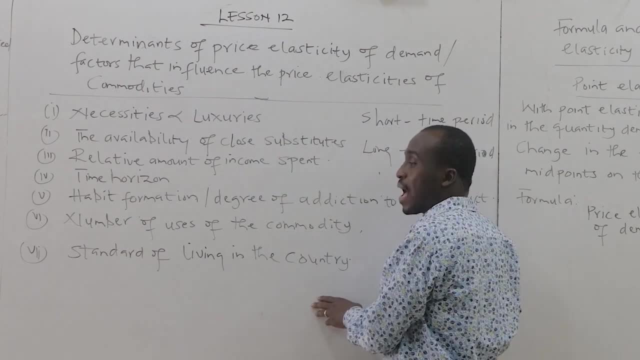 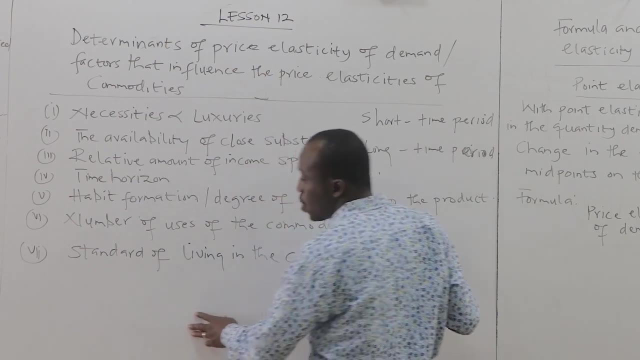 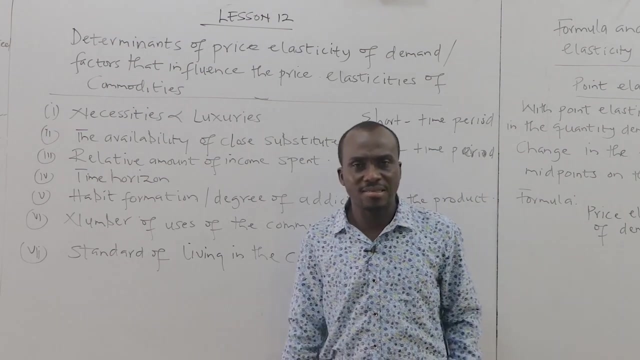 have any higher standard of living, the commodity tends to have elastic demand. so when the country is experiencing higher standard of living, commodities behave inelastic demand. when a country is experiencing low standard of living, commonly behave elastic demand. so these are some of the factors that make some of these goods. maybe you can also think about the durability. 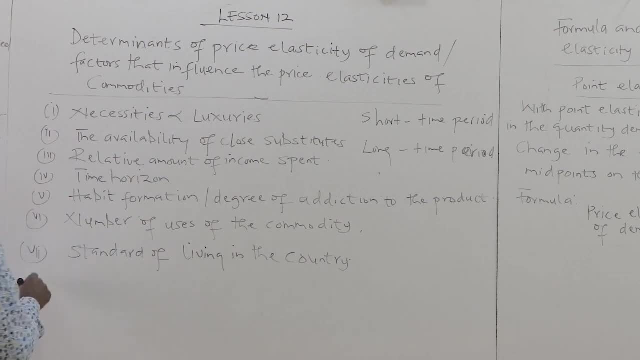 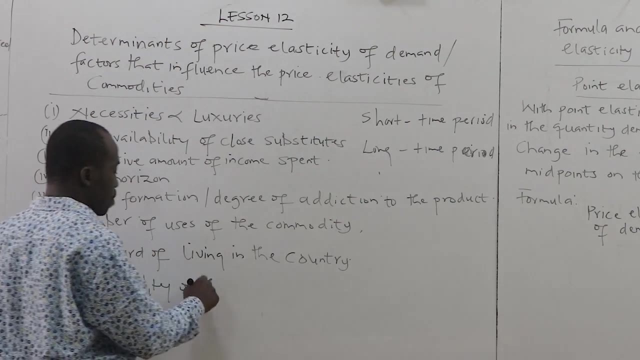 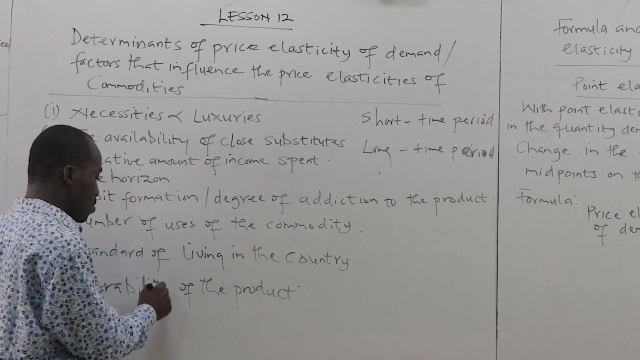 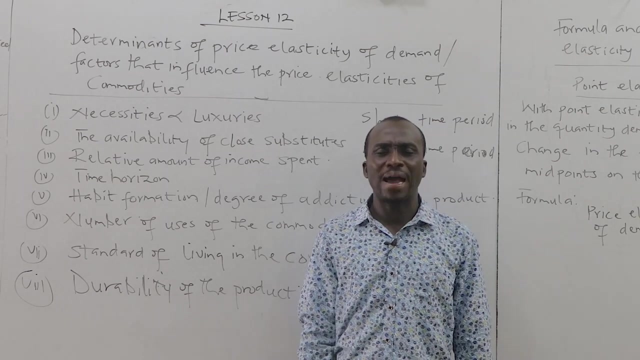 durability of the commodity. you can make it elastic or inelastic. the durability: a product, the product is durable. a product can last long. you can buy a product that means that, oh, if i buy toyota cars it lasts long, if i buy their engine, last long. in that case, 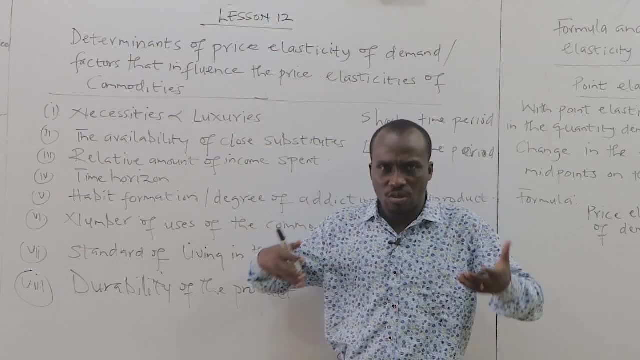 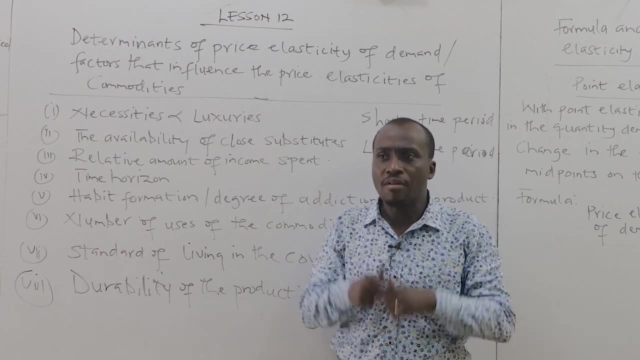 even the price even goes up, you buy it, but because you know that you are rest assured that when i buy that price will last long for me. if i buy, maybe binatom, iron- i bought a binatom and it lasted for about six years- if i buy it, if it's expensive, i buy it. i know it's going to last long for me. 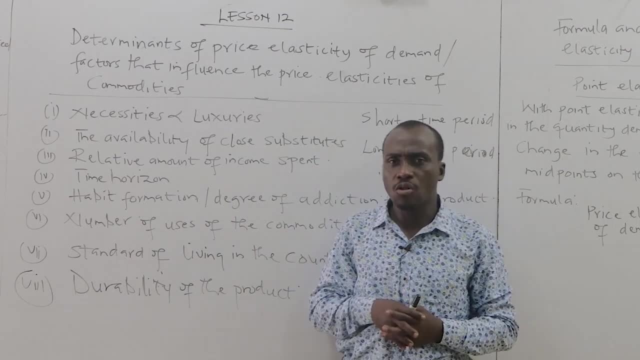 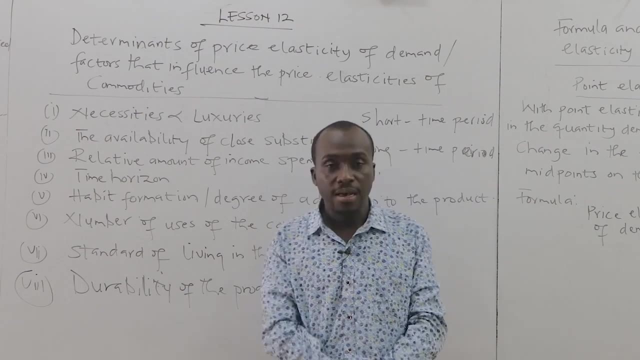 in that case your demand becomes inelastic. but commander does not last long. you have commodities, you buy it one or two days it doesn't function again. in that case, that commodity, your demand will be elastic. so these are some of the factors, factors that make some of the goods we buy, you and i, we buy on the market, on the mall. 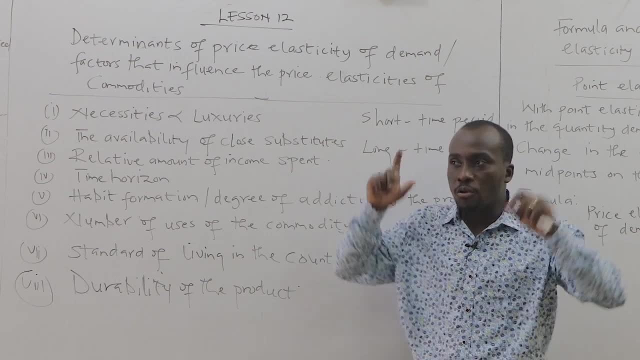 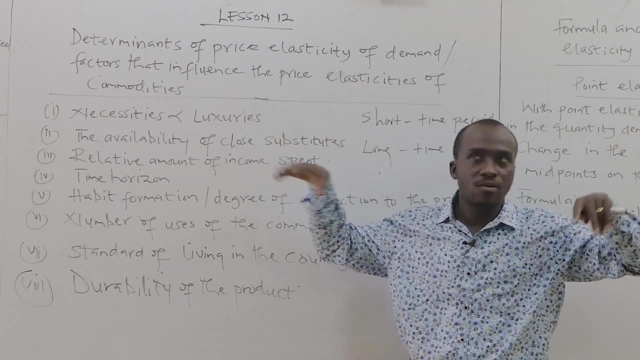 it makes them behave elastic or inelastic. so start wrap your mind around it. the things you buy every day now, every day when you go to the market, you buy things. check the things i buy. are they elastic or inelastic? my demand for: is it elastic when it lasts? what are factors that are actually? 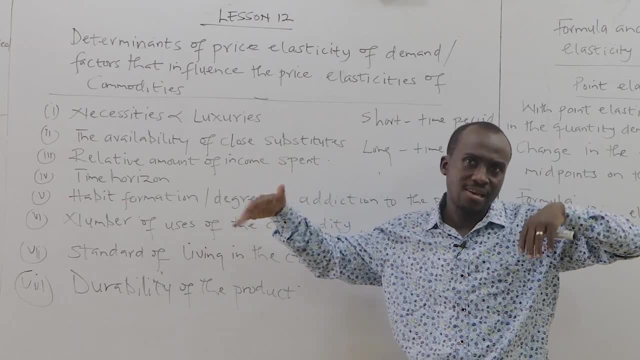 precipitating that role. what are some of the factors that is making my demand for the product elastic or inelastic? so start doing that. so this is not only for the classroom, it's for your everyday life, how you try it. if i'm going to be a good teacher, if i'm going to be a good teacher. 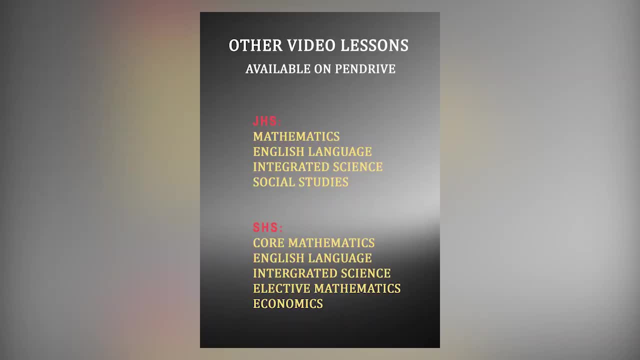 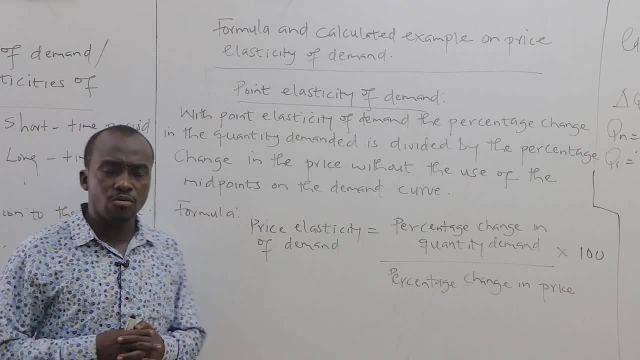 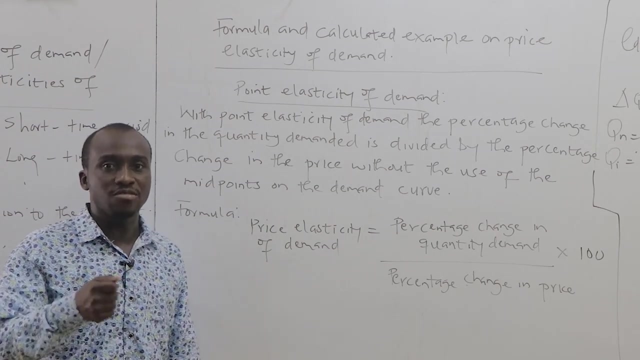 you have to take these concepts and intuition for your life, so you want to find out. you're going to learn how to calculate price velocity of demand. in most washi questions you are supposed to calculate the price velocity of demand. right, and we have two approaches in calculating price of demand. you're going to first. you have 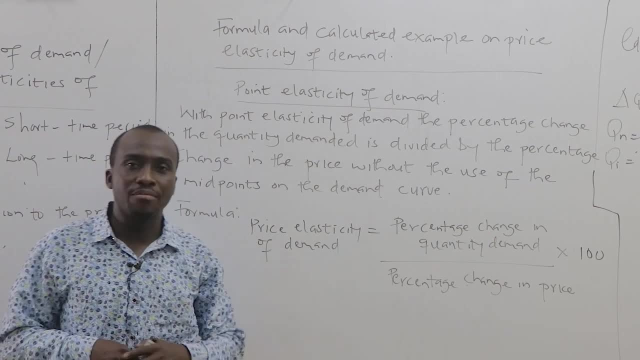 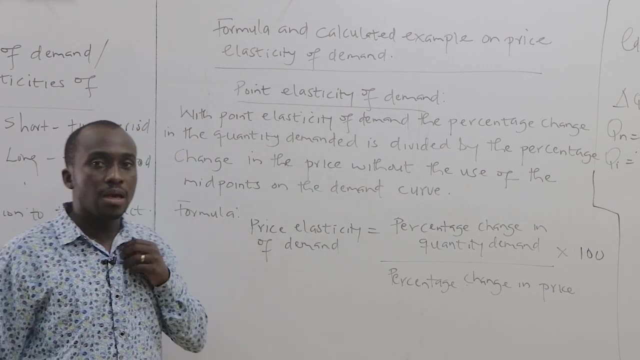 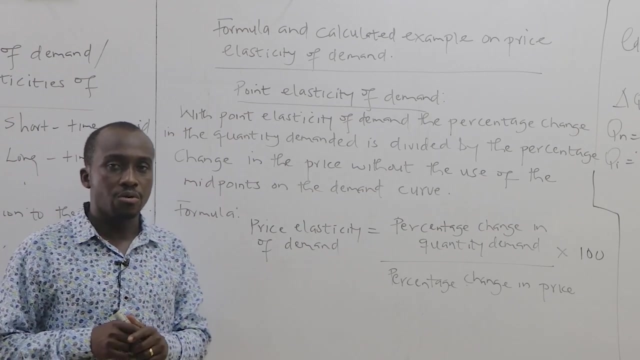 the points point elasticity of demand and we have the act velocity of demand. so what you're going to do right now, you're going to first take the point velocity of demand and understand it. after that we move to the act elastic demand and you understand how it's being used, right? so in most, 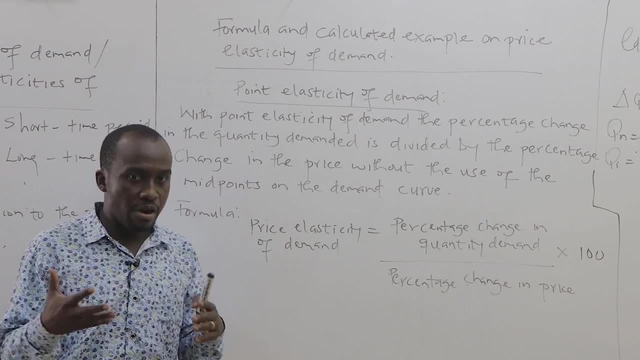 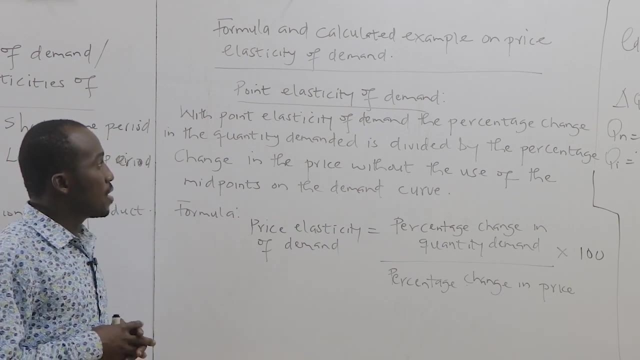 of these things. you're going to calculate in atoms, so you have to be very abreast of the calculation. let's see how the point last of the man, how it works out, the point elastic demand, the point approach, so it is like the point last of the manual points. 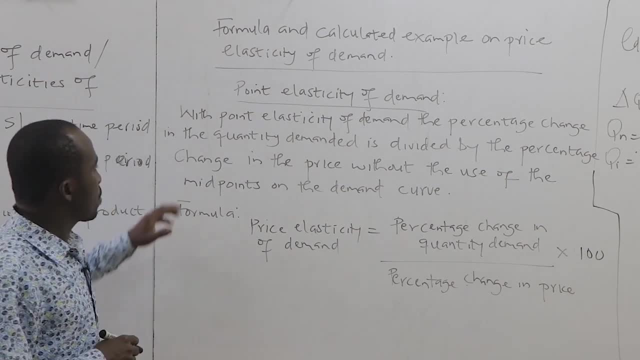 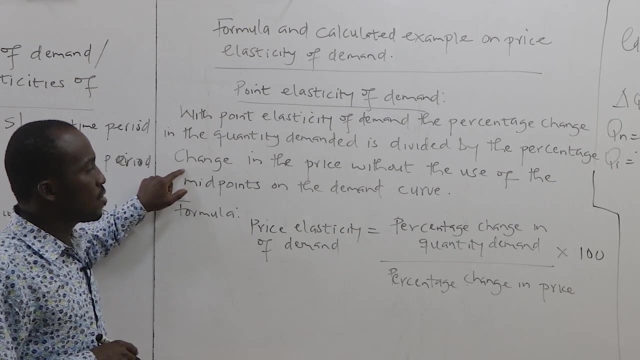 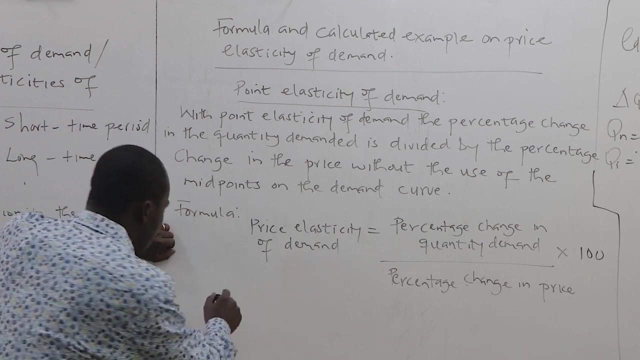 elasticity approach of calculating the price velocity of demand. with the point velocity of demand calculation, the present change quantity demanded is divided by the present change in price, without the use of midpoints on the demand cave. so let's take, let's look at this diagram. i hope you can see from here if price is here. here is quantity demanded. 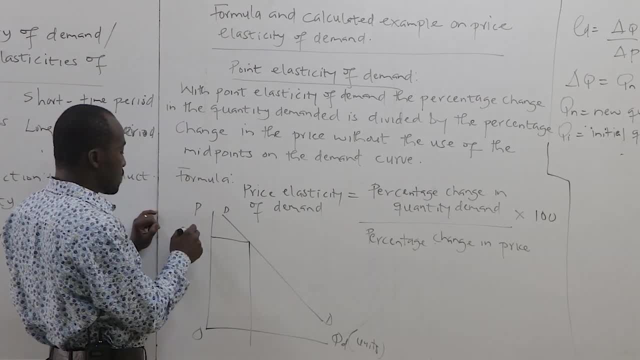 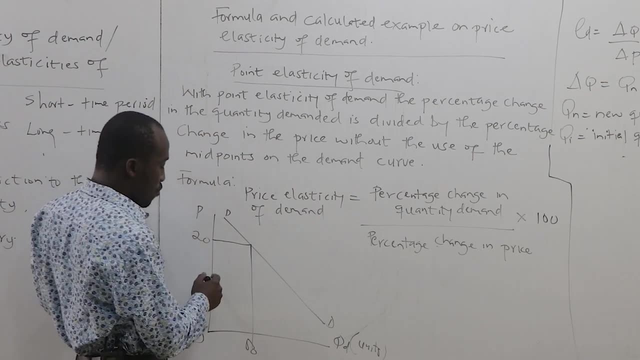 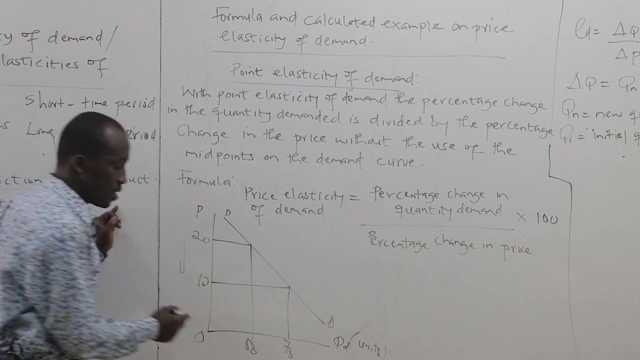 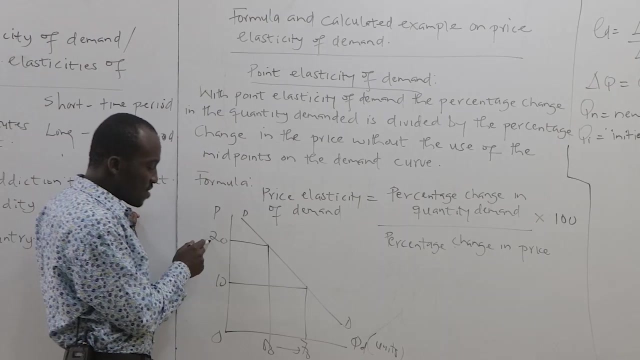 price was 20, demand was 50. right. when price reduced to 10, demand shoots to 70. so first price has reduced demand. as what increase? with point elasticity you're looking at how there was a change in price from here to here and changing demand from here to. 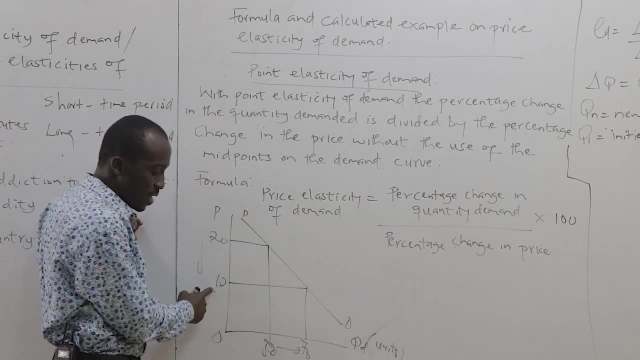 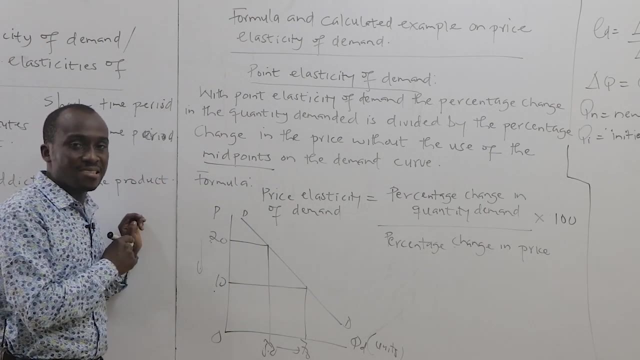 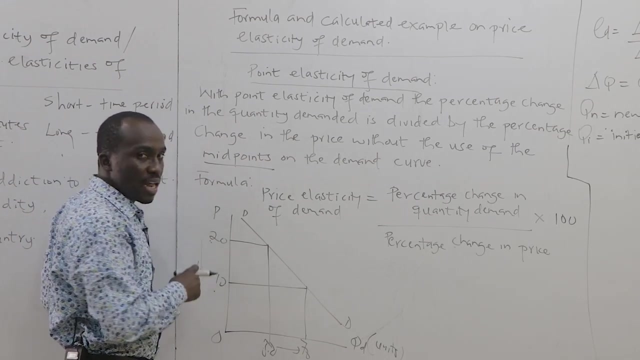 here. so you're interested in these points, this one and this one, this one and this one- you're not going to find the midpoint. my midpoint is that the midpoint approach is the arc, is the way you look at 20 and 30 and you find the average. so 20 and 30 put together give you 30 divided by 2. 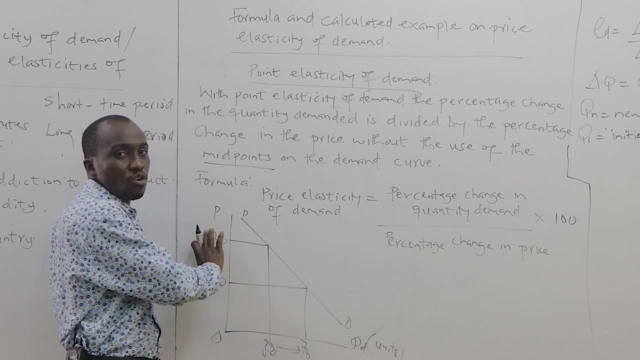 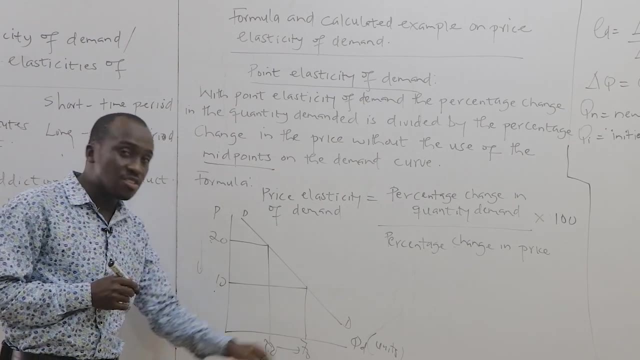 get 15.. you are trying to find the midpoint. what is the average of the change, right? what is the average between the two numbers from 20 to 30? and you find the average from 50 to 70. you find the average right, but with point elasticity we are not. we don't do that, we just look at the values. 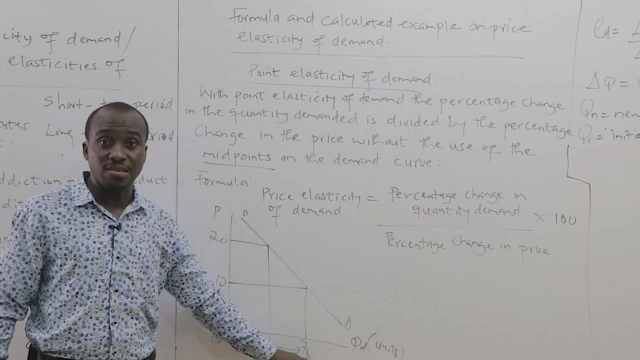 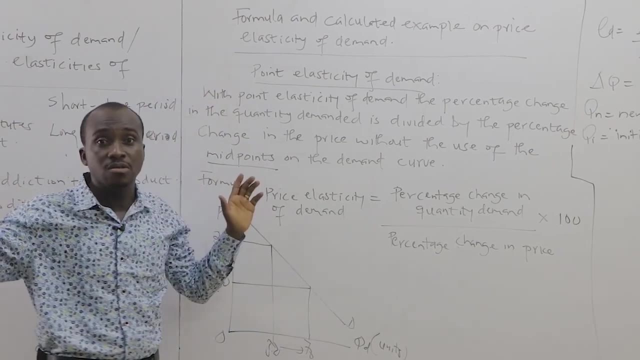 and find the differences, and that's the reason so we point elasticity. for instance, i look at this price and that price, this one, this one, and i find the differences and i use that for the estimation. i don't look at the true price and find the average, the two quantities, and find the average. 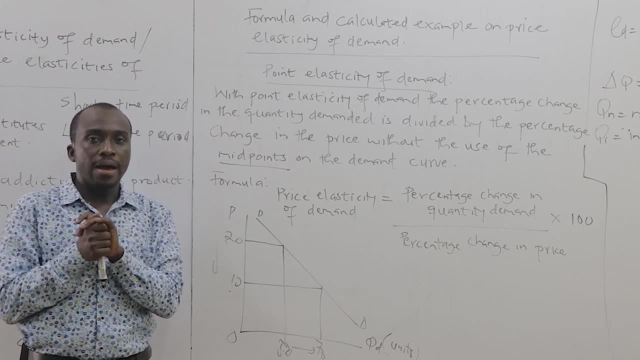 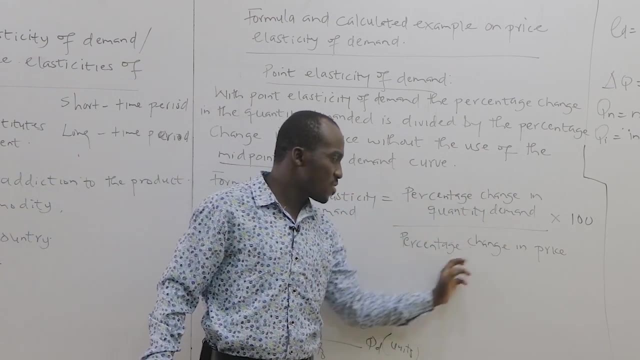 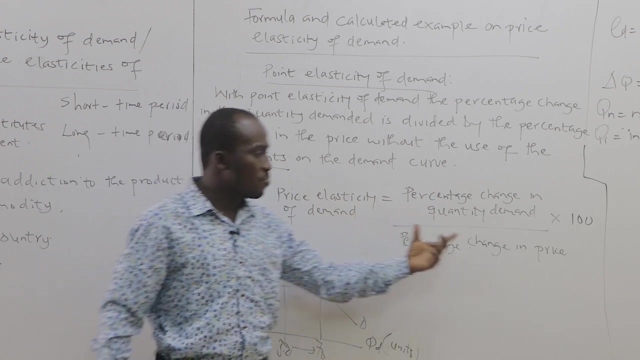 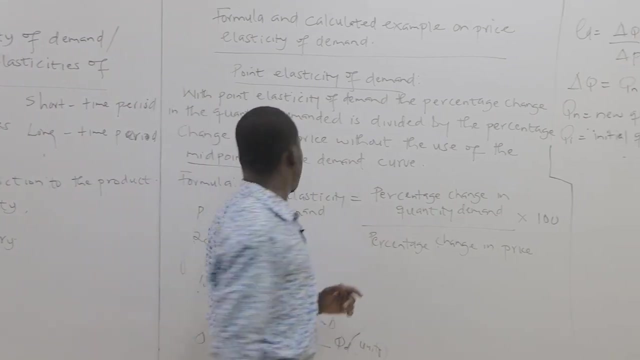 no, we don't do that. and so let's see: with price of the going to have percentage change in quantity demand divided by percentage change in price times 100. what happens? the percentage change in quantity demanded is equal to percent change in price times 100.. that's one of the formulas, or or you can say that the this: this is the symbol for price. 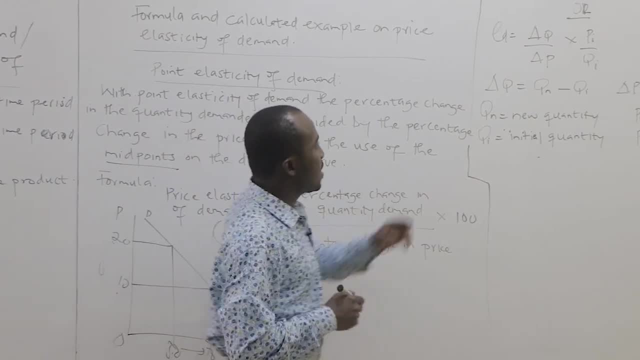 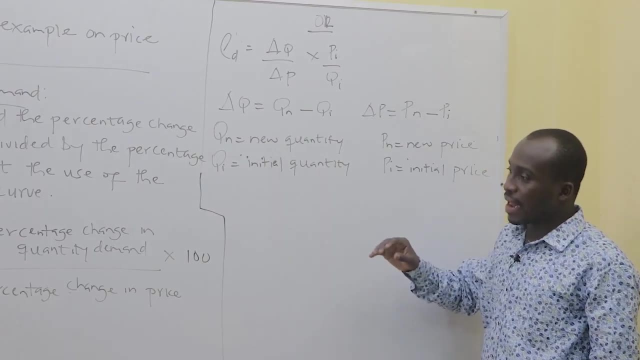 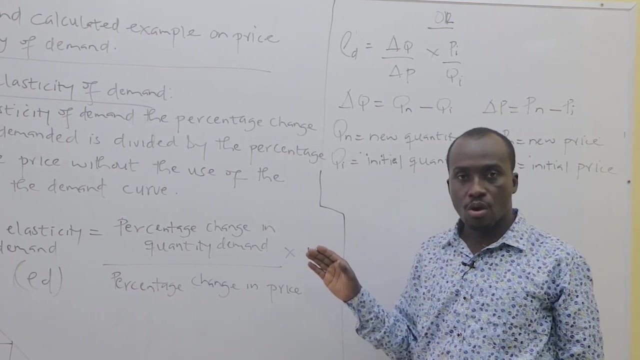 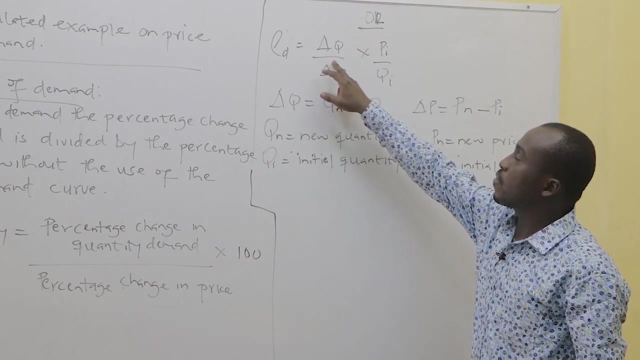 resistance of demand, or you can say that the price elasticity of demand here. so another- this is the first approach for the point elasticity: the percentage change: quantity demand divided by percent change in price times hundred. later i'm going to take data response question. you see, or you're going to say that you're going to. 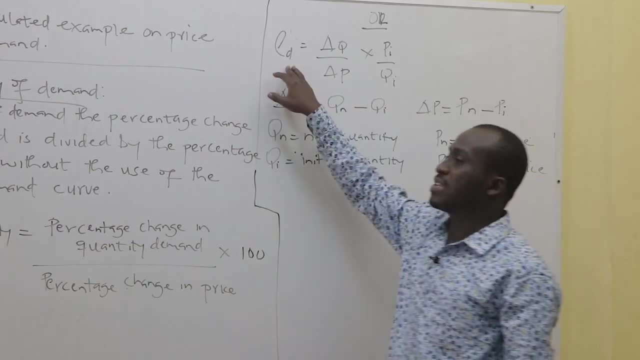 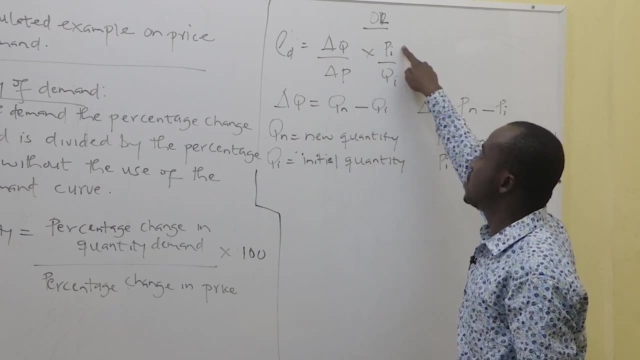 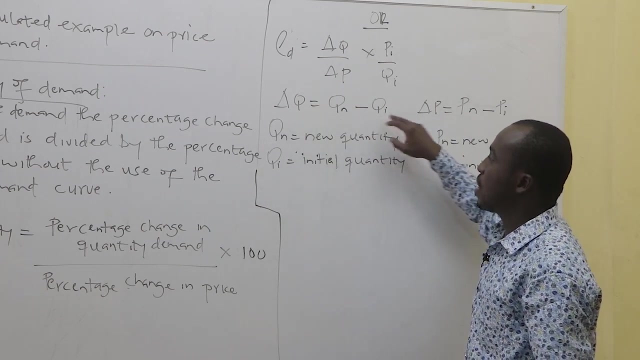 say that the change in quantity demand, the price analysis of demand, which is ed e subscript d, it's going to be change in quantity of a change in price times, the initial price time, initial quantity. what is the change in quantity demand? the change quantity demand is the new price. my initial initial is the change quantity demand is the new quantity minus initial. 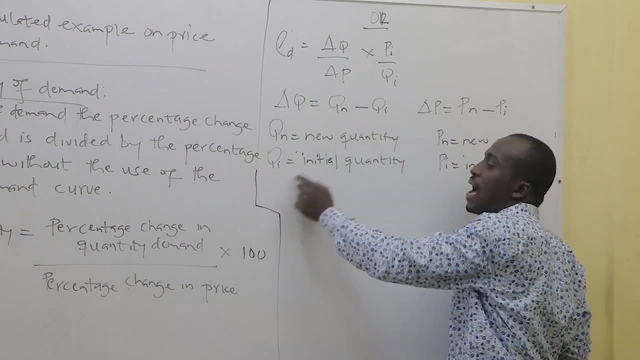 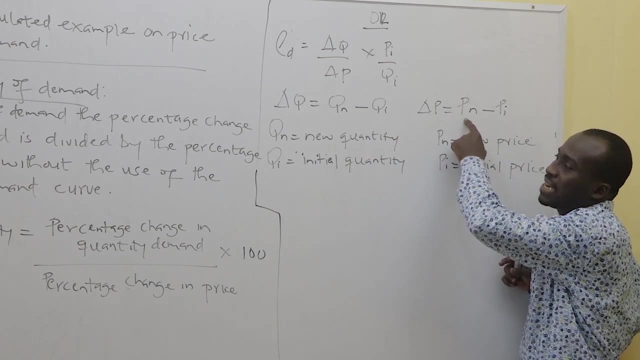 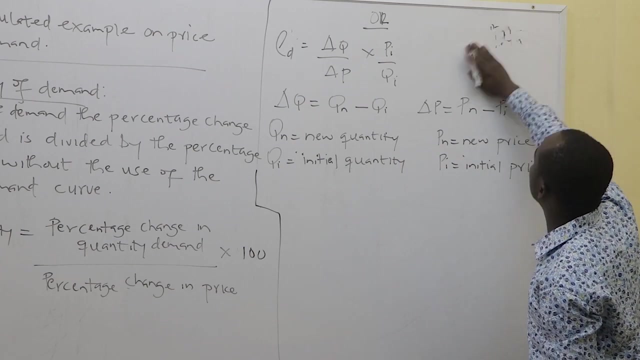 quantity. so q m is the new quantity and q i is the initial quantity. what is the change in price? the change in price is the new price. the p? n- they are subscripts. p n, p, i don't write it. p n- no, no, no, they are not, they are subscript. yeah, just a small little. 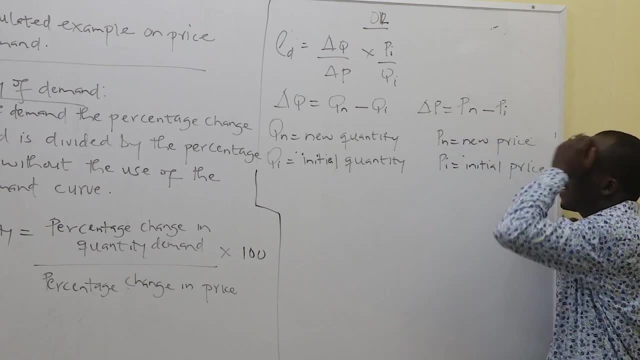 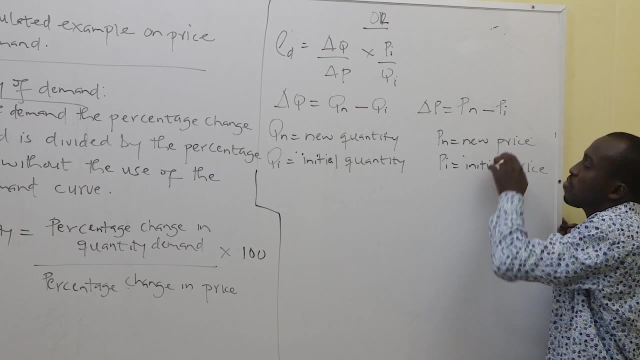 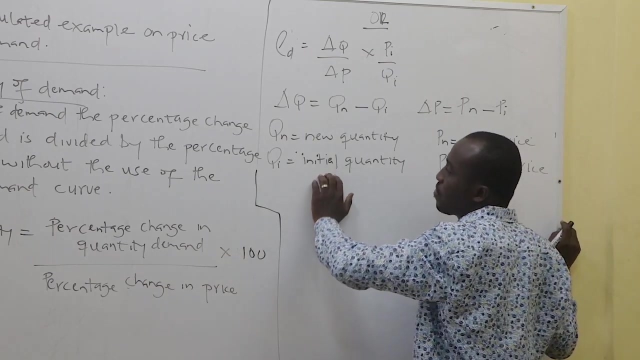 strange subscript: p n minus p i. what is p n, p n is the new price. what is p i is the initial price right. so if you subtract the initial price from initial initial price, from the new price, you're going to get a change in price. if you subtract the initial quantity from the new quantity, you're. 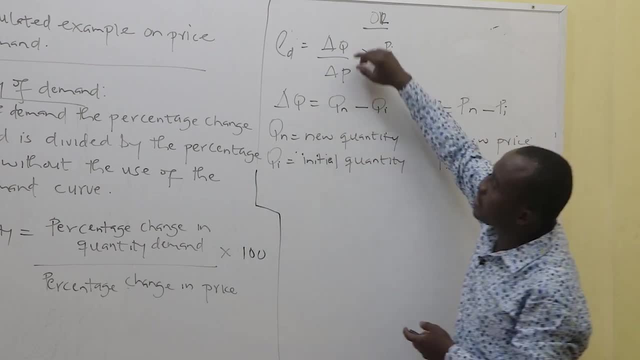 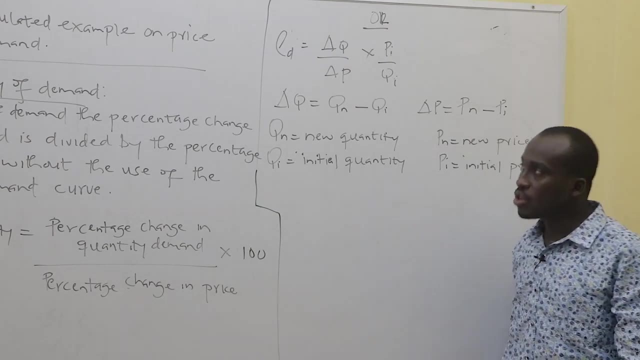 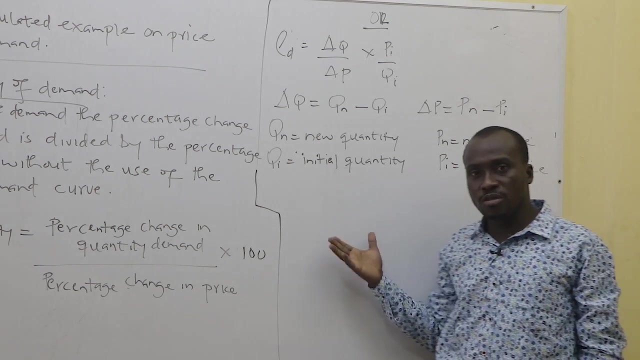 going to change changing quantity. so if i get a change in quantity by changing quantity times the initial price from the initial quantity demanded, you're going to get your point elasticity of demand right and most in most at times in wasi they ask you to use the point elasticity, the act. 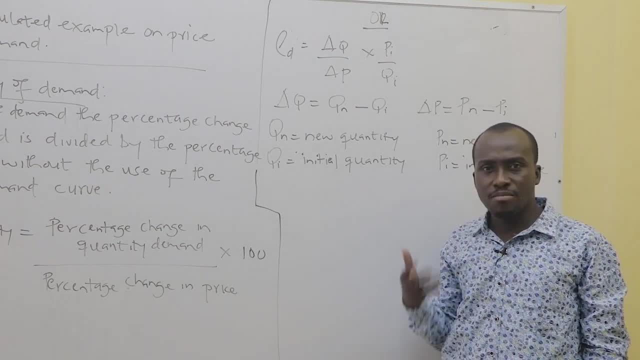 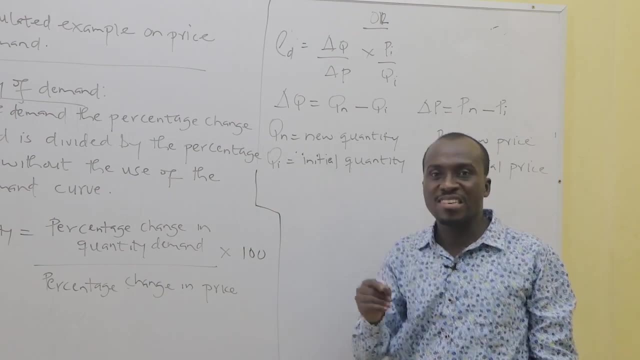 elasticity is hardly used in exams. the most of the time the demand that you use the point they tell you calculate price of demand. and most of the time they ask you to, when they say, calculate the price of demand if they didn't expect, specify that, use the accuracy. you have to use the normal, the point, elasticity, if they tell you let. 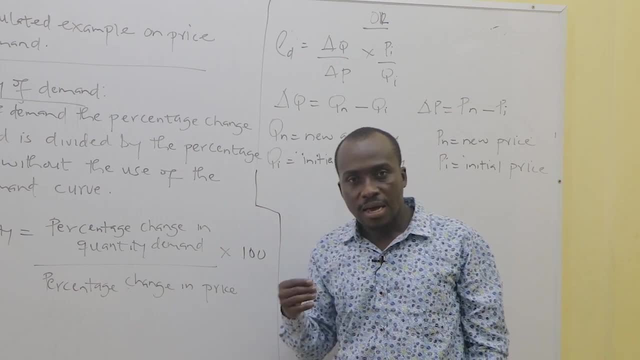 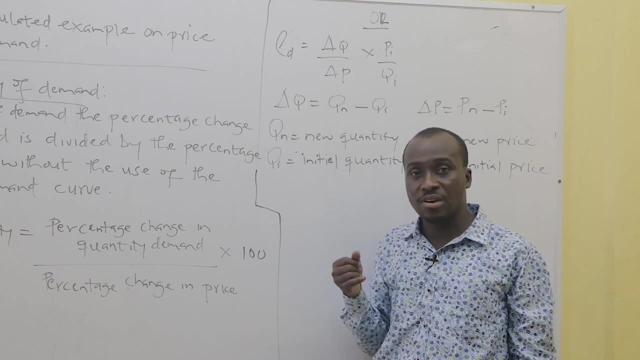 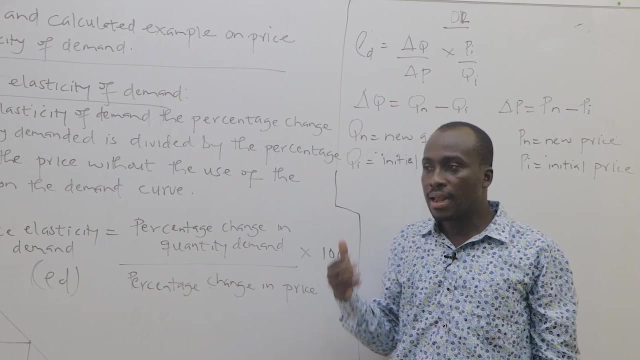 me restrict myself again. if they say that calculate the price, that's the demand if they're giving you a question. if the question didn't specify that you should use the accuracy for estimation, then use this approach, unless it's specified, and tell you that use the accuracy. later you're going to. 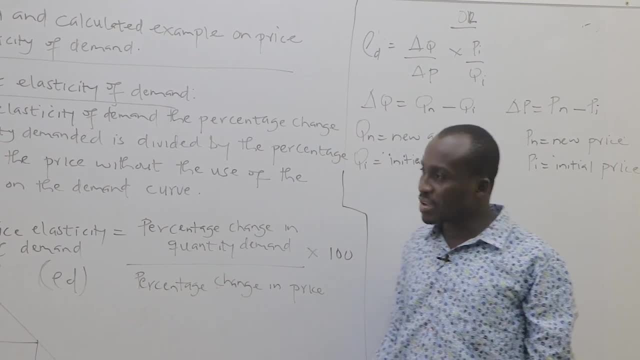 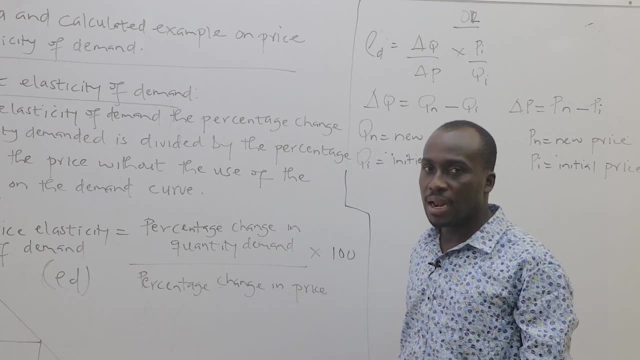 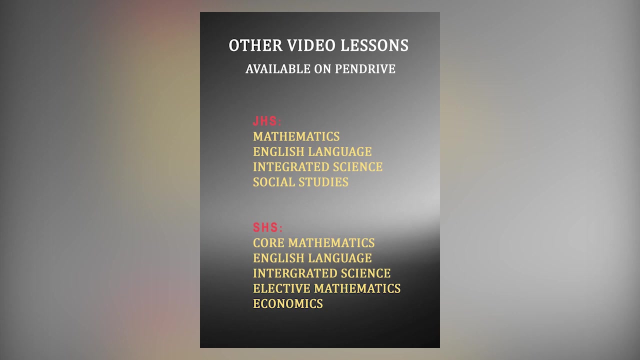 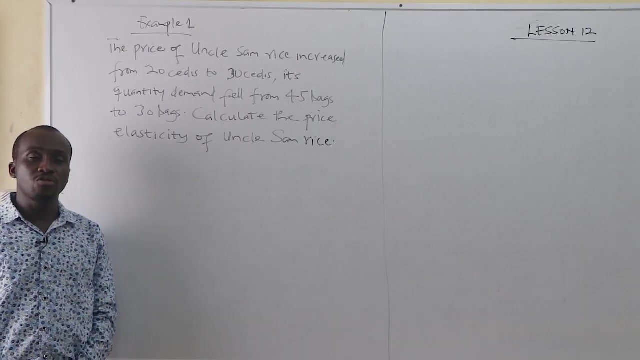 solve a question with the agla system. you see how it works out. there's a question here we want to solve to explain the price of demand estimation using the point elasticity. let's take that question so that we understand things better. so let's see, we have an example here we want to use to explain what we just spoke about. 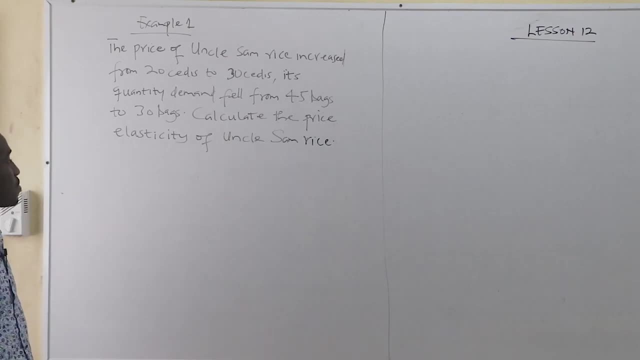 the price of angelson writes english from 20 cities to 30 cities, 820 demanded from 45 bucks, 30 bucks. calculate the price last year of the samurais. so let's see we have in ghana there's a rise. we all like so much american right we call. 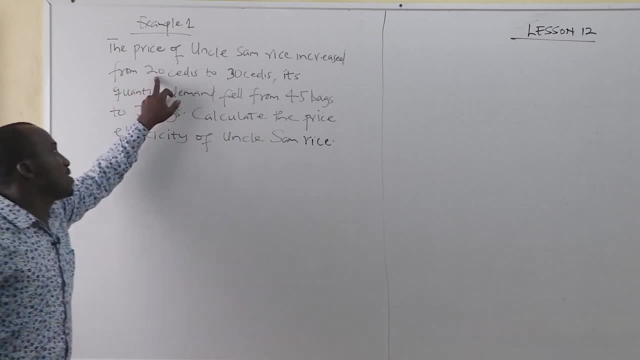 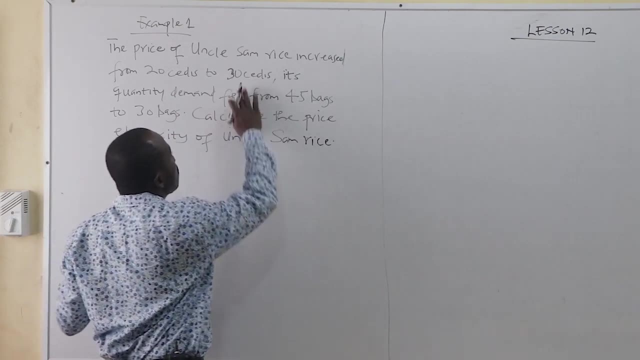 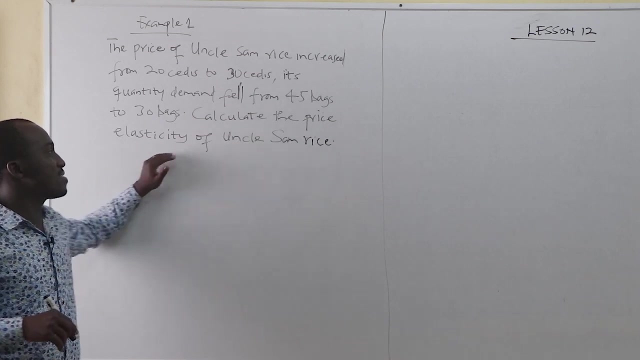 it, uncle sam. we are assuming that the price was 20. it increased to 30. and when it increased, what happened? the demand fell from 45 bucks to 30 bucks. calculate the price elasticity of the angelson rights. here we're going to use the point elasticity because the question didn't specify that. 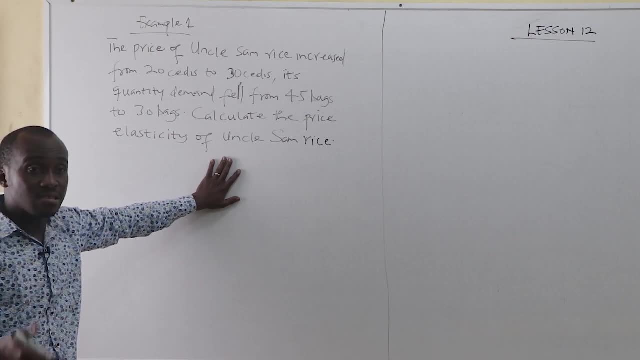 we use the accuracy. later i'm going to teach you how we use the accuracy, but here the question didn't specify. just use the point like, just use the point elasticity, right? so let's see later. you take a question, that's what's the question, and we solve it. this is just something to explain to you. 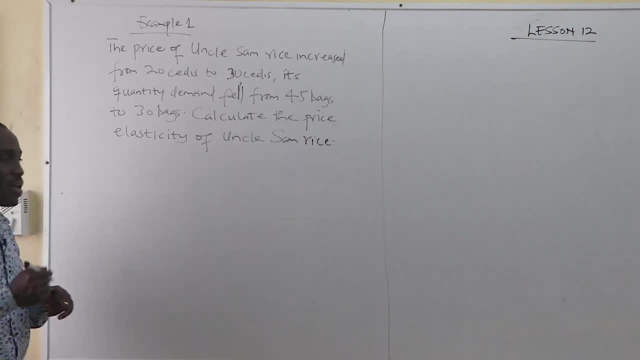 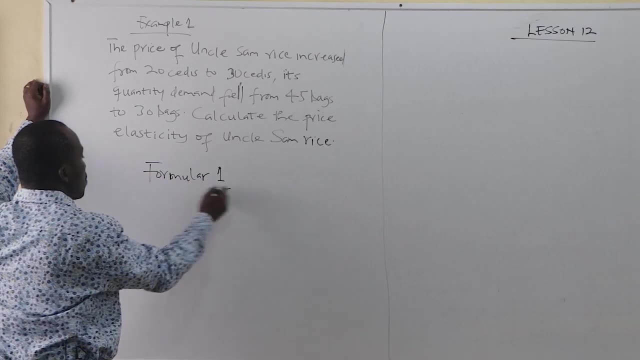 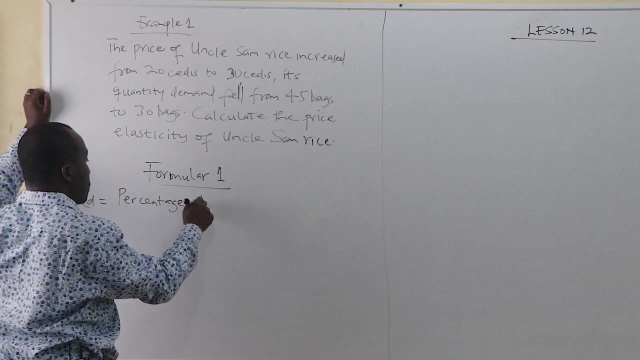 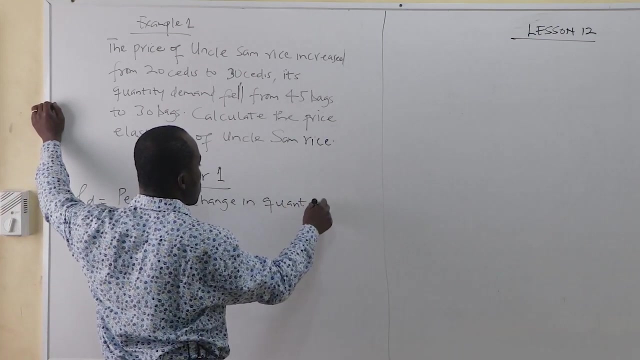 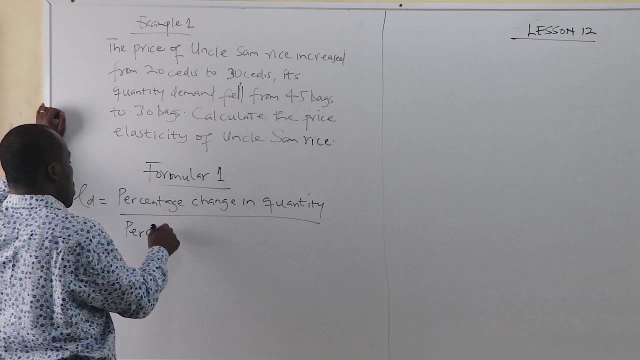 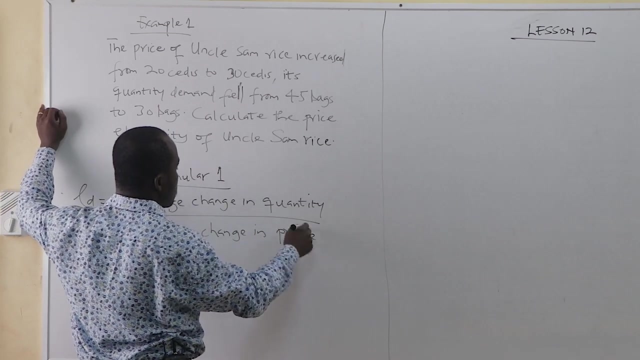 so that you understand the formulas i gave you. i gave you two formulas. let's go to the formula one. in formula one, with the elasticity of demand is equal to the percentage of price change in quantity demanded divided by the percentage change in price, right? so let's see first. 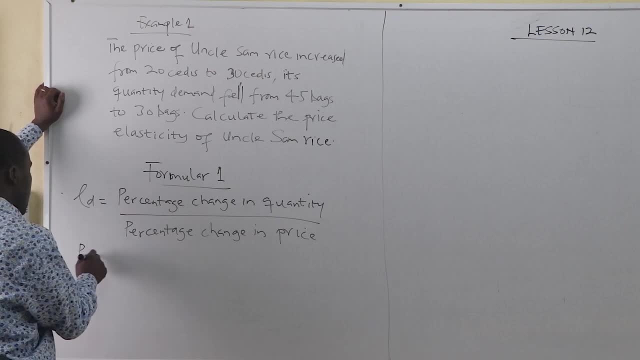 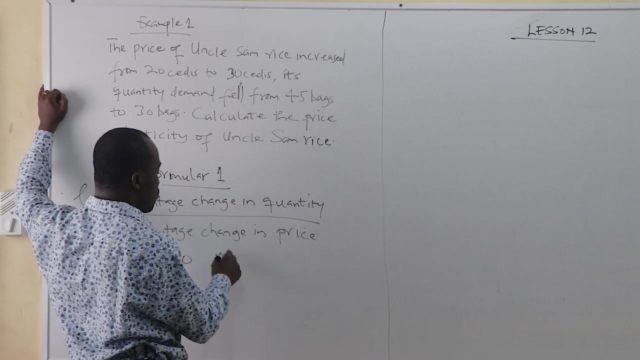 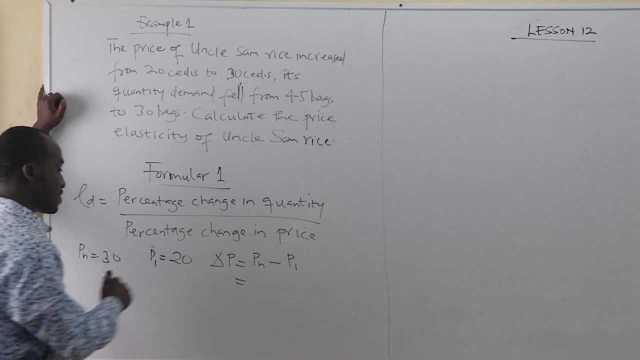 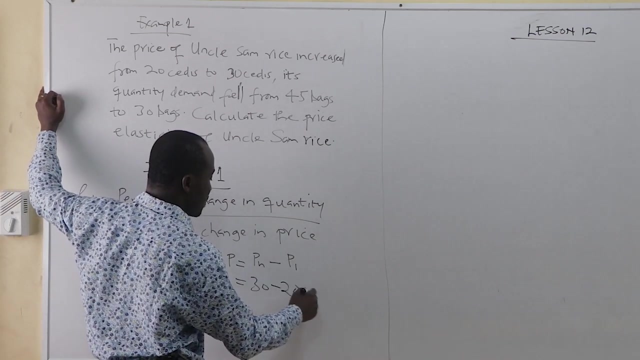 new price? the new price is 30. what is the initial price? the initial price is 20. what the changing price? changing price equal to the new price. by initial price, the new price? the new price is worth 30. what the initial price? the initial price is 20. what the difference? the difference is 10. so if you want to find, 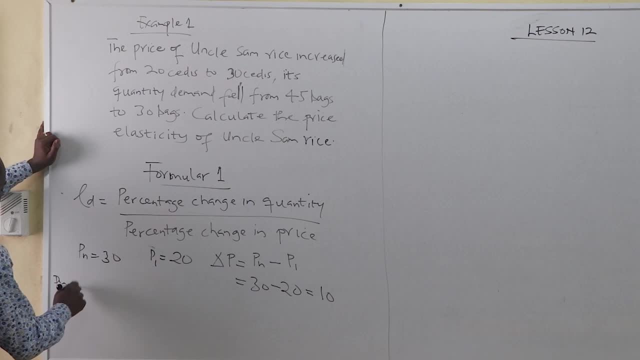 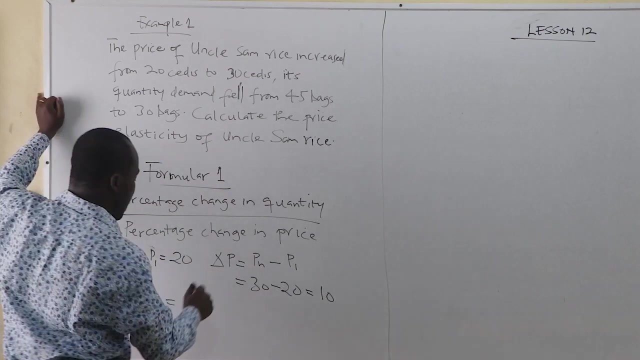 a percentage change, the percentage change. if you want to find a percentage change in price, it's going to be the change. what the change now is? what the percentage? let me see the percentage in price. it's got to the chain. a chain is 10 divided by the initial price. 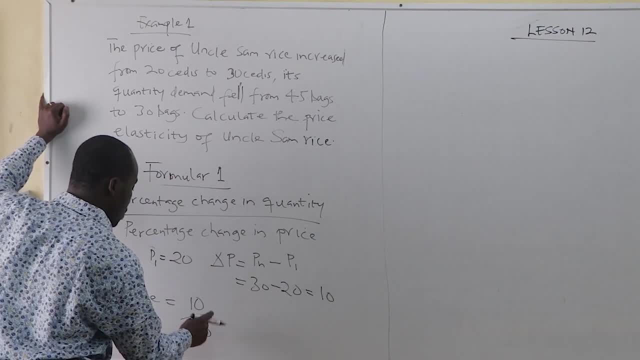 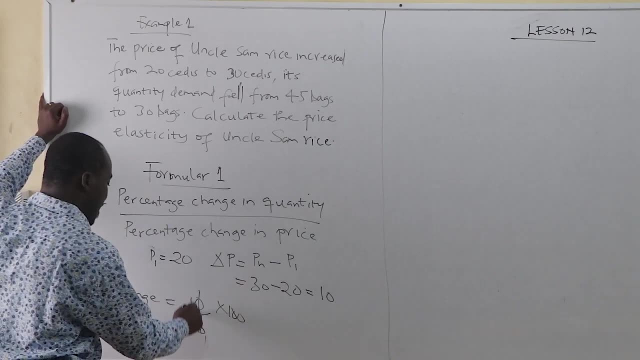 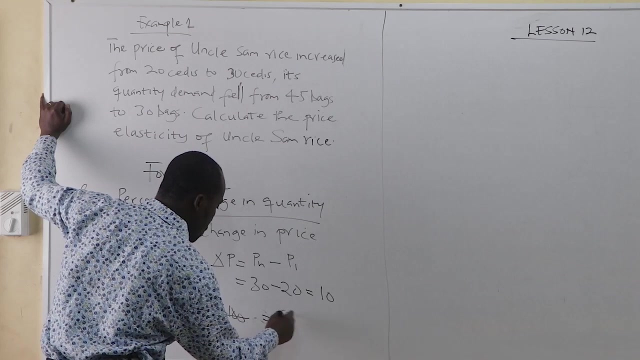 initial price is what 20? 20 times hundred, 20 times what hundred. so this council, this, this council, is what you get. you get 50% right is what you get. you get 50% right is what you get, you get 50% right. so the former is the percentage change in. 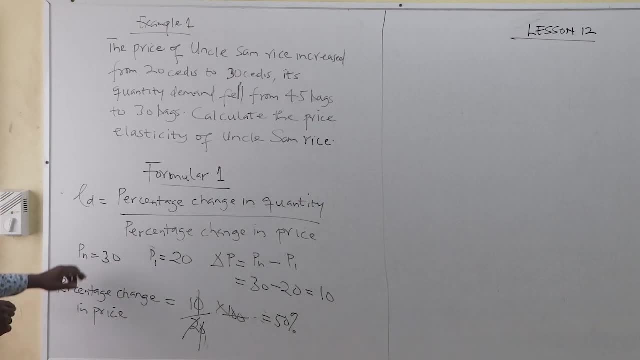 so the former is the percentage change in. so the former is the percentage change in quantity demanded. about a percentage quantity demanded. about a percentage quantity demanded. about a percentage in price. you have seen a percentage in in price. you have seen a percentage in in price. you have seen a percentage in price. we find out a new price was 30, the. 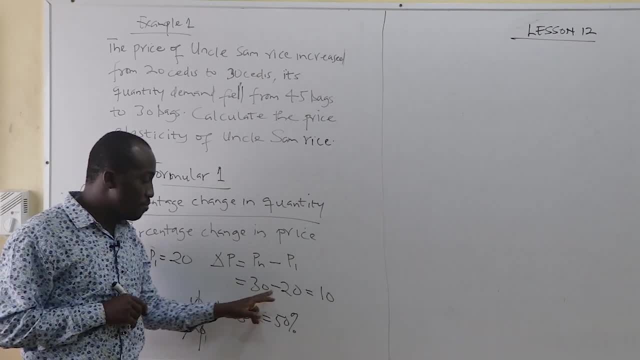 price we find out a new price was 30. the price we find out a new price was 30. the initial price was 20 and therefore the initial price was 20 and therefore the initial price was 20 and therefore the changing price is a 30 minus 20. that 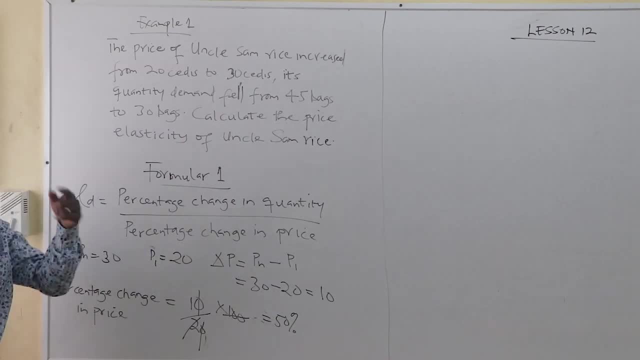 changing price is a 30 minus 20. that changing price is a 30 minus 20. that gives you 10. so you want to find a gives you 10. so you want to find a gives you 10. so you want to find a percentage change here. interested in the. 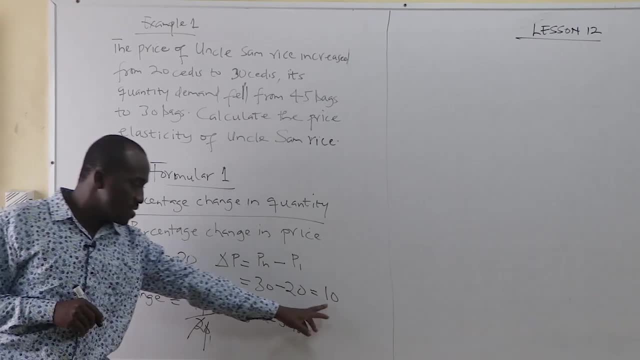 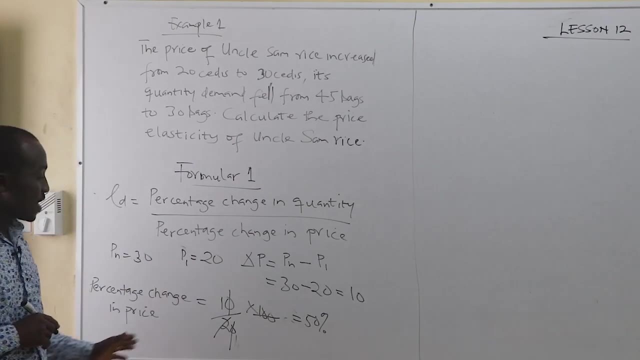 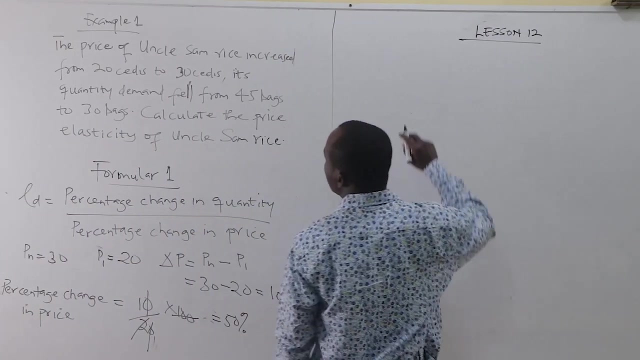 percentage change. then the new: the change does the 10 divided by the initial price as 20 times hundred, and when you cancel you are going to get 50 percent. let's find out the percentage change in quantity demanded. so the percentage change in quantity demanded. what's the new? what is the new demand? the new. 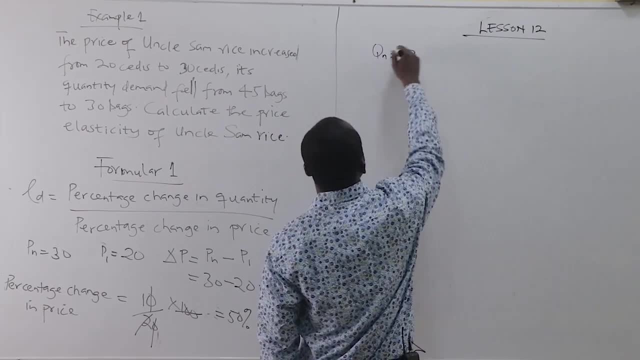 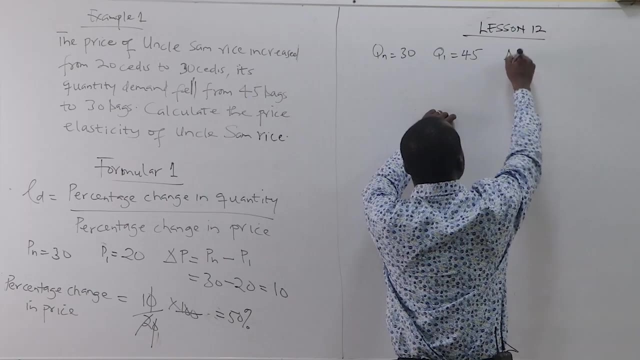 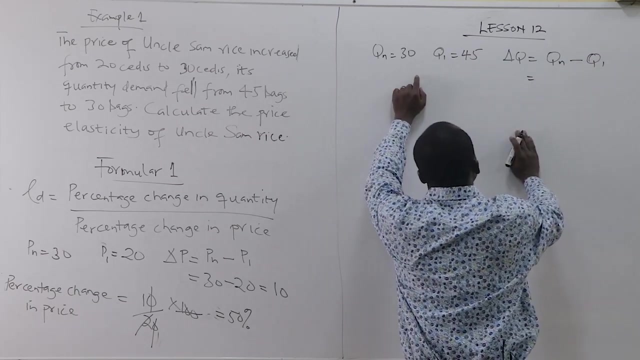 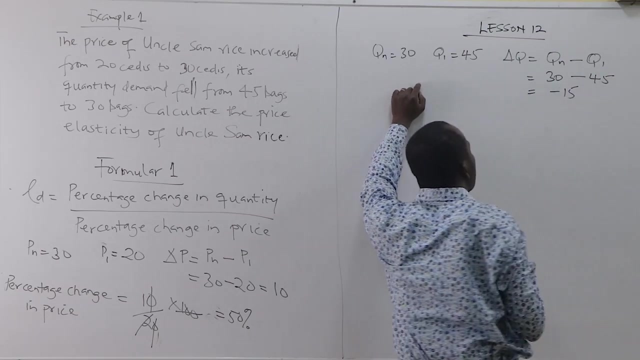 demand is what: 30. the initial demand is what: 45. what did you change in quantity? the change is the new minus initial. what is the new one? 30. what is initial one, 45. what do we get? negative: 15. so the new quantity is 30. 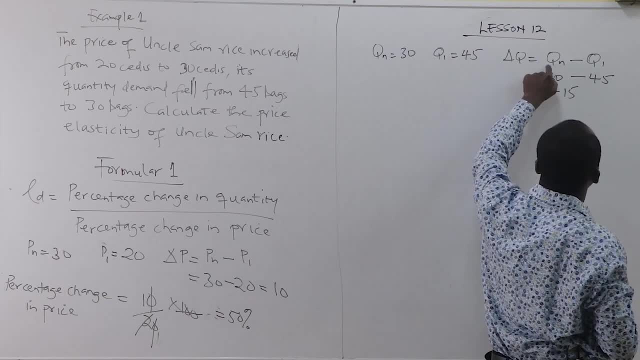 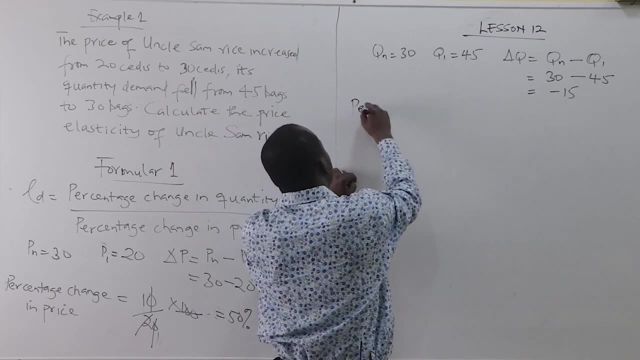 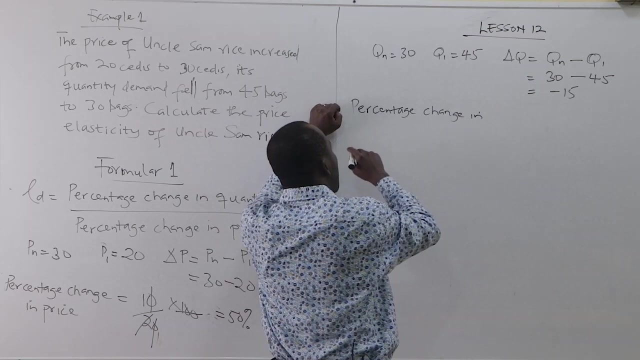 The initial quantity is 45.. So what's the change in quantity? The change in quantity is the new quantity minus the initial quantity: is 30 minus 45. That's the change. What is the percentage change? The percentage change in quantity. 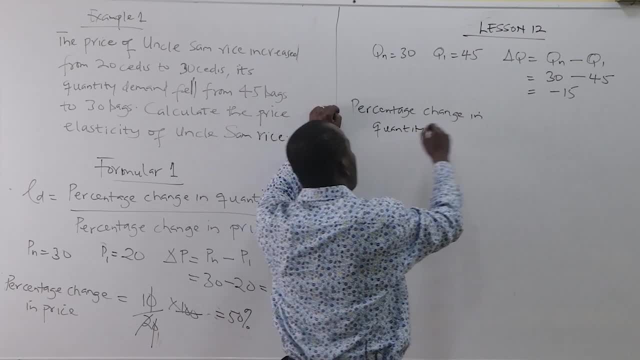 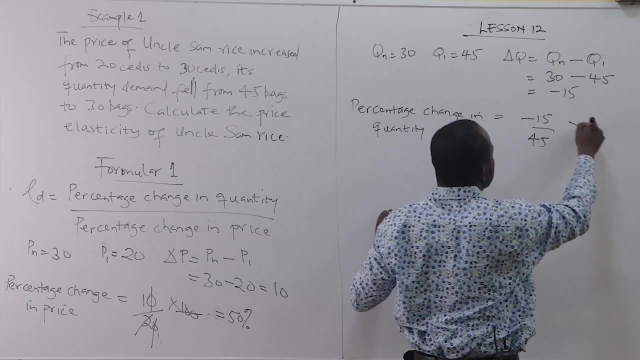 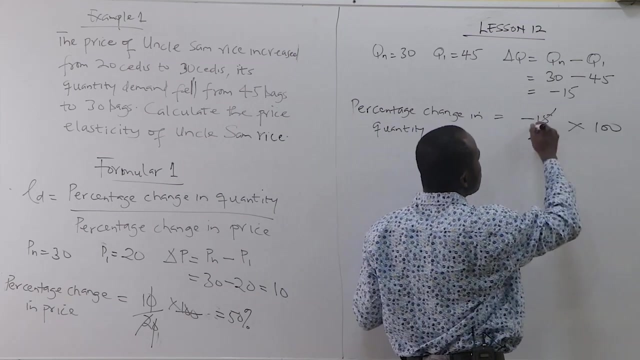 So that's going to be negative. 15 divided by the initial quantity is 45 times 100, right, So 15 goes to 15. once 15 goes here three times, We're going to have negative 100 times 3.. 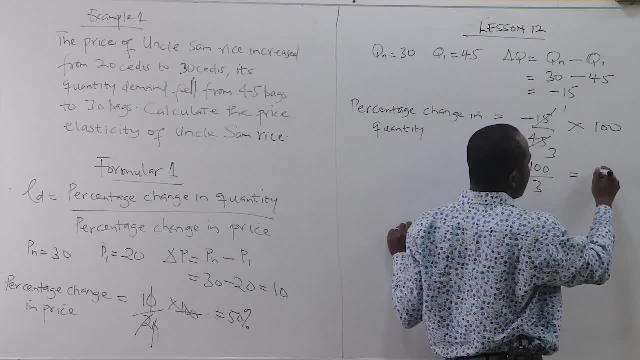 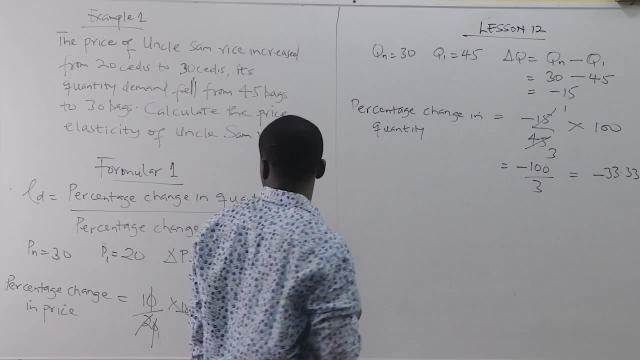 What are we going to get? We're going to get something like negative 33.3.. 3,, 3, 3.. Okay, So what's the elasticity? Let's find the elasticity. The elasticity here, as I told you, is the percentage change in quantity demand. 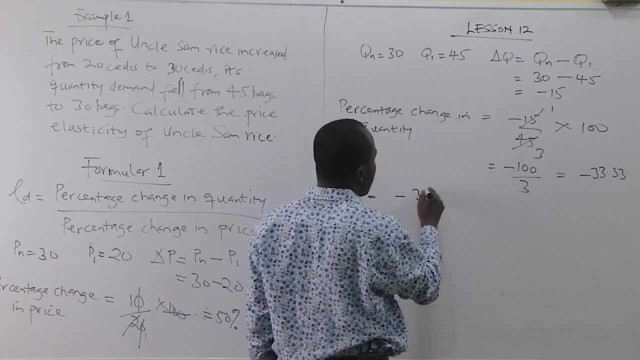 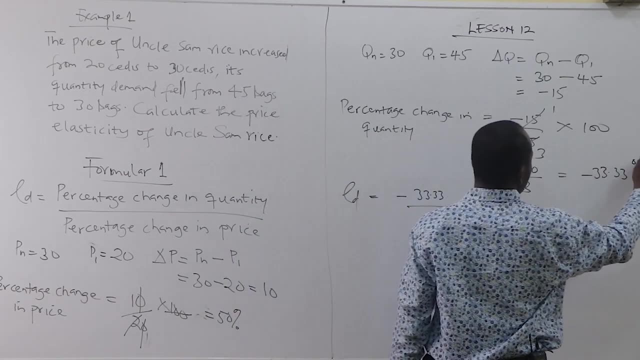 What's the percentage change in quantity demand? It's equal to negative 33.3.. And what's the percentage change in price? The percentage change. so this one is percent, This is percent. What's the percentage change in price? The percentage change in price is what. 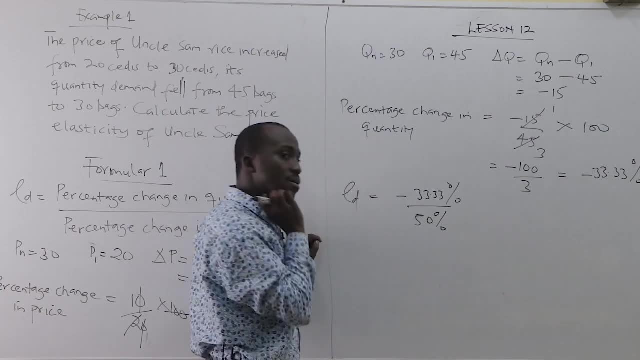 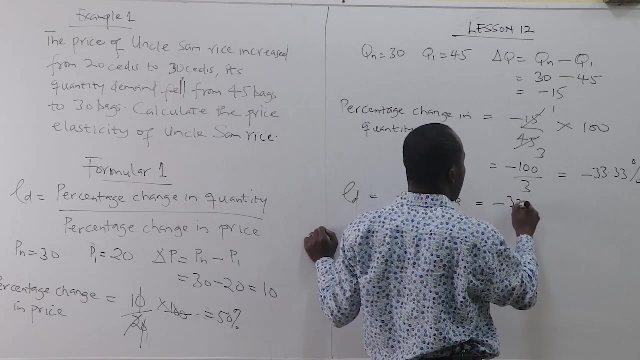 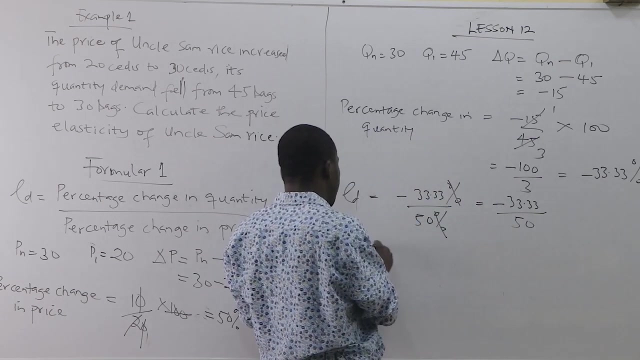 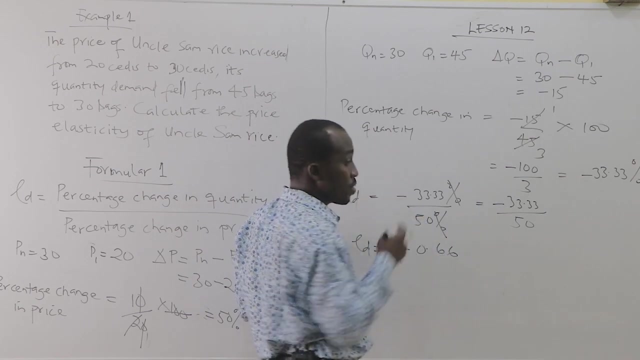 50 percent, right. So let's cancel the percentage. what's left is like we have negative 33 over 50.. So you can use the calculator to punch and let's see what you get. So if you divide, you're going to get 0.666, right. 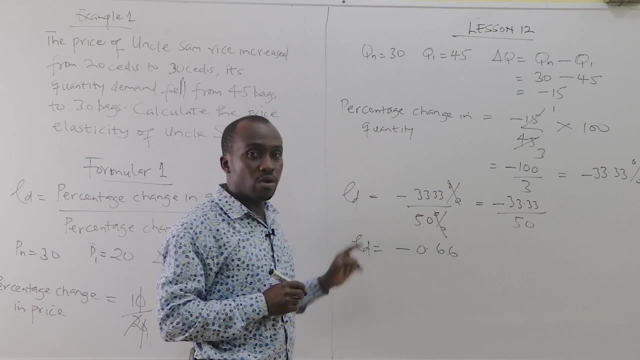 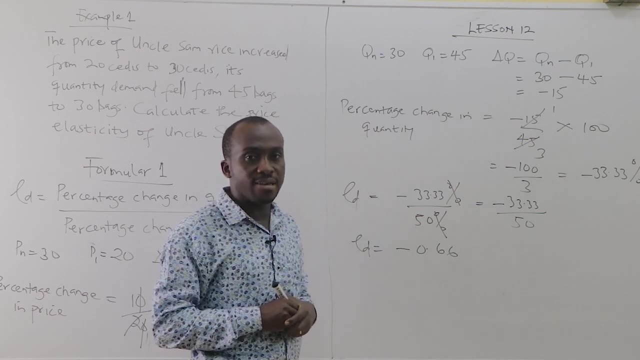 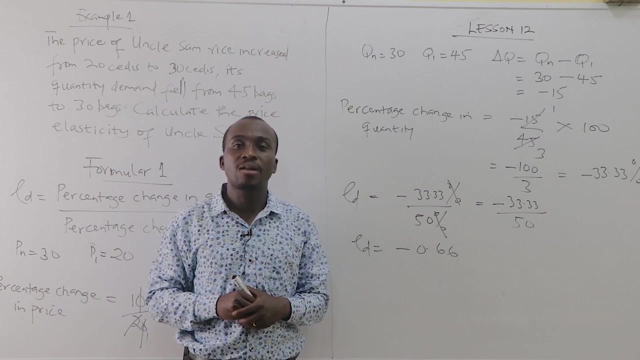 And let me say that any time you do price velocity of demand, you're going to get a negative figure. Why? Because the relation between price and quantity demand is negative. If price goes up, demand will fall. If price goes down, demand will rise. 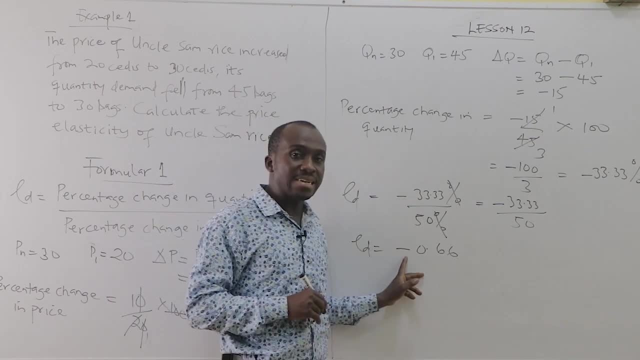 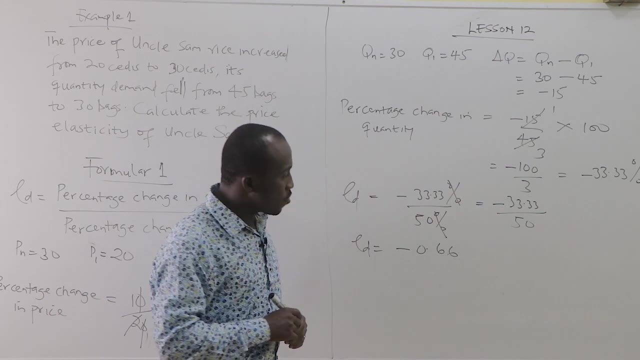 And therefore the elasticity of demand is always what Negative right. So any time you can use price velocity of demand, your answer should be negative. So if you want to interpret, what you have to do is that you have to take the absolute. 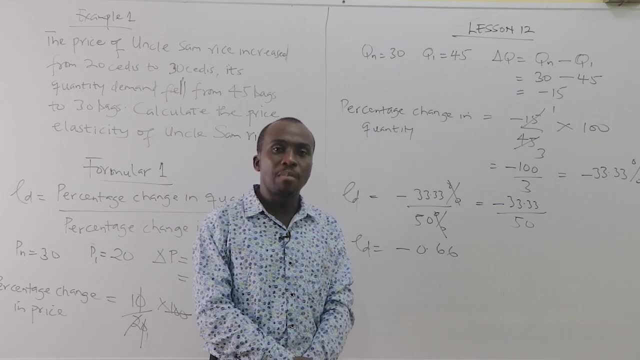 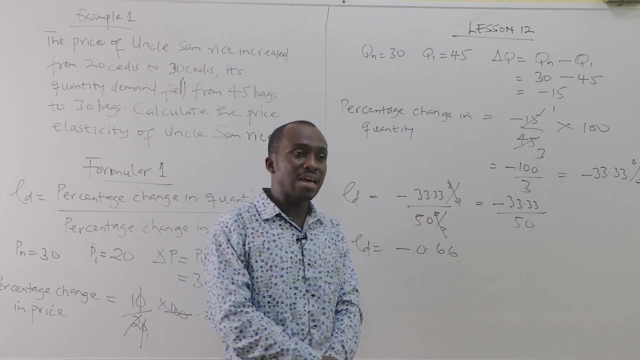 If you want to take the absolute, It means that make the figure positive. If it's negative, make it what Positive, Right. So let's take the absolute. So the reason why you have to take the absolute before you can interpret, because always your 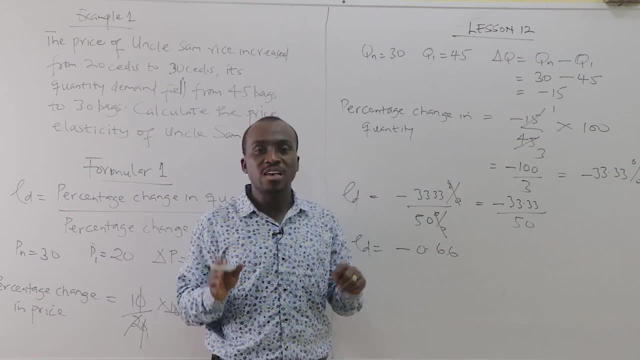 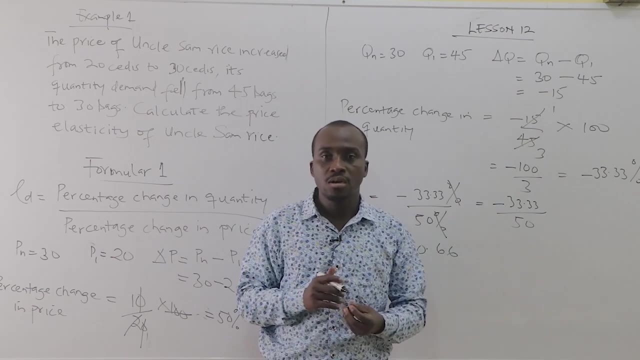 answer is in negative. Otherwise you say all gos are inelastic because they are all less than one, Because always the answer will be in negative Because of the negative relationship between price and quantity, all three above the value. you have to understand well that the relative sensor 沒有 distraction. 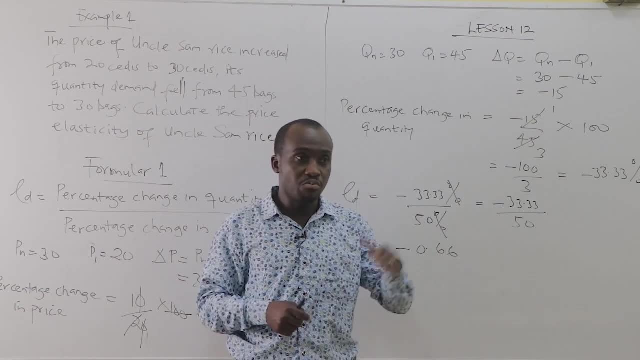 So I remember when I'moo singing. this is the stacking of the values on your instrument. When you're going into a big Square, you usually have a big Spanish square. What does that do to the across the square? It salt it. 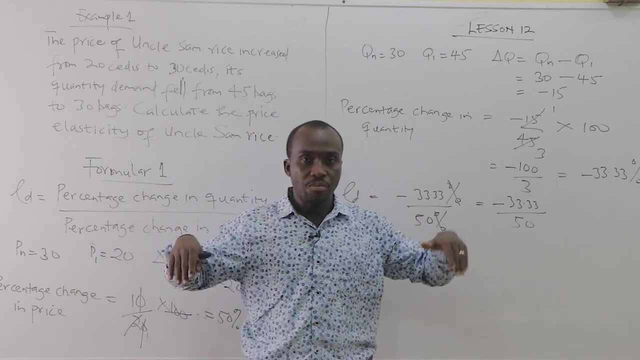 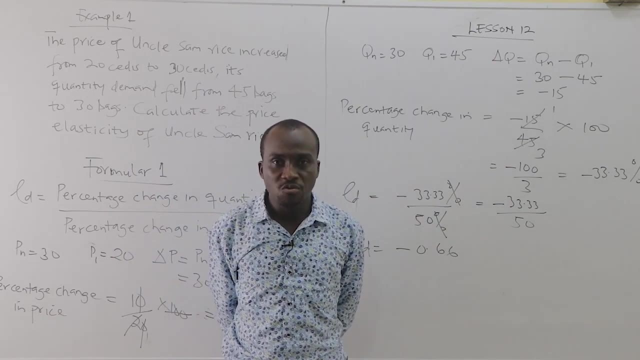 quantity demanded, right, if price goes up, demand falls, and when price falls, demand rise. so there's that negative relation. so always you have a negative answer. so for you to interpret, what you do is to take the absolute. you take the positive figure and interpret whether is it greater than one or less than one, if you 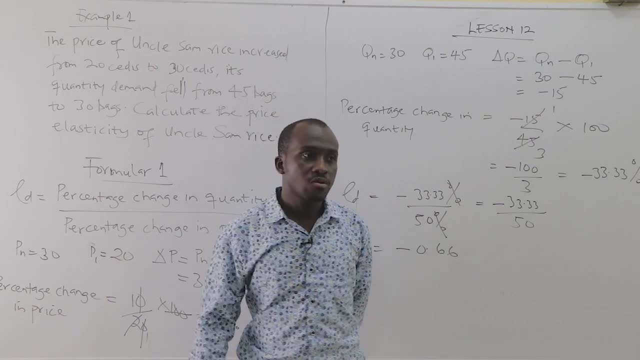 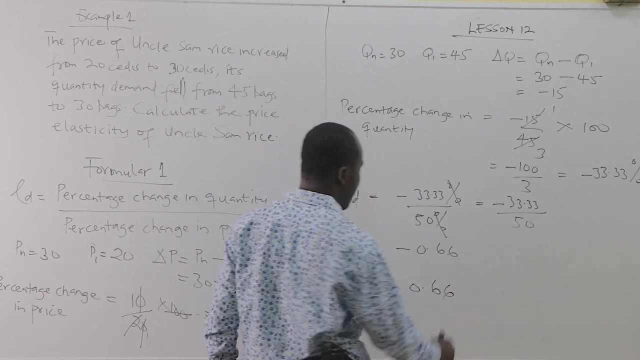 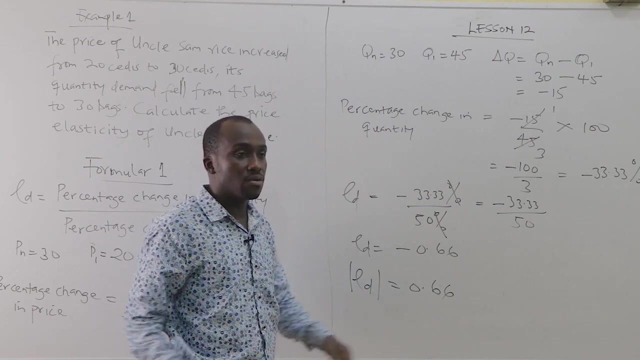 don't do that. always all your answers will be less than one because of the negative sign. so let's take away the negative. let's take the absolute. absolute- there's a symbol- gives you 0.66. so the absolute value will give you what 0.66 make it positive. is it less than one or greater than one? it's less. 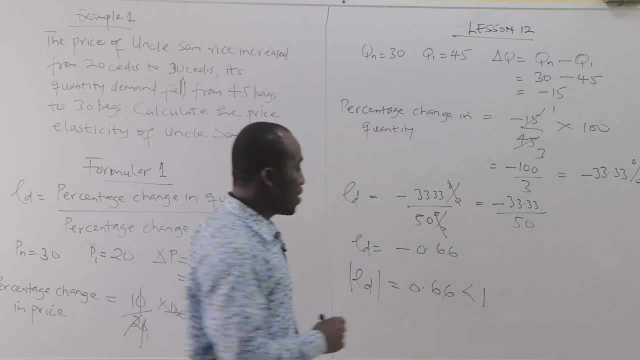 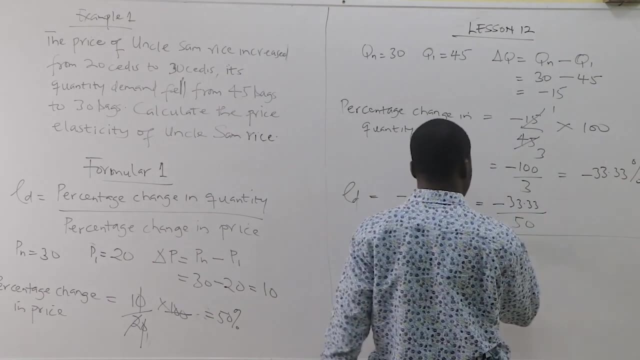 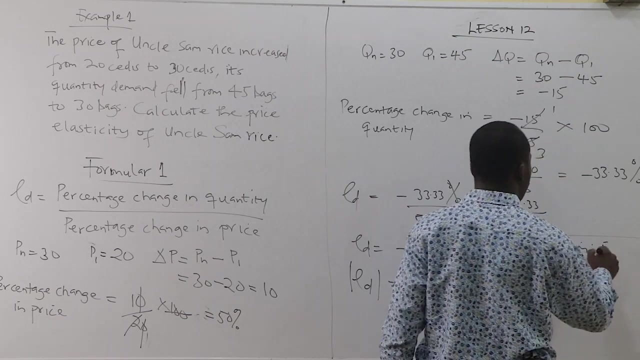 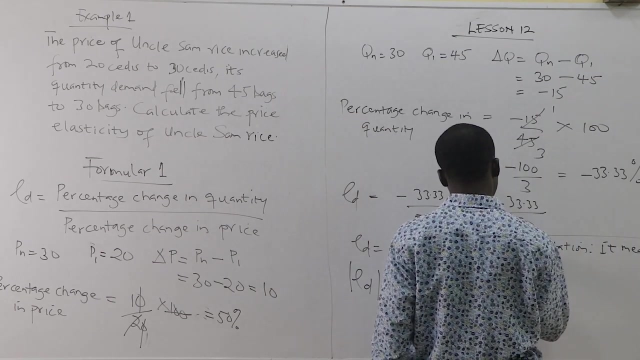 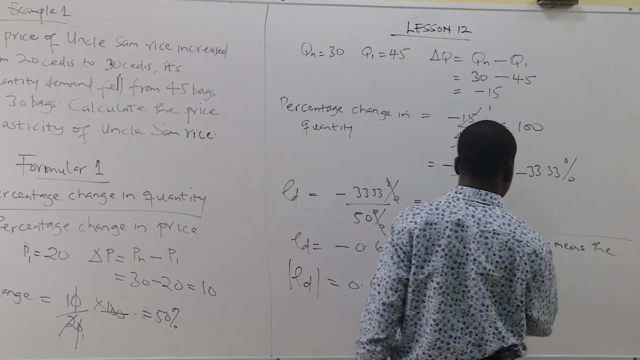 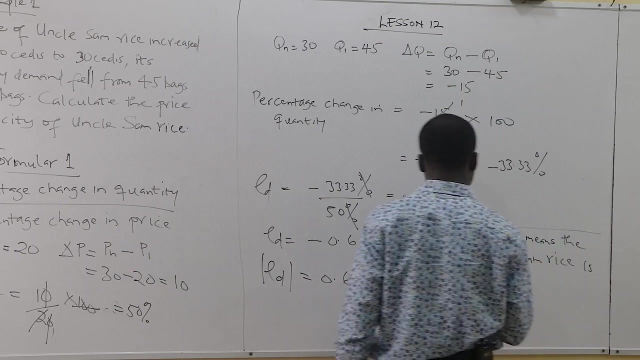 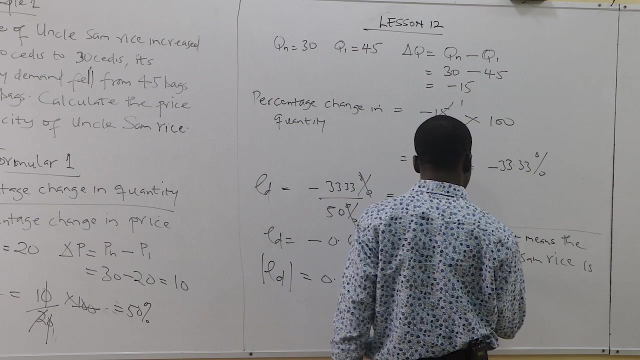 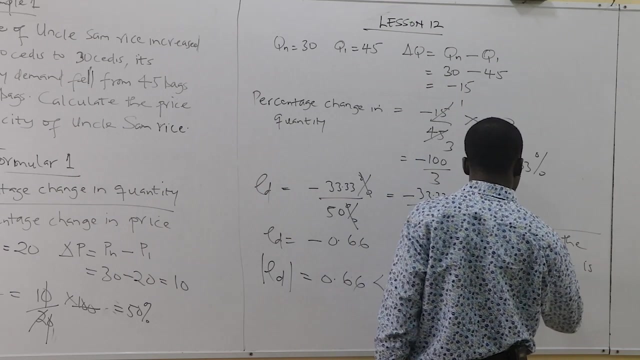 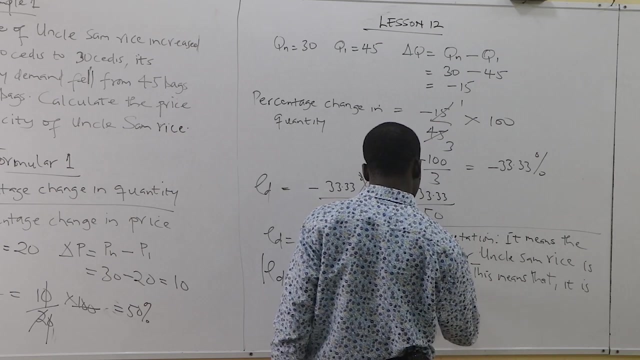 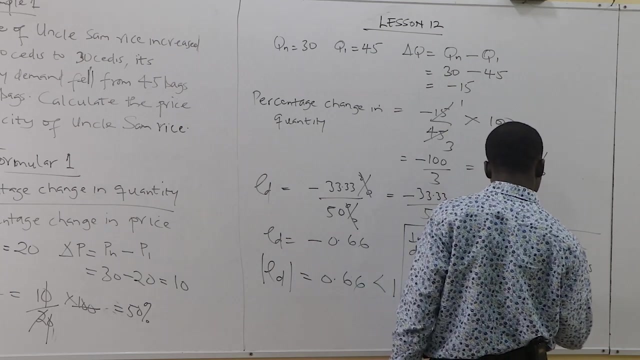 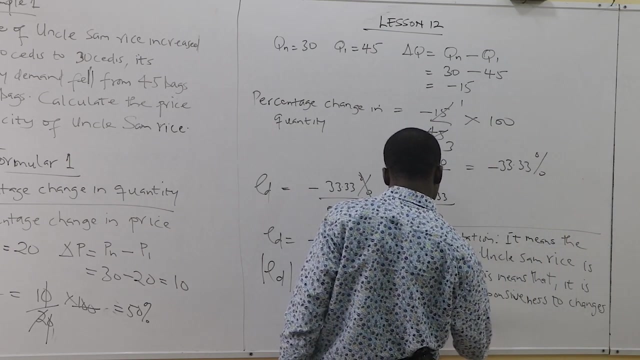 than one and when it's less than one, it means the demand. what does it mean? interpretation? let's see. what does it mean? let's see the interpretation. it means the demand for uncle, uncle sunrise is in an inelastic meaning. this means that it is slightly responsive to change in price. 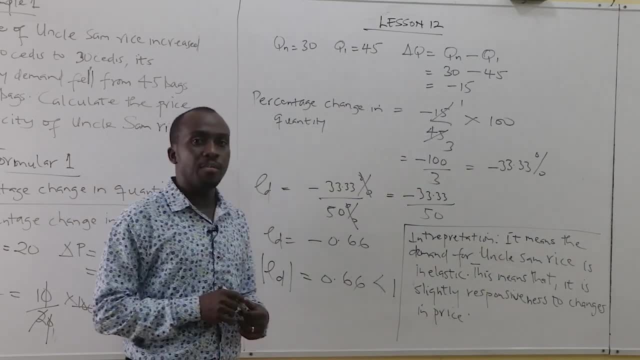 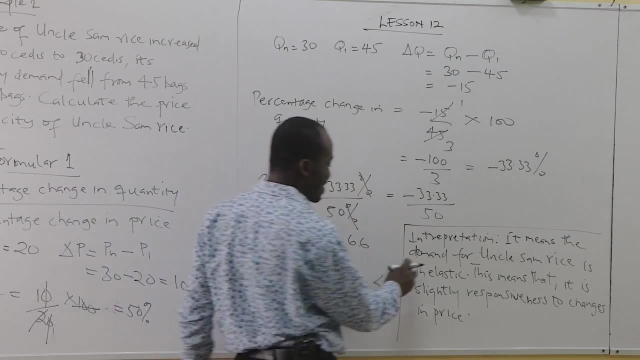 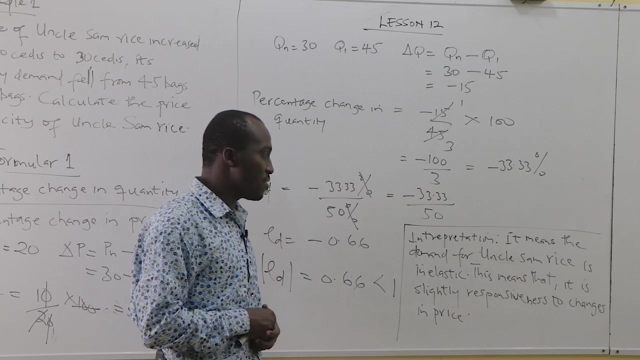 so I told you that when the elasticity is less than one it means that the commodity is in elast. so it means the demand for uncle sunrise is inelastic. what does it mean? that it is slightly? the demand for uncle sunrise is slightly responsive to change in price. so even if 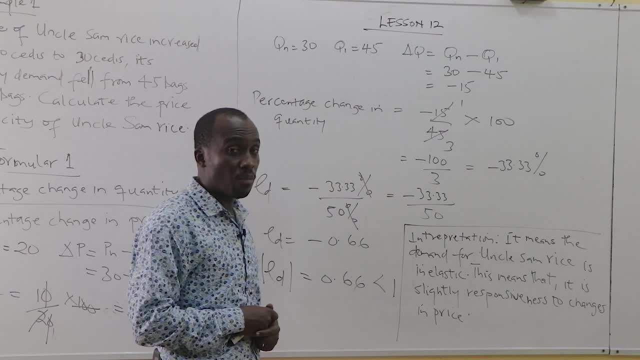 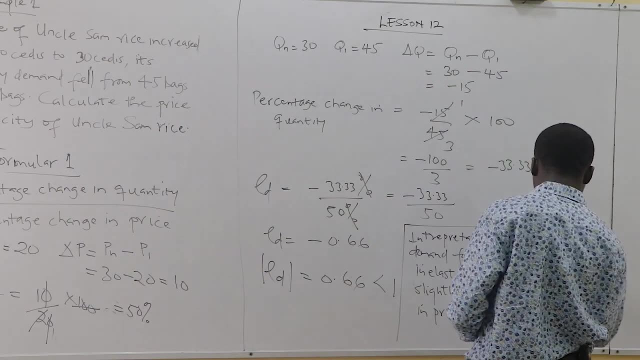 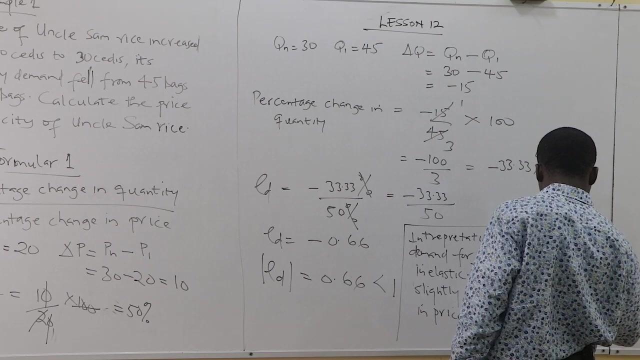 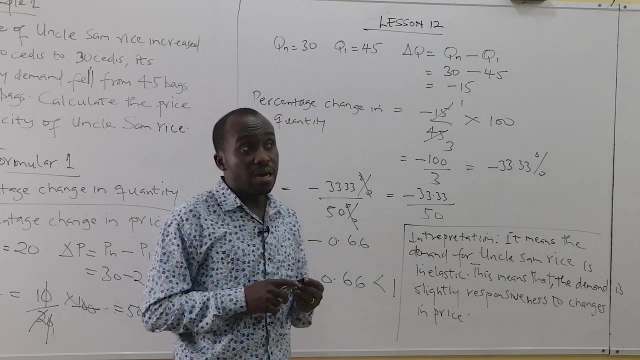 the price increases, Ghanaians will still be buying. only a few people will stop buying, but they like the price. that's what it means. if the price even increases, it means that the demand- okay the demand- they demand a slightly responsive to change in price. so if the price even increase from maybe hundred hundred ganas, it is to recognize. 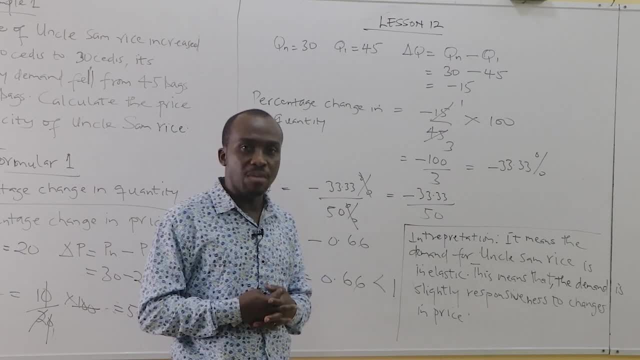 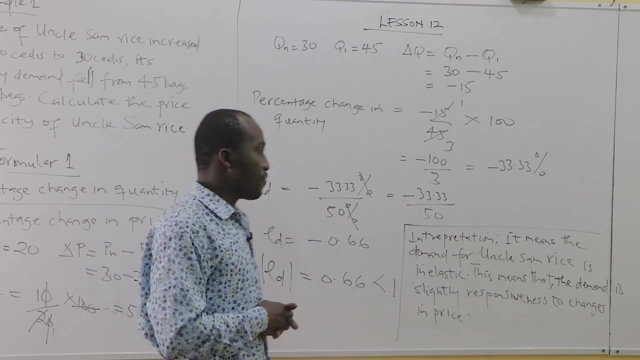 it is only people stop buying. a lot of people keep on buying, meaning that the demand for Uncle Sam rice in Ghana is inelastic. people like Uncle Sam rice. they're not worried about the increase in price. that's the first formula. so anytime you do elasticity here you have to interpret. don't leave it like that. 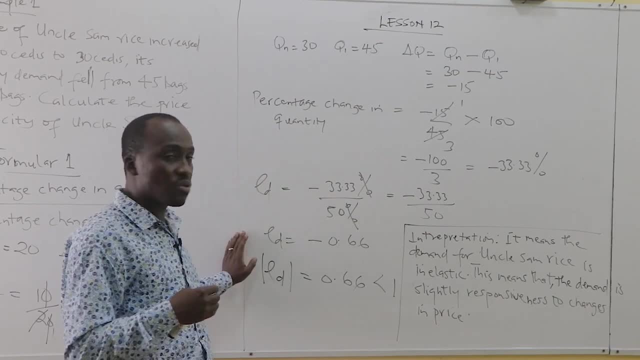 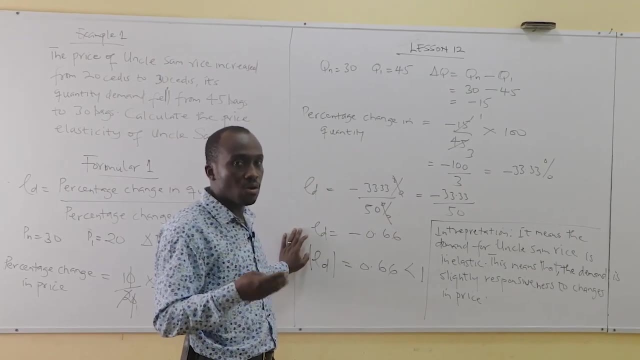 now they will mark you wrong. interpret first: take the absolute, make it positive, find out: is it less than one or greater than one? if it's less than one, it's inelastic. if it's greater than one, it's elastic. then you interpret. what does it mean? let's use the formula two. we are still on this question. we first. 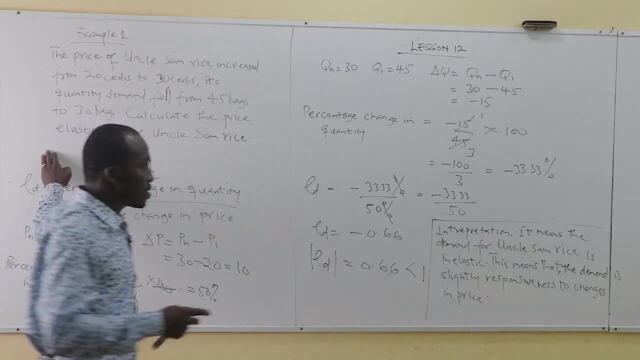 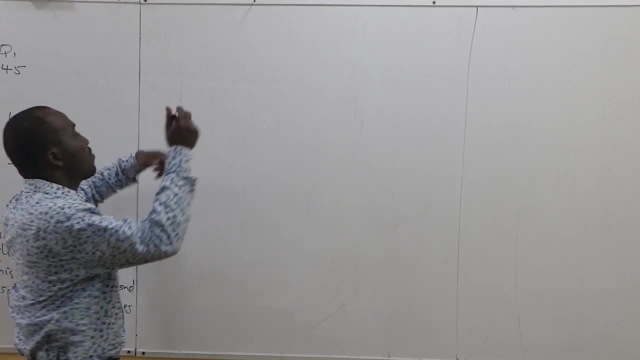 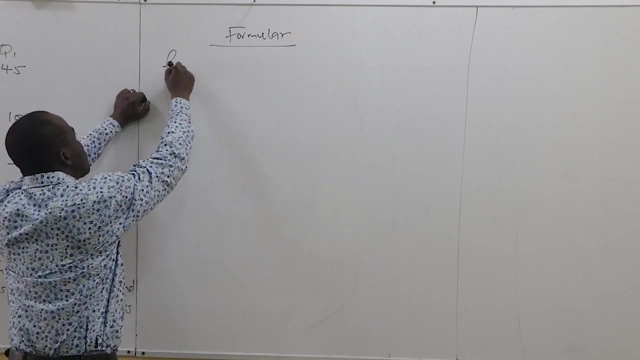 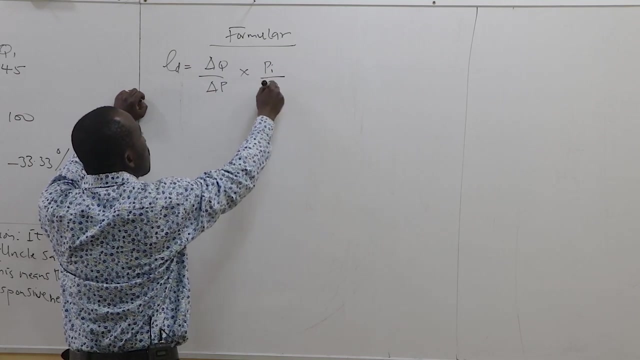 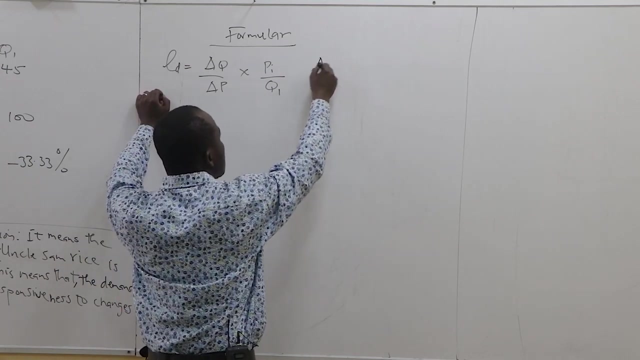 use the first formula to solve it. now let's use the second formula to solve it. let's get the formula two still on the point, elasticity. the formula two. these are aware often demand is going to change in quantity by changing price times, initial price times, initial quantity. right, and I tell you that the change in quantity 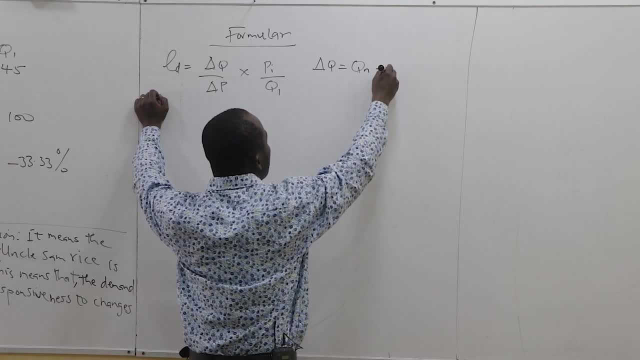 because of the initial, the new quantity line and initial quantity. the change in price differently can be always changed to a change in quantity. but this is fixed quality and only change the min if конечно price like choose price value to change in quantity. the new lens quality line is the nic bize quantity. it change in price. you change in priceif the price in a point less elastic Greetings from multiple subjects waiting for your questions. 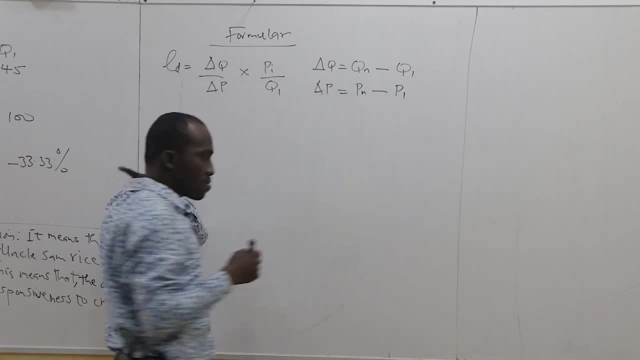 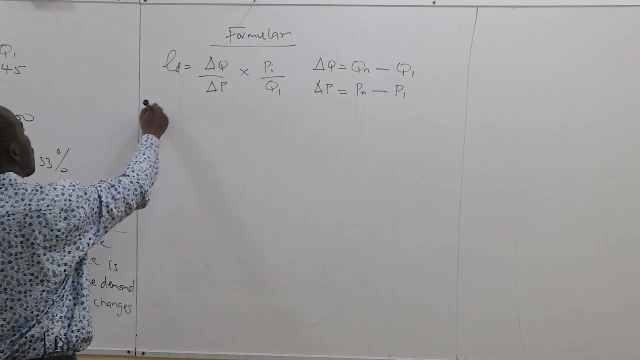 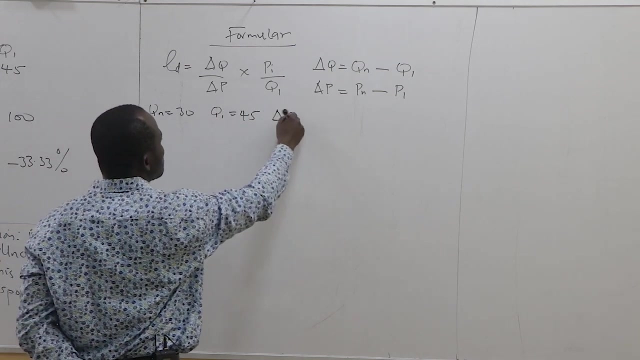 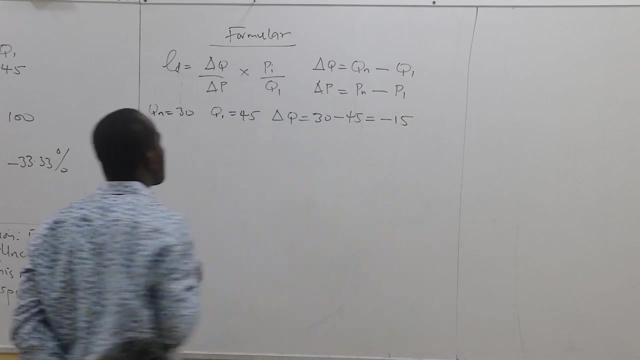 equal to the new price minus initial price. what the change in quantity? the new, what is the new quantity? the new quantity is 30. the initial quantity is what- 45. what they change? the change is 30 minus 45. that gives you a negative 15.. what about the new price? the new price is what? 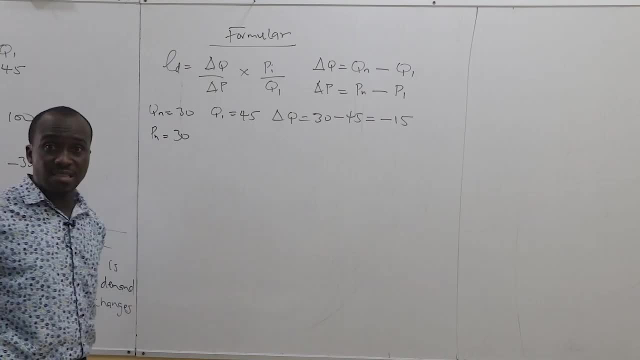 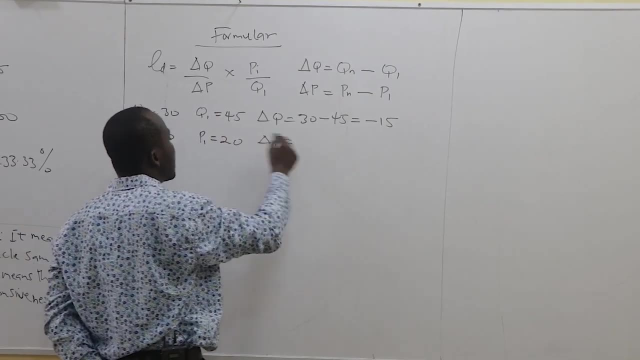 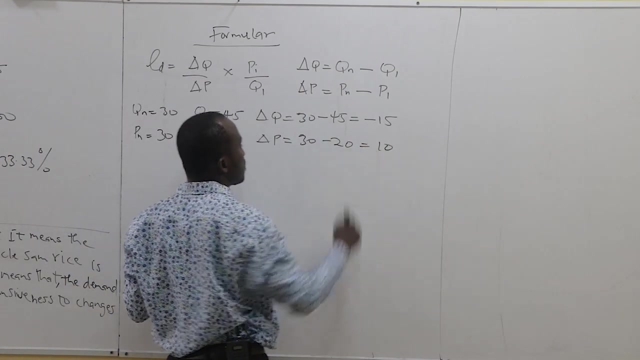 30 from the same question. we are using the same question. the initial price was what? 20 what the change in price? it is the initial, the new minus the initial. that gives you 10.. so we have that. so when you finish you have to fix them back into the formula. 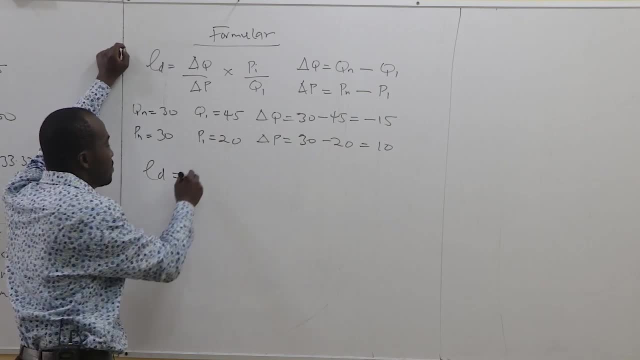 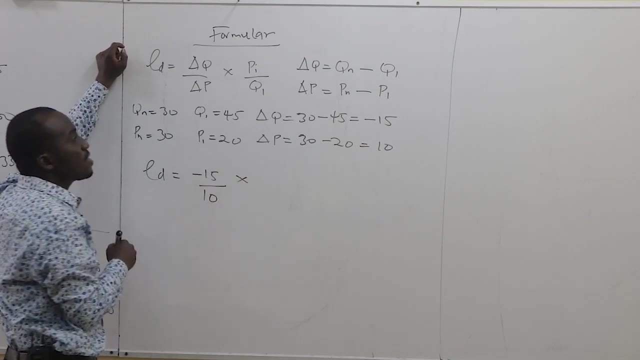 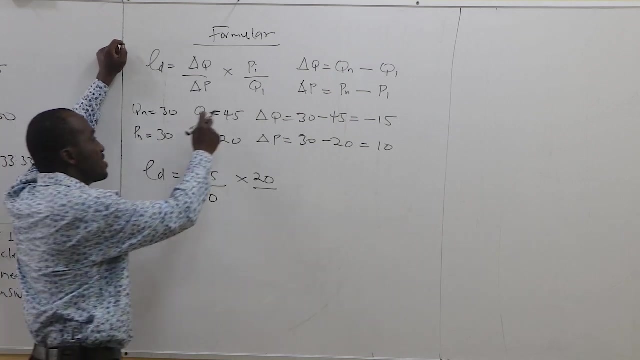 the formula says that the change in quantity, the change in quantity, negative, 15.. why the change in price? the change in price is 10.. what's the initial price? the initial price is 20, is here, and what is the initial quantity? the initial quantity is here. is what? 45.. so you have this. 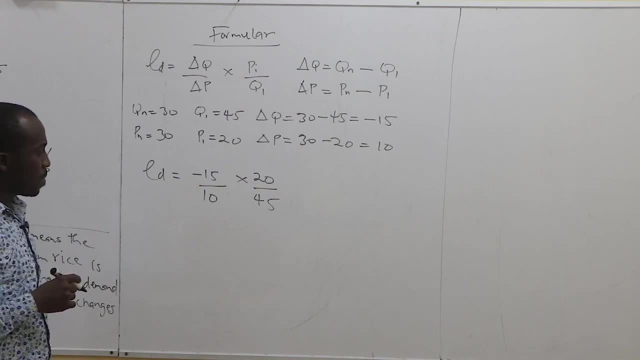 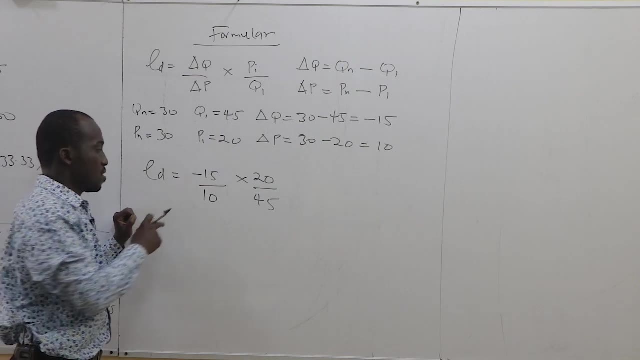 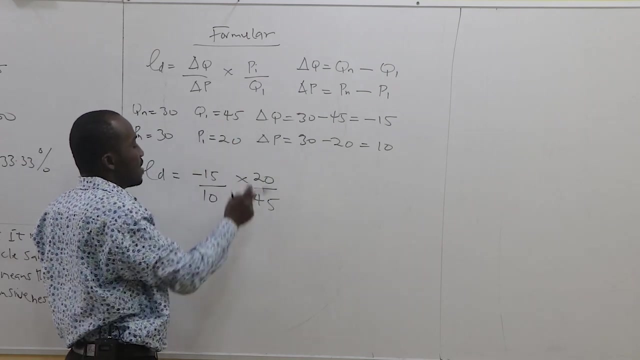 negative 15 minus 10 to the new change in quantity is the negative 15, the change in price is 10, the initial price is 20.. the initial quantity is 45.. so let's see, let's see what will be our final answer: zero or zero. 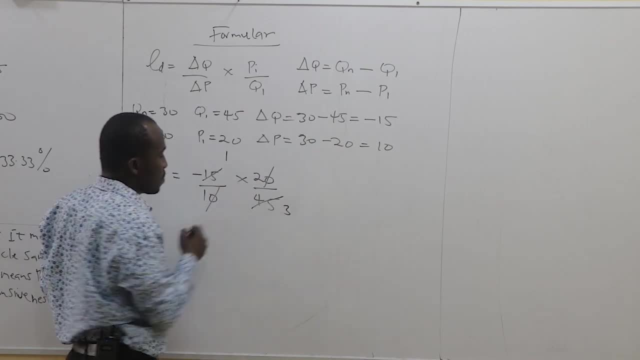 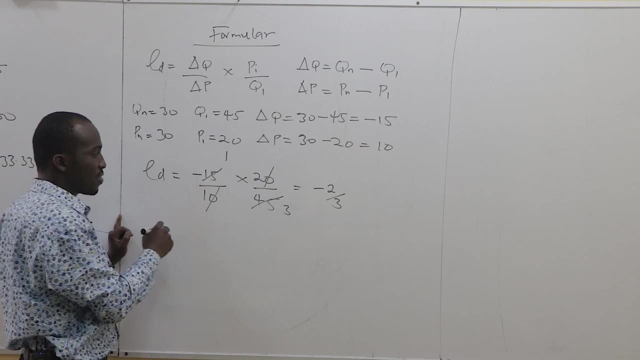 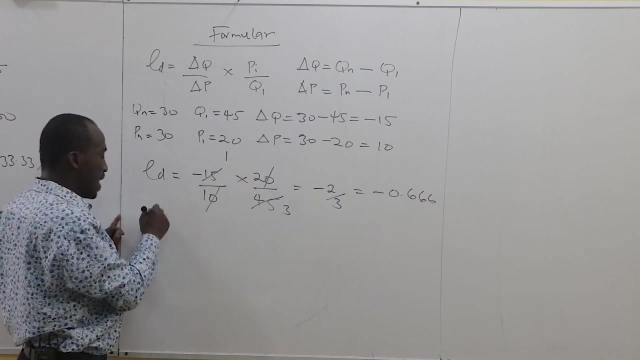 15 goes into 15 once 15 goes here three times. so what do we have? we have negative two divided by three, and when you divide, never give it two by three- you're going to get negative 0.666. it continues, so the elasticity is equal to negative 0.666. whatever 0.6, it's okay. 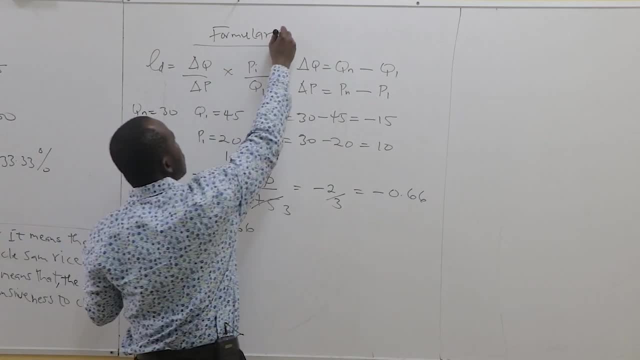 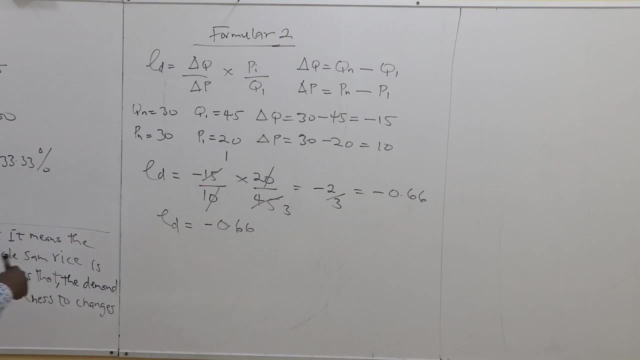 so whether you use this approach, this formula 2, for the point elasticity, what? i use this approach for the point velocity or use this approach for the point elasticity, you end up getting the same answer. right, but i use this approach for the point velocity or use this approach, formula one, from latin, the answer is still. 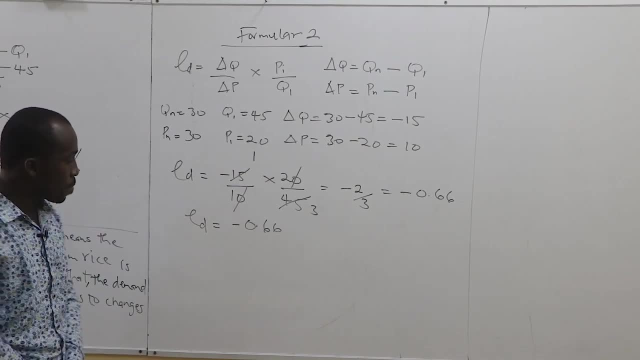 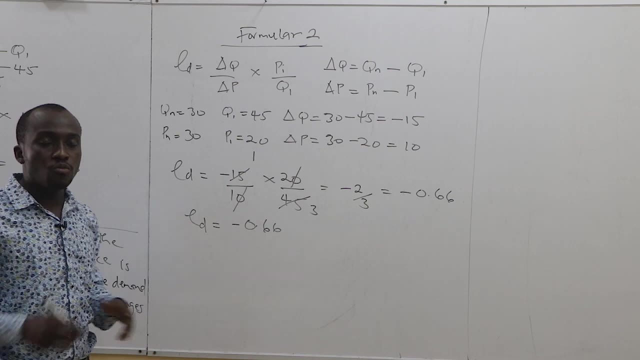 the same, so you can use which one. they're very convenient. and i tell you that, the same way, in order to interpret, you have to find the absolute so that you make it. you make it, uh, positive, because always the price of demand will give you a negative figure because of the negative relation. 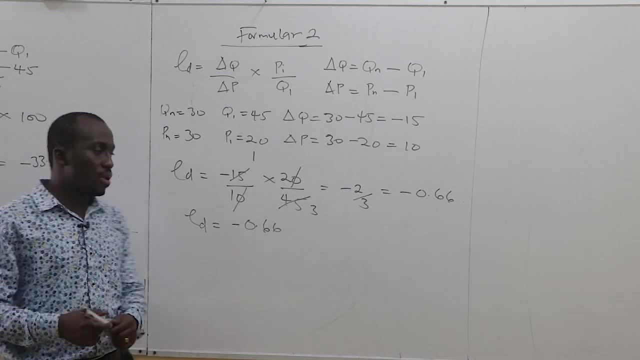 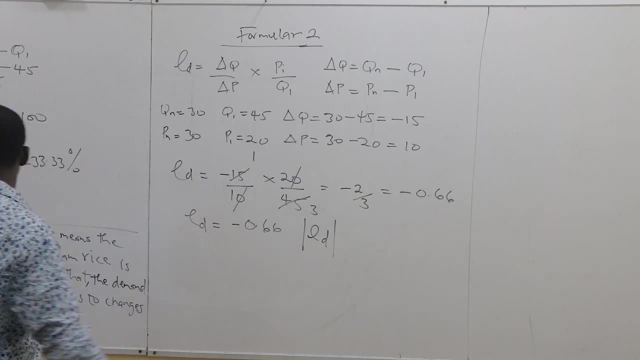 between price and quantity demand. so let's find the absolute. the absolute. this is the symbol. when you bring this symbol means absolute the bracket. so here to the same thing. when you bring that symbol means absolutely, you're making the figure positive. if you got not, it's negative. 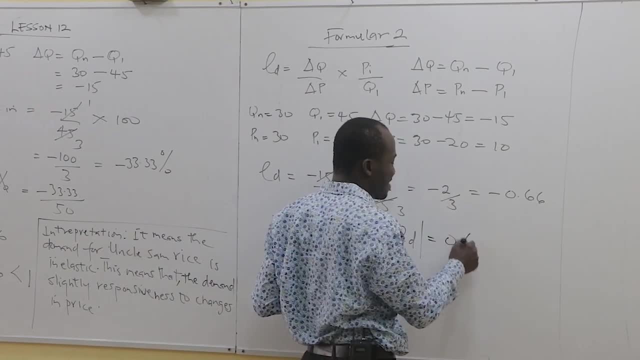 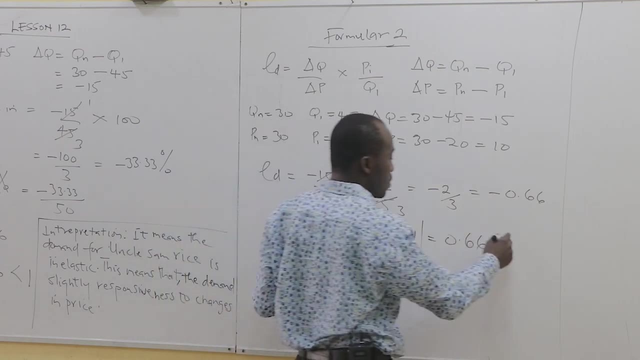 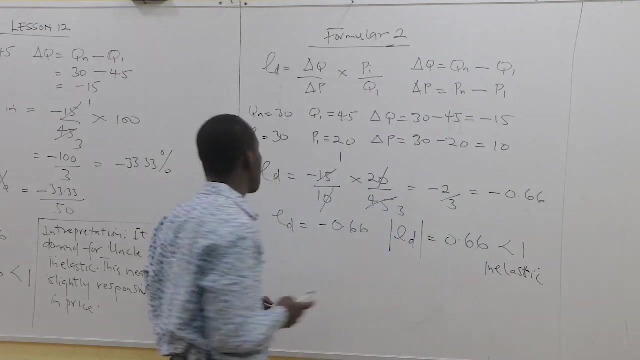 make it positive. when you do that, you're gonna get 0.66. is it less than one or greater than one? it's less than one meaning. that is what inelastic. so the same interpretation as we did here. so what are we able to understand? we understand that. 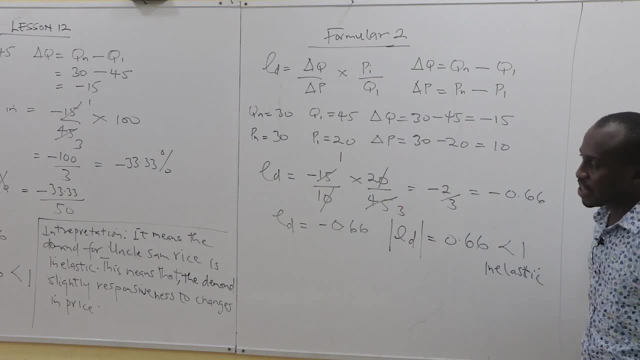 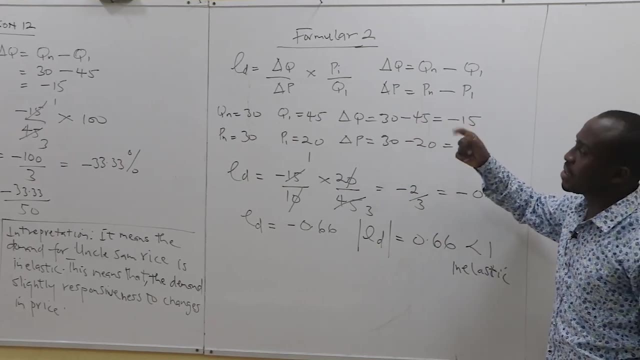 we're the point: elasticity. whether you use the first formula, the position, a change in quantity demanded, demand number divided by the percent change in price, or use this formula: price like this: is going to change in quantity demand of a change in price from the initial price, initial one demand, while each only formula you use, you end up getting the same answer. 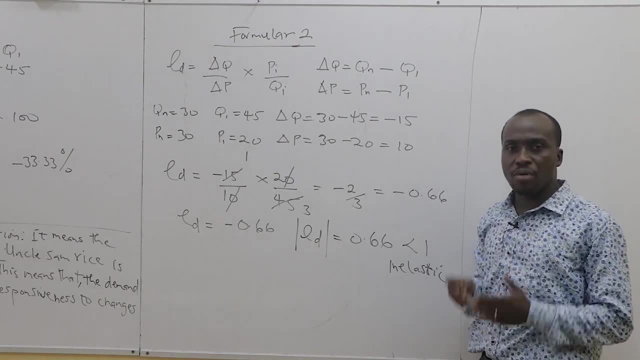 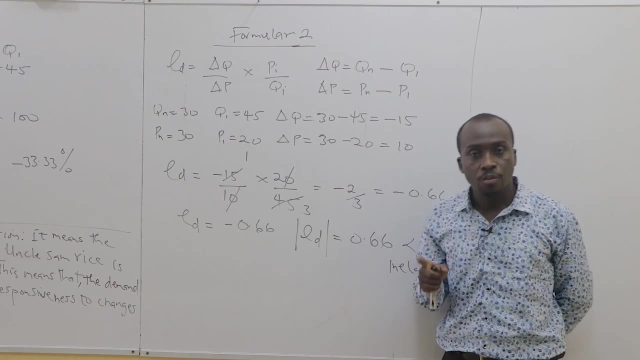 and let me also restrict that. any time you calculate price as a demand, you're supposed to get a negative answer. if you don't get it, it's wrong. it doesn't follow intuition, because we are able to understand that a lot of demand makes us understand that. 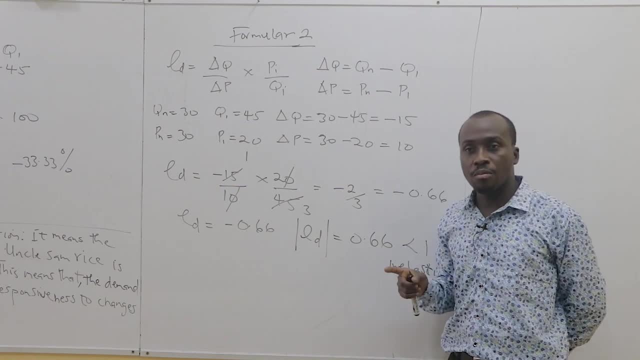 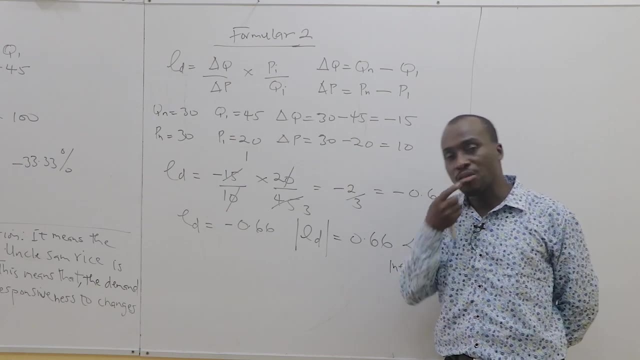 the price and quantity demanded is negative related. when price goes up, demand falls. and you see from the example, when price increases from 20, 30, demand decrease. and when price decrease to demand falls, a demand increases. the way of that reason, always your answer will be negative. so 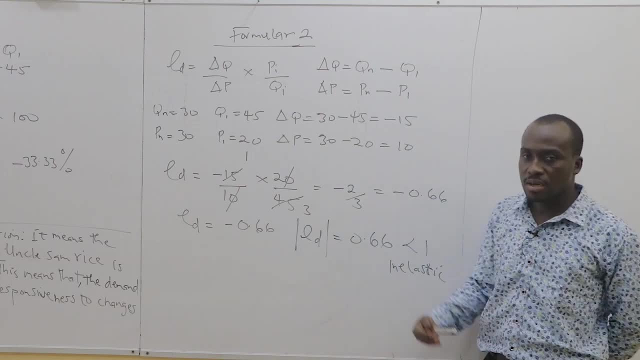 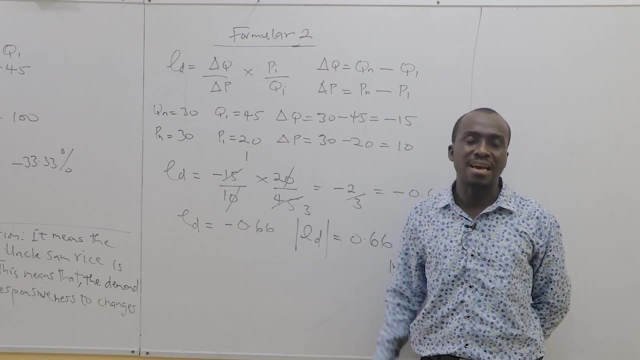 when you get a negative you take the absolute, so you make the answer positive. then you interpret: if it's less than one, it's inelastic, mean that the commodity is slightly responsive to change in price. if it's greater than one, means elastic, but the commodity is very sensitive to change in price. 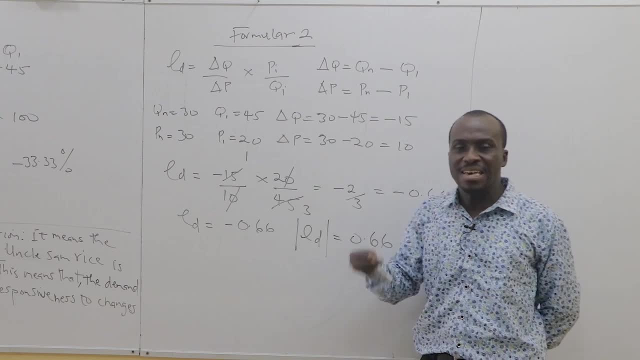 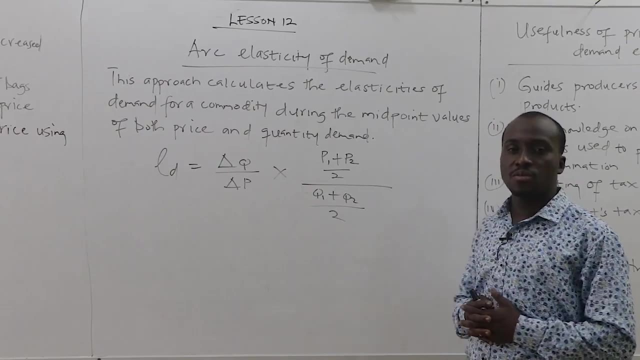 so that's the one we all going to: take the actual system of demand and see how it. also, we work it out with the last act last of the month. how does it work out? so i tell you that, when it comes to electricity, we have the point elasticity approach for estimation. if you have the arc in the arc, like this, what do? 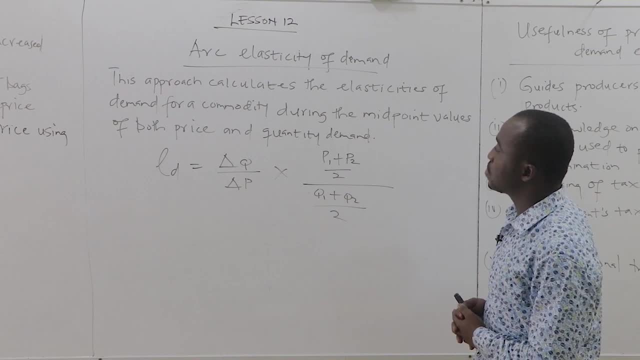 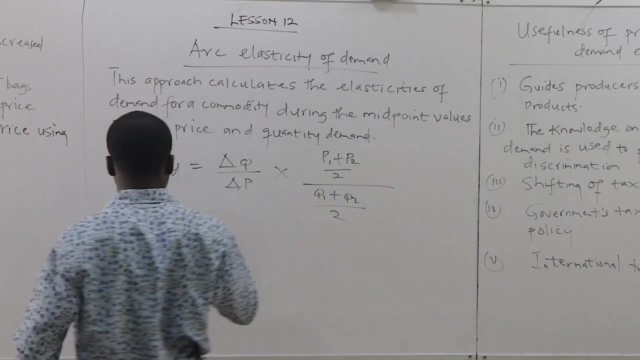 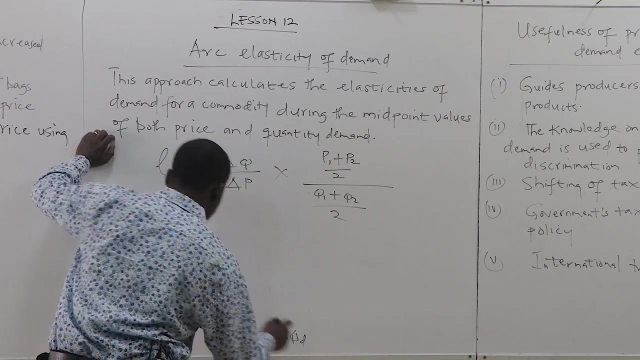 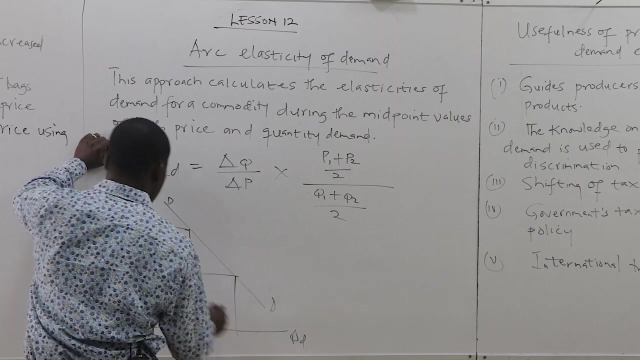 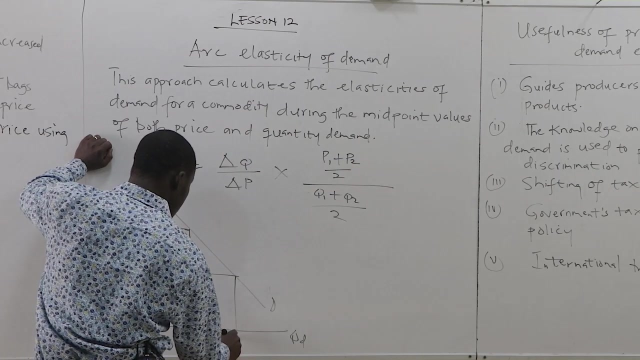 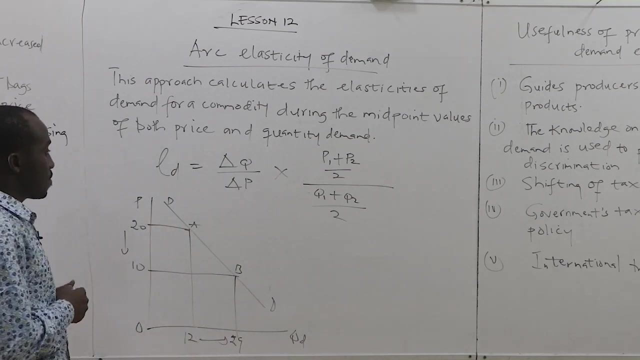 you see this approach: calculate the elasticity of demand for a commodity using the midpoint values of both price and quantity demand. so, for instance, if i have this place for this, for instance, let's get this. let's look at the big point we are talking about. let's tell you we have the product, the price was. 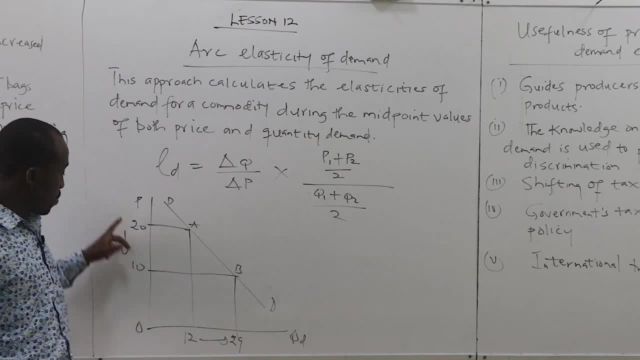 20, the demand was 12.. the price reduced to 10, the demand goes to 29.. so what is the? this is the new, this is the old price. this is a new price. this is the old quantity is a new quantity. so, if you are finding the midpoint, you add this one: 20 plus 20 plus 10, you give you 30, you divide it by 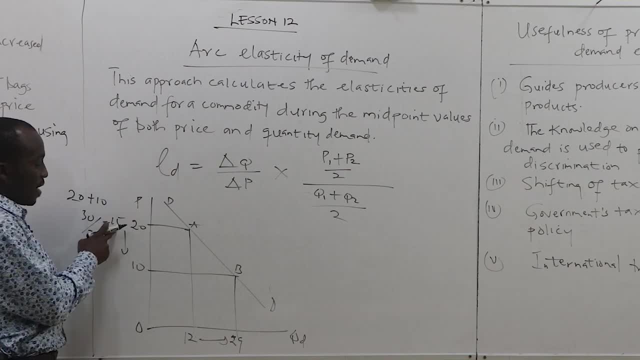 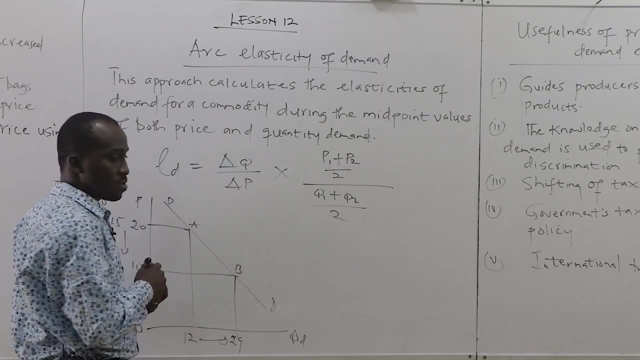 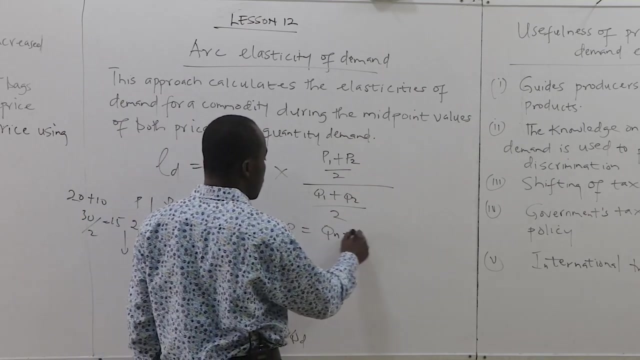 2, you get 15.. so here you use the average to do the estimation. so you see that here is going to be a change in quantity by changing price. what the change in quantity here? the change in quantity, as you know already, it's going to be the new quantity, my initial quantity, the change in price. 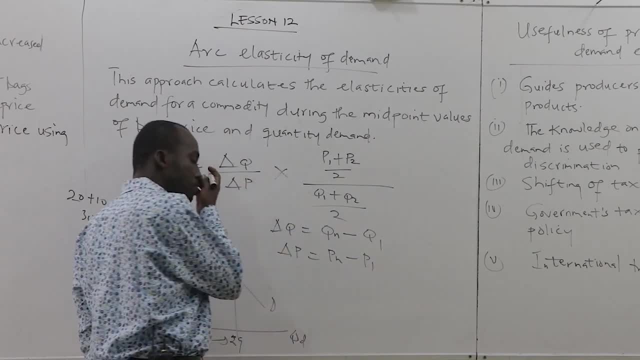 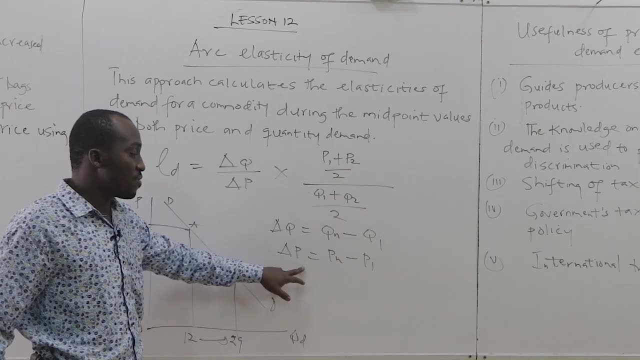 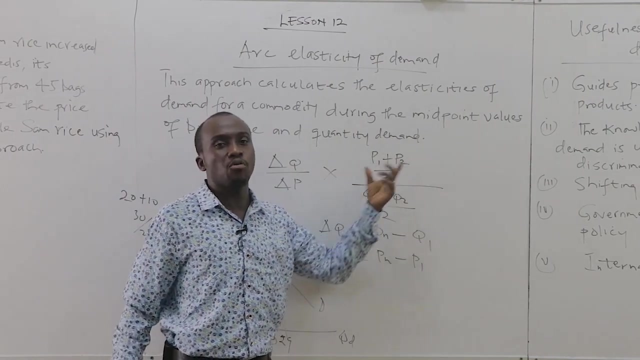 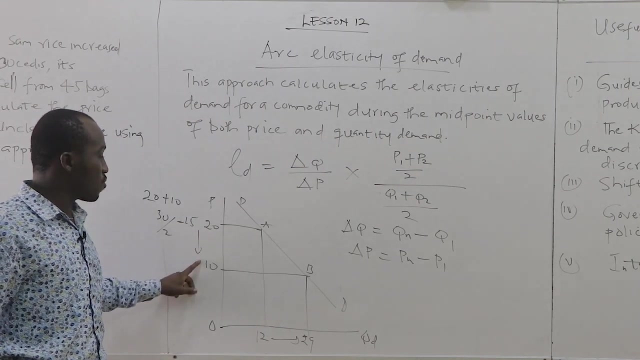 goes to the new price, my initial price. so the change in quantity. we have the new quantity minus initial quantity, the change in price. you have a new price, my initial price. so when you come here, you're going to use the midpoint. why the midpoint? instead of using 30 plus 20, will give you 20 plus 10. sorry, 20 plus 10 will give you. 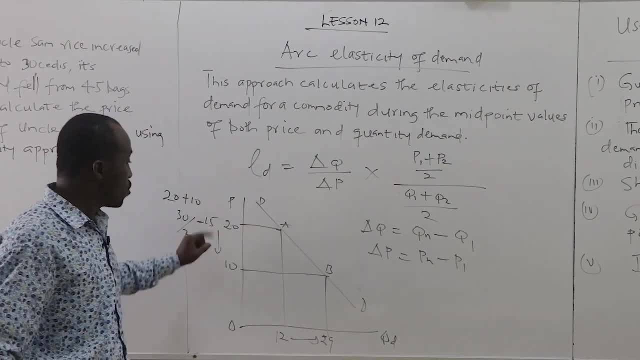 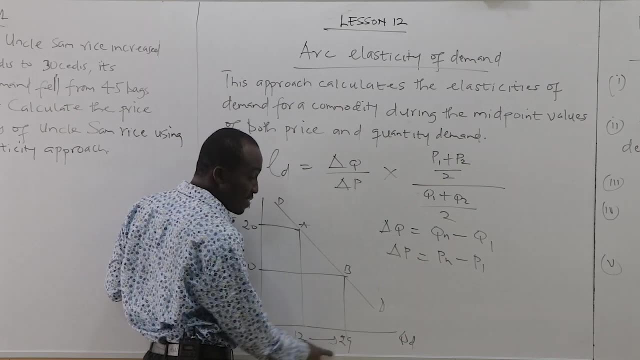 30 divided by 2, so that you don't use only one of the product, you one of the one. you use the midpoint value when it comes to demand to you. we have 12 and 29, so you add 12 and 29 divided by 2, so i use 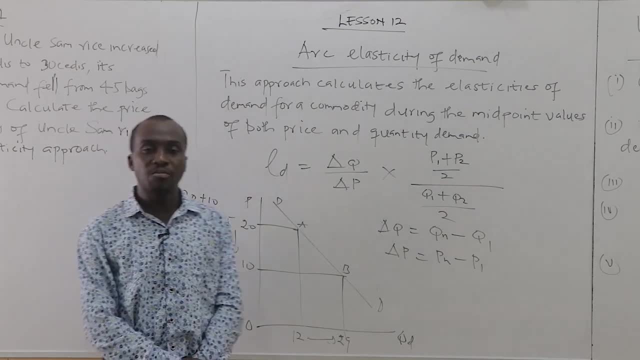 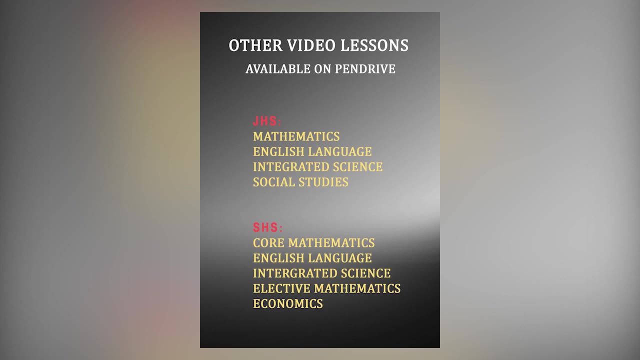 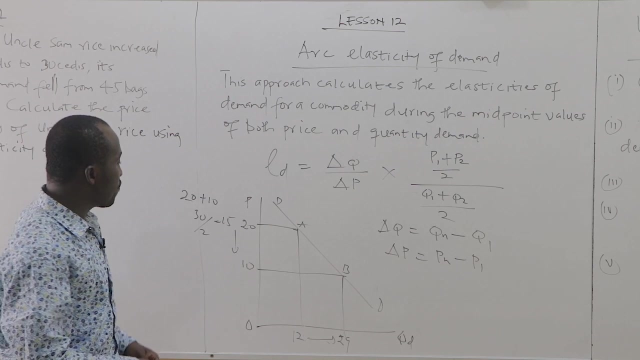 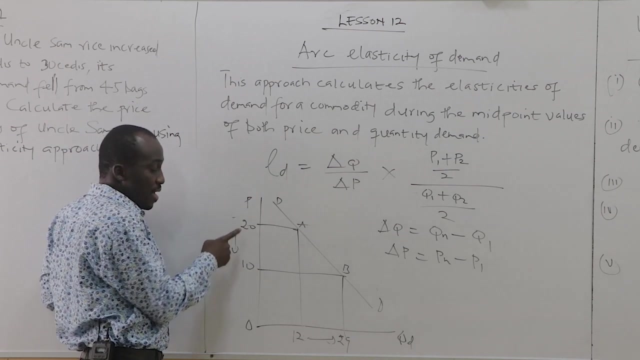 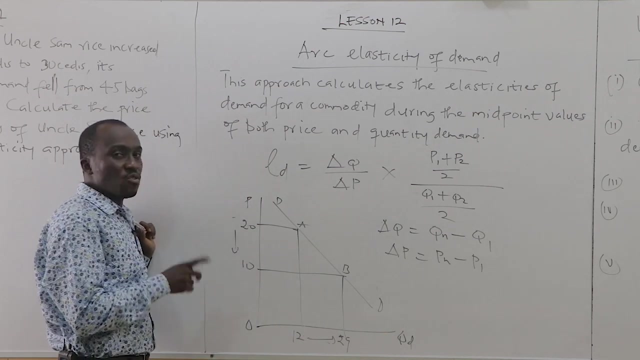 the average. the reason why we use the midpoint is that with the point elasticity, if you change, for instance, if we point elasticity, for instance, if I say that the price was 20, the demand was 12, it degrees to 10, then demand is 29. right, if I use that to calculate the point elasticity, you get a. 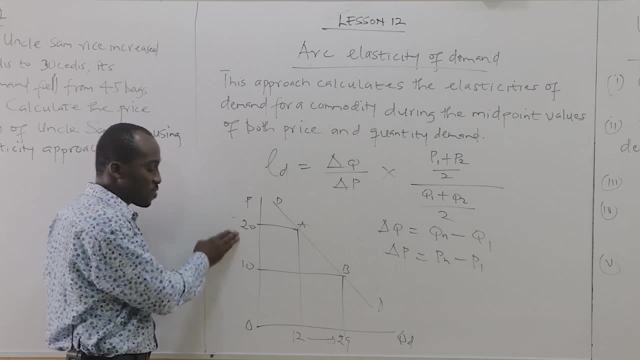 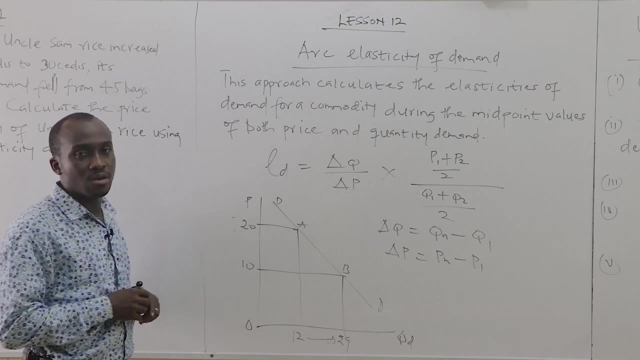 different answer. but when I turn it up and say that the price was 10 and increase to 20 and the demand also reduced from 29 to 12, when you start to estimate you get a different answer. so people didn't like the idea of the. 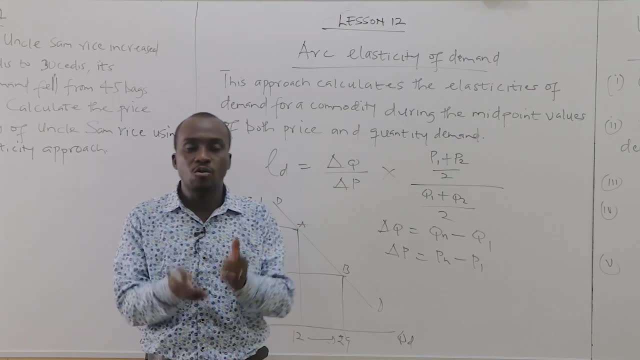 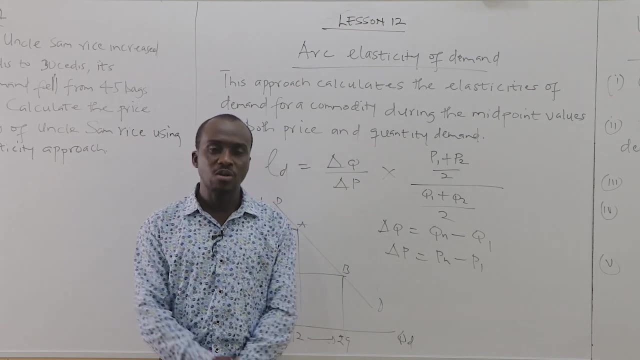 pointless. if you change the figures and you bring one become new, one becomes old. and then the other instance you change, one become new, one got older. used to estimate it. you get different answers. so they saw that the midpoint to solve that problem, because it'll give you one. 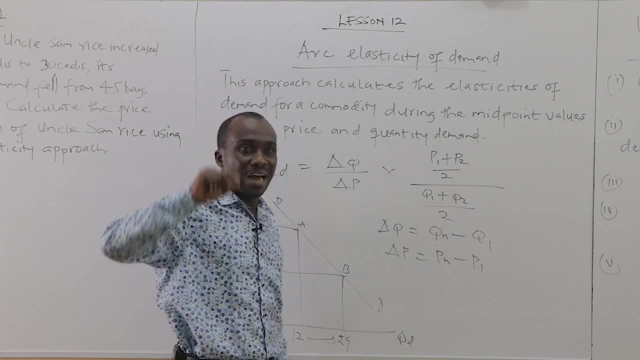 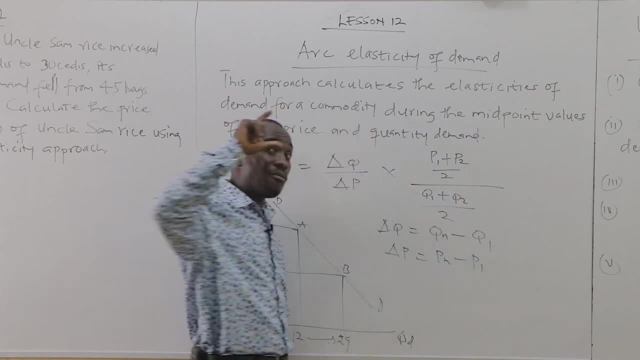 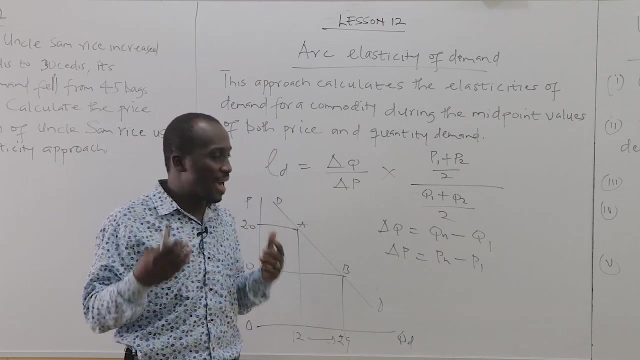 value for the two prices so that I don't get a midpoint, so that you don't get different values when you change the figures in the same way here, to give you one value for the quantity, one quantity, so I don't get different values. that was the idea by most exams. the pointless is what they use. our glasses highly use. 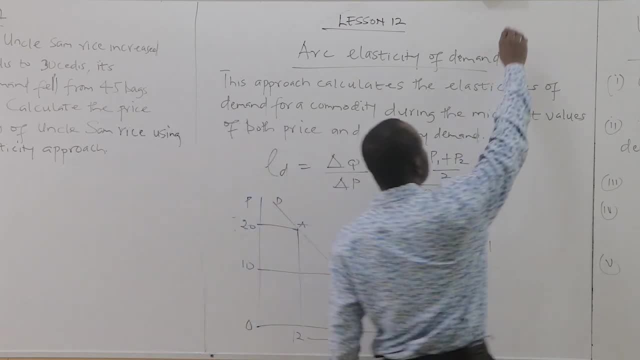 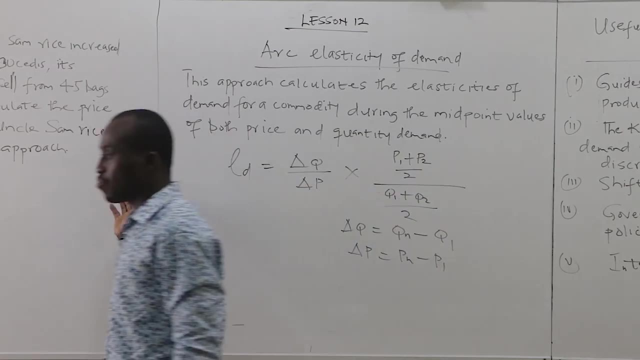 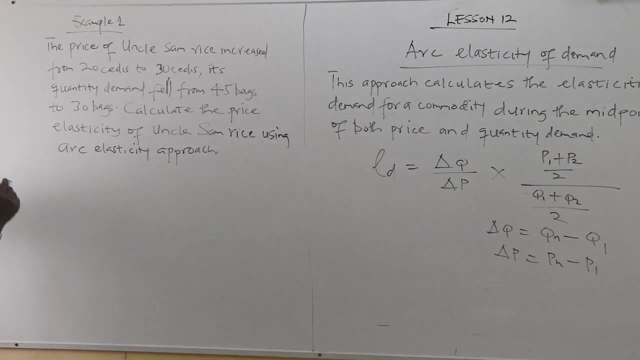 unless the questions specify here, what do you see? so let's come here, let's use this example, the same example we use. they're not gonna use the pointless distance to see how a slime is going to be, what we do already that. let me go over example one: the price, of uncle, some rice. 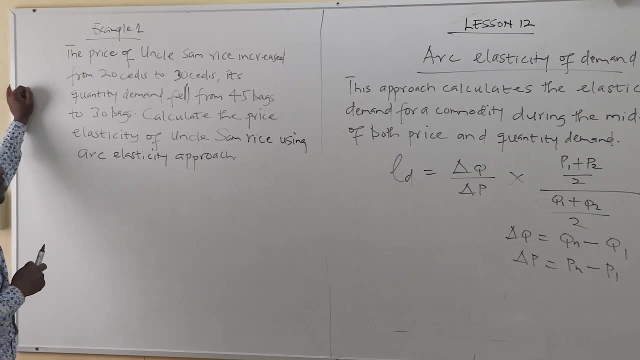 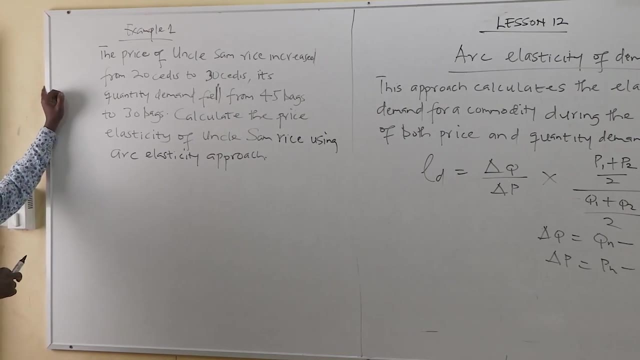 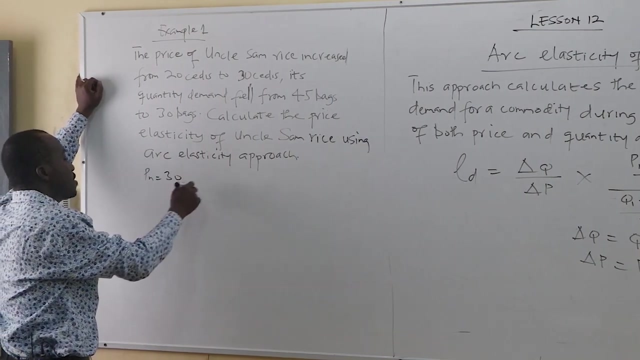 increased from 20 cities, study cities, the quantity demand from 45 bucks 30 bucks. calculate the price of the price of the chocolate, the same rice, using the ARC elasticity approach. so right now we have here, we know that a new price is 30, the initial price is 20, while the 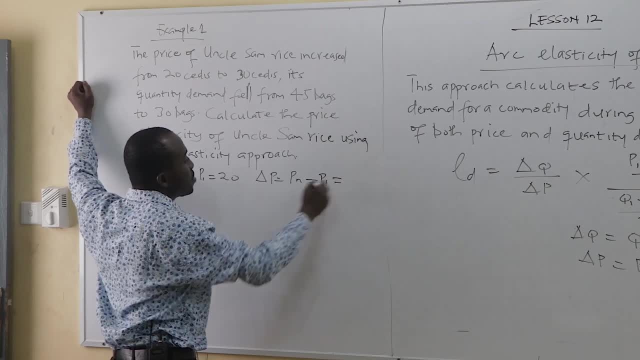 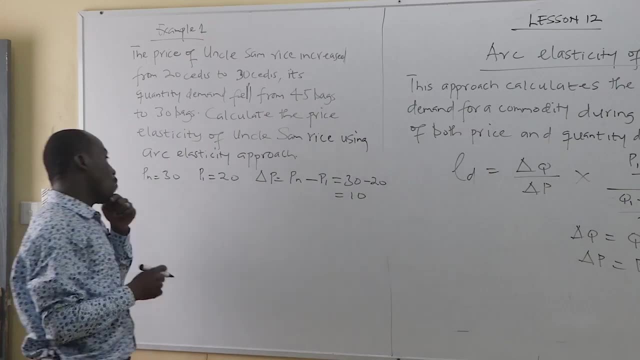 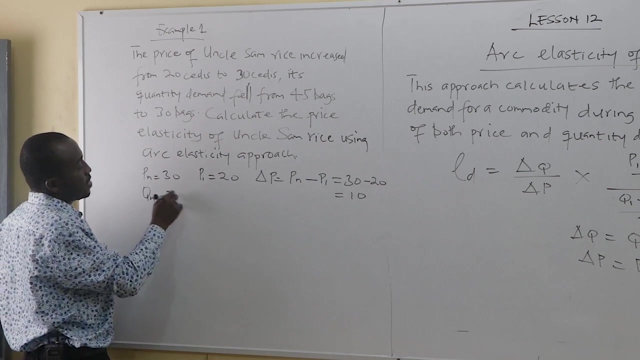 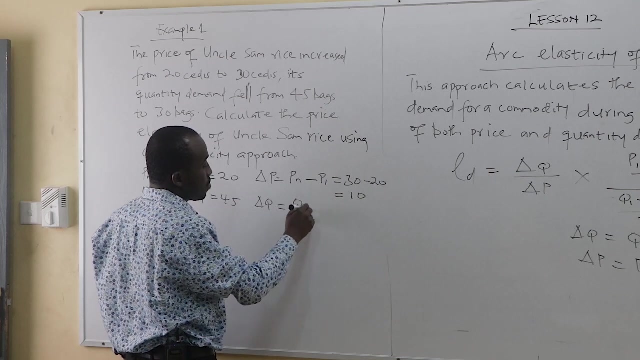 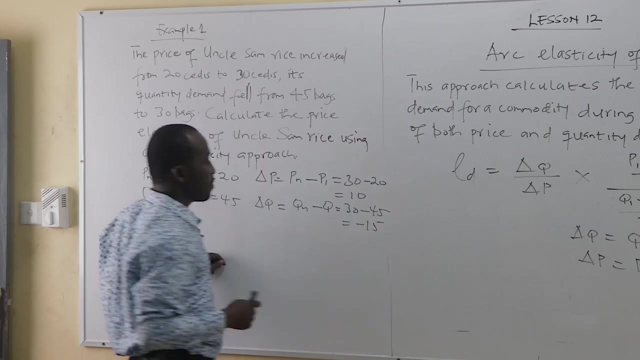 changing price: the new price minus initial price, which is equal to 30 times 20, that gives you 10. what about the new quantity? the new quantity is what 30, the initial quantity is what 45. therefore, the changing quantity is the new quantity minus initial quantity, which is what 30 minus 45, which gives you negative 15. so 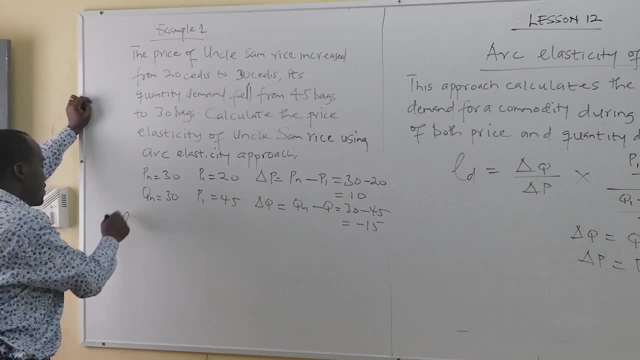 let's use that for the. let's put that into the formula. the formula says: the change over days gives you the new quantity, which is what? negative 15 plus initial price, which is what the changing price? the changing quantity is negative 15. what the changing price? the change quantity is negative 15. the. 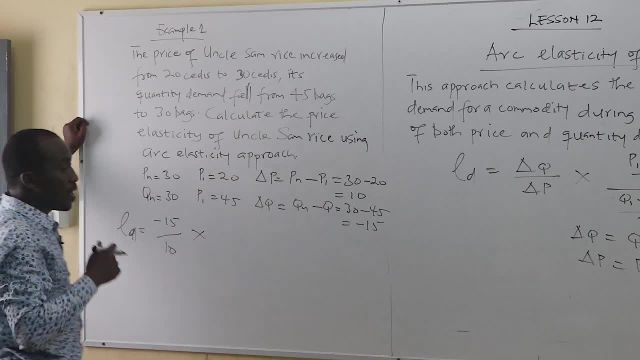 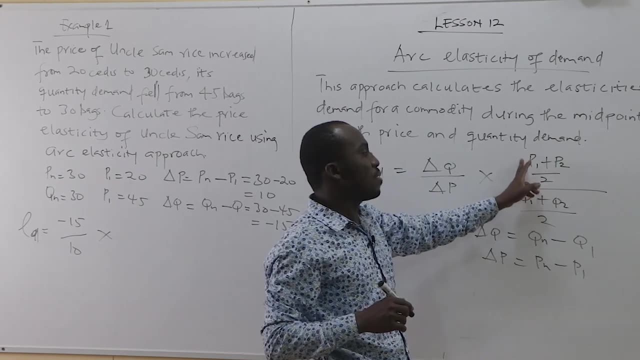 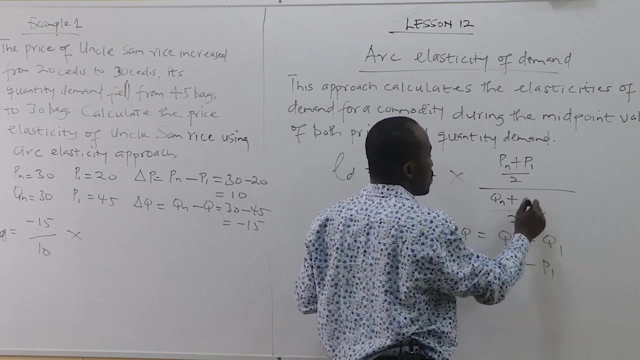 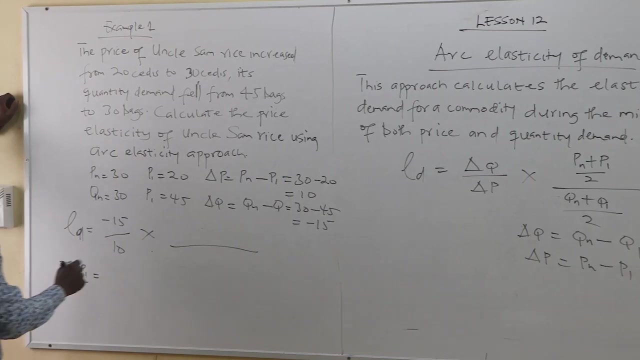 changing price over days 10. when you come here, instead of using the initial price, like what we're doing in the pointless, they're going to use both the price, the new price, the new price and initial price and you find the average, right, the two, instead of using the initials. n plus 1 divided by 2, that is 30. 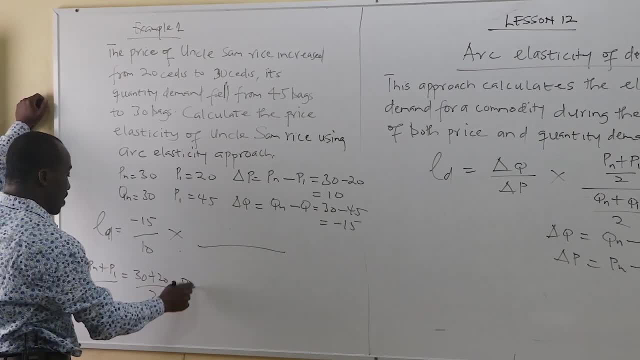 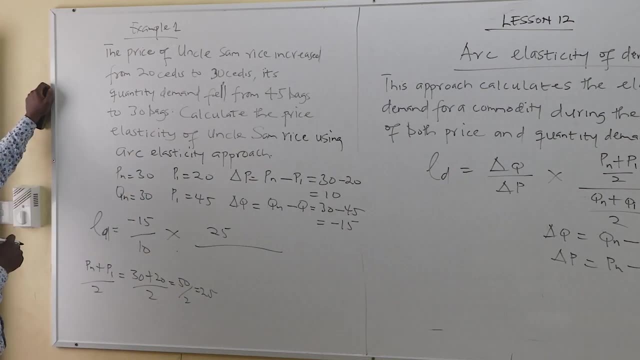 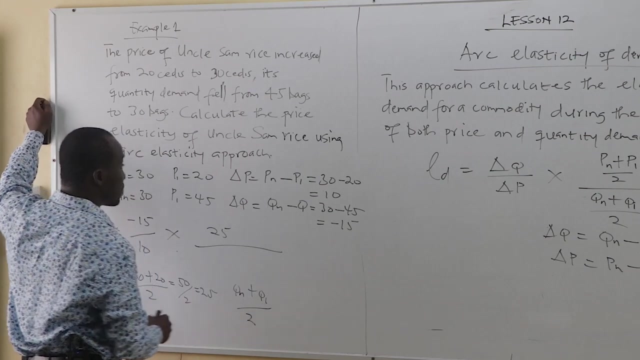 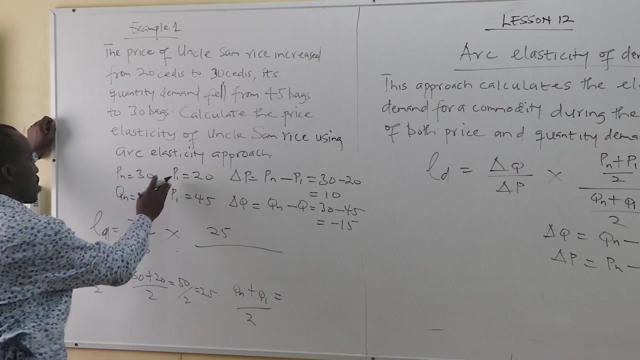 plus 20 plus 20 divided by 2 gives you what 50 divided by 2 gives you what 25, whatever that probably man que see las que 1 divided by 2, again, that gives you, that gives you for you, that's Katy, plus 45 words, 15 times 0.25, thirty percent minus 50, hvis you update to 23. 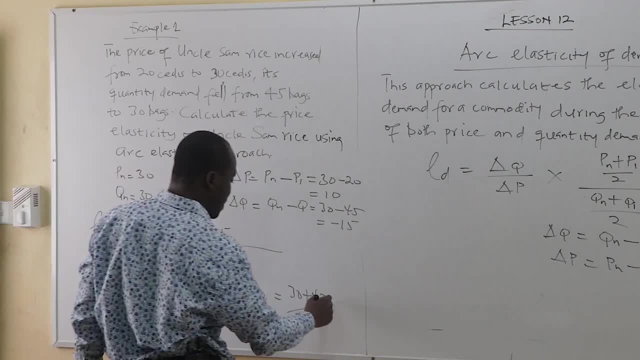 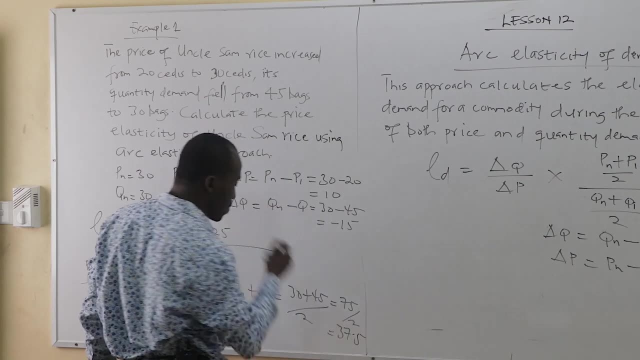 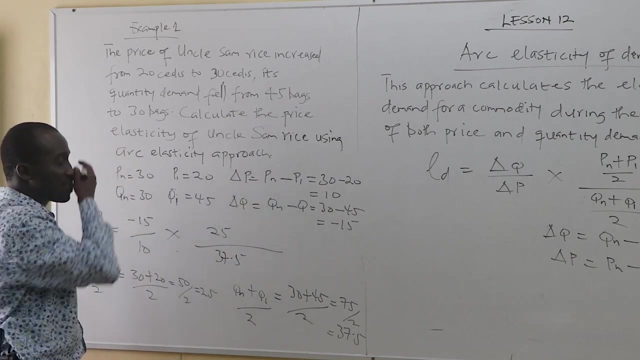 divided by 2, that's 75 divided by 2, and then you're going to get something like 37.5, right? So when you come here, this will give you 37.5.. I think my guess is true. So it means that. 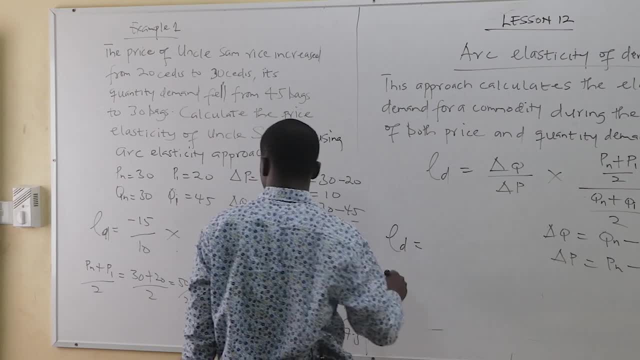 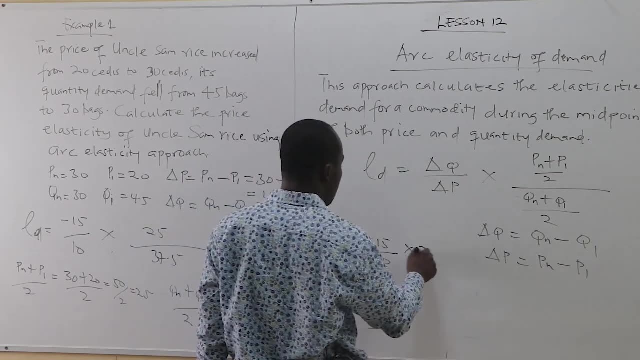 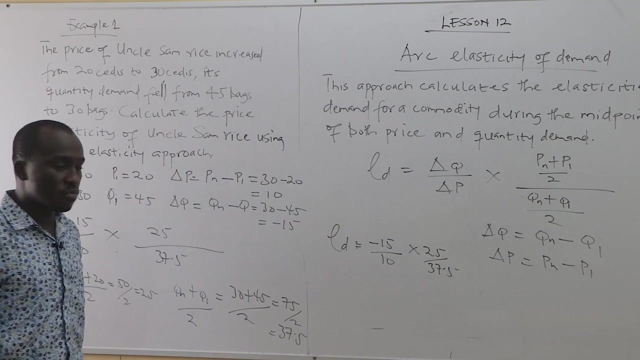 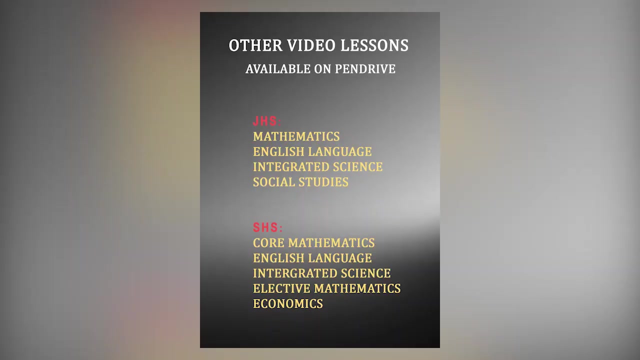 the elasticity can be rewritten here as negative: 15 over 10 times 25 divided by 37.5,. right, You can punch the top, multiply the top, multiply the down and give it a. So when you multiply the top, you're going to get something like: 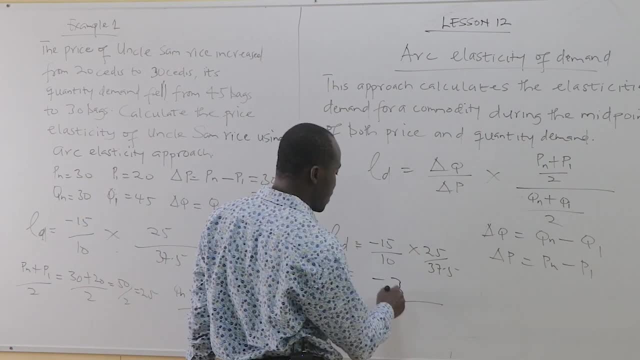 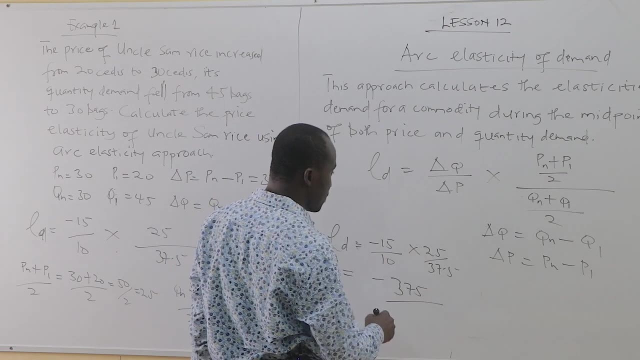 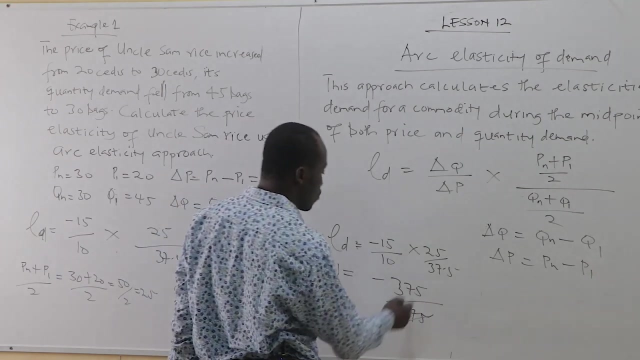 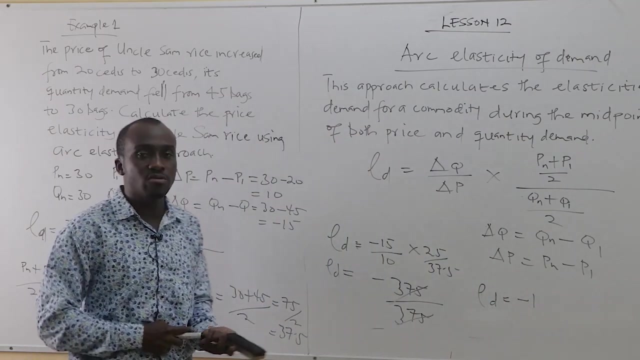 negative 37,, negative 375, and the top one gives you negative 375, and the down one gives you positive 375.. So when you divide, you're going to get elasticity which is equal to negative 1.. So you see that the elasticity you are getting, elasticity negative. 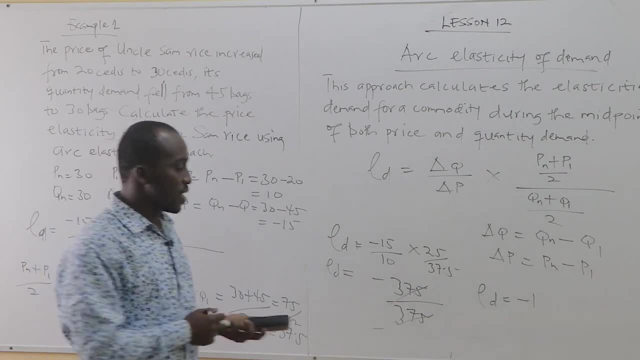 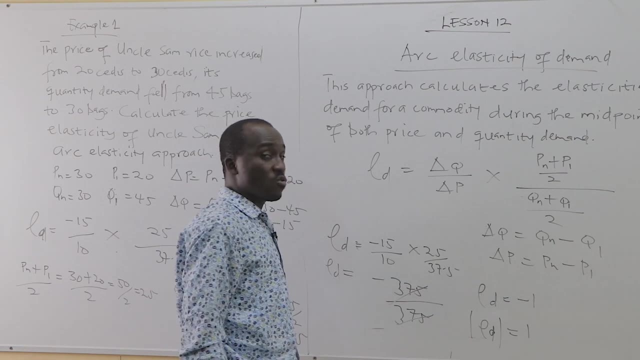 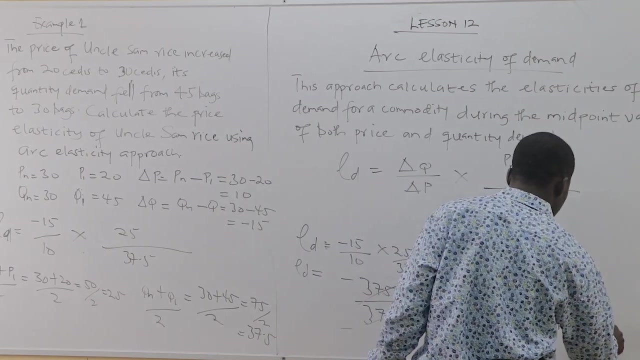 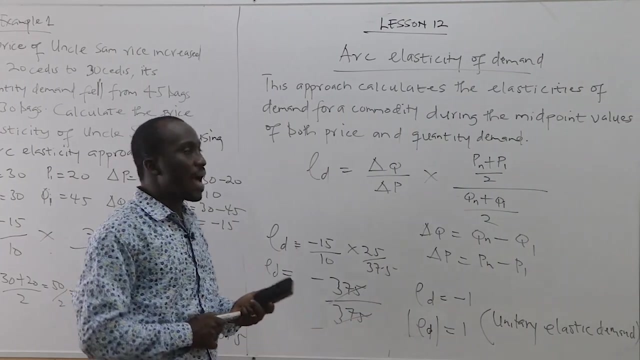 So, when you take the absolute, you're going to get elasticity which is going to be 1.. When elasticity is equal to 1, you're going to get elasticity which is going to be 1.. So you see that when we use the arc elasticity, 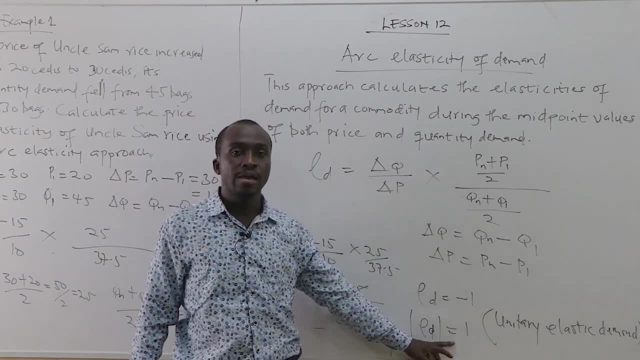 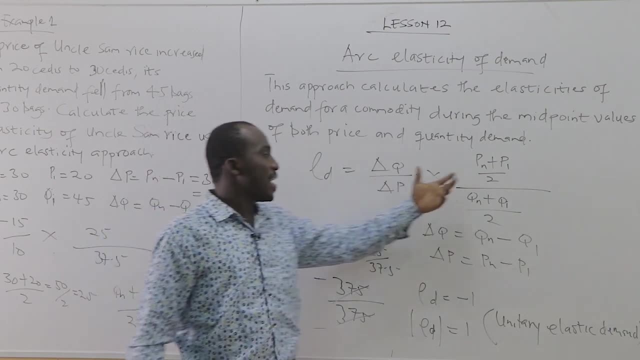 the answer we are getting here is different from when we use the point elasticity. Here we got the answer 1.. The point elasticity: we got 0.66.. Why? Because here we use the midpoint, We use the average of the two prices. 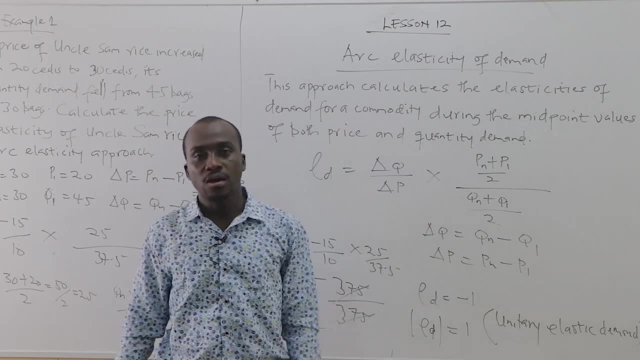 Here we use the average of the two prices. Here we use the average of the two prices. That's why we are getting different answer. That's why I'm telling you that if in Waseda the question doesn't specify, 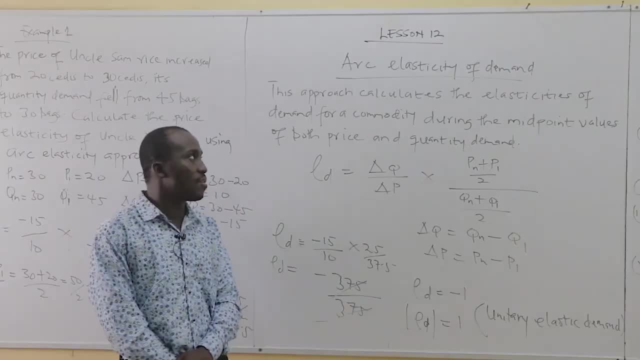 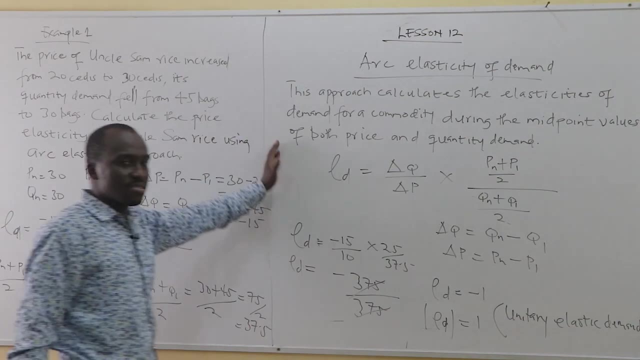 just use the point elasticity. That's the most ideal case. So you have seen, you are able to estimate the same question using the point elasticity and also using the arc elasticity where the midpoint comes in. I think, before we take, before we move from the price elasticity, 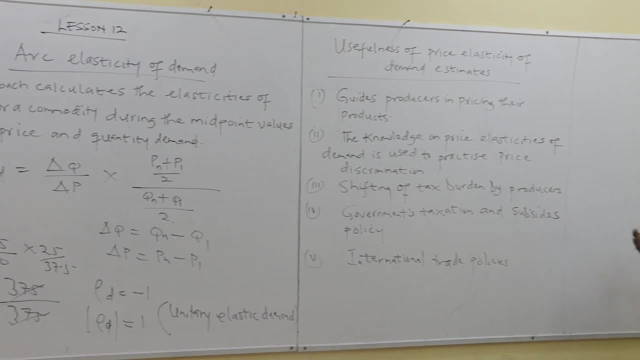 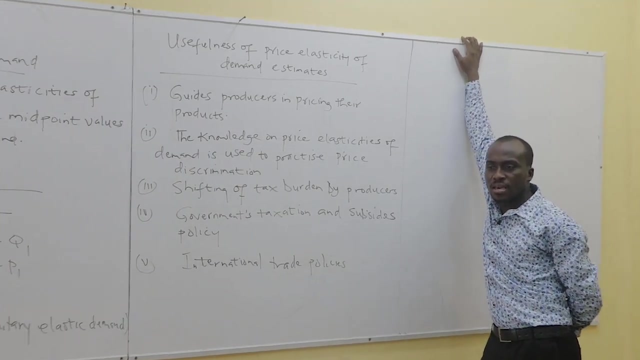 to the income elasticity we want to look at. what is the relevance of knowing the price elasticity? What is the price elasticity of a commodity? And I told you that most of the commodities we buy on the market are either elastic or inelastic. Why is it relevant for you to know? 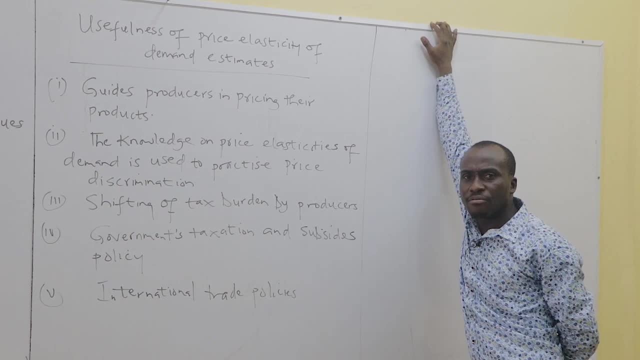 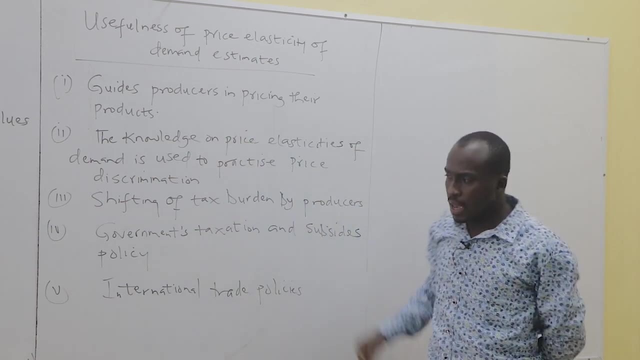 Not only for the exams, also for your everyday life. If you're a producer, what does it mean to you? Number one: it guides producers in pricing their product. If now, after school, you finish school and you want to start a business, and you find out, 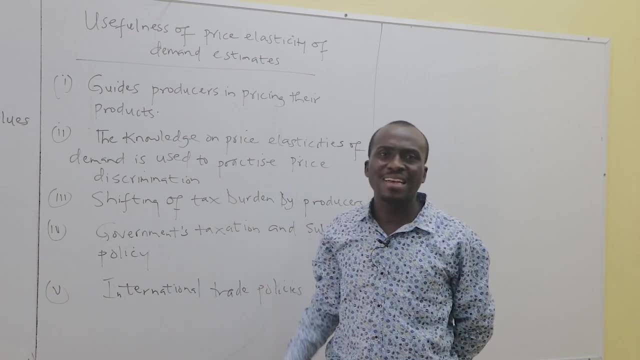 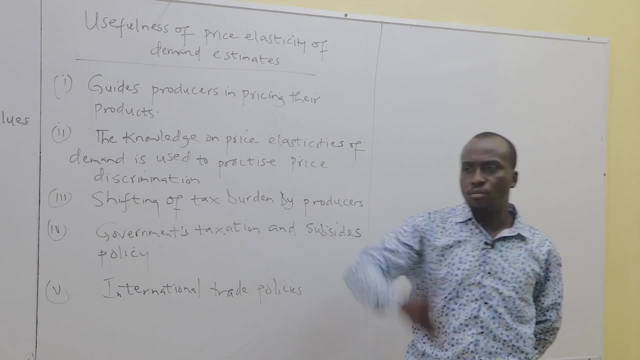 that the product you're selling. it has inelastic demand. That means when you're increasing the price you're not afraid because only a few people stop buying. A lot of people will buy and make your profit and you go away. But if you detect that the commodity you are selling 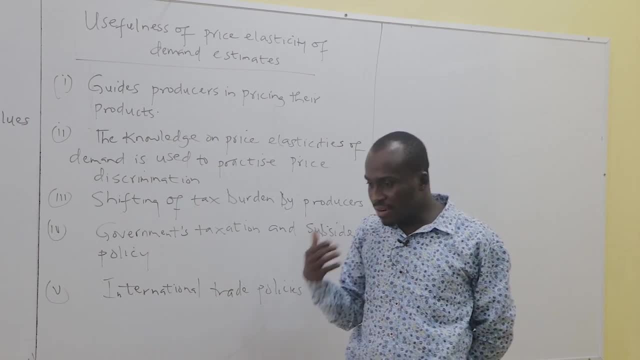 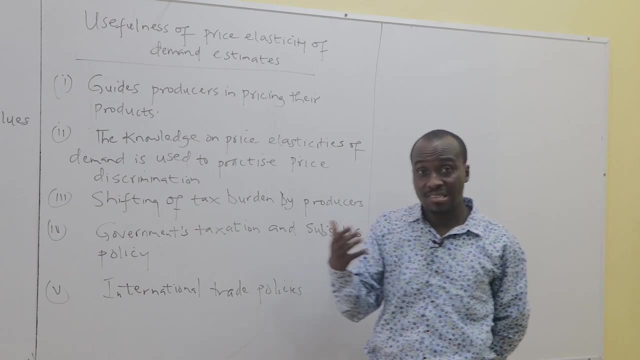 has elastic demand, then you have to be very careful that if I increase the price marginally, a lot of people will stop buying and I'll lose right, Especially when your commodities are substitutes or they are luxury. So if you're a producer, it gives you a very good idea. 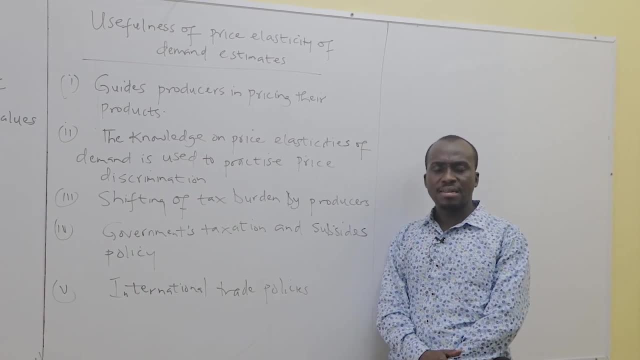 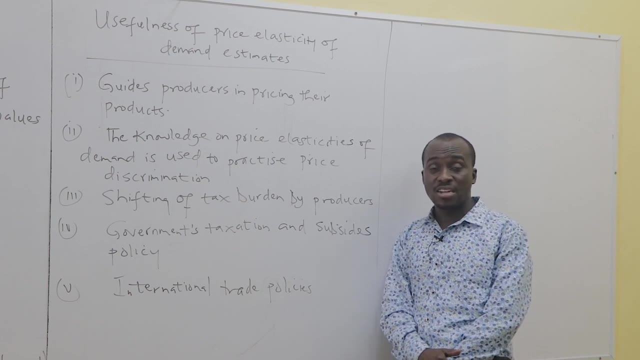 how to price your product. So companies like Toyota, Nissan, Samsung, BYD, all these companies back in Europe, all these things, they take all these things into cognizance, Whether their product is elastic or inelastic before the price. 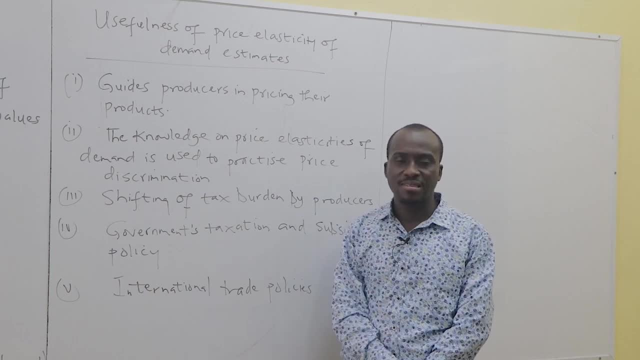 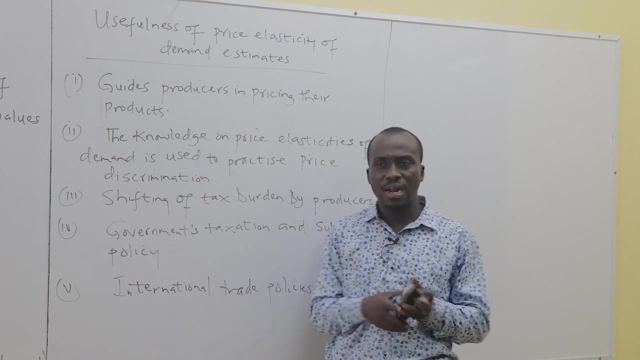 Those who sell in the market: Makola, Akomishi, Kajitsiya, Kantamanto, Kotrokraba Market, all these people, they take some of these things into account and you have to know whether their product is elastic. So they are very careful in pricing. If it's elastic, if the price goes up marginally, I'm going to lose a lot of customers. They're not going to buy my product again. If it's inelastic, if I increase the price marginally. 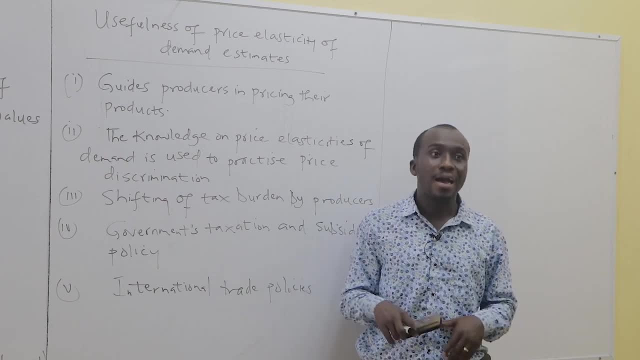 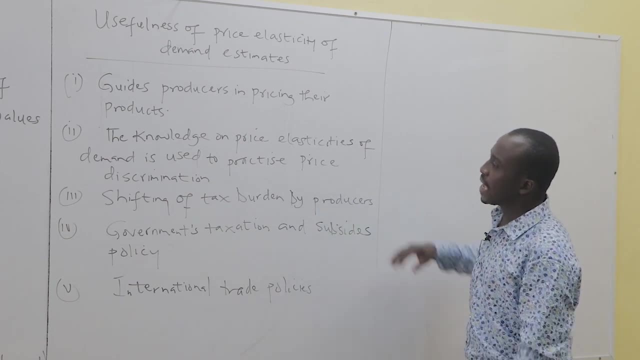 or if I increase the price, only a few people stop buying and I'll make my profit and go away. So these are very important, not only for the WASI, also for your everyday life: The knowledge on price and life of demand. 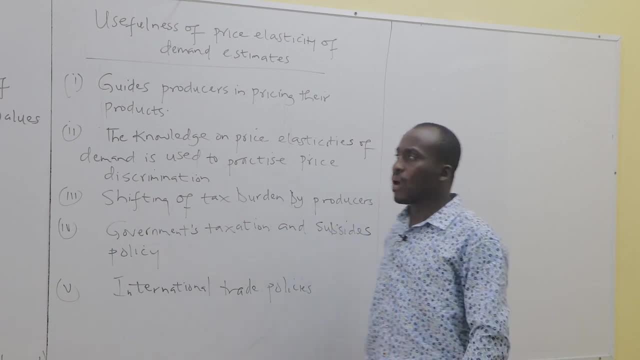 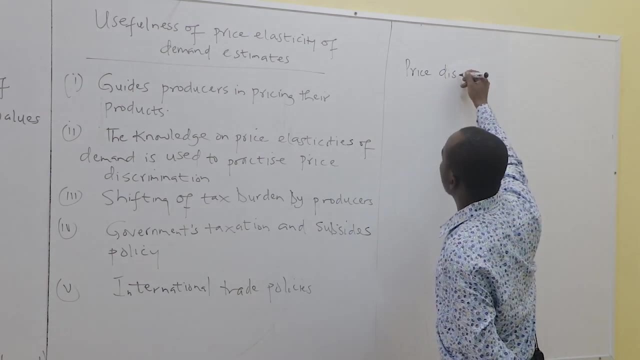 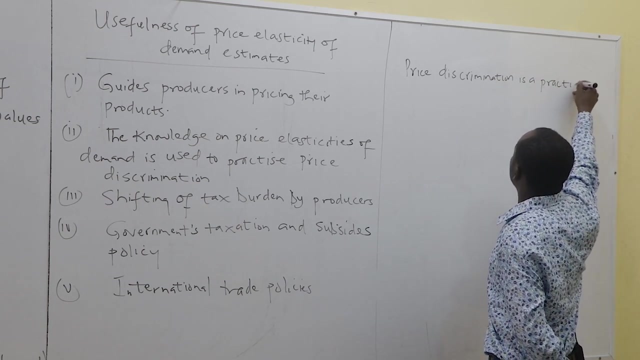 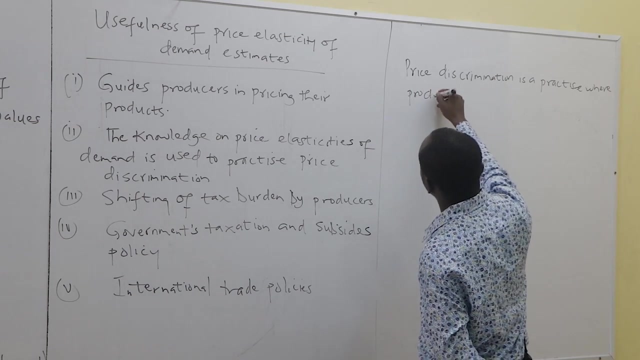 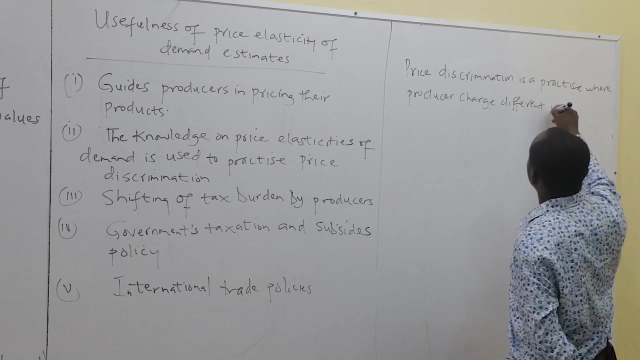 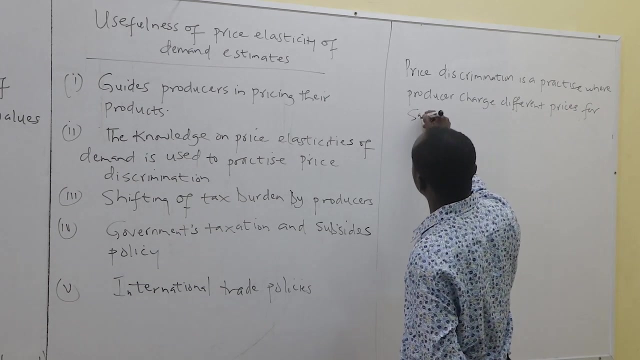 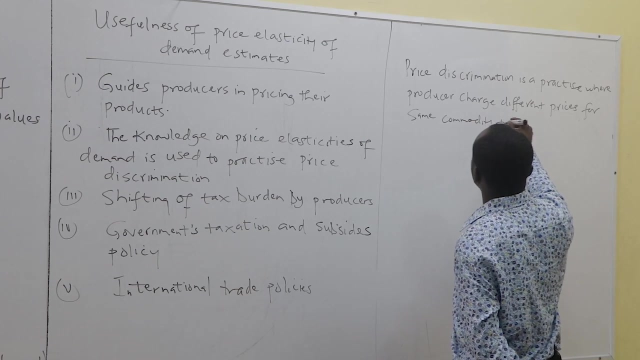 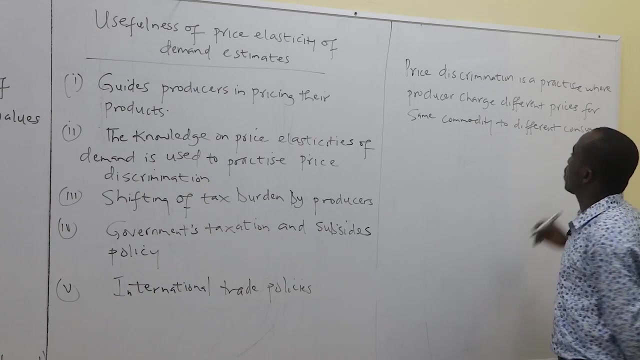 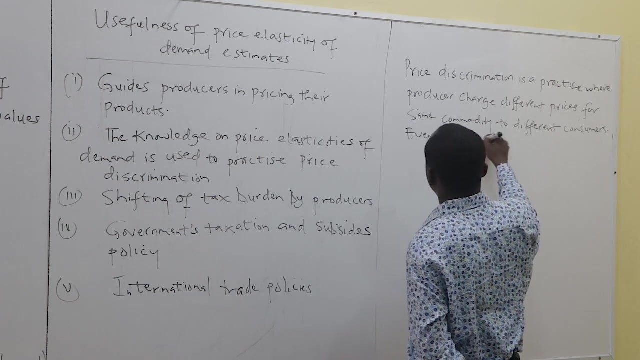 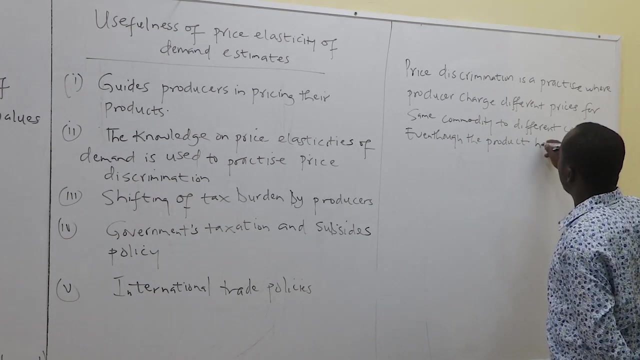 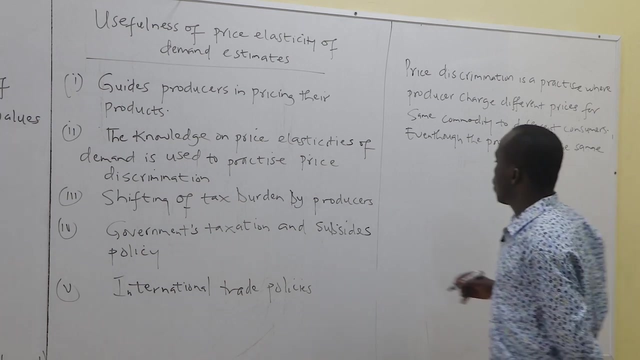 is used for price discrimination. What is price discrimination? Price discrimination is a practice where producers charge different prices for the same commodity, for the same commodity, to different consumers, Even though the product has the same, has the same cost, the same cost of production. The price discrimination is a practice where producers charge different prices for the same commodities, different consumers, even though the product has the same. the product has the same cost of production. what do you see with prior discrimination? the producer said: i produce. 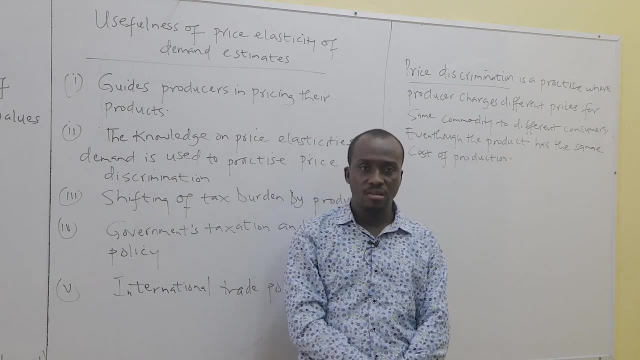 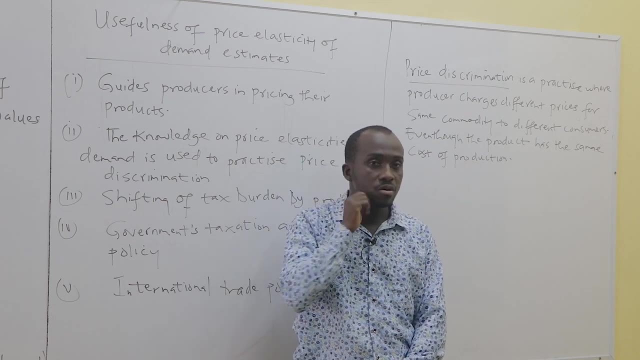 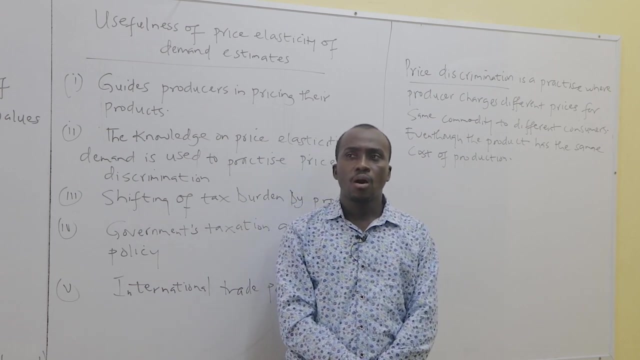 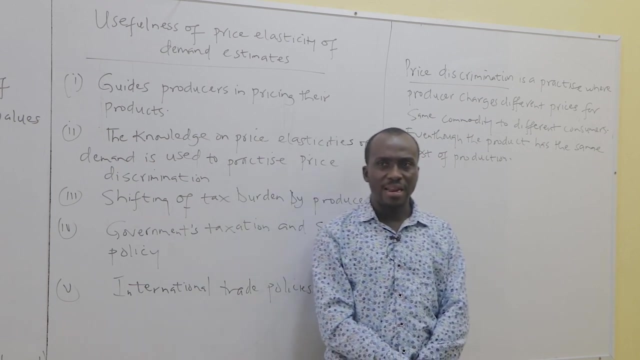 something that the producer charges different price for different consumers, even though the goods is produced at the same height, it's produced the same at the same cost. for instance, maybe i'm producing, maybe cars- right, i've seen that, the cars. if i take you to places where rich men are, 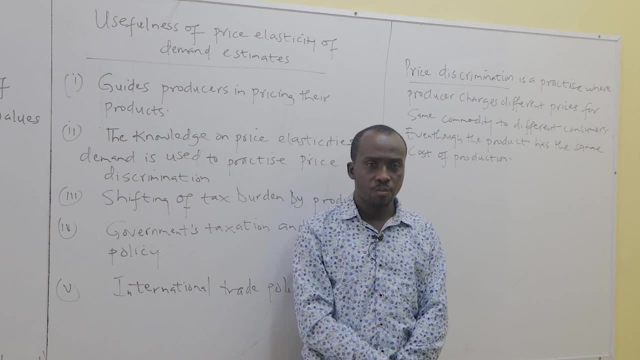 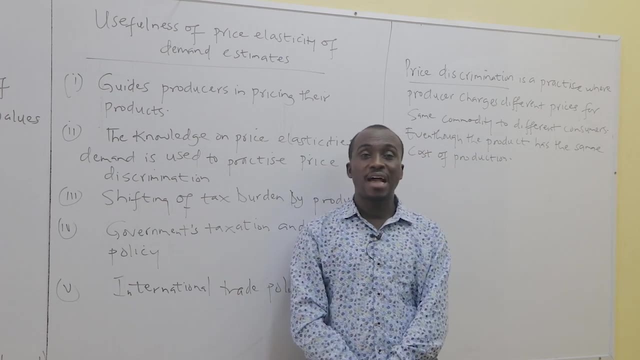 i'll tell you. if it's hundred thousand dollars, i'll tell them 150 thousand dollars. but when i take it to a different country where the people there are not rich, you're not that worthy, i would charge eight, maybe eighty thousand dollars. why? maybe they have different. 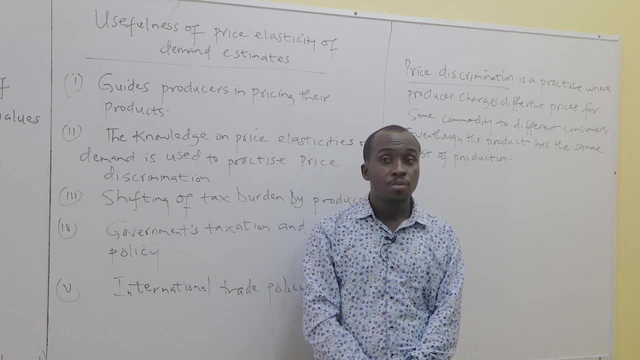 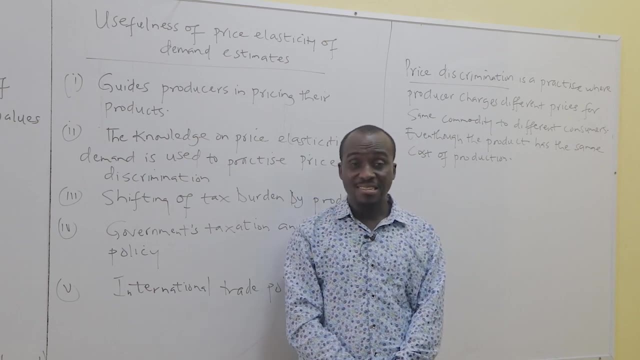 last, and that rich environment when you go. even if the price is too high, what they are ready to, still buy it because their elasticity is inelastic. if the elasticity in elastic the same product, i'll take it to different places and sell to them at different price, because maybe these people 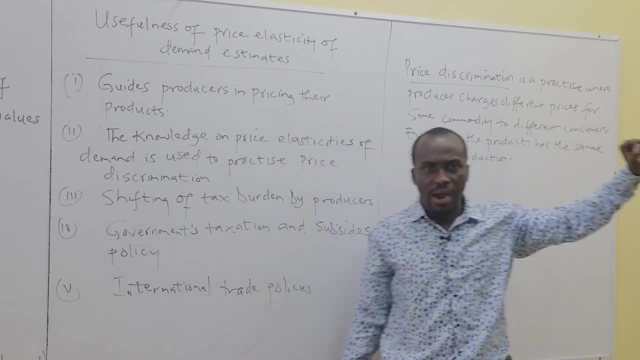 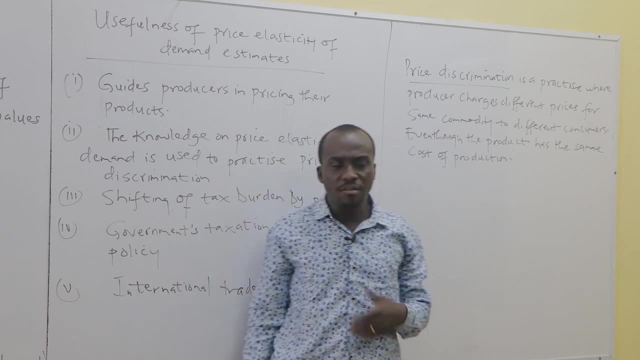 their demand for my product is elastic. if i go and increase the price that they will stop buying it. but if i go and give it to different consumers in different locations, their demand might be in elastic for my product and therefore if i increase the price they'll still be buying. so if the producer 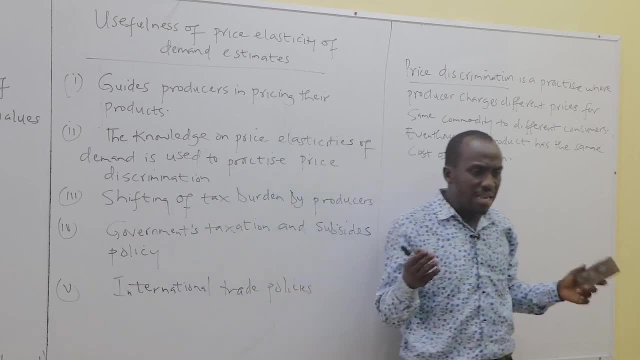 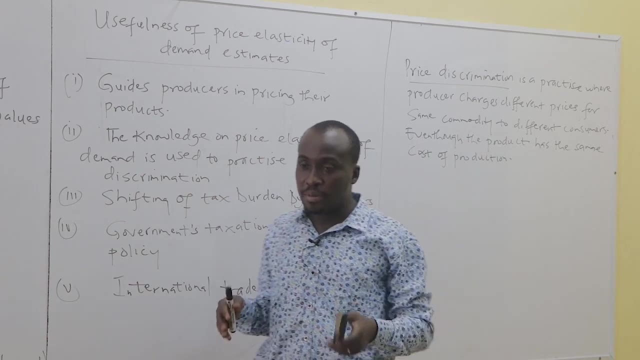 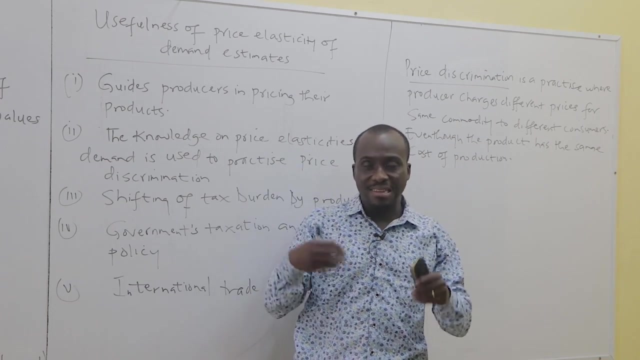 is able to phantom that these consumers maybe they're maybe going to take consumers in different countries. if you're able to phantom that- consumers in different countries, different environment- this will have elastic demand for my product. this will have inelastic- you can do prior discrimination. those that have inelastic demand, you can charge them a higher price and those are those that have. 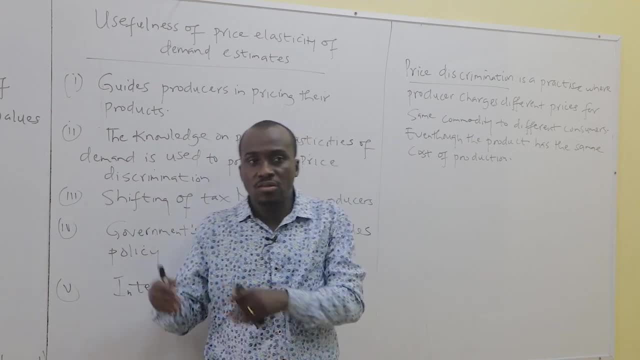 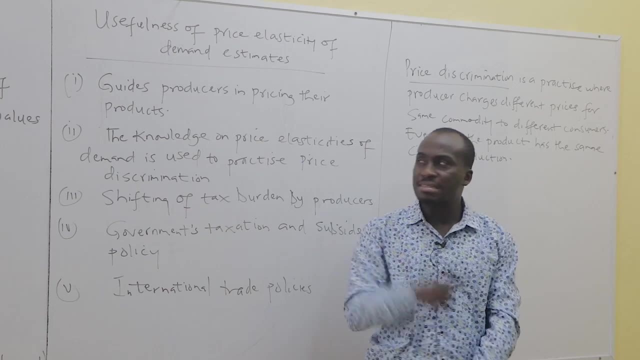 inelastic demand, you decide to charge them a higher price. and those that have elastic demand, you will charge them a lower price. so that he takes, he makes more profits, he takes advantage of the elasticity, different logistics for their product- this would be a demand that's in the elastic. i'll discriminate. 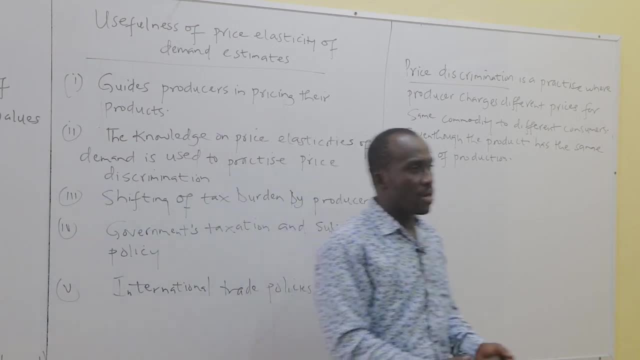 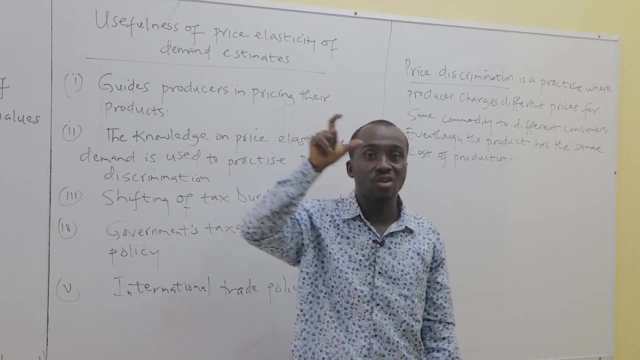 outside the higher price. so this would be a demand, for my product is in the elastic, so i charge him a lower price. at the end of the day he makes more profit because the product was still produced at the same cost. it wasn't produced at different costs, was produced at the same cost. 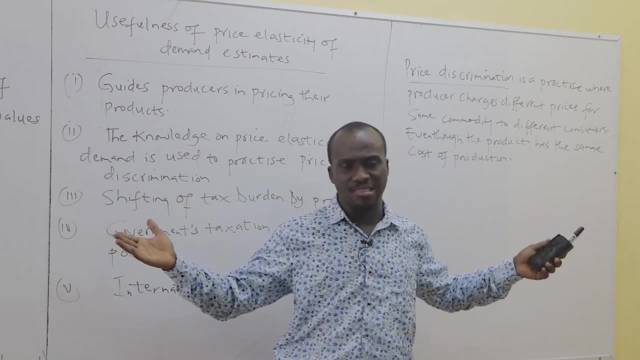 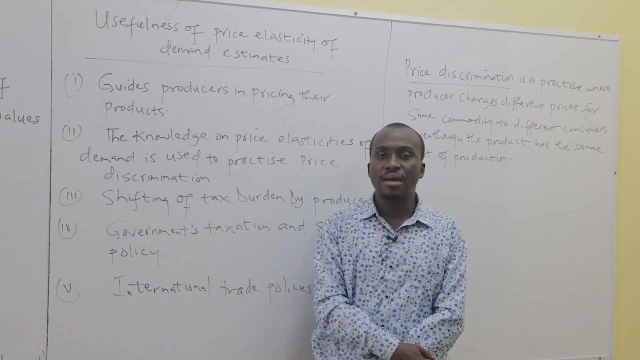 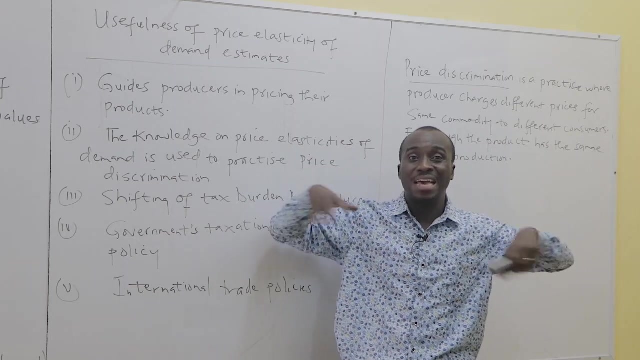 by charging different consumers different price because they have different elasticities, and this is done day in, day out in the market. somebody can be in china or somebody can be in america, produce something and sell to different consumers at different price in different parts of africa, based on the elasticity of their demand. so the concept is very important for producers. 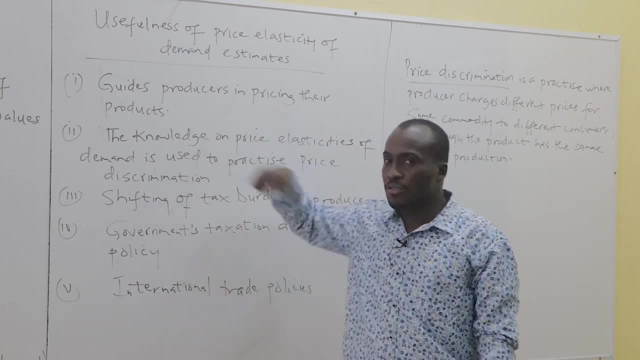 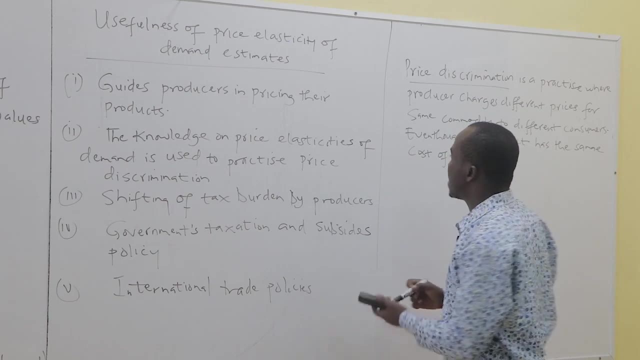 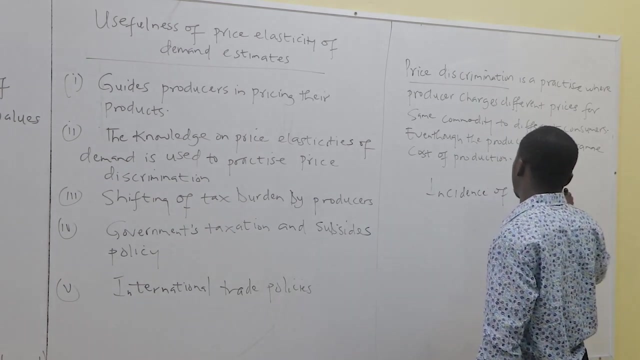 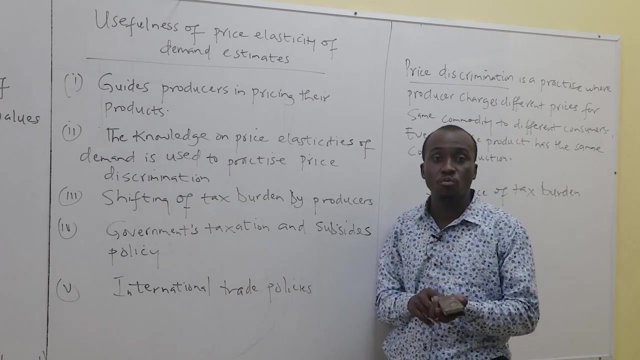 if you want to practice price discrimination, it's also good for producer. if you want to, they want to price their product. also, when it comes to shifting of tax burden- what they call the incidence of incidence of tax- the incidence of tax burden, that is, the ability of producers to shift their taxes to consumers. if government tax me, cannot shift it to consumer. if government impose a tax, maybe every product i sell government sell to me. if i produce a product ten dollars, government impose a tax on maybe four cities, four dollars, right, i produce a product as ten dollars, can i impose a tax of four dollars? can i shift all these four dollars to my consumers so that they will pay thirteen dollars for the product, so that i shift all what i call incidence of taxation, the ability to shift your taxes to your consumers, whether the producer can shift all these taxes to your consumers or can. shift depends whether the consumers demand is elastic or in elastic. if your demand is in elastic, can shift all to them and they still buy the product and it's okay if their demand is in elastic. if their demand is elastic, if your demand is elastic, that means you cannot shift all to them. 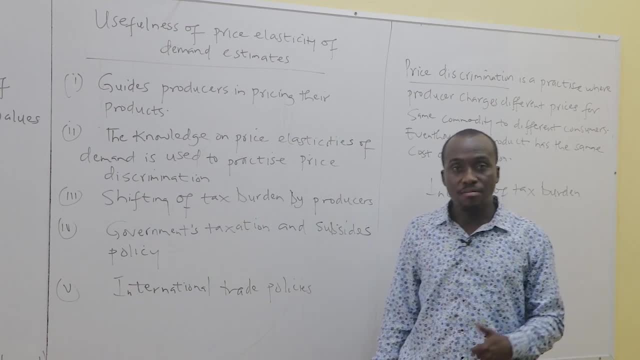 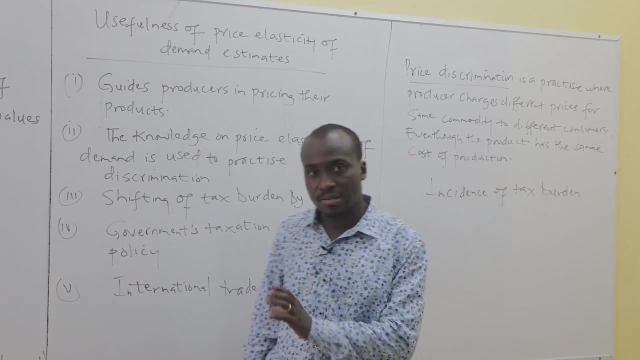 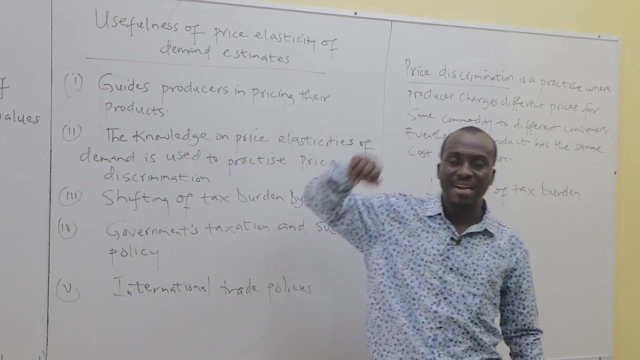 if you should more and the price increase once the demand is elastic, they will cut down their demand and that will affect this business. so the magnitude of the tax you can shift the consumers determines whether it depends whether the people their demand for that price is elastic or inelastic. if you take that their demands inelastic and shift more taxes to them and they 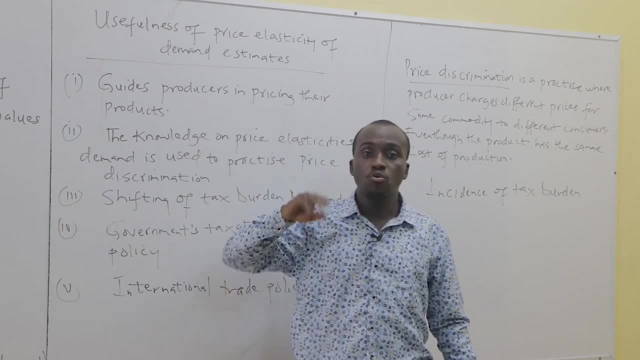 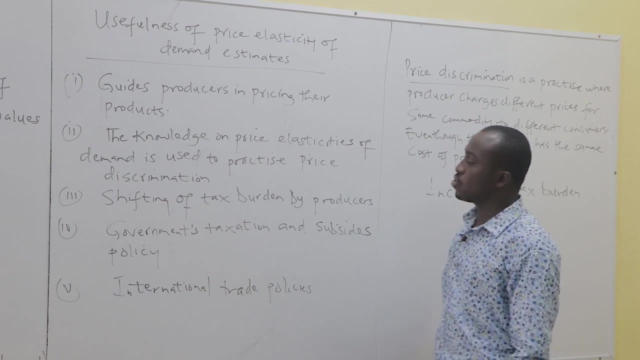 still buy it. if you take that the demand is elastic, you will see small amount of the tax, so you might not even shift it. so the price is very low and keep on making his money. so it's good also for producers when it comes to deciding whether to shift their tax burden to for the consumers or not. 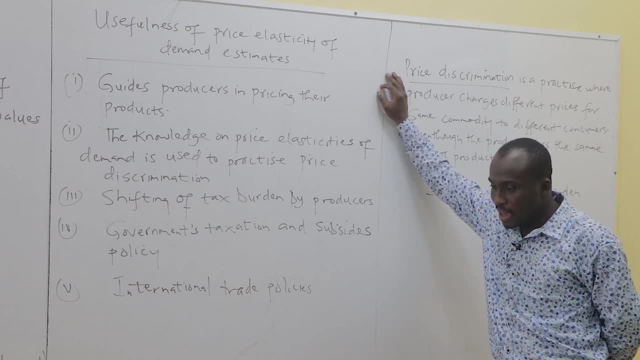 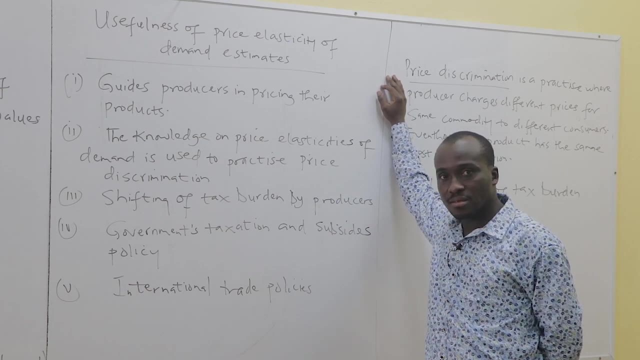 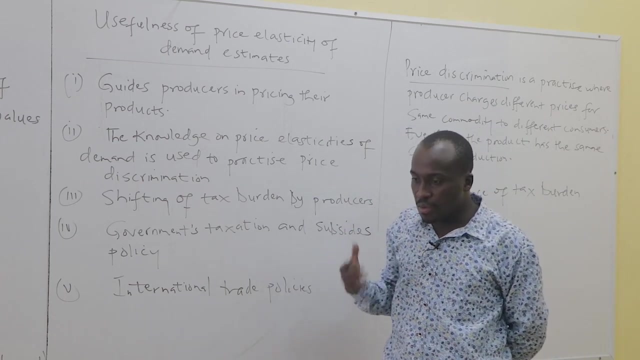 iv: government taxation and subsidies in the area of government too is a very good for government too. government decides on taxes. okay, if i want to give taxes and subsidies, if i want to tax which commodity should i impose more taxes? if i impose more taxes on goods that are inelastic? 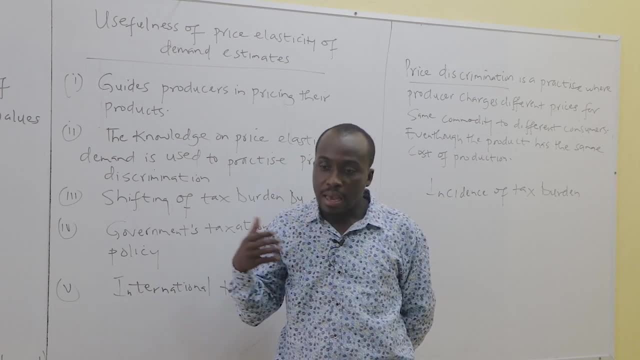 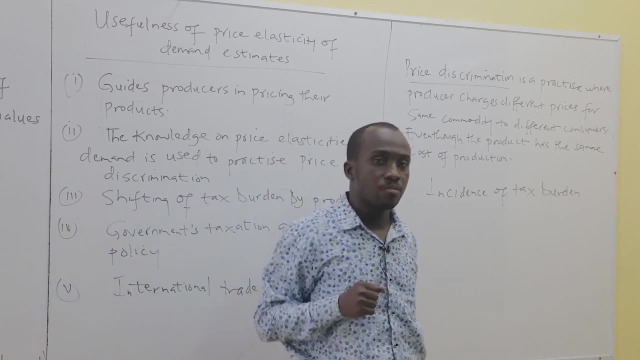 still they will buy. i'll make my tax revenue go away. and then let me post more taxes on goods that are inelastic so that i'll make my profit. impose less taxes on goods that are elastic so government is able to decipher which product is in the last. 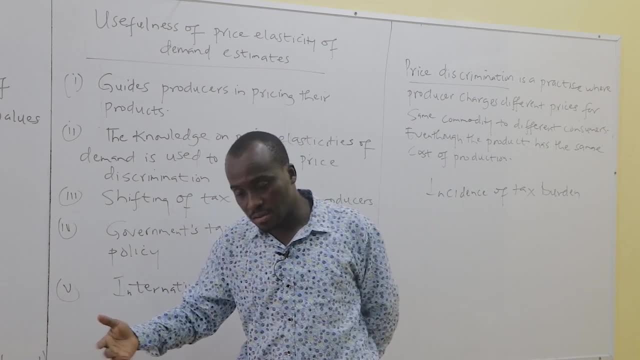 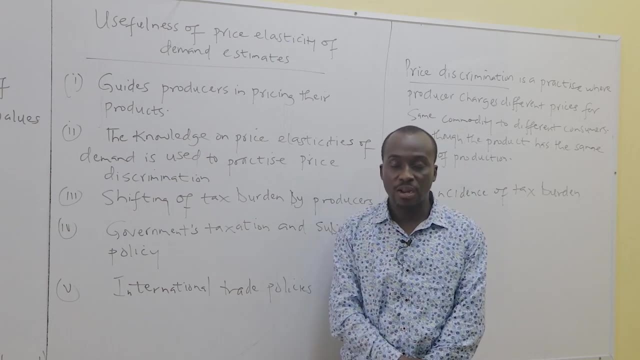 of that is calling them we put more taxes on it. they will still buy the product. which products are elastic? let me put less taxes? let me give you a trick example: in 2008-2009, during the media buy it read in ghana. the minister then said that all of the zero's character have setting. 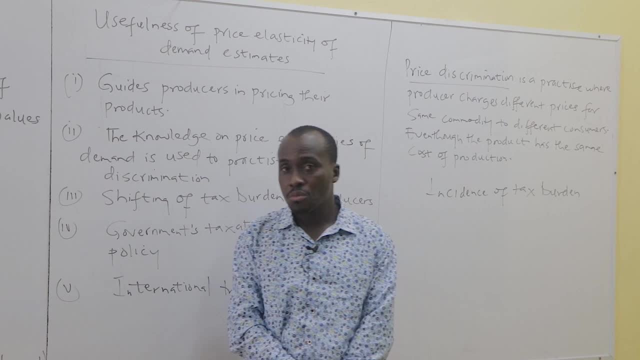 engines. they are imposing specific taxes on them and at the time of cards that we're mentioning were covered, were used by the worthy people who were worried in a society. so they, Baronร, imposed taxes on them where they know that drugs for話 to Chan mention in the warning to za the society. 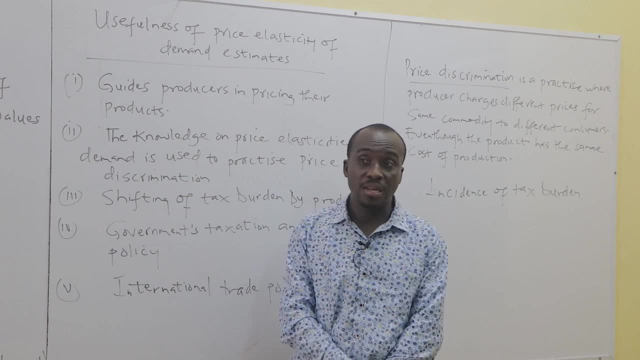 so they impose taxed on them where they know that their people are rich. people are people on the side are wave. the popular talking poetry is what the children are talking about. there are people who are rich men even without with a tax yesterday will buy and government do all those things very well. they look at the goods that are. 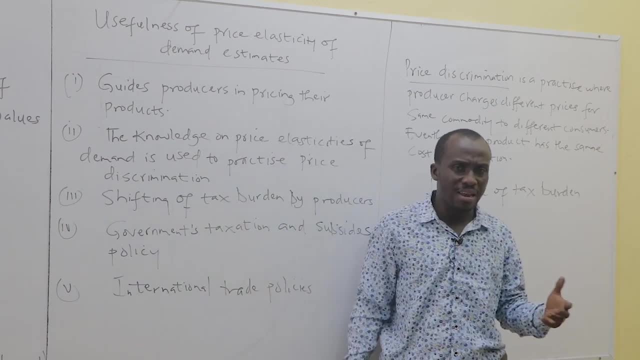 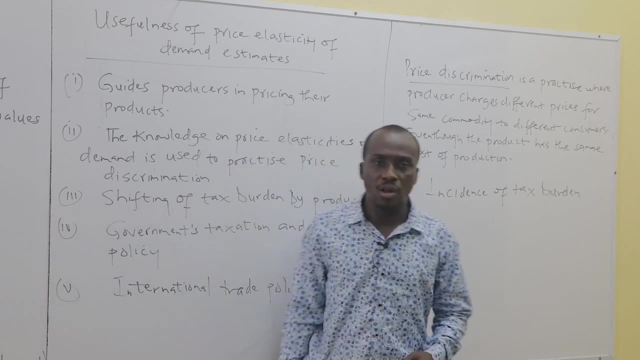 very inelastic goods that is demanded by people are relatively the the worthy class- they still put taxes on it yesterday- will buy in america, for instance. they are planning what they call the wealth, the wealth tax, where the wealth tax people who are, who are millionaires and billionaires. they 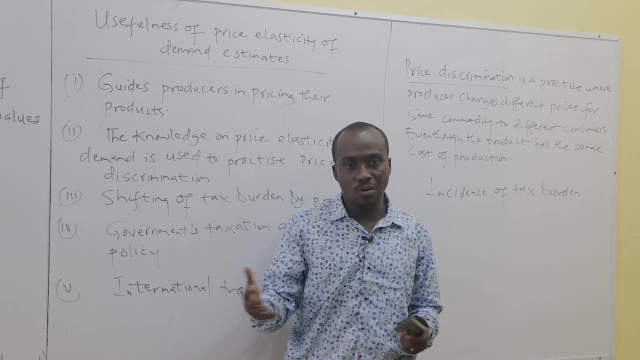 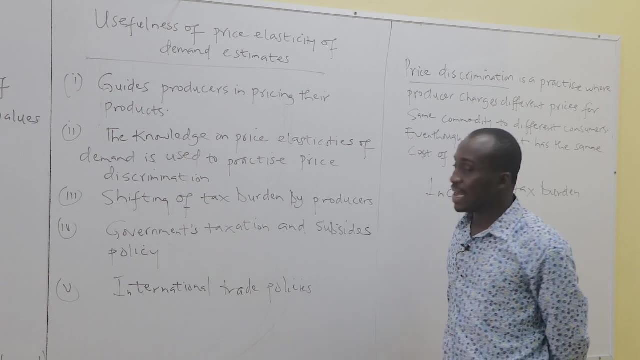 want to impose taxes on their world right. so they think that they will still be moving on because they have a lot. people have about 100 billion dollars and they can still be moving on. if your company has elastic demand, the government might decide to be very careful. 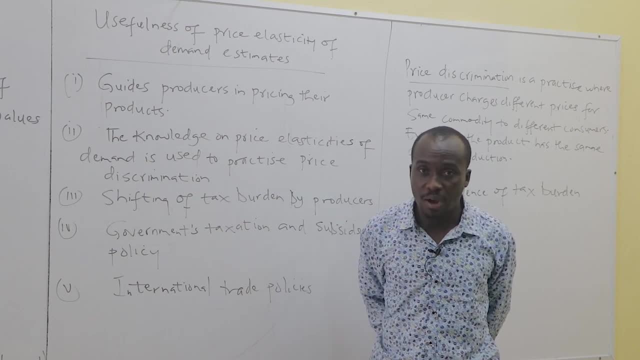 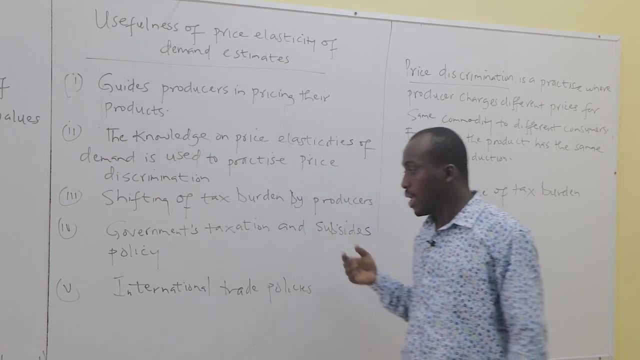 imposing type or taxes on it, because if you post too much, people will not buy. the government will lose. if people are not buying the product, government cannot make the revenue he wants to make. if government want to make, if government want to give us subsidies, what are subsidies? subsidies are the opposite of taxes, right, that is, instead of government imposing amount on it, government takes a part in subsidy, government takes part of the cost of that production. for instance, you produce a product, the product is ten dollars. right, you want to go and sell for ten dollars ants? oh, go and sell for two. 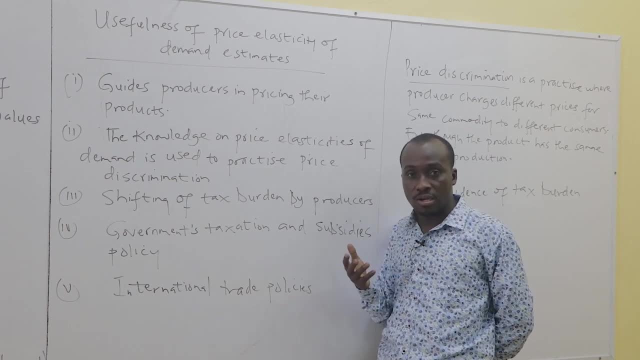 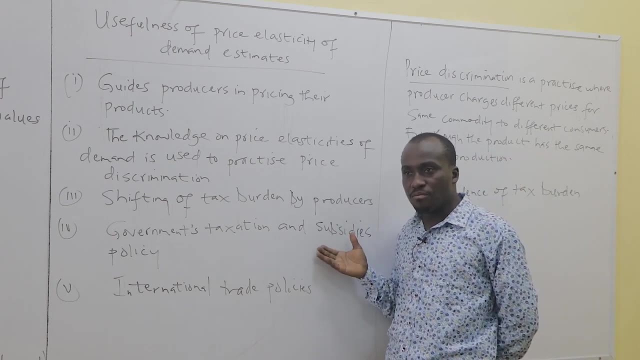 dollars, i'll pay you the eight dollars. so if you take part of the cost, so the goods will be very cheap. so that's the opposite of taxes. in subsidies, government can give more services to goods that have inelastic demand and basin but not sufficient generated good as a type of 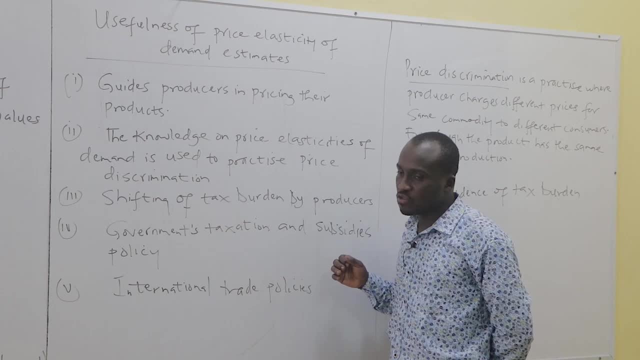 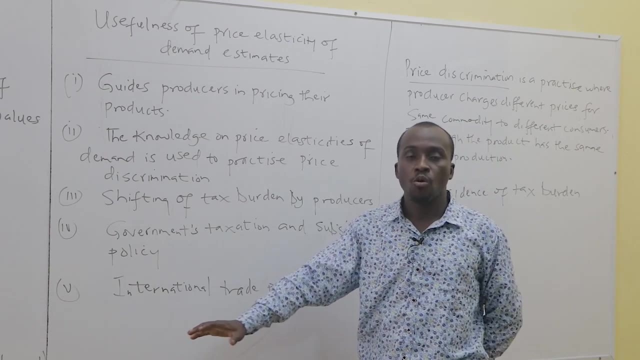 demand. right, Let me give more subsidies to goods that are inelastic, that have elastic demand. sorry, Government can give more subsidies to goods that have elastic demand. Why? Because government thinks that these are goods that are demanded by people when the price changes. 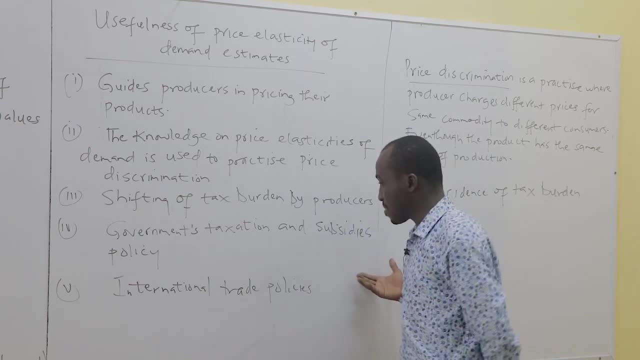 a bit, they will stop. So if I bring the price and they will buy, So government can give more subsidies to goods that have elastic demand, because when the price is good and they will buy more and maybe probably a lot of people demand those things. but people 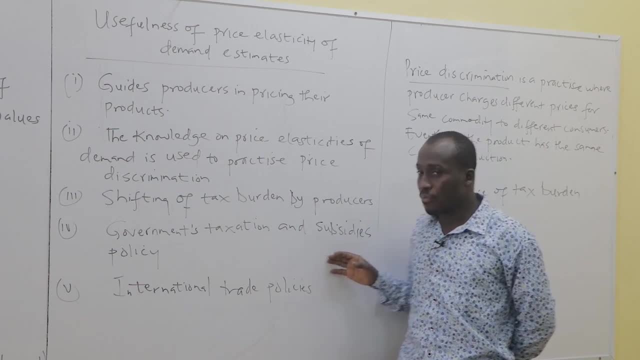 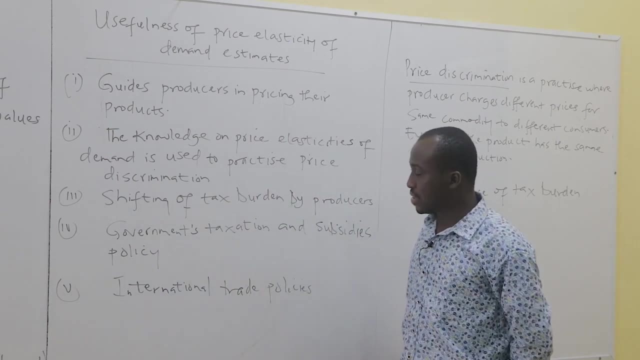 are maybe probably economically at a disadvantage. Therefore, if the price comes and they will buy more, for me that will propel productivity, production and export. In the same reason, in the same sense, government may impose less subsidies. government can impose less subsidies. 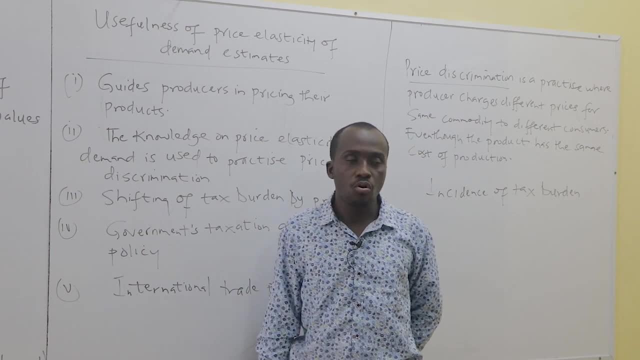 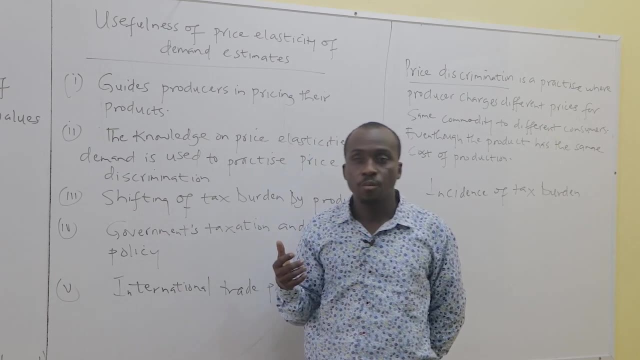 on goods that are inelastic, Because maybe government thinks that these people, even if the price is high, they will still buy, So there is no need to impose more subsidies. give them more subsidies on goods that are inelastic, So government can look at goods. 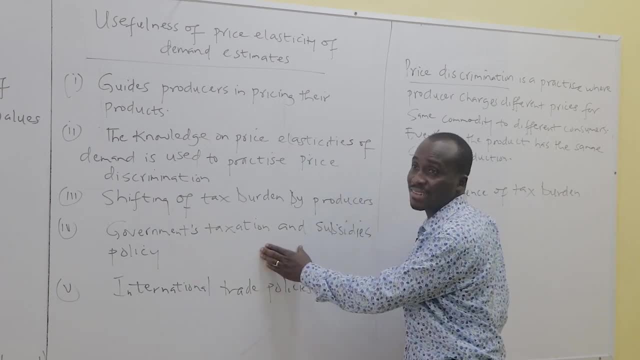 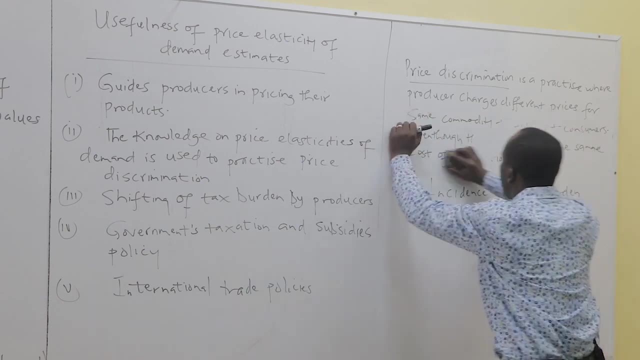 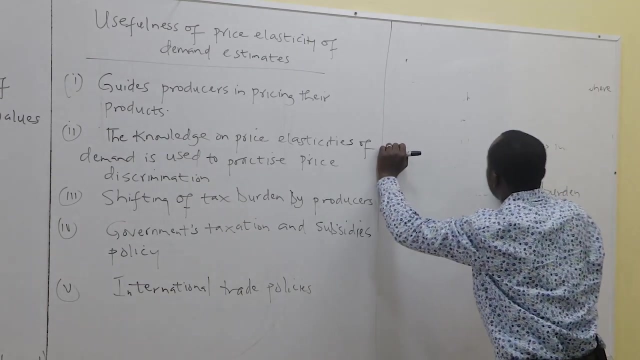 that are elastic, give them more subsidies, and goods that are inelastic, give them less subsidies Again. so when it comes to international trade policies, international trade government and international trade experts have to know your export and your imports. is it if people demand for? 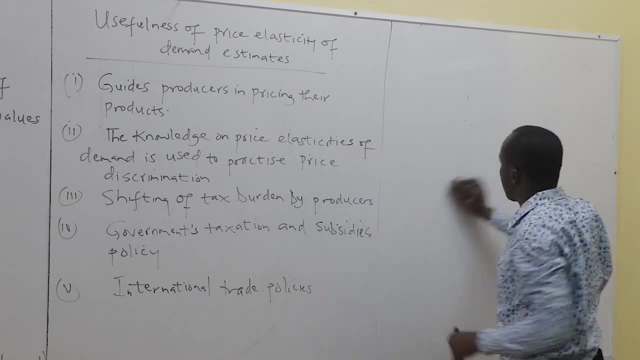 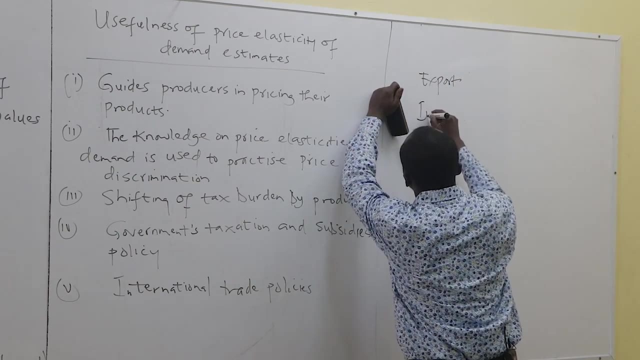 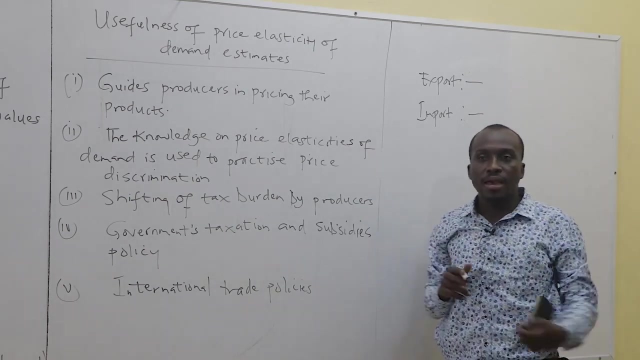 your export and imports. is it elastic or inelastic? right, If people demand for your export, let's say the country's export and your imports. is the demand for export elastic or inelastic? Ghana, we export things. we export cocoa to Beijing. the kingdom of chocolate to Switzerland. 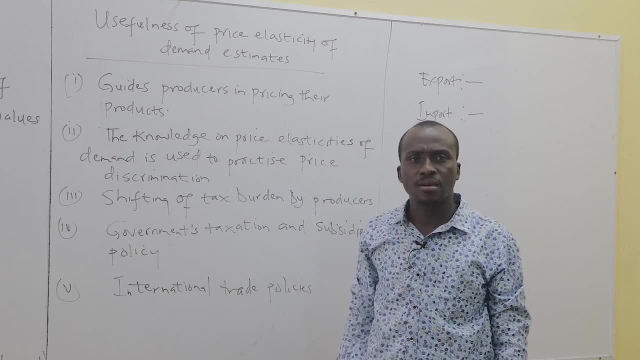 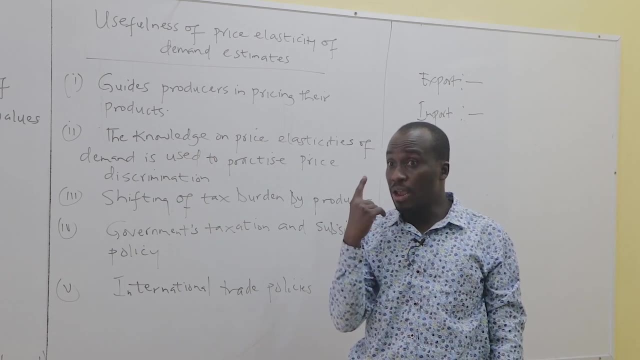 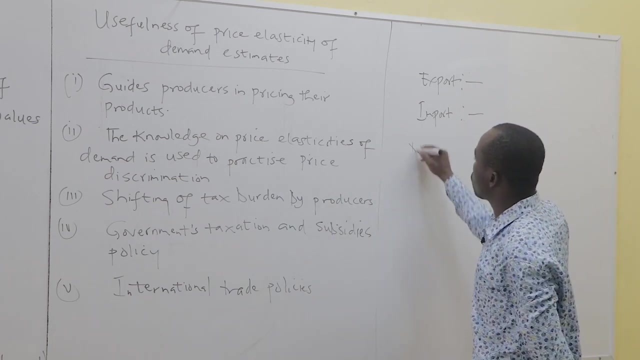 If the people in Switzerland their demand for cocoa. is it elastic or inelastic? We import goods, The things we import. is it elastic or inelastic? It's very important for trade policies, Why? Let me tell you why. We call something in the economy we call devaluation. 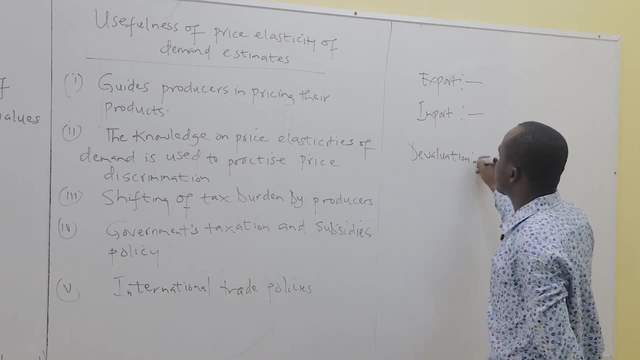 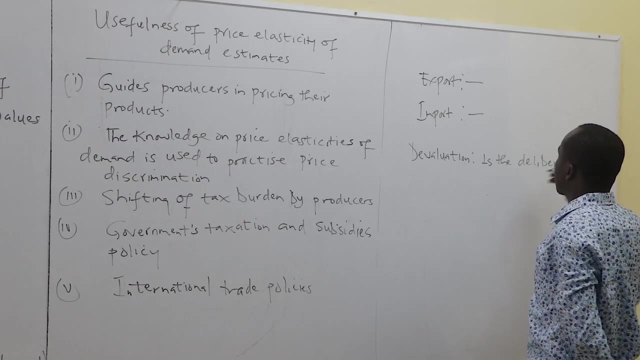 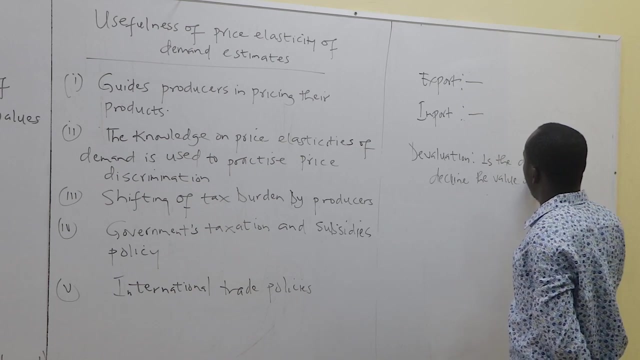 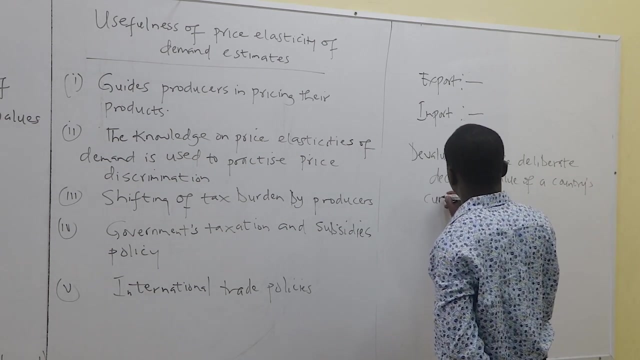 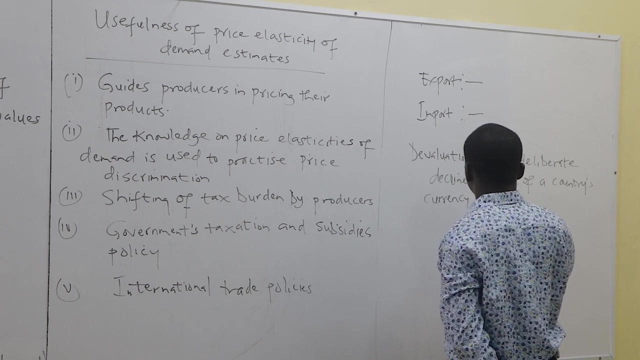 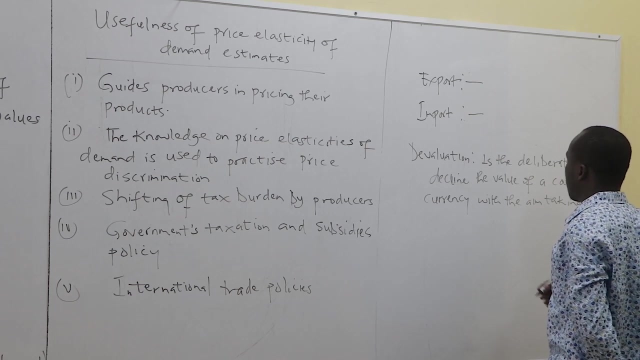 We call something in the economy, we call devaluation, Devaluation, Devaluation, Devaluation, Devaluation, Devaluation is the deliberate decline in the value of a country's currency with the aim of the aim, of the aim of taking advantage of trade. 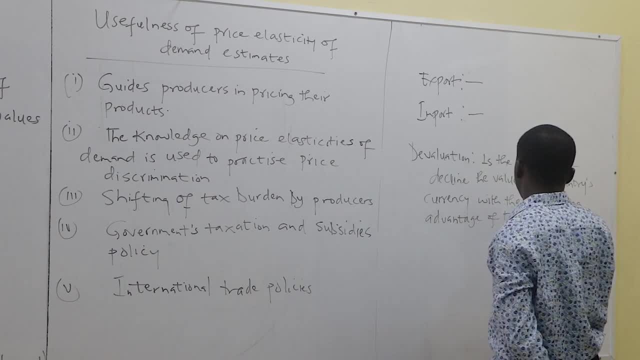 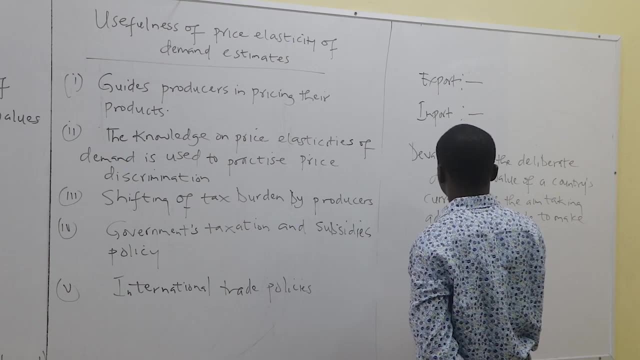 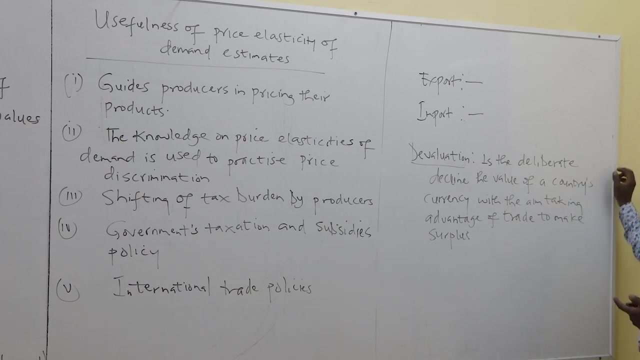 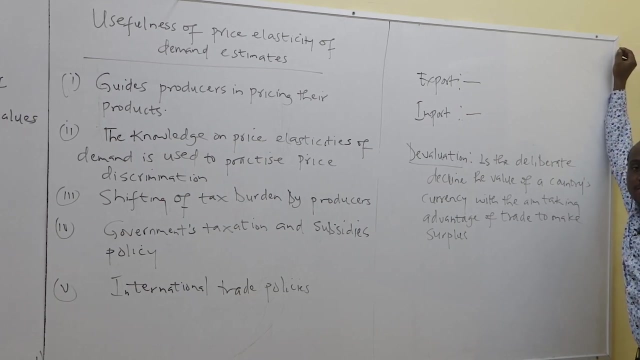 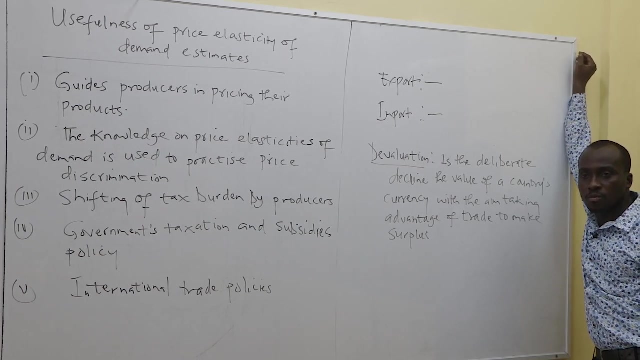 of trade to make surplus. So I said that it is very important for international trade policies. For instance, if you export, you should be able to detect: is my export? is it elastic or inelastic? What about import, The things my citizens, they import? is it elastic or inelastic? 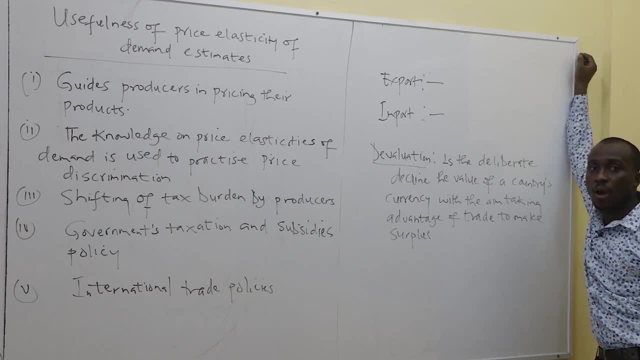 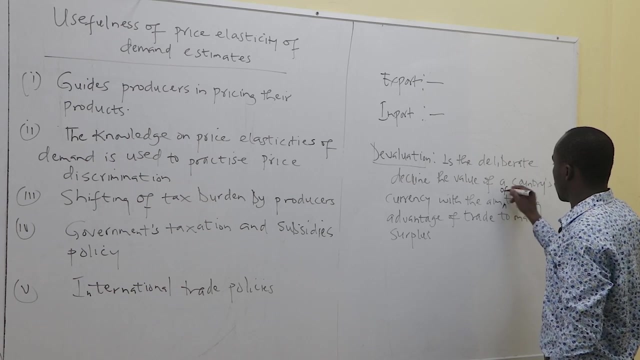 Why to take trade policies? One of them is what we call devaluation. What is devaluation? It's a deliberate decline in the value of a country's currency, with the aim, with the aim of taking advantage, with the aim of taking advantage of international trade to make. surplus, Why A country can intentionally devalue their currency. They will bring down the value of the currency. If four cities were exchanged for one dollar, the country said: okay, let's make it six cities to exchange for one dollar. That means you need more cities to exchange for the same dollar, right? It was four cities. It was four cities. It was four cities. You have six cities to exchange for one dollar. Now you have deliberately devalued your currency and made it six cities to one dollar. What it means? that now you need more cities to get the same amount of dollar. 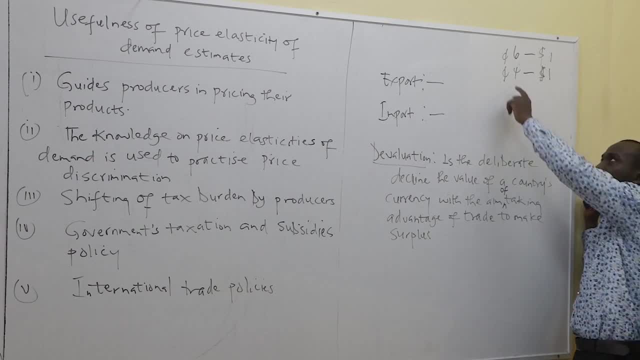 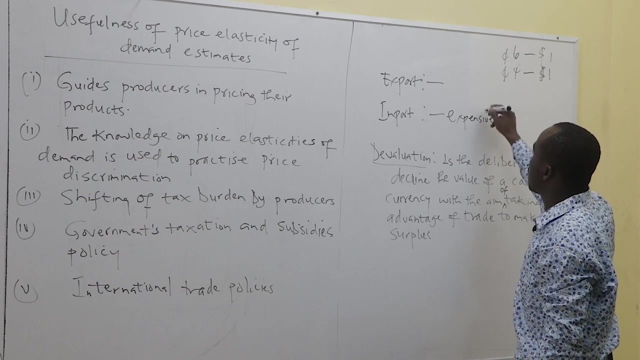 That means your country, the city have lost value. First you're using four cities to get one dollar. Now you're using six cities to get the same dollar. So that means your currency have devalued. When your currency devalue, it makes exports expensive and imports cheap. 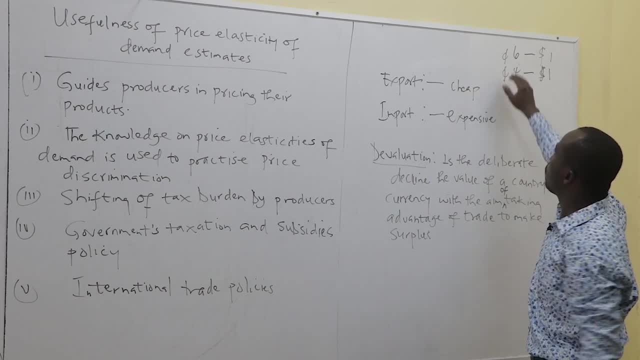 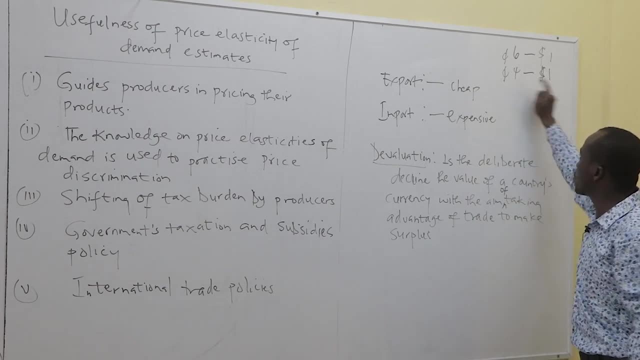 Because people need more cities to get the same amount of dollar to imports. So when they import they become very expensive. First, when you have four cities, you can get one dollar. Now you need six cities to get one dollar. That means the value have fallen. You need more to get the same amount of money you were getting. Right, You need more cities to get the same quantity If you need $100,000.. First, you're using 40,000 cities to get $100,000.. Now the value. we have lost value. So now you need- you need 600,000 Ghana cities to get the same amount of money you were getting Right: 600,000 Ghana cities to get the same $100,000.. 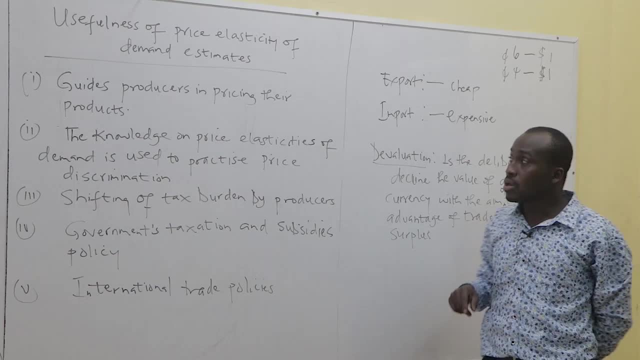 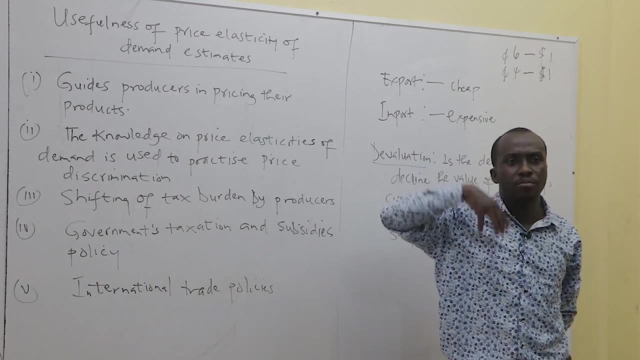 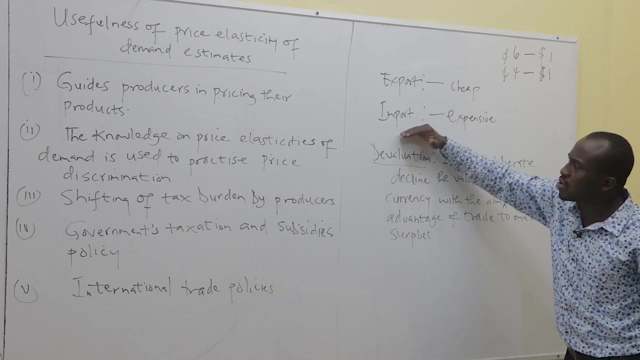 That means the country's currency have lost value. When that thing happens, what does it mean for trade? It makes your export expensive Because people will need more money to bring it, And when they bring it they will increase the value. Again, it makes your import expensive. 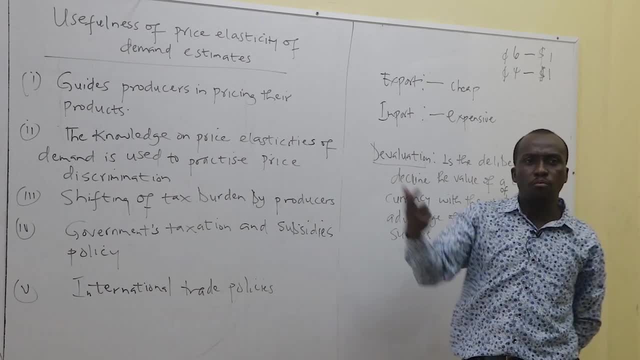 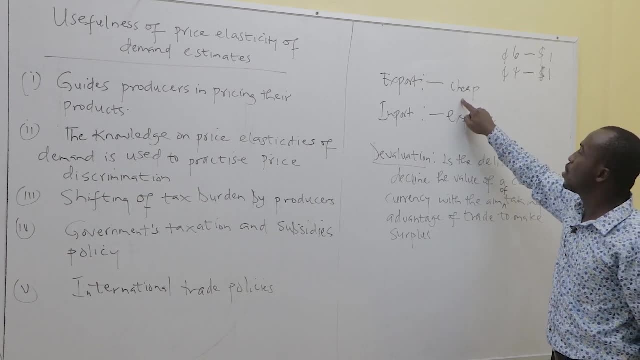 Why does it make it expensive? People need more dollars to go and import the product, And when they bring it, it becomes very expensive. What about your export? Your export becomes very cheap Because even now I export things to Europe. When I come, I will make more money. 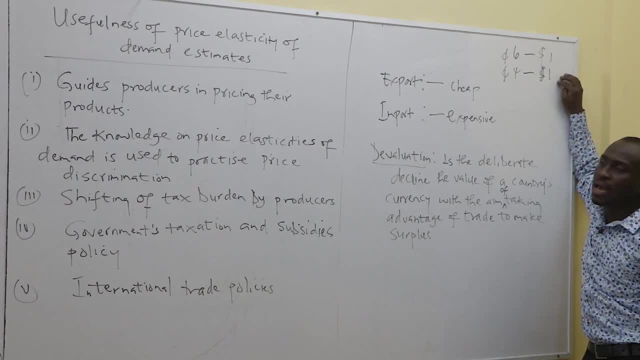 If I go and make first, when I bring $100,000, I was making 400,000 Ghana cities. Now, because the value have devalued, when I bring $100,000, I'm going to get 600,000 Ghana cities. 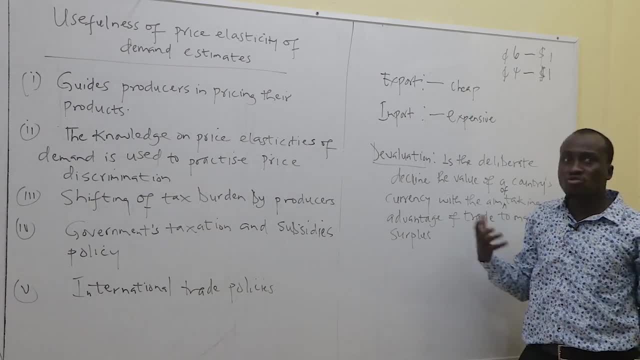 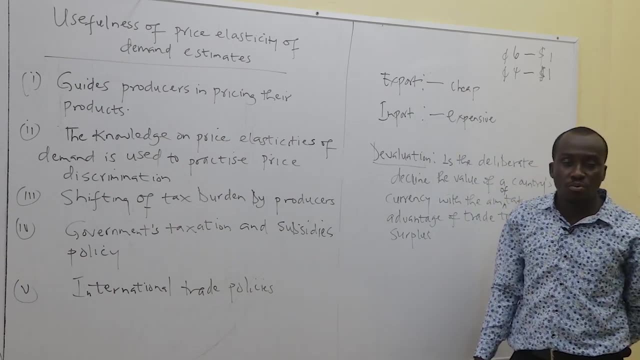 I'm making more. So even producing can produce more and even reduce the cost. So you make your export cheap In your eyes of international market. your export becomes very cheap. Your export becomes very cheap. Your import becomes very expensive. When this happens, it's good for you as a country. It's good for your country for two reasons. If the country produces more, that means you can produce more and make more trade surplus. Two, if the country's citizens, their demand for imports, is elastic, then it's good news for you. 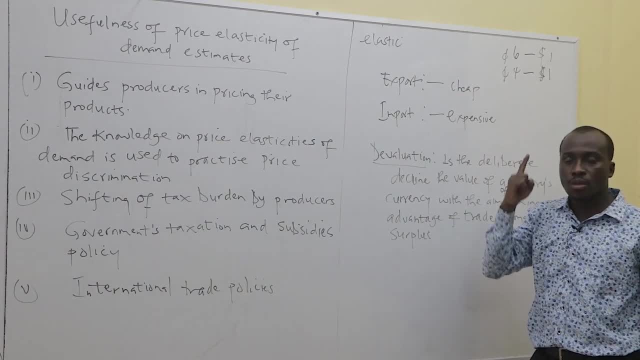 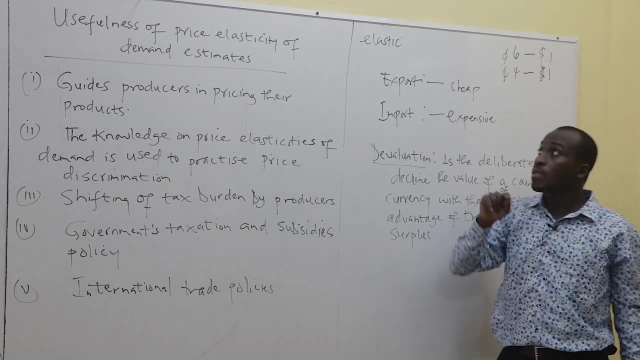 For a country to produce this and be successful. one: the country should be able to produce more So that they can export more, Because export have become very cheap. Two: import your citizens. their demand for imported goods should be elastic. Why? So that when the price becomes expensive, they will stop buying. When the price becomes expensive, they will stop buying. It favors you, because you cut down importation, You save the economy. So for this reason, So for this devaluation to work perfectly, people demand for imported goods should be elastic. 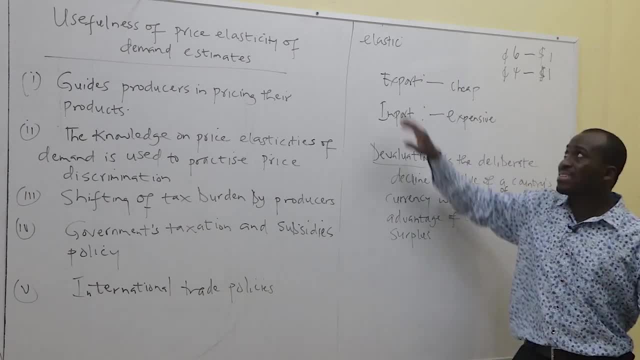 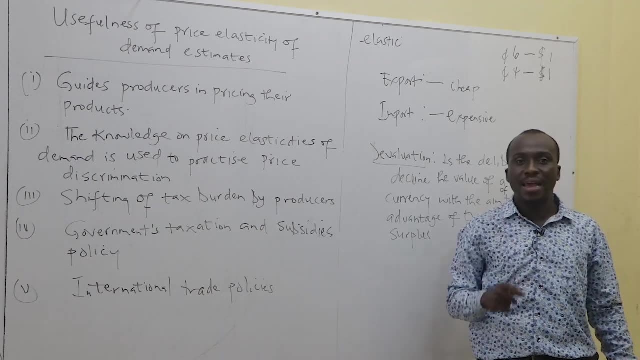 So that when they become expensive they will stop buying. You know that when a commodity is elastic, when the price goes up, a lot of people will stop buying So that it saves your economy from excessive import. But if their demand is inelastic, then you are dead. 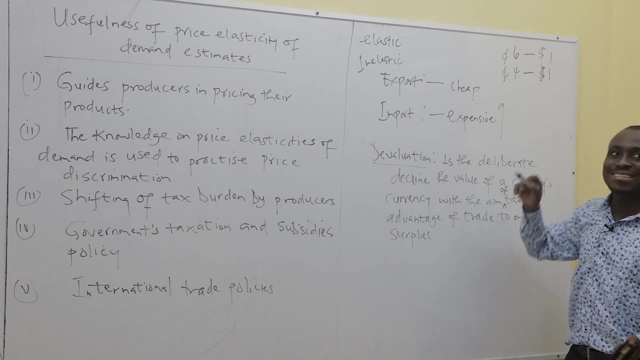 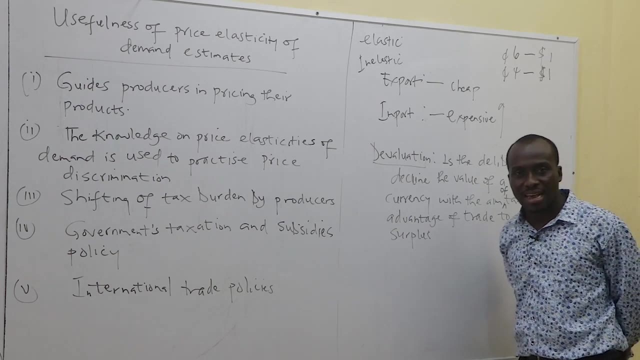 Because, even though it's expensive, just so do we buy more And that will even worsen your situation, Like in Ghana, when things that are produced in Ghana people don't like things that are produced in Ghana, Because everybody wants things from Europe. 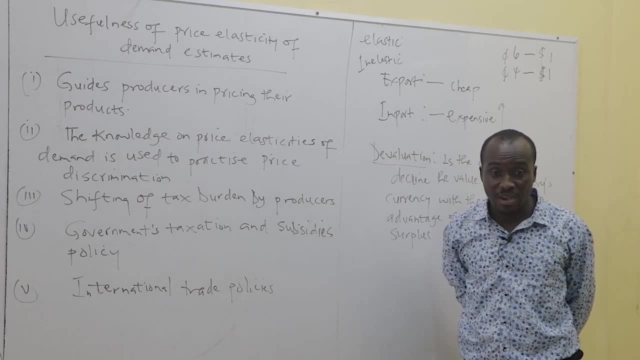 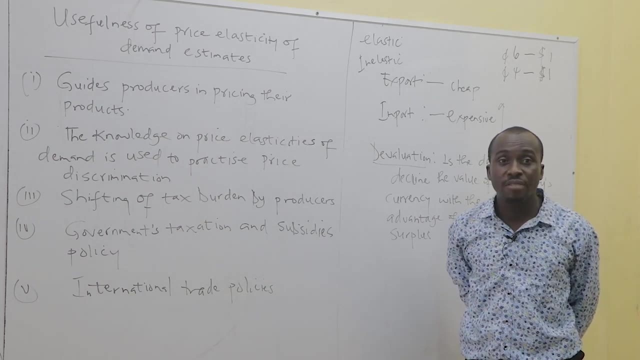 If the thing is produced in Ghana, no, They say, oh, it was made in Italy, it was made in America or Canada. Such people with that mentality, this thing will never work, Because even if it becomes expensive, they will buy more. 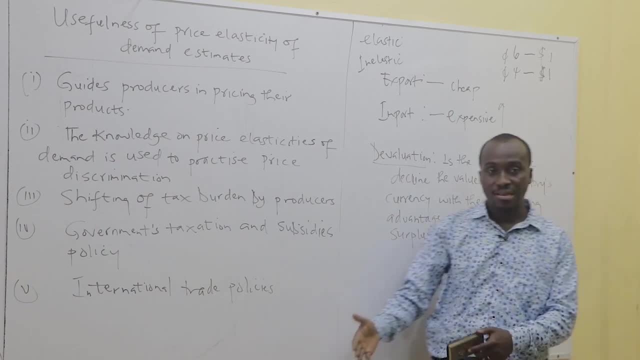 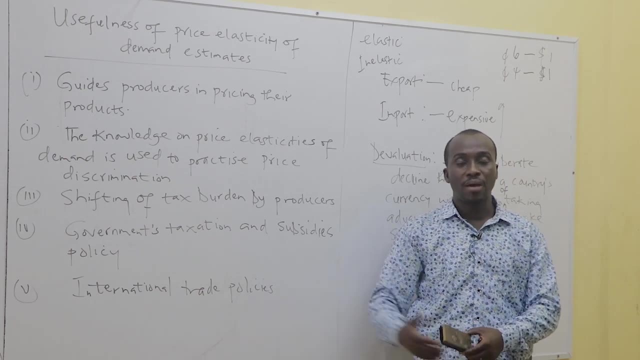 Because, even if the local product is there, they won't buy a foreign product Because they feel that the foreign product is better. People produce things that are quality, Yes, so people go and buy foreign products. Last time in parliament around 2014,. they were changing the chairs in parliament in. 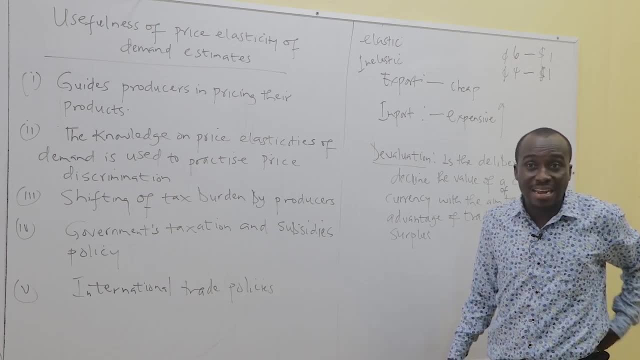 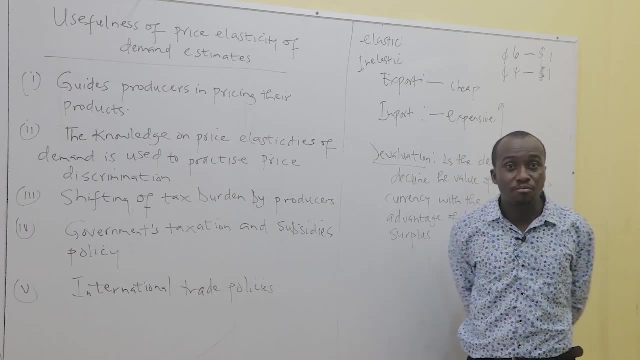 the parliament of Ghana, The ministers and other people. they wanted to buy the chairs from China. Wow, there are a lot of good Ghanaians that can produce chairs. This is the sort of Ghanaians you have. If you have such people, group of people, in your country and go and practice dibaluisi. 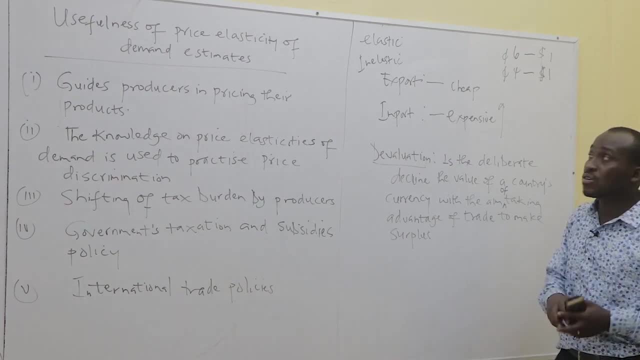 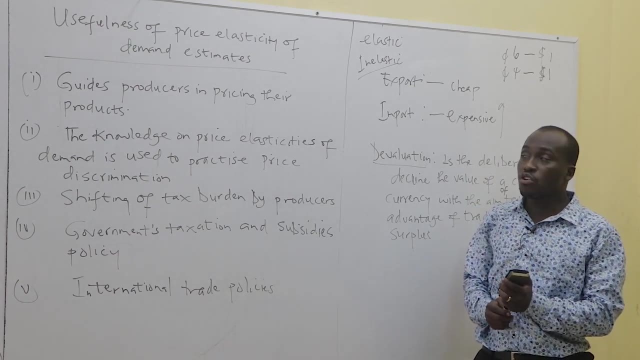 your import becomes expensive. Yes, so they will buy it, Because the demand for import is inelastic And that will worsen your situation. So for you to practice this system, for you to devalue your currency number one, you should be able to export more. 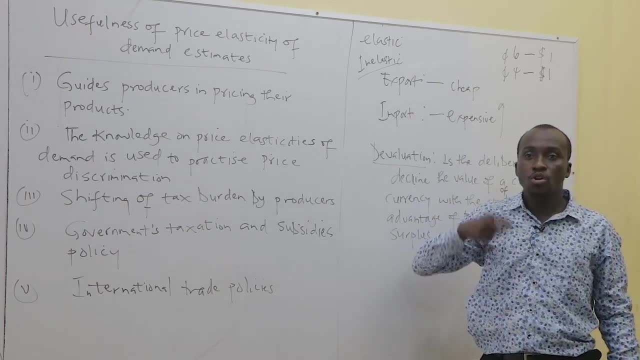 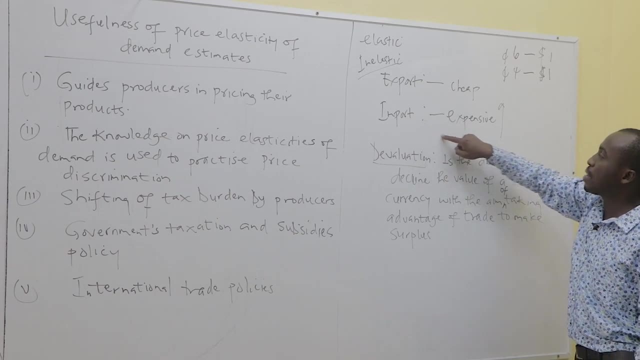 So that when the export becomes cheap, you export more and make more revenue. Number two: your demand for import should be elastic, So that when export goods become expensive, they will stop buying, So that they save the economy from excessive importation. 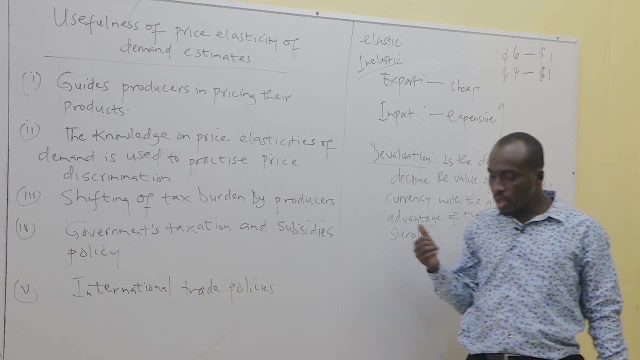 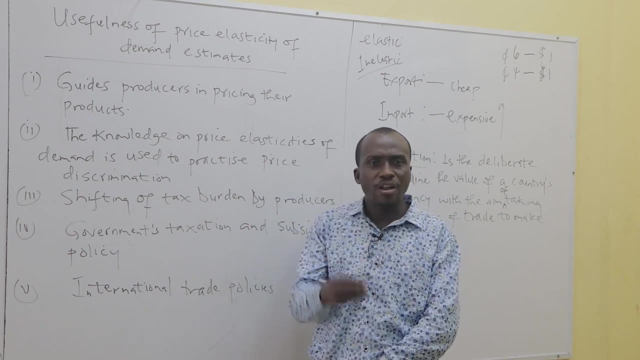 So you see that the concept of price as of demand is very important. It plays a sort of potato's role. It plays a sort of potato's role when it comes to understanding how the economy works: for international trade, for government tax revenue, for price discrimination, for pricing. 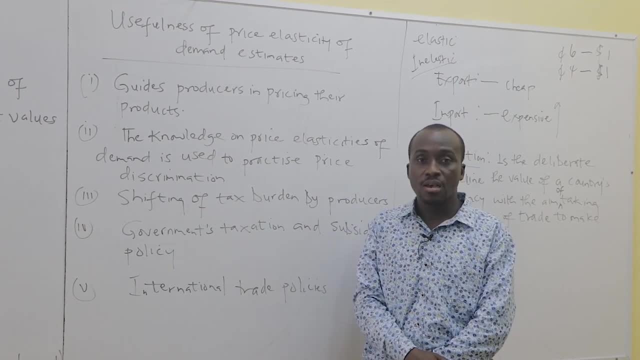 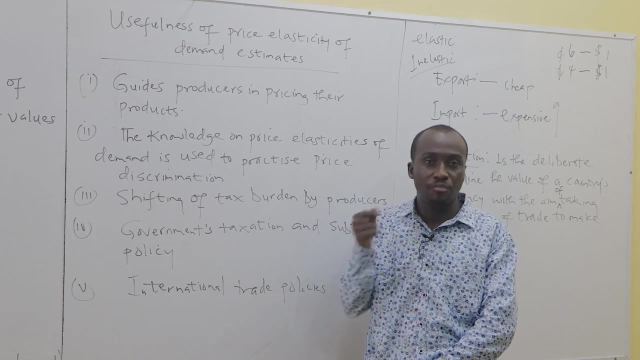 a product and for shifting of tax, tax burden, what we call incidence of tax, incidence of tax. So it's a very important topic for your life. The knowledge is for your life, It's not for writing exams and passing. You need the knowledge. 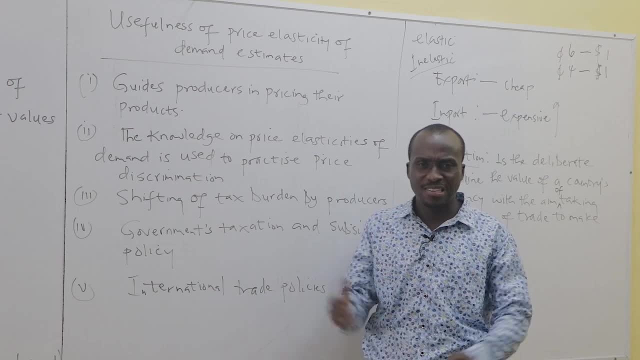 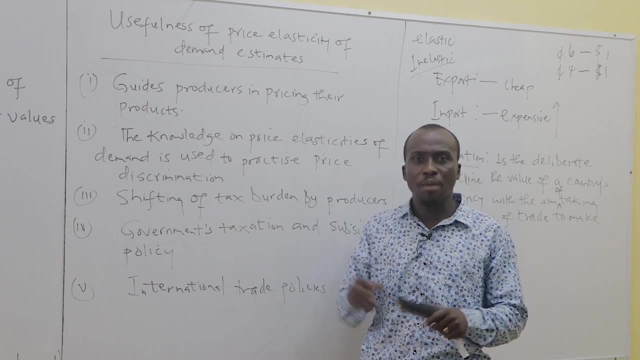 Maybe you might be one day going to be a business mongrel or this business tycoon or business magnet And you need the knowledge on elasticity so that you can stay very long in business. So thank you so much. We are going to look at the other type of elasticity. 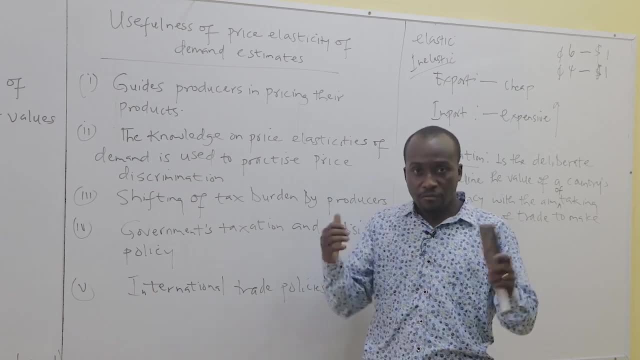 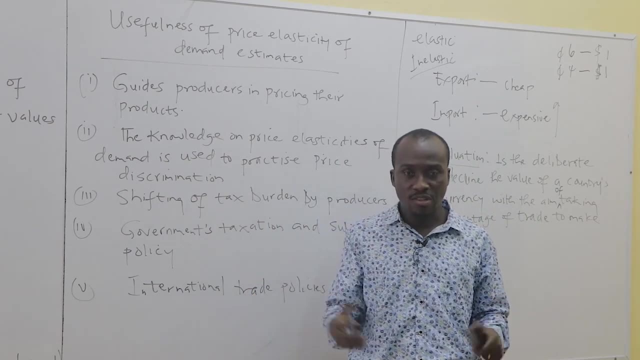 We are going to look at the income elasticity of demand. First, let me say that we have all these lectures on a pen drive. There is a 12-lecture out of the 15. Get a pen drive for yourself. Go through all this and get abreast of some of these issues.